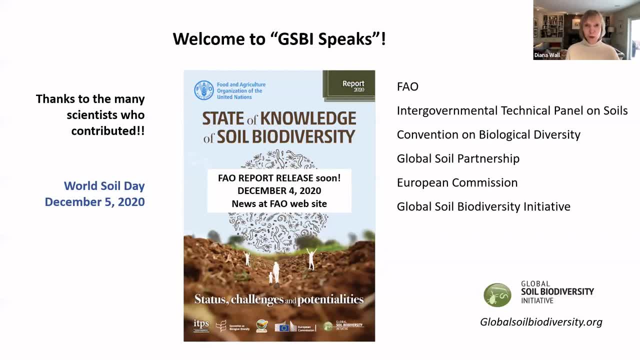 So, just before we get started, I'd just like to give you a few ground rules on how this is going to work. The chat room is not operating, so put your questions and your name in the questions and answers. Then also, we're going to record this video, this webinar, and you'll be able to get it and we'll let you know later when we have it up. 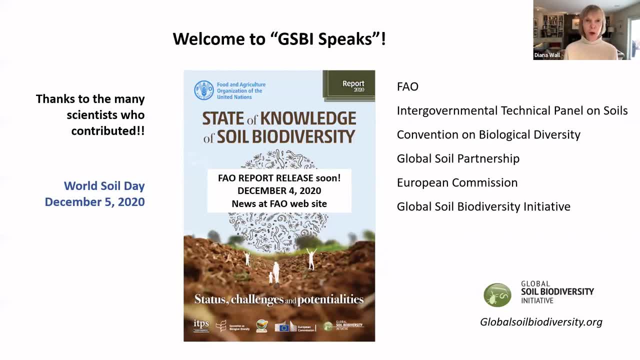 And so first I'm going to introduce Richard Bargett, who will introduce the panelists. They will go through about five minutes of remarks about the report and their involvement in it, and then we'll just open it up to everyone for questions and answers. 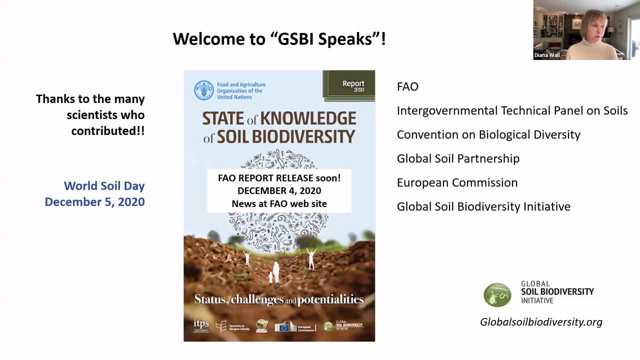 So be sure and put your questions and answers, And we apologize in advance if we don't get to every single question. We have a lot of people signed up for this webinar and we know there are going to be lots of questions And that would be pretty much it. 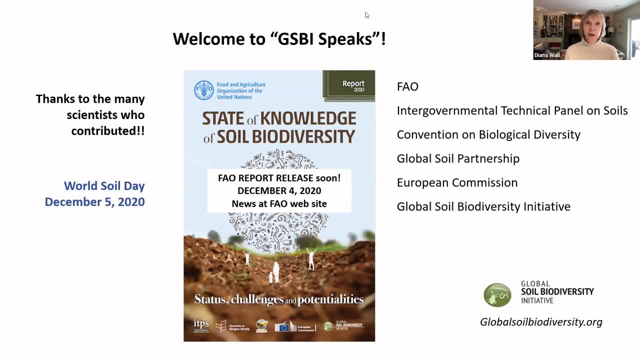 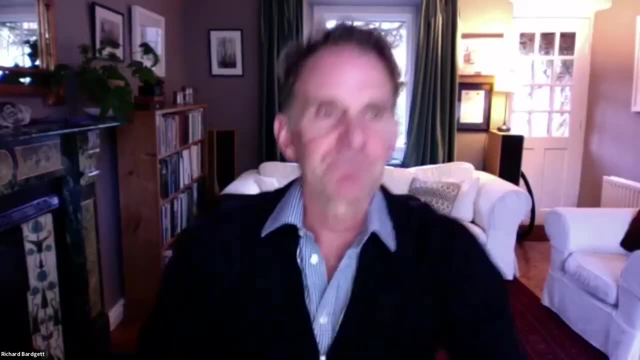 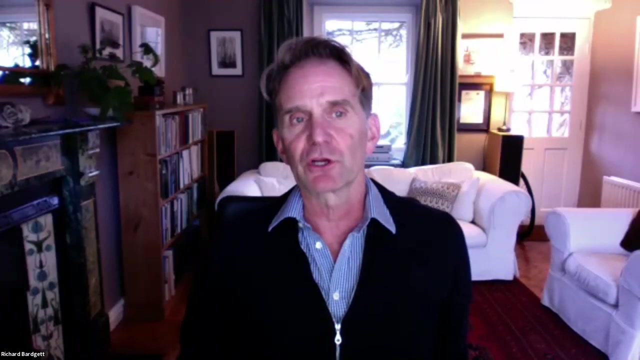 And so now I would like to invite Dr Richard Bargett, who is a member of the GSBI Scientific Advisory Committee and who will moderate this session right now. Thank you, Diana, and hello and welcome to everyone to this GSBI Speaks webinar, which is about the first global biodiversity assessment: from science to policy. 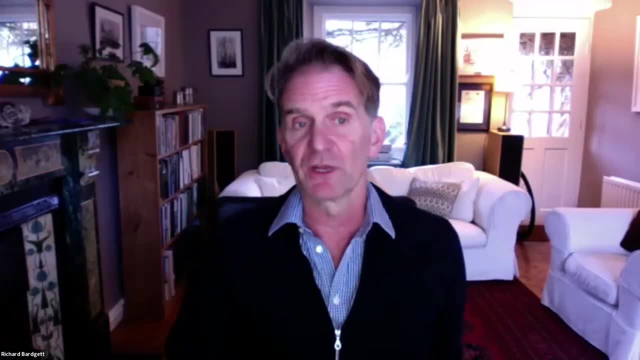 And this is actually part one of two webinars that will be running on the forthcoming State of Knowledge of Soil Biodiversity Report, which, as Diana mentioned, will be launched in conjunction with Soil World Soils Day on the 5th of December this year. 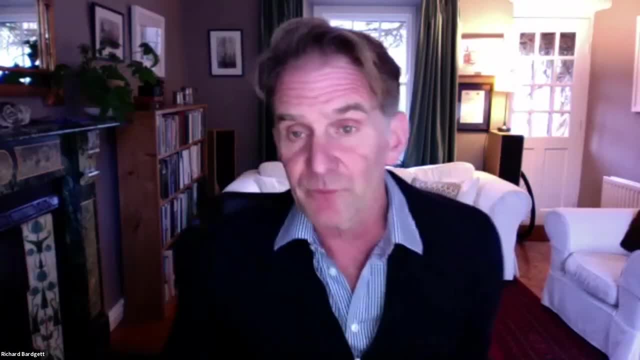 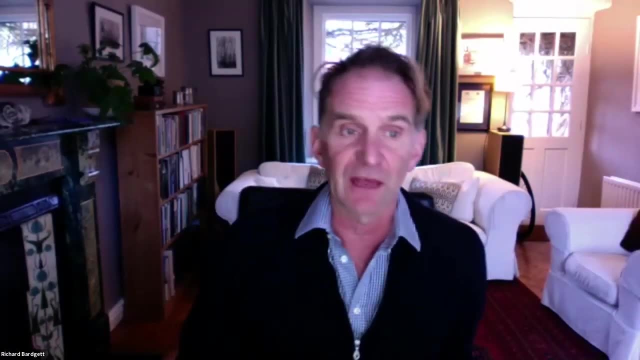 Thank you, Diana. Now on today's panel, we have four members. We have Kelly Ramirez, and Kelly is an assistant professor at the University of Texas at El Paso and she focuses on the diversity and distribution of microbial communities in the soil. 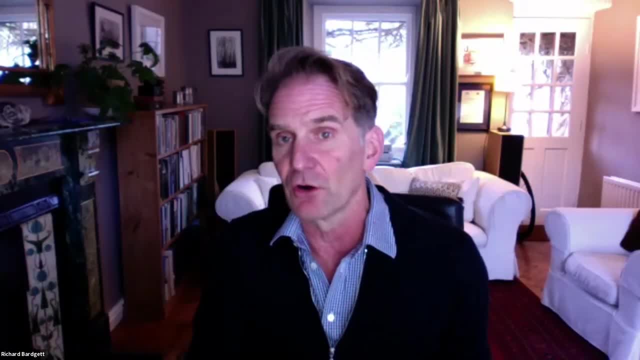 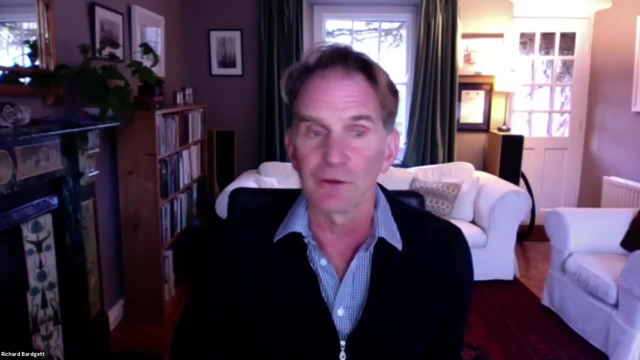 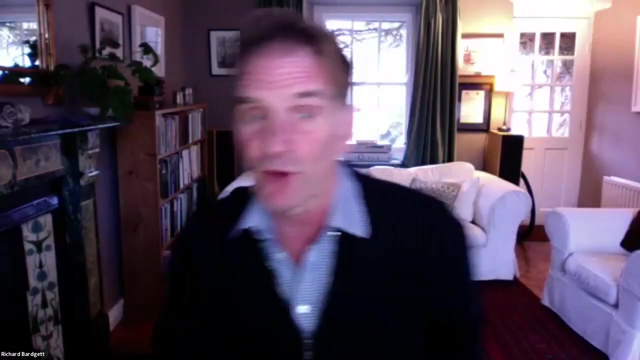 Kelly was also one of the managing editors of the report. We also have Elizabeth Bach. Elizabeth is an ecosystem restoration scientist. Elizabeth is an ecosystem restoration scientist. Elizabeth is an ecosystem restoration scientist And she works on tall grass prairie restoration, but with a particular focus on the role of the ecology of the soil. 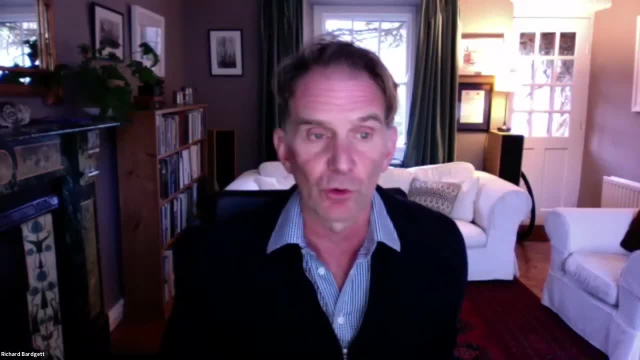 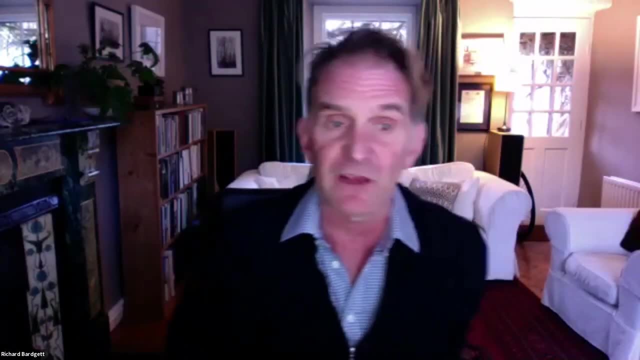 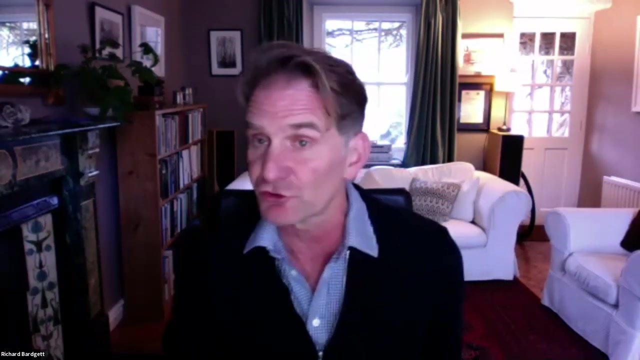 She was also a coordinating lead author on the report, so also had a significant role. We have Zoe Lindo. Zoe is an associate professor at the University of Western Ontario in Canada and Zoe specializes in the study of biodiversity and ecosystem function relationships in the soil system. 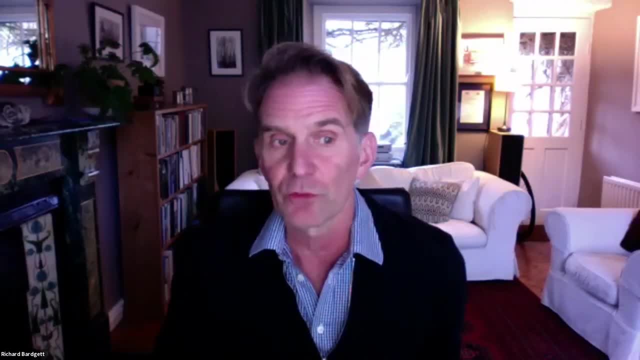 Zoe is an associate professor at the University of Western Ontario in Canada and Zoe specializes in the study of biodiversity and ecosystem function relationships in the soil system And she was also a coordinating lead author. And she was also a coordinating lead author. And, last but not least, we have George Brown. 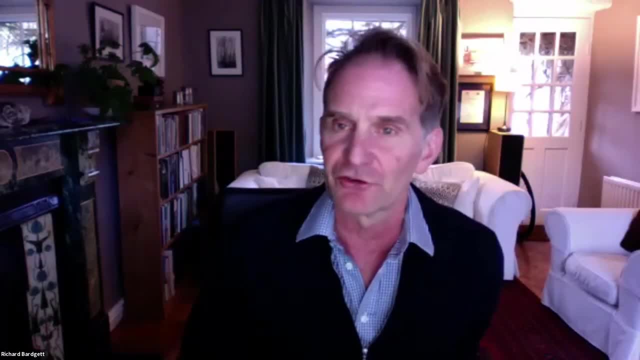 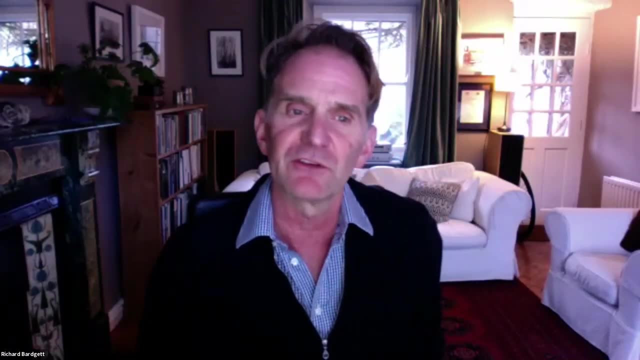 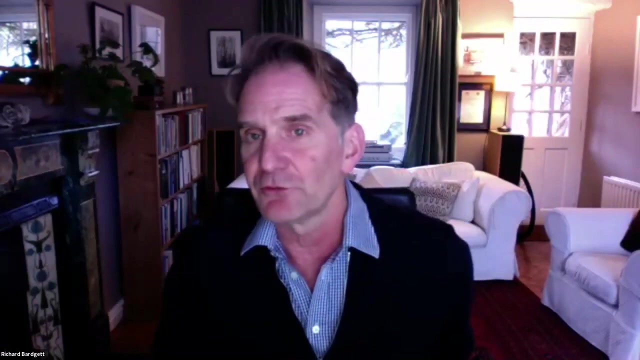 And George is a researcher at the Brazilian Agricultural Research Corporation in Colombo and he's also a professor at the Federal University of Parana in Brazil. And George specializes in the Earthworm ecology and was also a coordinating lead author. Now Dinah set a few ground rules. 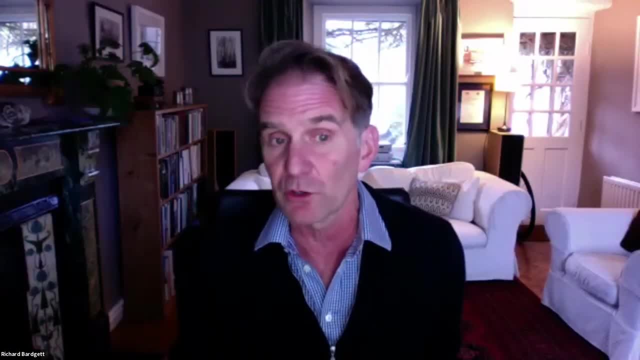 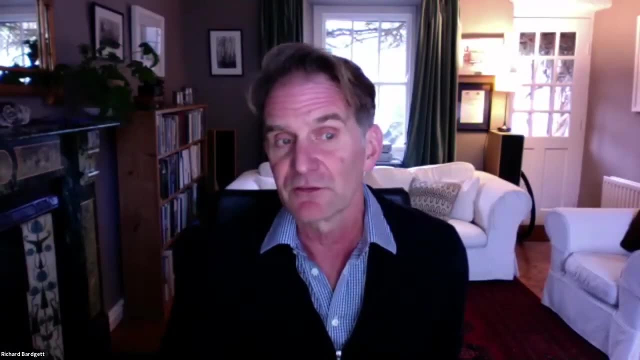 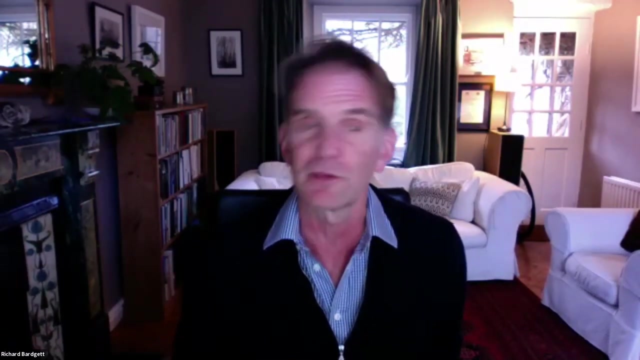 And we do have a very large order audience and after all the panelists have spoken for five minutes, we ask you to engage through the Q&A system to ask questions, which I will then direct to the panelists. Now again, as Diana said, we have a lot of people in attendance so we simply won't be able to answer all questions, but I can. 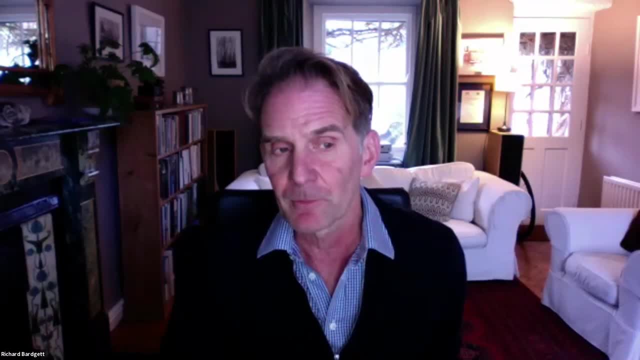 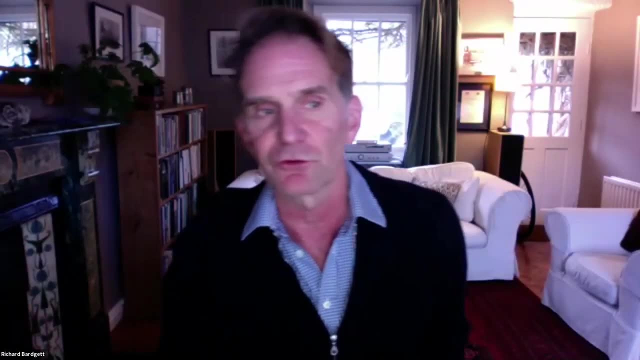 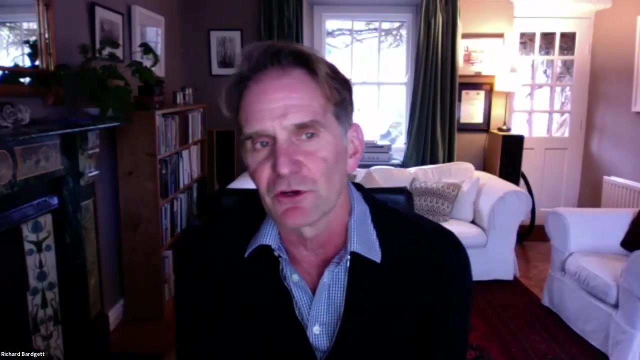 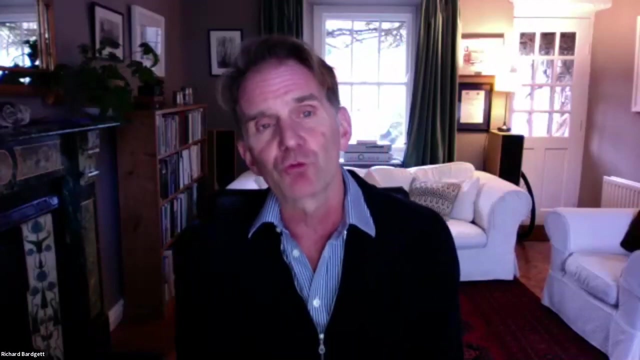 assure you that we will do our best. Now I just wanted to say a few words about the report and just the background, general background- to this area of research, because soil biodiversity is an area that's very much out of sight and out of mind and while scientists, farmers, gardeners have long 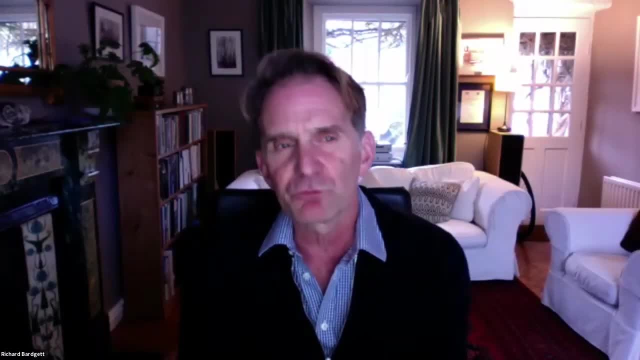 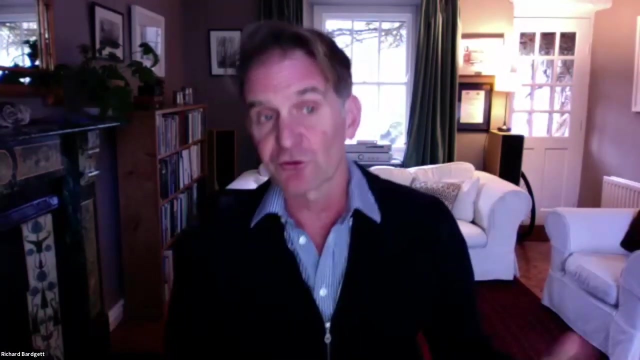 recognized the importance of a living soil. it's only really in recent years that we've began to fully appreciate how vast the diversity of life and soil is, and how important that diversity is is for a healthy soil. Indeed, the last two decades have witnessed what I would say is a 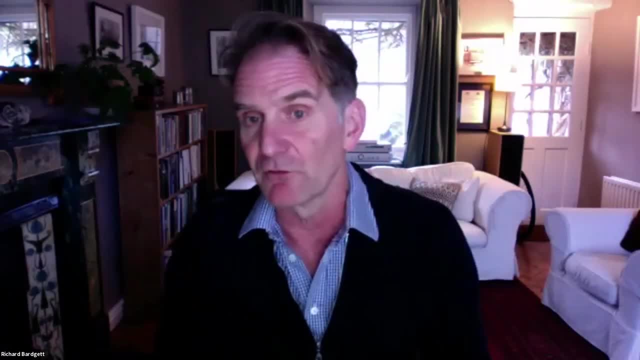 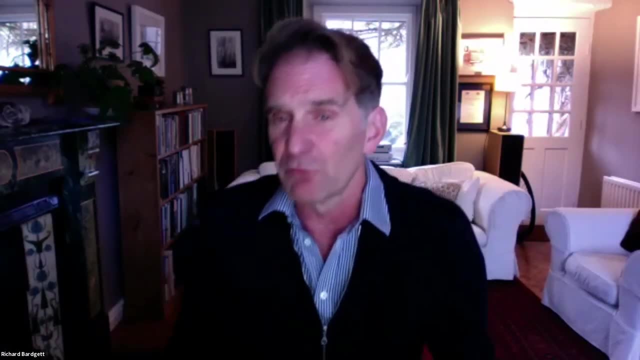 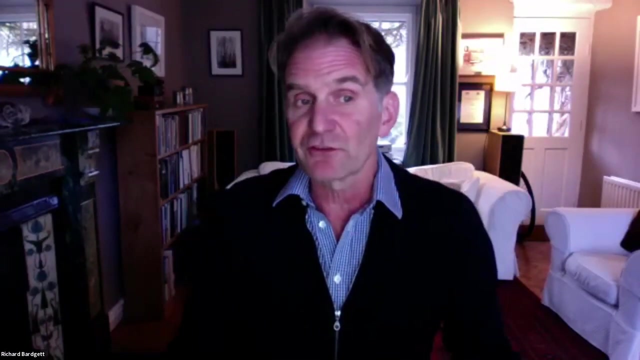 remarkable surge in interest in the study of the biological diversity of soil, and I think that's reflected in the GSBI itself, in that we have, I think, over 4,000 members from many parts of the world and as a result of that interest there's been major advances in our understanding about 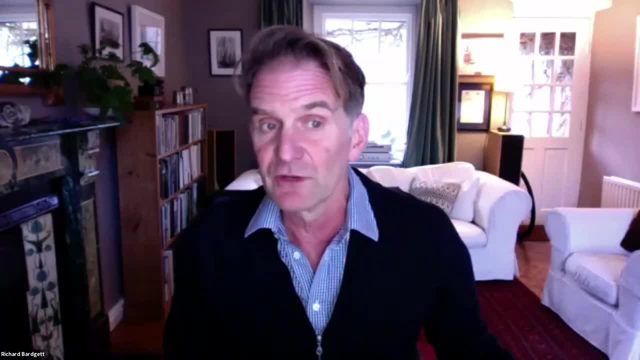 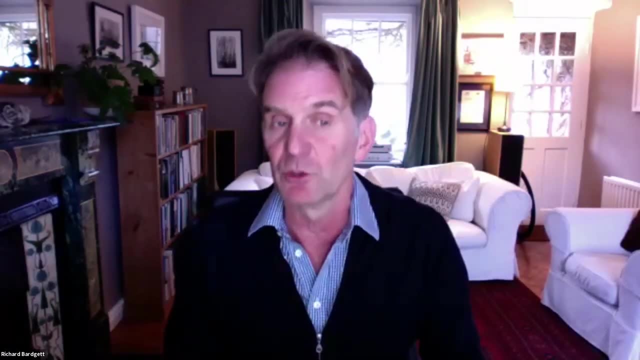 soil, biodiversity is distributed at different stages of life, and so I think it's important to understand that the role of soil, Of nature is actually very historically revealing. The size of soil is going to change over life. they change because they can действ seva different. 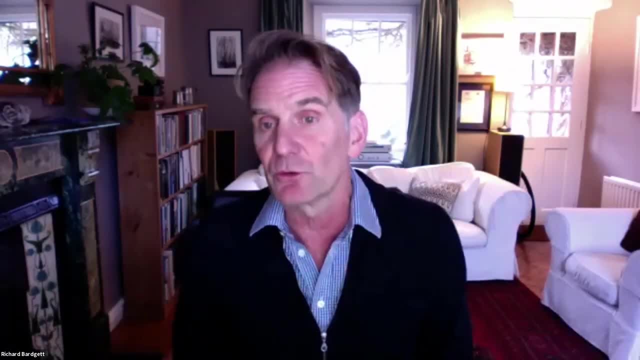 stages: How it is affected by social scales. how it is affected by global change, climate and land use change. how ES. how it is affected by global change, climate and land use change. how changes in the structure and diversity of communities influence above ground diversity: the plants, that the animals, that we can. 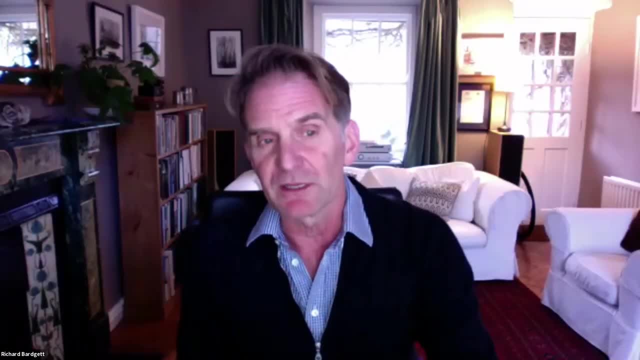 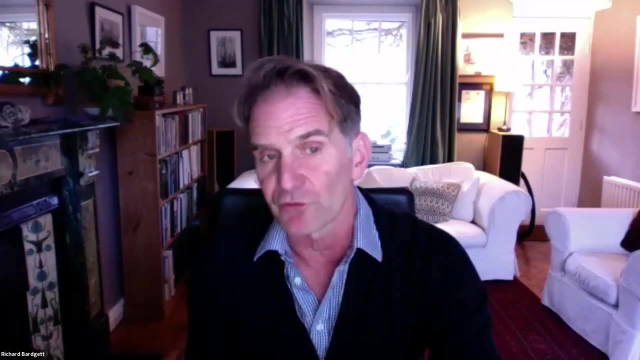 see above ground and also the functioning terrestrial system. Put simply, the study of soil biodiversity, I would say, is booming as a topic and there is now increasing awareness of the importance of soil life for a healthy soil and also the capacity of soil to deliver more crop name Meine. 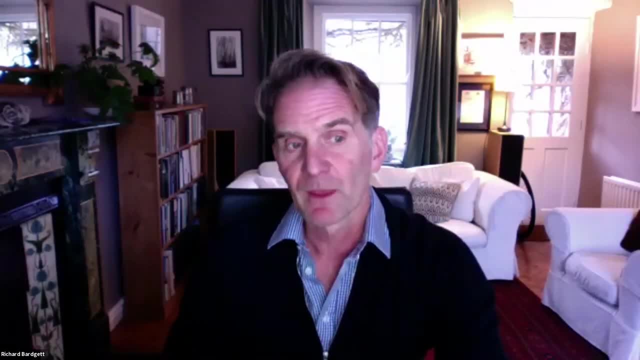 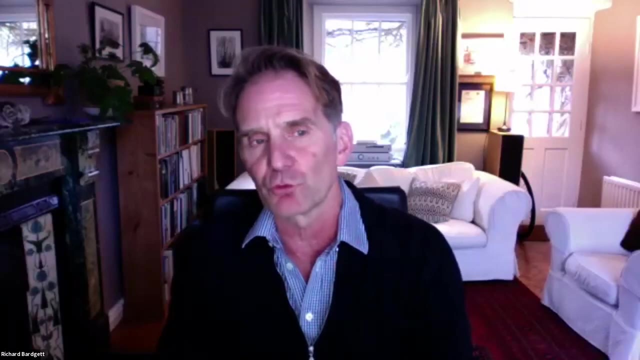 auch kein multiple ecosystem services. Now, this report, as Diana said, began from the GSBI. A small group of members felt that there was a need for such an assessment, And I just want to finish by saying why I personally think it's particularly important, And I've got four reasons I think. first, 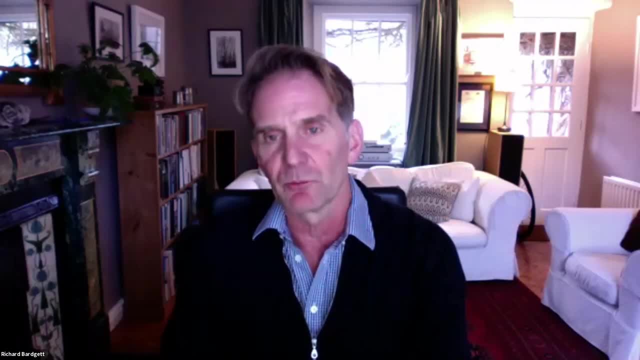 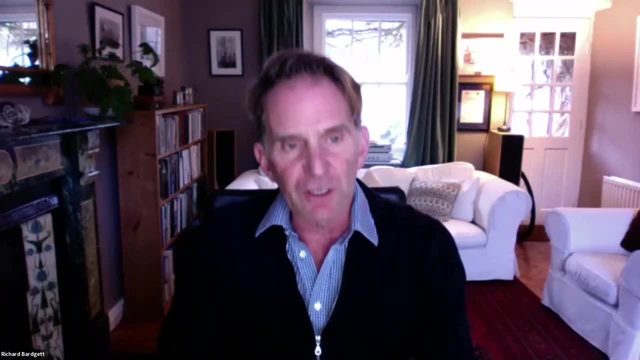 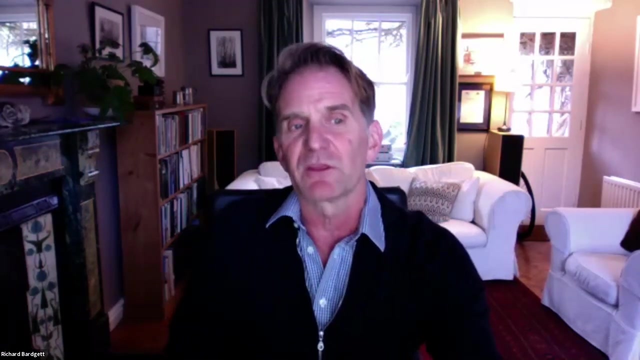 it represents a truly global effort by a large number of experts from all regions of the world. Second, we acknowledge that there are still major gaps in our understanding and knowledge of the diversity of soil, but this presents what is arguably the best available knowledge of soil. 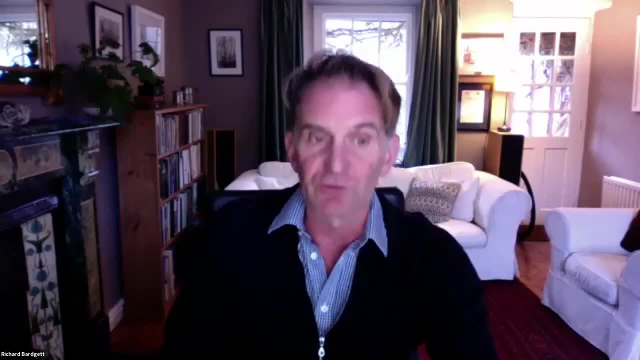 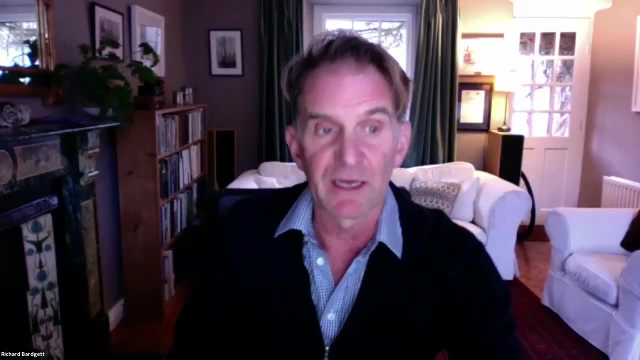 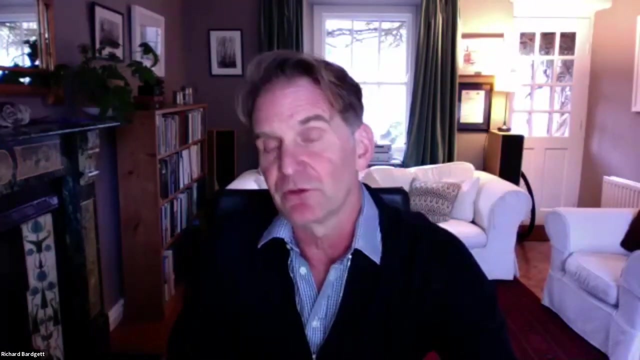 biota, the functions they provide and the services that they also provide. Third, it presents actions for the protection of soil biodiversity that we'll probably hear about and also solutions that soil biodiversity can provide related to agriculture, climate mitigation, medicine. 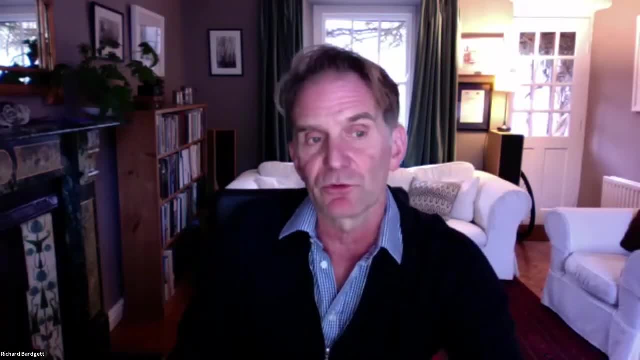 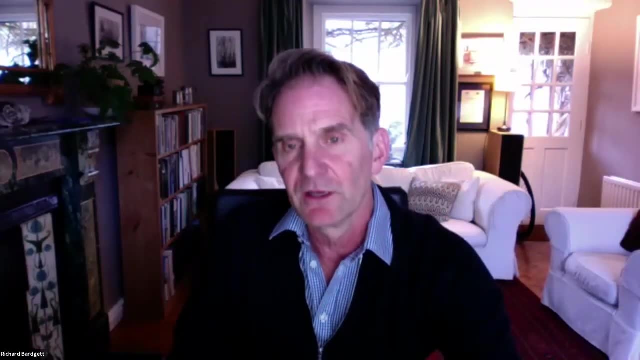 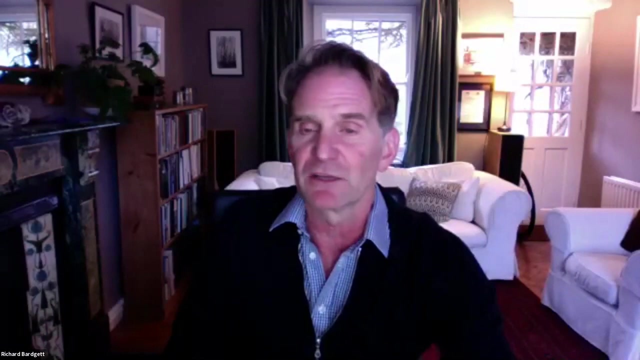 and the remediation of polluted soils. That's just some of the examples. And finally, one of the things we really hope with this report is that it will serve to raise awareness of the fascinating but hidden diversity of soil and highlight its fundamental role in providing solutions to many. 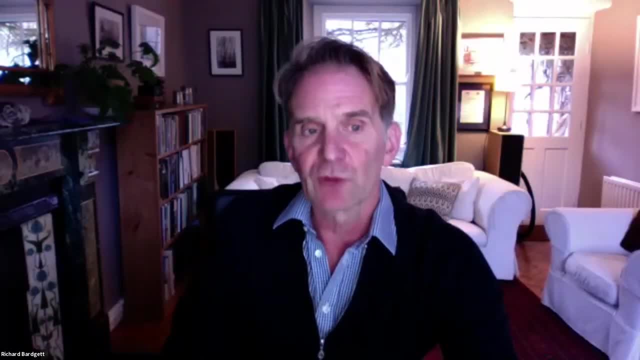 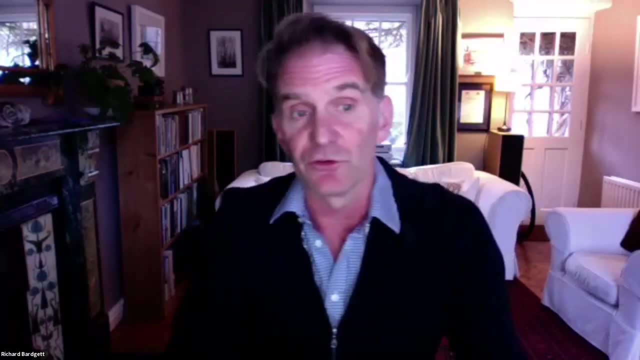 of today's global challenges. So I'm now going to pass over to our panellists, and what we're going to do is ask them to address three questions. What were their reasons for joining this effort? What are the main messages from the report, or their 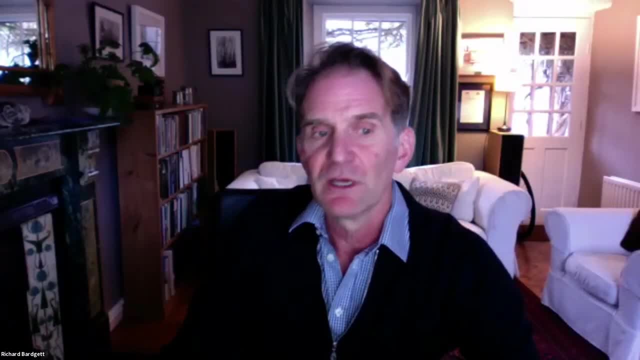 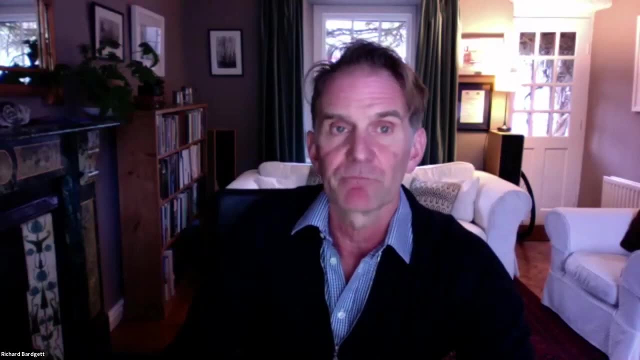 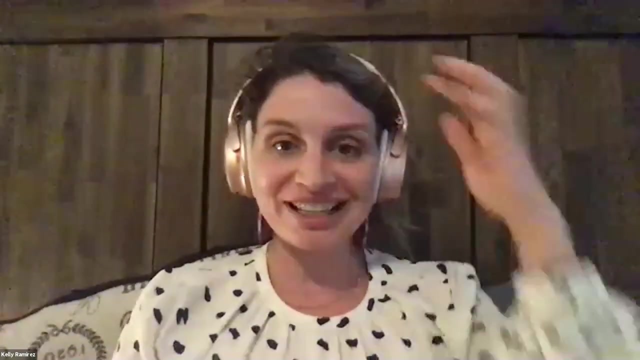 chapter, And how do they think this information will contribute or influence or shape soil biodiversity research and policy in the future? So with that, I'd like to now pass over to Kelly, Kelly Ramirez, who will give her first presentation. Hi everyone, Hi, thanks, You can hear me all right, Yeah, right, So I'm Kelly Ramirez. I'm 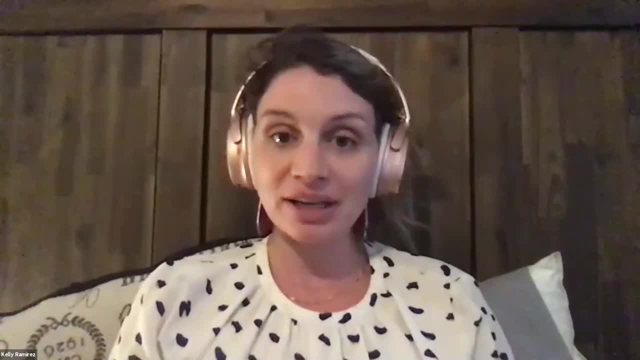 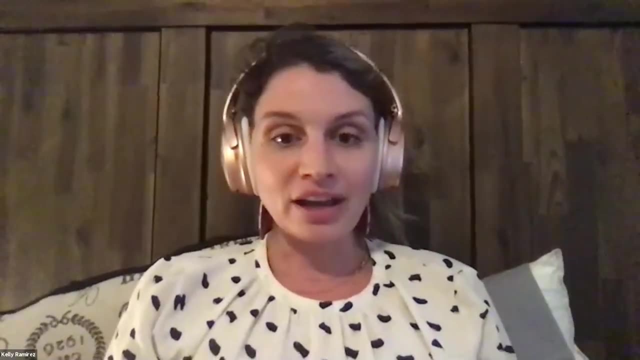 going to go a little bit off topic from the questions. just because I was the managing editor of the report or one of the managing editors and I didn't have one specific chapter that I worked on, I'm going to share some slides because that will help us pay more attention right when we switch. 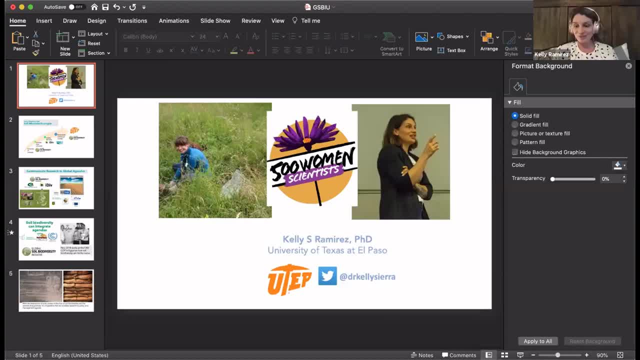 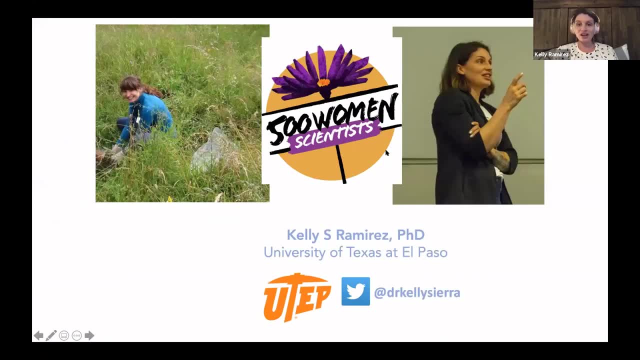 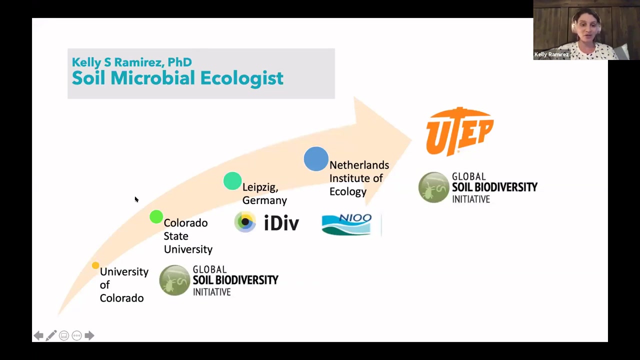 back and forth between things. Let's see Slides. Yeah, Okay, So right, I'm an assistant professor and I'm an associate professor at the University of Texas at El Paso now. My interest in soil biodiversity for policy began back in 2012.. So I got my PhD at the University of Colorado. 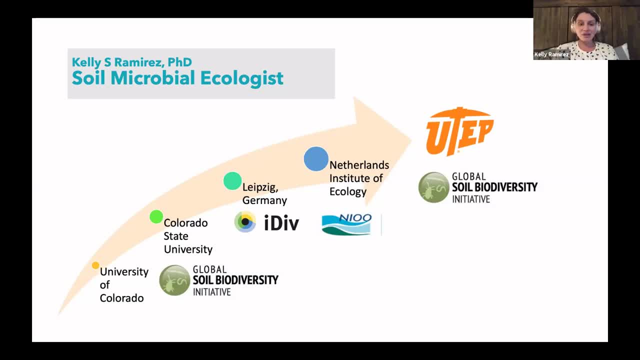 I did some really cool research there on microbial communities and soils And then I heard about this postdoc position that Diana had advertised for the Global Soil Biodiversity Initiative, And the aim of this program was to really put on the map with regards to soil biodiversity. 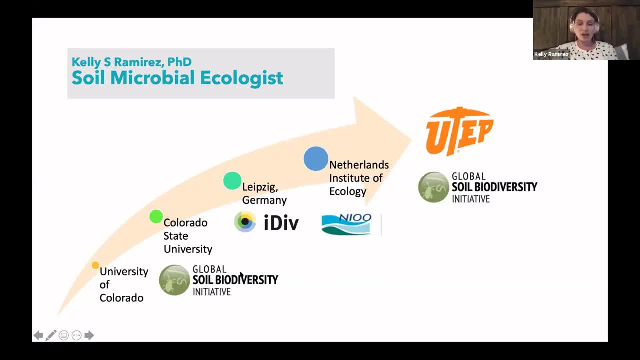 And I was the executive director of this initiative for about a year and a half And then I moved on to back to research. I did a synthesis project with iDiv, moved to the NEO in the Netherlands, but all this time I kept in touch with Diana. 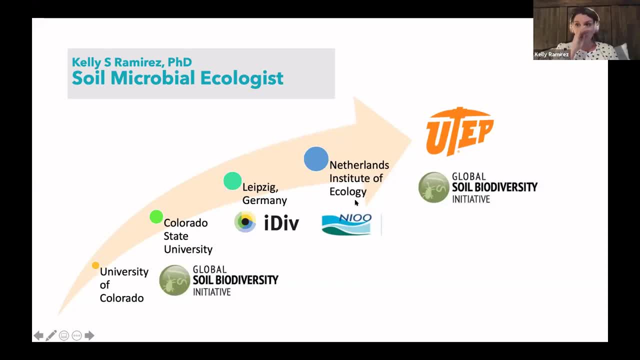 and the GSBI initiative, kind of bringing it along with my research. So if I was doing research at Leipzig I wanted to have some role of soil biodiversity initiative in it, And the same for the NEO, And then, right before I transferred to UTEP, 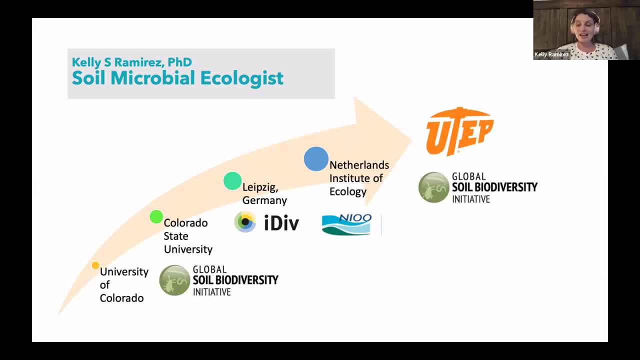 there was this great opportunity to manage this report, And that was in conjunction with the GSBI, And I'll just say they. let me go to Egypt, to the COP- the Convention on Biological Diversity- COP in 2018 to present on how soil biodiversity can be the nexus. 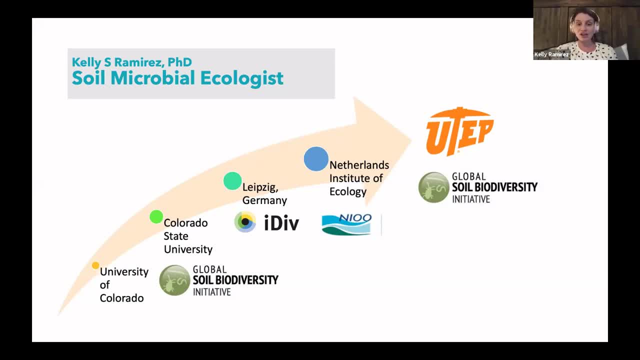 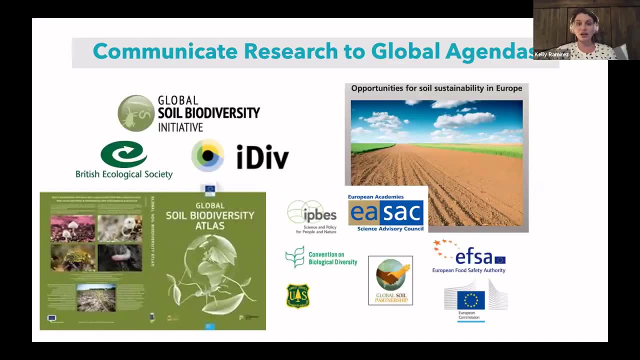 And this was really cool because it's not just talking about my own research, but how all of the different research of soil ecologists- soil biodiversity- can be collated together and be used in global agendas. One thing that we worked on with the GSBI was this Atlas. 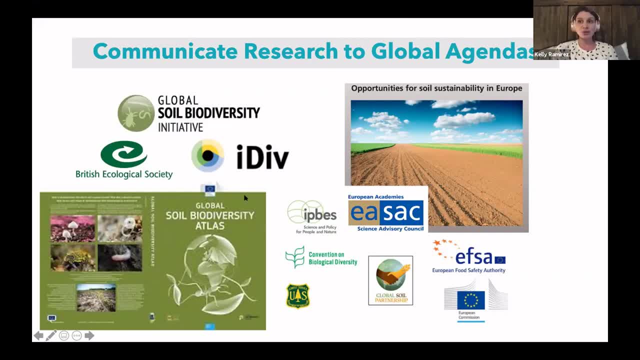 Many of you have probably seen this beautiful book And this is a great policy tool to show people in policy how dynamic and beautiful soil biodiversity is and how intricately it is tied to ecosystem services that we all rely on. I worked at the NEO with Wim van der Poeten. 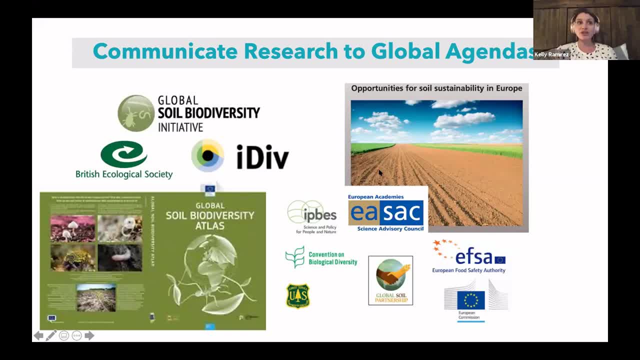 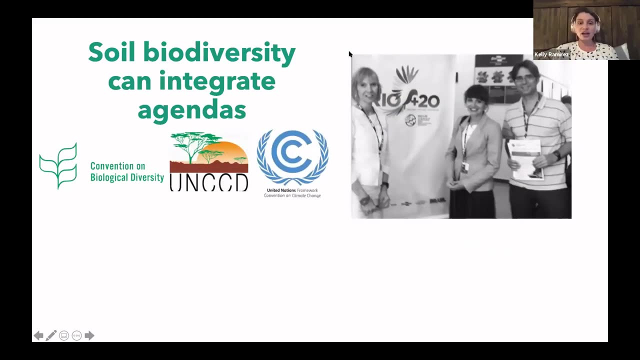 on opportunities for soil sustainability in Europe. So, again, this is taking our research of soil biodiversity and translating it for use by policy and land managers, And a lot of different organizations have been involved in all of these steps. So, like I said, soil biodiversity can integrate agendas. 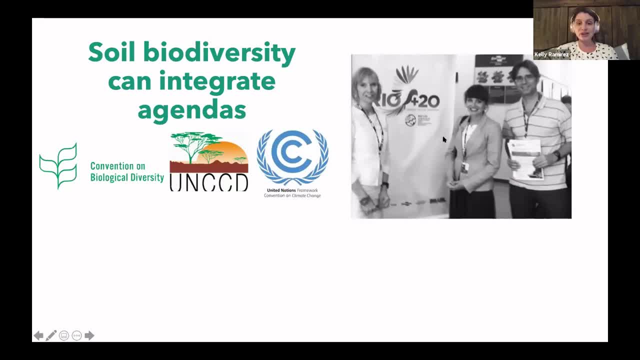 This was us back in 2012 when we went to Rio plus 20 and Diana was there to present on soil biodiversity, And this is George, George Brown, to the other side of me, And so this was the first example of us going somewhere. 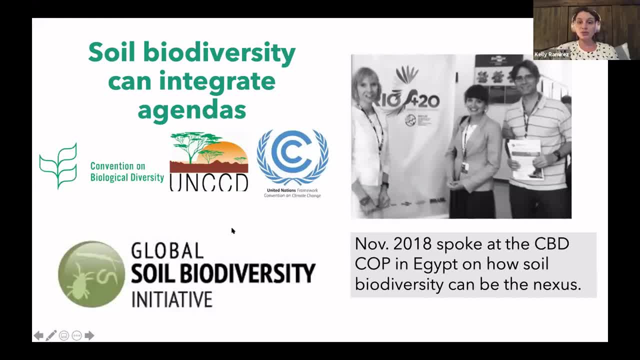 as the GSBI to really push the agenda that soil biodiversity should be included in policy, whether reports or, and because it integrates all these different UN agendas, from biological diversity to climate change. And so that's when I went to Egypt to speak on soil biodiversity. 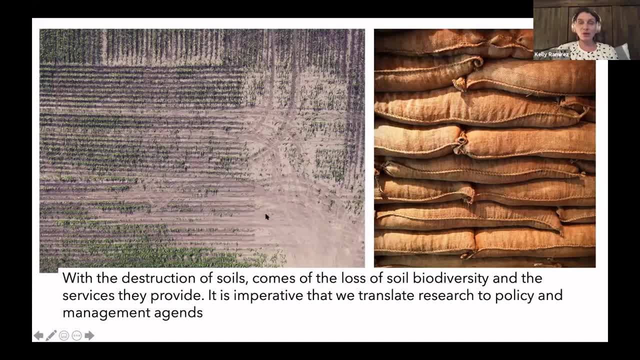 Oops, sorry, Really, to drive home the message that with this destruction of soils comes the loss of soil biodiversity and the services they provide. So it's imperative that we translate research to policy and manage agendas. Okay, so that's kind of the background. 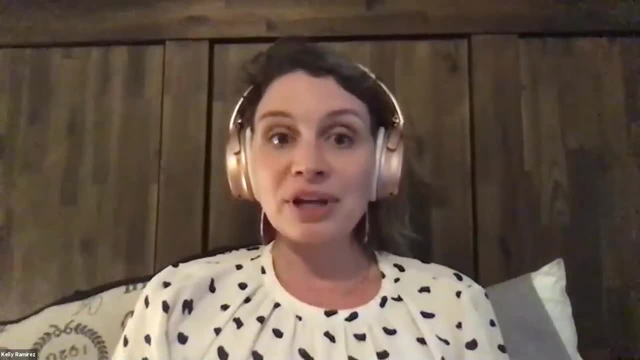 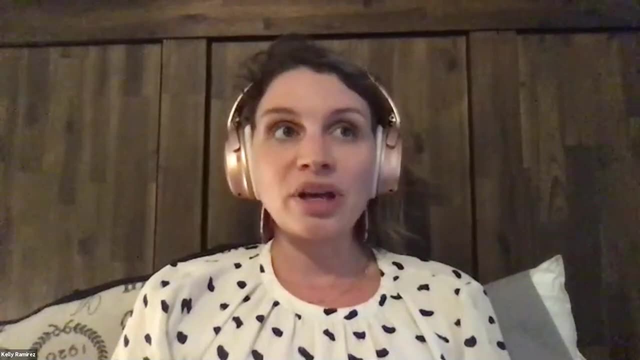 of what I've been working on and how I became involved with the GSBI and translating scientific research to policy. I wanted to do this because when I only worked on research alone, sometimes I got too far into it. I didn't know what I was doing. 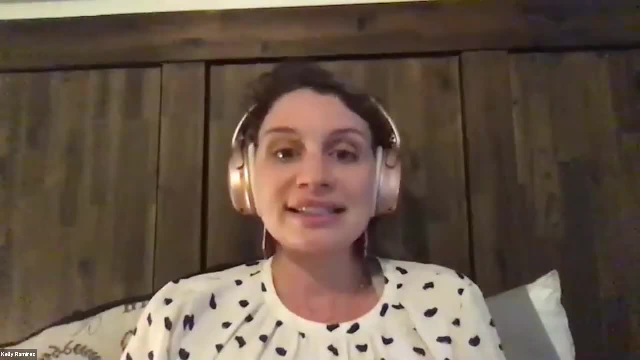 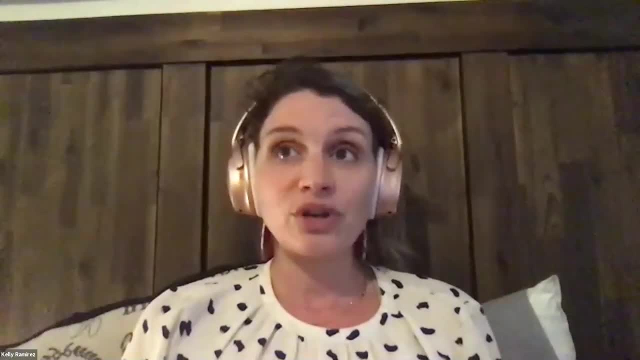 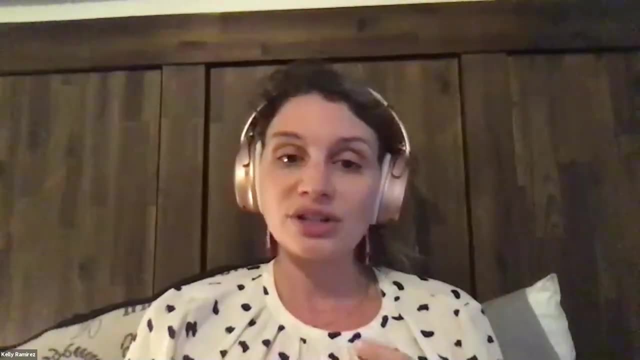 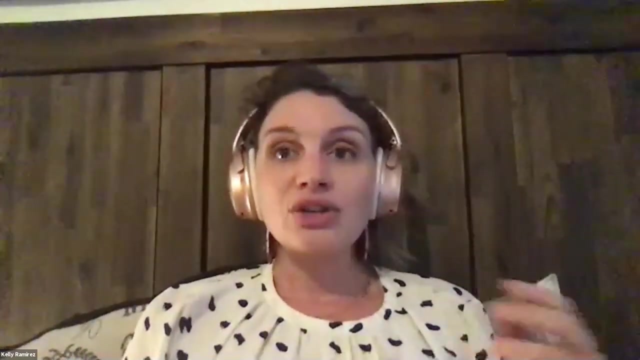 But if we keep publishing papers on soil ecology, it's interesting for us. but do we use that information for big decisions or even smaller decisions at the local and regional scale Right? How can we use our knowledge of biodiversity in the soil to change management or address conservation questions? 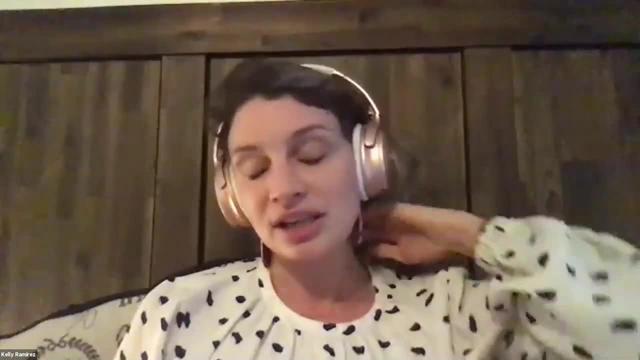 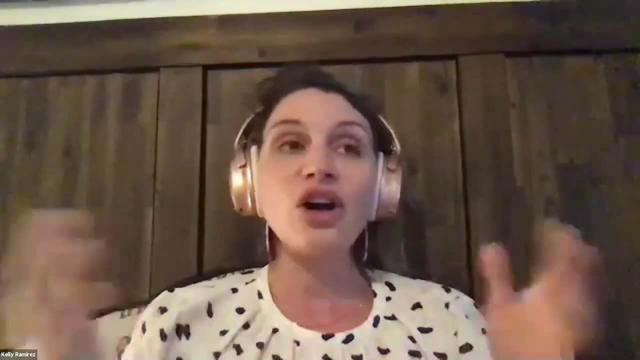 or restore ecosystems right, And so I wanted to find ways that we could do this And part, as Richard indicated, this is relatively new. So the pathways weren't there. It wasn't like: oh, we have this great research and just pass it on to policy. You had to create those. 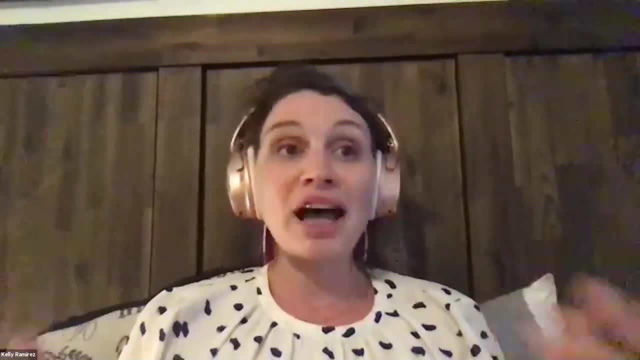 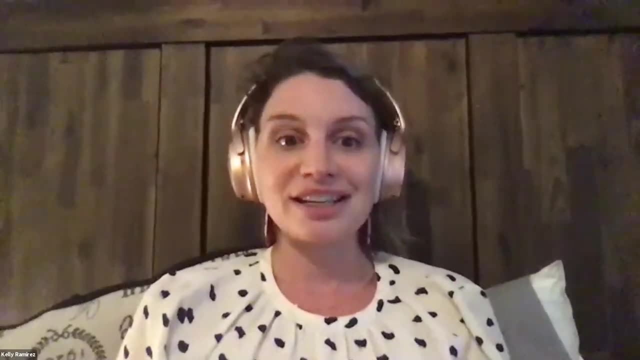 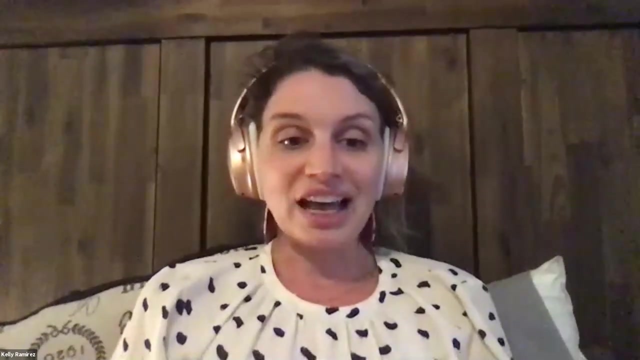 paths. So two to three messages from my chapter. I didn't have a chapter, but I would like to say that this was a wonderful opportunity for me to talk with over 100 scientists from around the world, as I suckered them into writing different chapters and sections in this report, Because 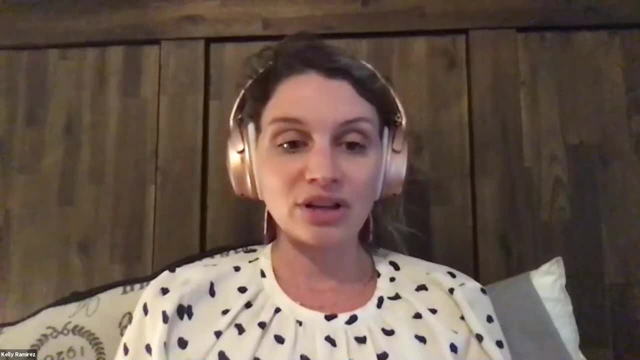 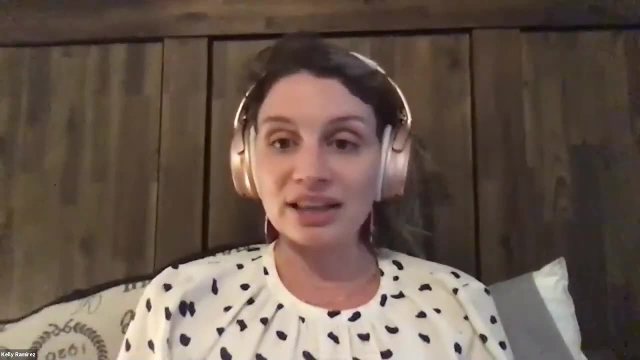 so many of these scientists that are on this report have been doing this work their whole lives, And so it's really great to see their knowledge be translated from a scientific paper into a report like this, And so the last question that I'm supposed to address is: how will this? 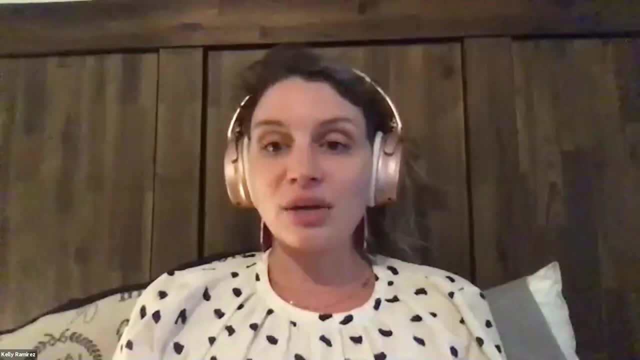 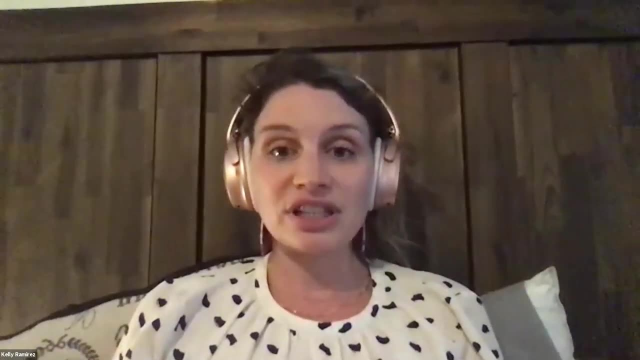 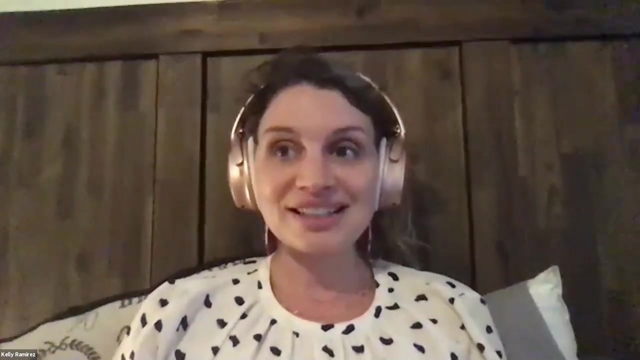 information contribute to or influence soil biodiversity research and policy, And I really hope that it continues to create those pathways so it's easier for scientists to translate their research to policy. Hopefully it will, And I think that ends up with more funding for us scientists, right that still need funding. 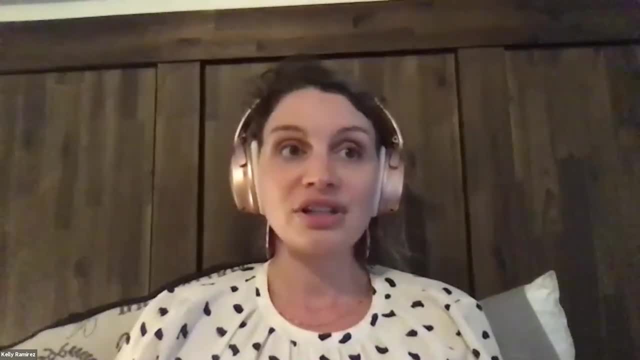 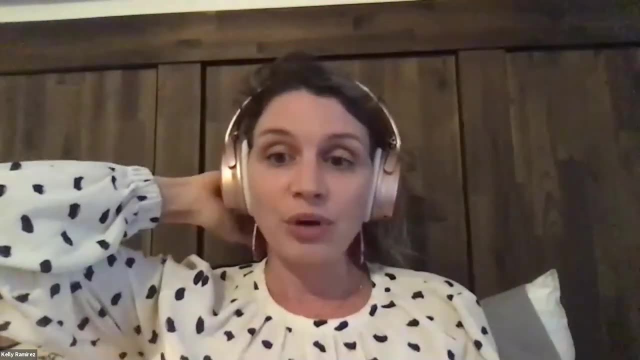 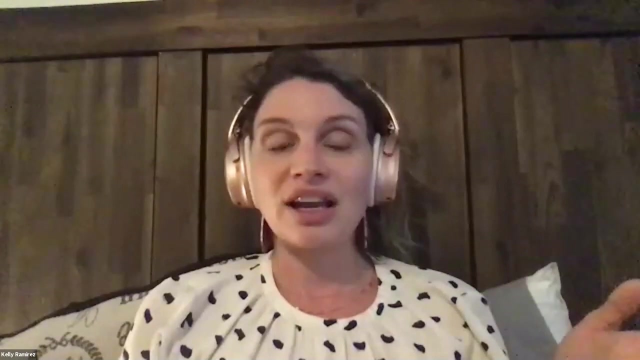 because if soil biodiversity is an important metric to use, then more funding will come our way. And I think, last but definitely not least, it's just really important that soil biodiversity is one of the metrics of biodiversity. Biodiversity we think of as something that has to be. 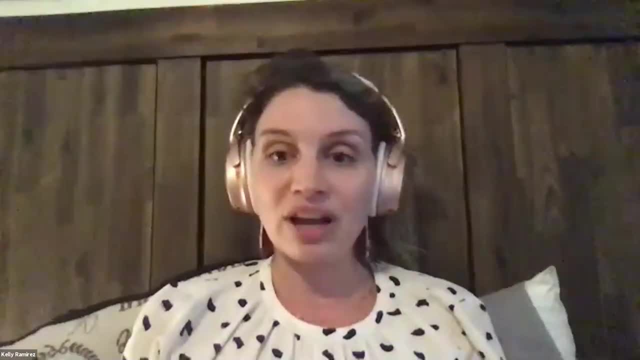 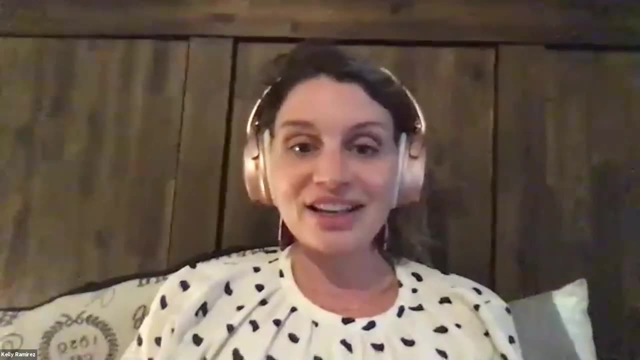 like this beautiful mammal or tree or flower, right, But the low ground diversity really deserves a voice because it's so critical And I think that's something that's certainly something that's something that is really important for us to continue to work hard to make accessible to our ecosystem services. 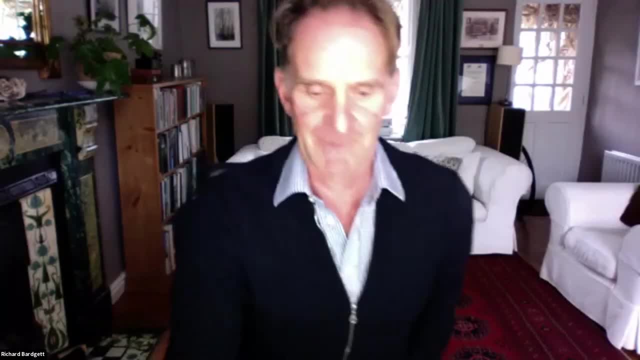 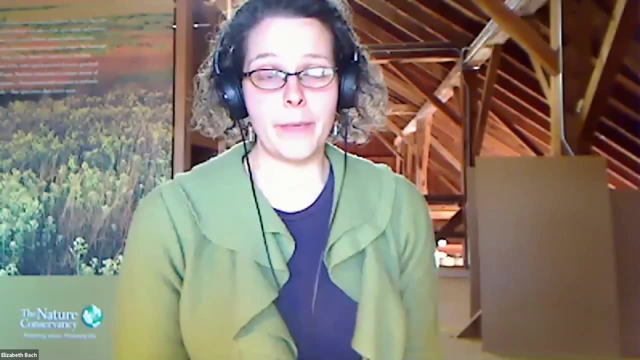 And I think I'll stop there because Richard's video is on. Thank you very much, Peli. We're now going to move straight to our next panelist, That is Elizabeth Vaak. Hi, thank you, Richard and Diana. It's really an honor to be here today with the panelists. 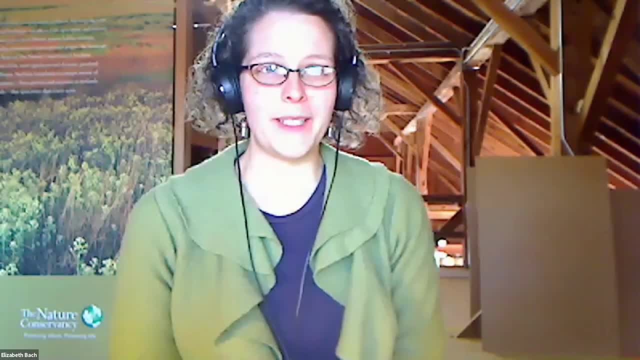 and with all of you joining from around the world, And I do want to take a moment to wish everyone all the best for good health and calm spirit during these times. I just want to say thank you. I think the most important thing is for the kind of work. 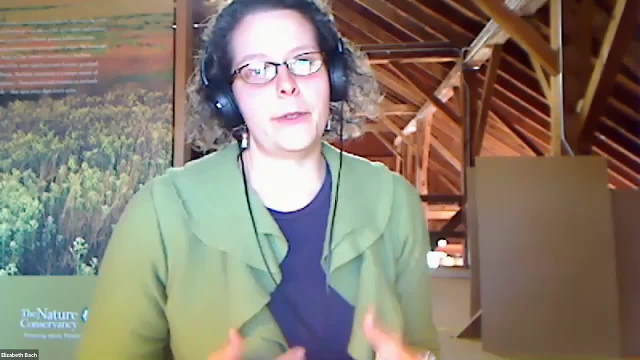 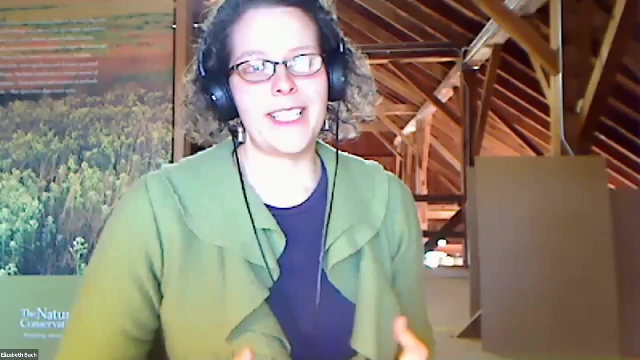 we're doing right now is to be able to keep everyone up to date with our data, And we can make it. My reasons for joining this global effort really are rooted in my reasons for becoming interested in soil biodiversity in the first place. As a young student, I came to the realization that 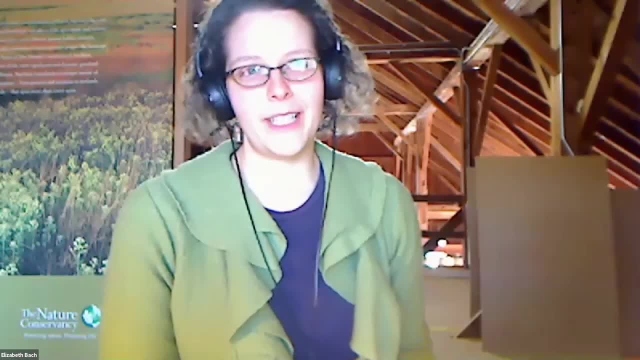 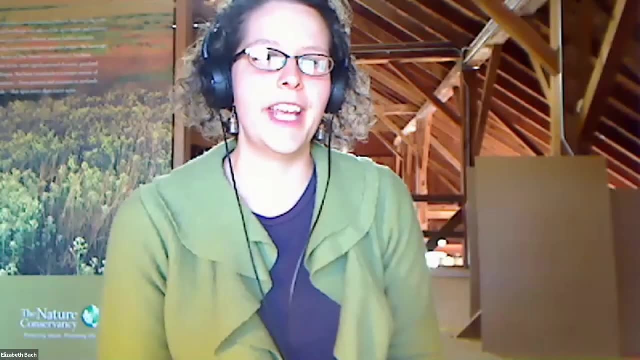 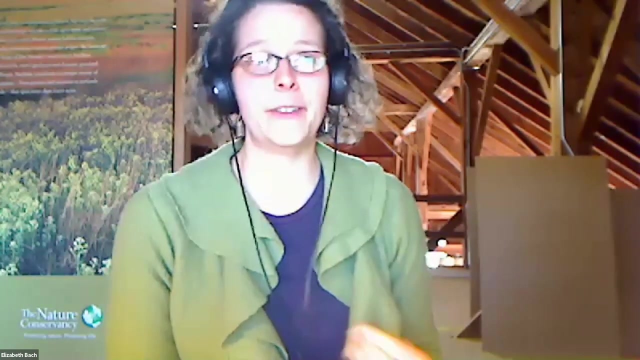 it's these living soil organisms that are recycling dead materials into the elements needed for living organisms to grow and thrive, both above and below ground. And over the years, as I've learned just how foundational soil biodiversity is to life on earth, including humanity, it's become really important to me to share that message and encourage action to 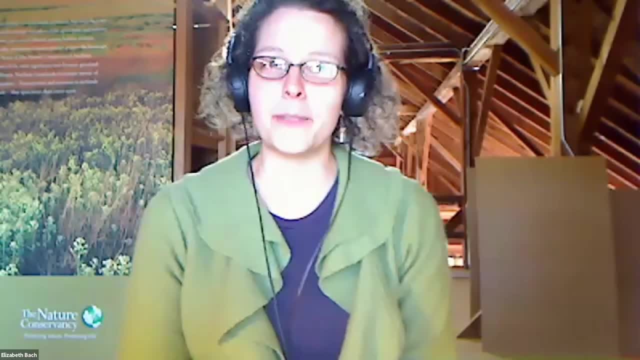 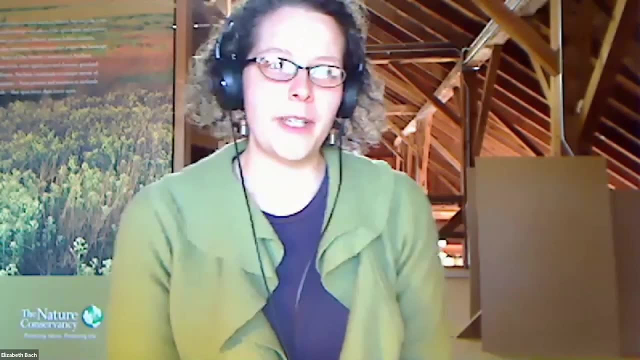 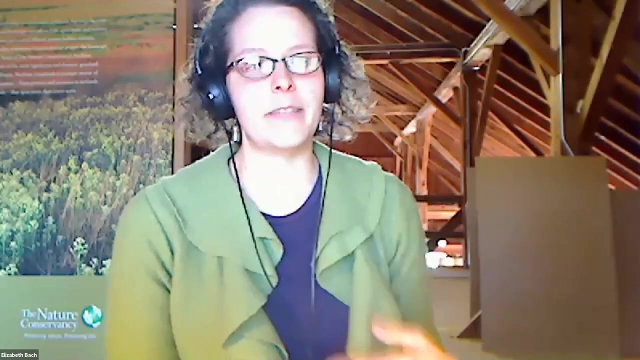 manage soils to sustain life on earth, And that includes some time working with Diana with the Global Soil Biodiversity Initiative. In recent years we've seen a tremendous growth of interest in soil in general, And yet this growth of attention hasn't necessarily reflected the 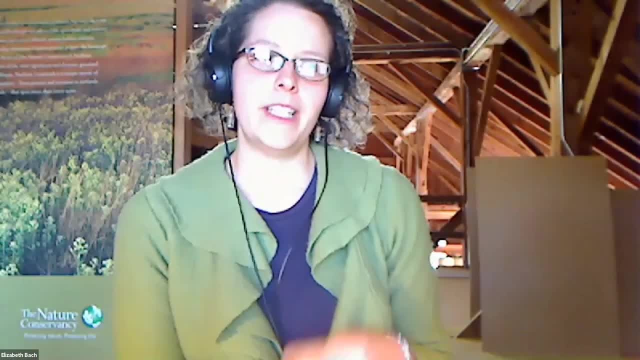 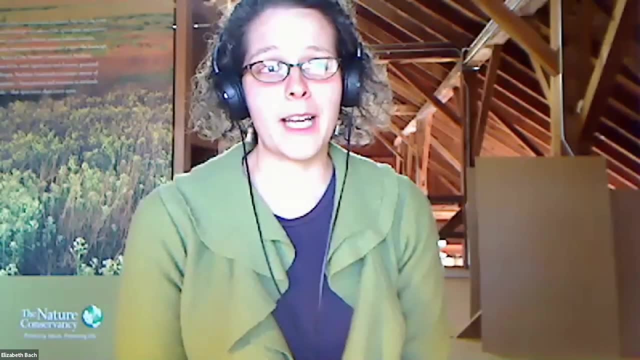 living component of soil to the same degree, And contributing to this global effort was a unique opportunity to bring the spotlight to soil biodiversity, And it's been an honor to work with experts from around the world to bring recognition to soil biodiversity and its role in sustaining the 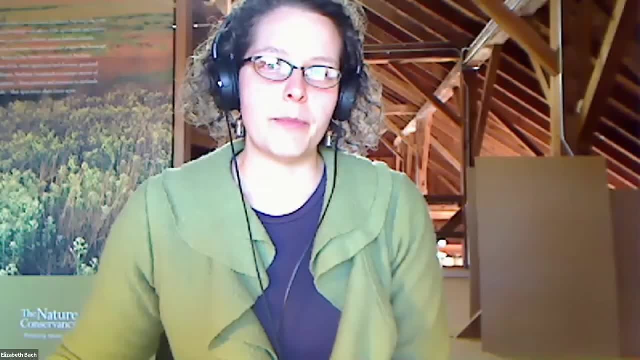 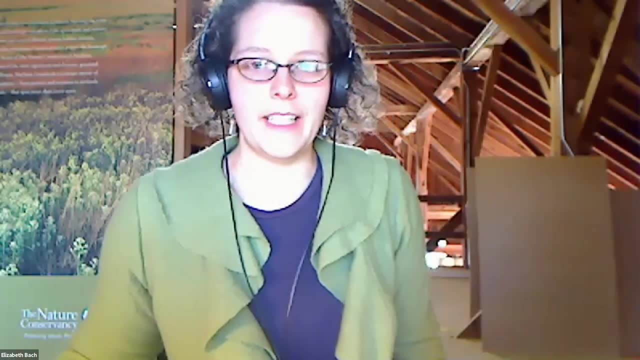 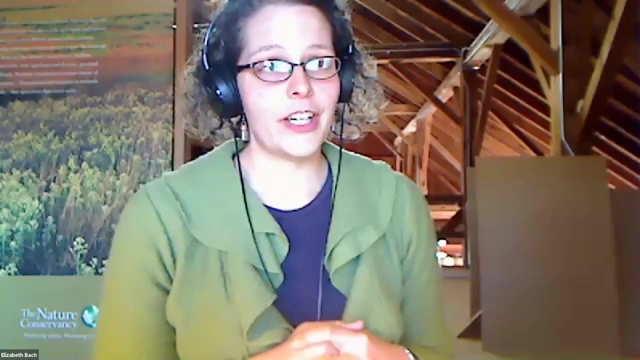 future. I was a lead author on chapter three, which looked at soil biodiversity and ecosystem functioning, And being told my sound is scratchy, I will scoot a little closer to the microphone. So I was the lead author on chapter three, which looked at how soil biodiversity 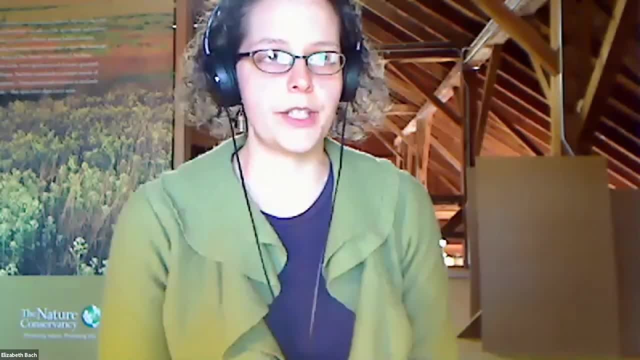 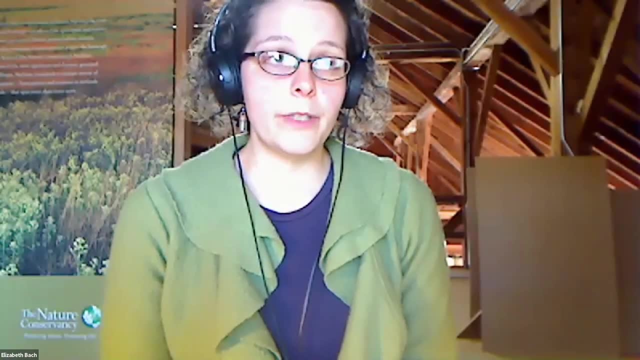 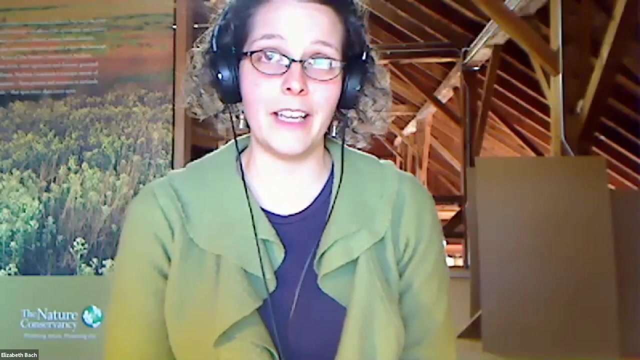 contributed to ecosystem functioning and services, And some of the key findings from this chapter are that soil organisms grow our food and fiber, filter our water, balance greenhouse gases to mitigate climate change and support terrestrial and aquatic life. Soil biodiversity is a source for medicines and vaccines, provides important cultural and recreational. 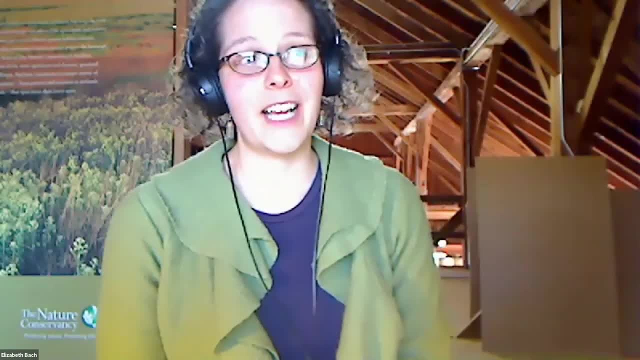 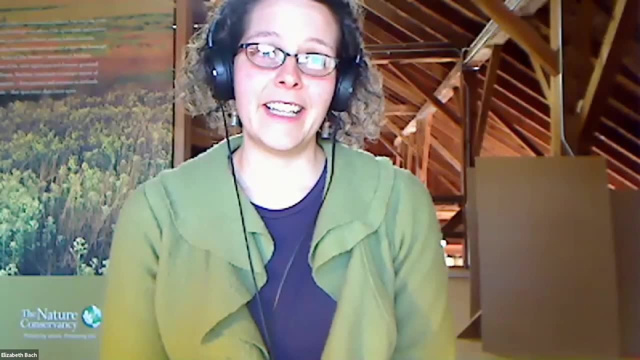 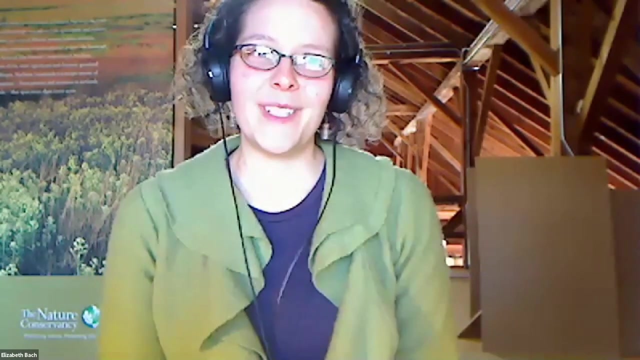 opportunities and is foundational to economic activities like agriculture. Protecting and bolstering soil biodiversity results in multiple benefits to humanity and can advance multiple sustainable development goals and global biodiversity targets. And the cool thing about soil biodiversity is it provides this holistic focus that can help us as communities and a global 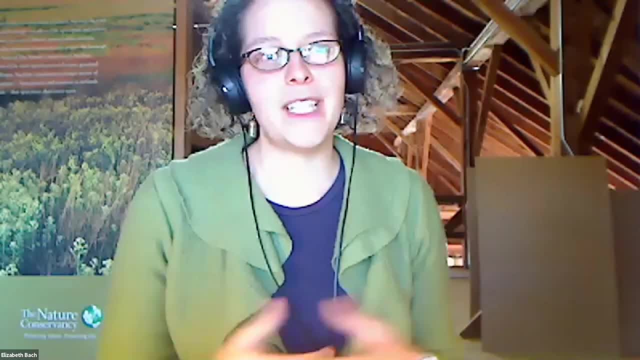 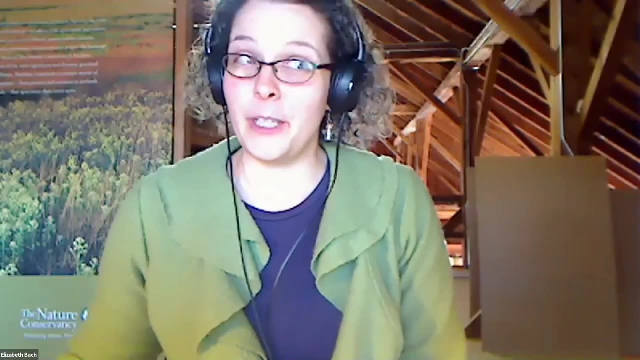 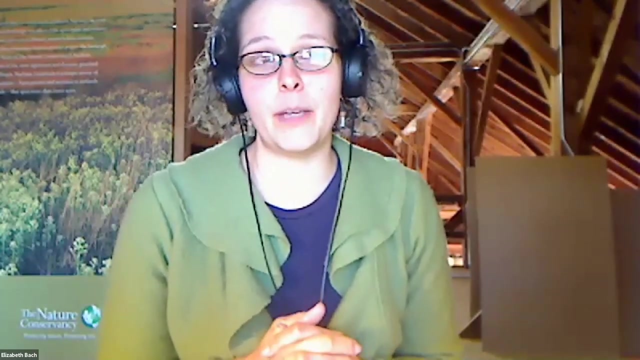 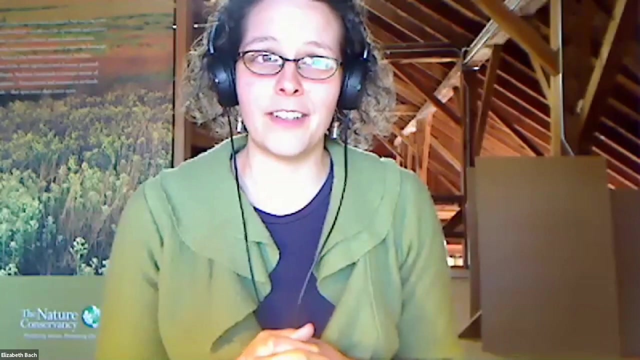 society advance multiple portions of these ambitious global agendas for a better future. So how does this contribute to soil biodiversity research and policy? Well, from the research perspective, this report illuminates many gaps in our current knowledge about soil biodiversity and its functioning. We have a lot to learn about soil biodiversity in places like South America, Africa. 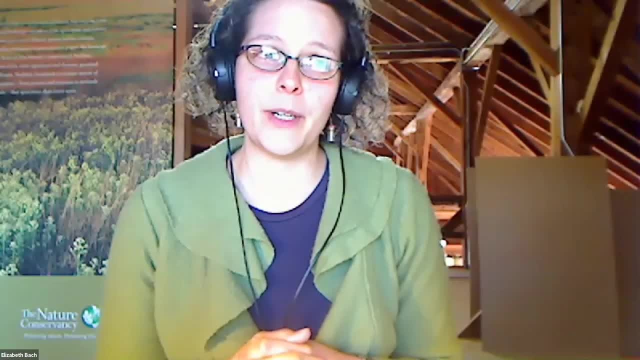 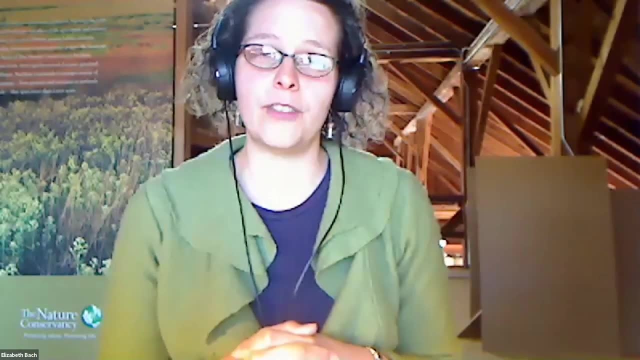 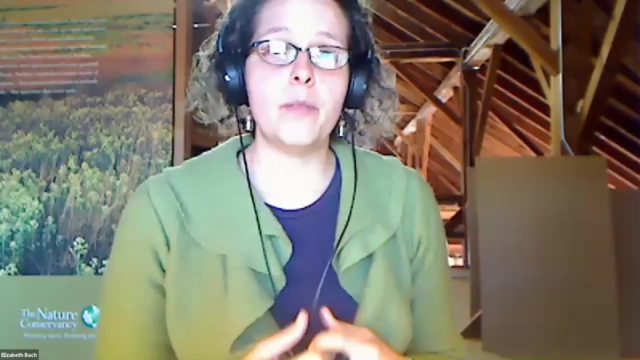 and Asia. Increased knowledge of soil communities in these parts of the world will deepen and expand scientific understanding of global diversity, patterns and the mechanisms that structures biological communities both below and above ground. In addition, in recent years we've seen boon and soil microbiological research, which has really been tremendous to be part of. However, 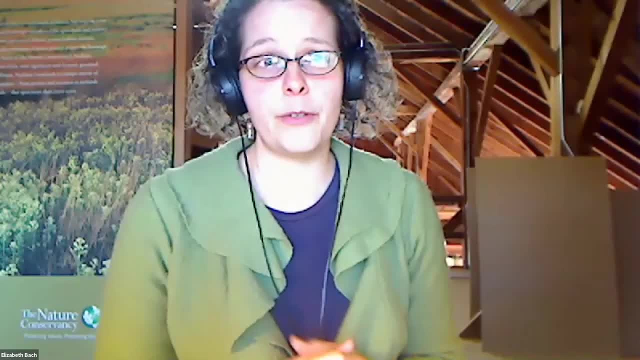 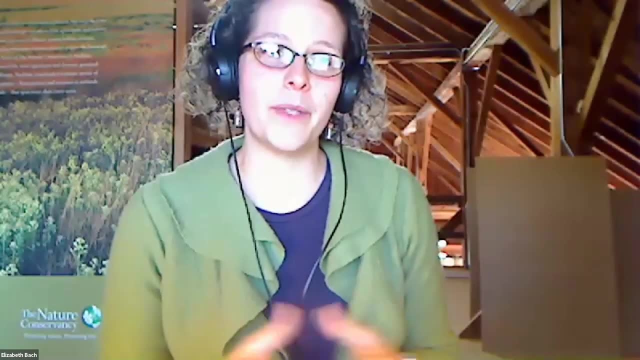 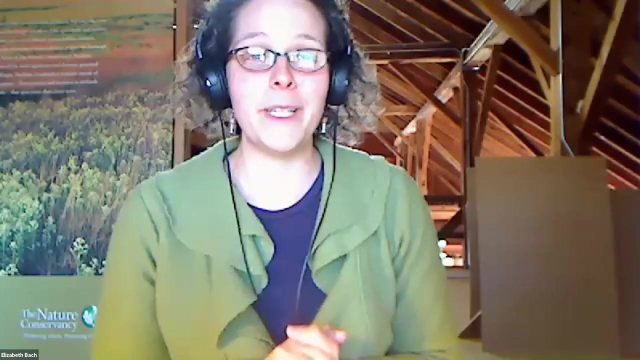 expertise in soil invertebrates like nematodes, earthworms and mites is dwindling and future research needs to both leverage sequencing technologies to help open up this world of invertebrates and build taxonomic expertise. in our rising generation of soil biologists We need 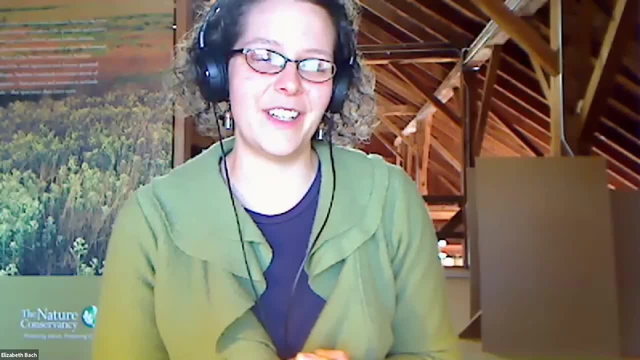 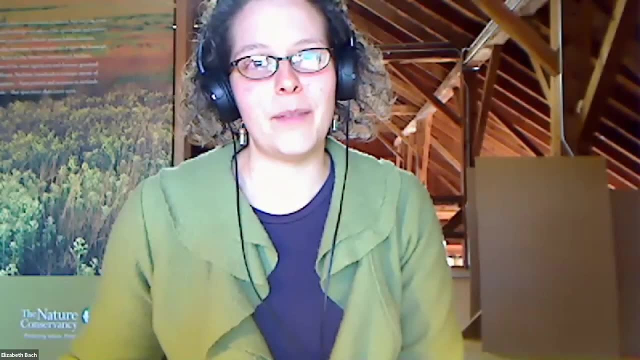 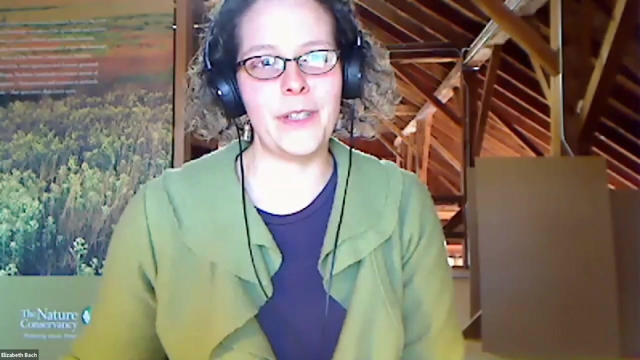 everybody at the table to address these questions and understand our world better. And last, I'll argue from the research perspective. we need research that fully integrates full soil food webs and looks at ecosystem multifunctionality, The thing that continues to energize me about. 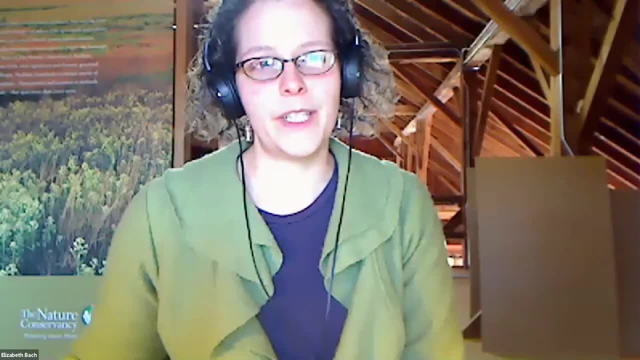 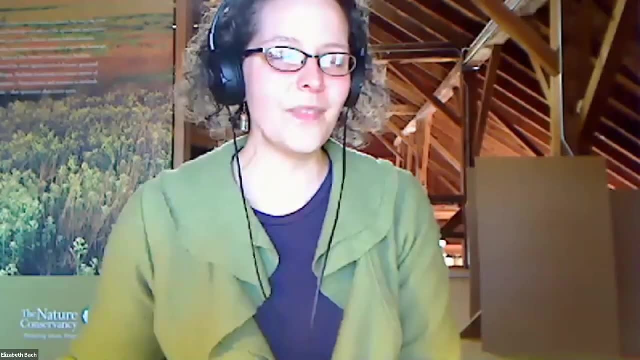 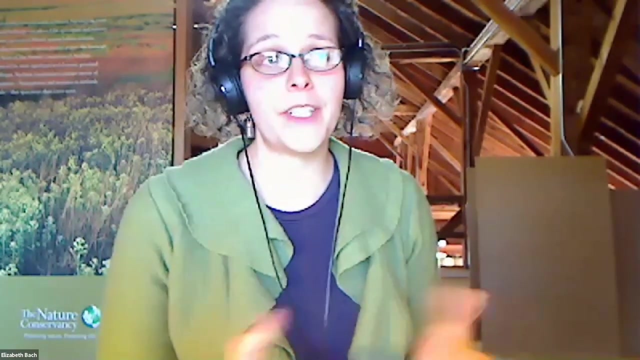 soil and soil biodiversity is how it provides this holistic focus, and we can think about more than one thing at one time by integrating all these parts. How does this report contribute to policy? This is the other cool side of this coin is, as Richard said, this report represents the state of knowledge as it is right now. and we do know a lot, and we know enough to recommend some actions. Soil biodiversity provides multiple services to us, and some of the things that we can do to support soil biodiversity today and for the future include protecting natural areas where soil biodiversity is already thriving and providing critical ecosystem services. This is also a boon to above. 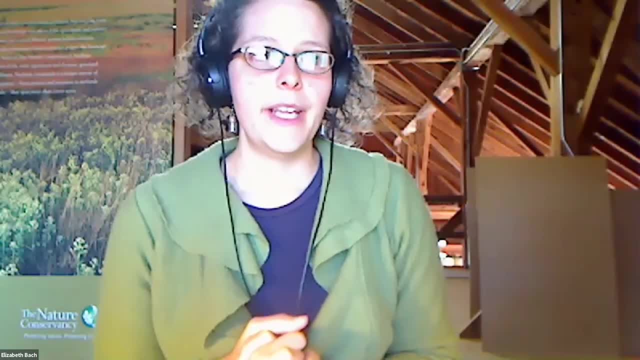 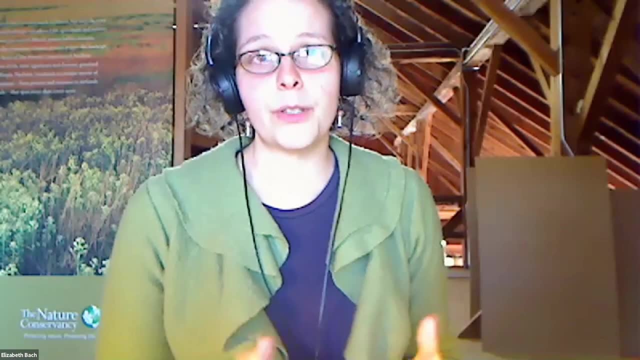 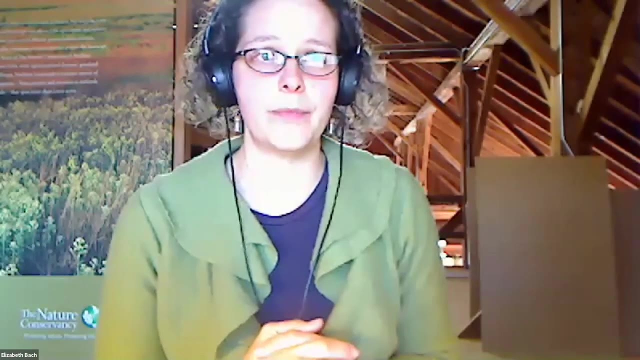 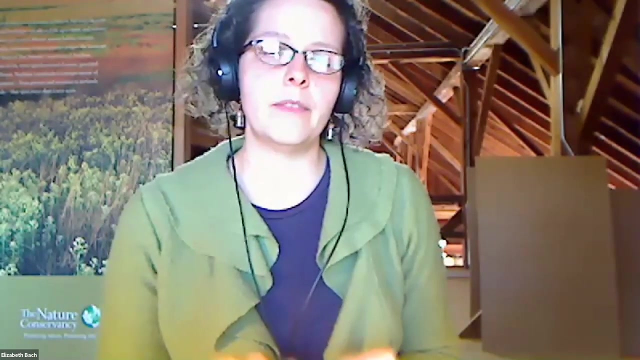 ground and aquatic life as well. In degraded systems, ecosystem restoration provides a really important opportunity to bolster soil biodiversity and improve ecosystem functioning for people in local communities and around the world. In our working landscapes, employing sustainable agricultural practices is really critical to leveraging soil biodiversity. 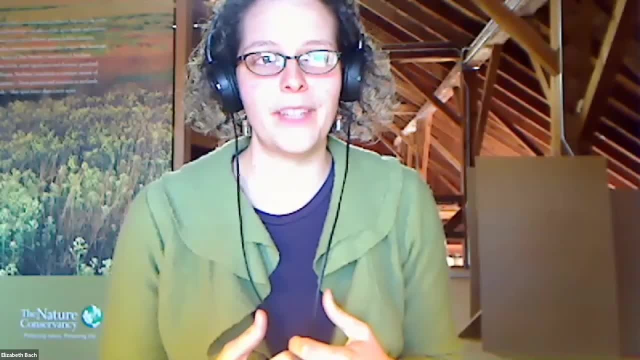 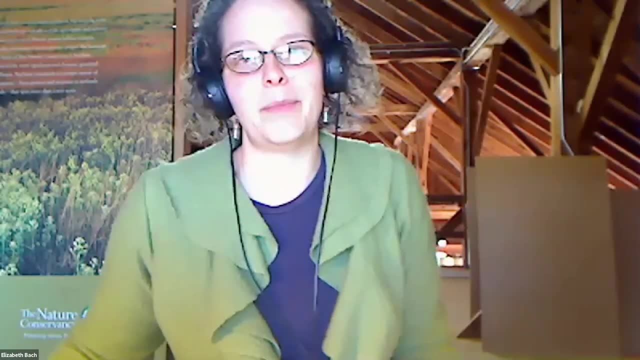 to produce food that we need today and into the future. Lastly, I'll say adapting urban areas for soil biodiversity is really important. They play a key role in cities- and pollutants. I see Richard's back on video, so I'll end there and pass it on. 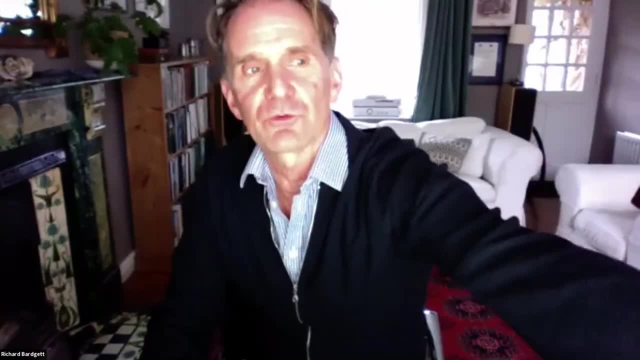 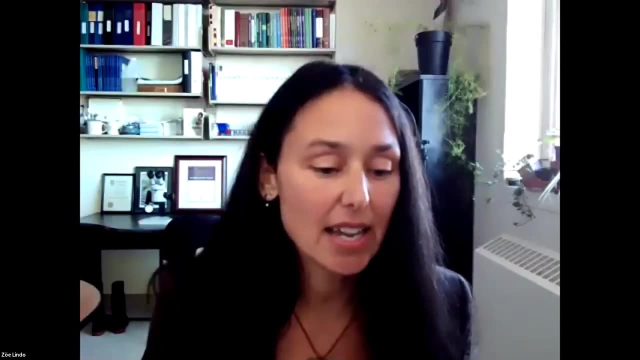 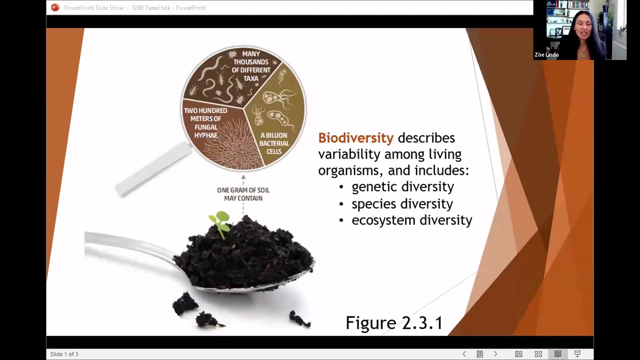 Thank you very much, Elizabeth. We're now going to pass on to Zoe Linder. Thanks, Richard and Diana, for this invitation. Just let me get my screen up here. So this report represents a landmark opportunity to highlight some of the incredible diversity. 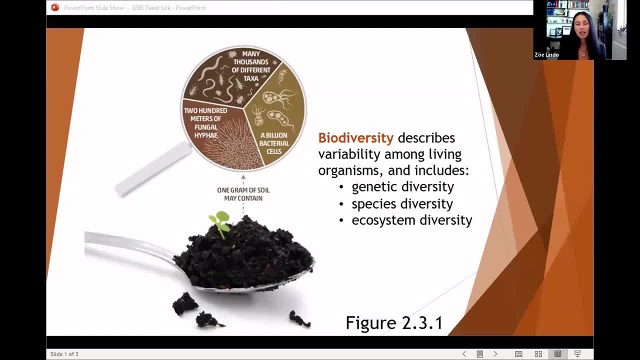 and the importance of soil systems and something that I feel has been, as Richard sort of alluded to, hidden in plain sight, something that I also hope will change with the release of this report, And, I think, one of the reasons that soils and soil biodiversity. 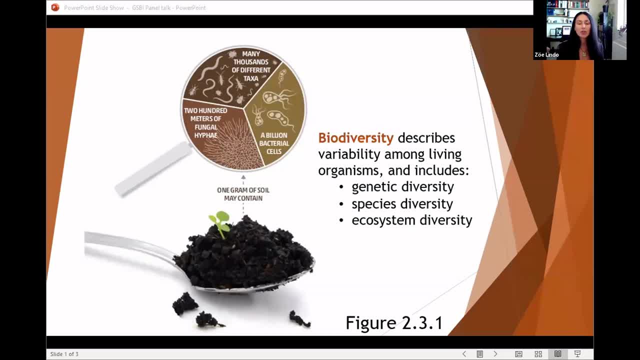 has been largely overlooked, despite their importance and their ubiquity, is that they are cryptic systems And therefore studying soils has some unique challenges for us. The world of soils is small, it's brown, it's opaque. you can't see through it like you can air or water and the vast majority. 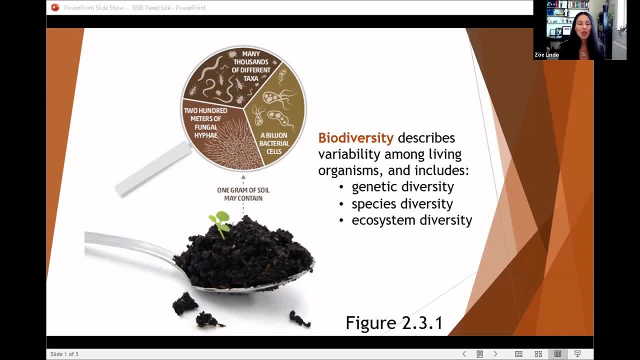 of its inhabitants are microscopic. We don't know the names of many of these creatures, nor what they do, but we do know that biodiversity is extremely high in soil systems, And this image that I'm showing you here from the report is just an example of that. And this high biodiversity is part of our 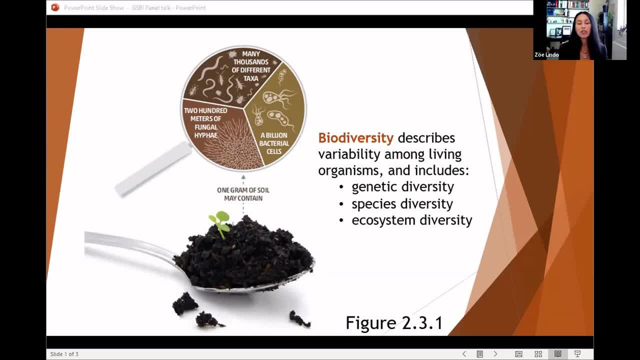 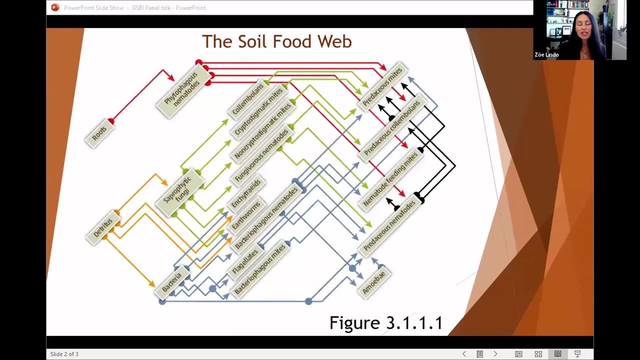 challenge as well as that, the ecology of the species is generally complex. Interactions among species are often indirect, and this makes quantifying their specific roles in the in the environment often difficult to measure. But we do know that these species form a food web. 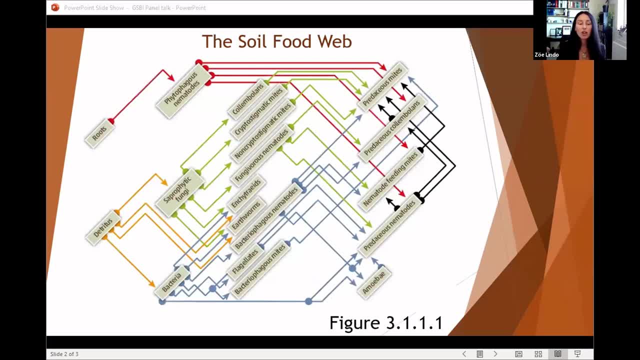 that directly drives decomposition and therefore, in the environment, indirectly contributes to above-ground primary productivity, And so soil systems are of parallel importance to ecosystem functioning, as above-ground systems are, And that's why I joined this global effort to bring the previously invisible to the global stage and let others 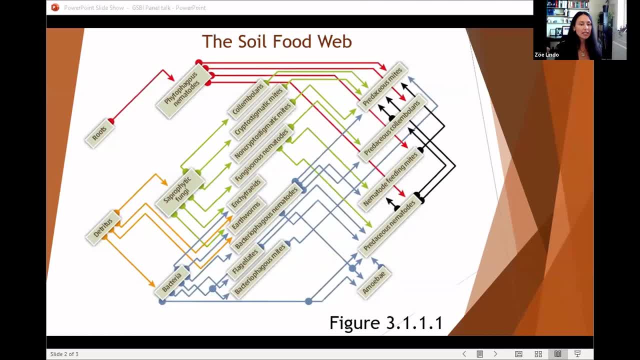 see what I see every day As the lead. on chapter two, we highlight how the diversity of soils isn't restricted to just one or two broad taxonomic groups, but rather the diversity of soil systems, And so I'm going to start off with a little bit of a summary of 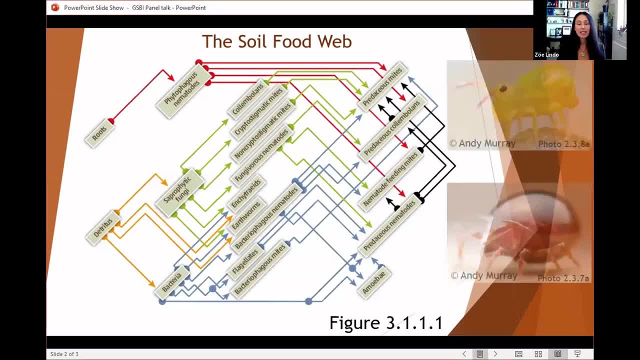 the diversity of soil systems. So soil systems are a complex system that includes organisms across all domains and kingdoms, and includes organisms that most people have never heard of and few people get to see, such as columbula and orobated mites. Soil organisms also spend multiple orders. 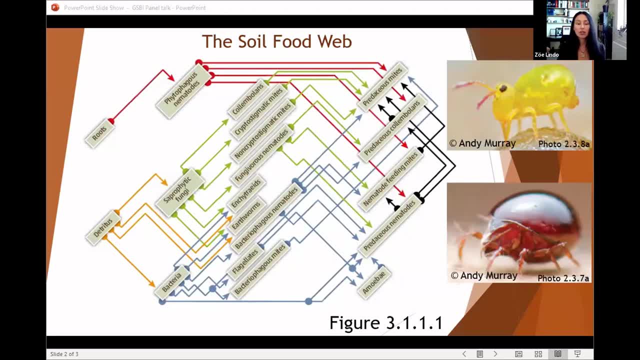 of magnitude in terms of their body size, such that the soil food web is not just complex because of its diversity, but also because it has a nested, three-dimensional and hierarchical structure to it. Soil food web plays crucial roles in the functioning of the planet, like decomposition. 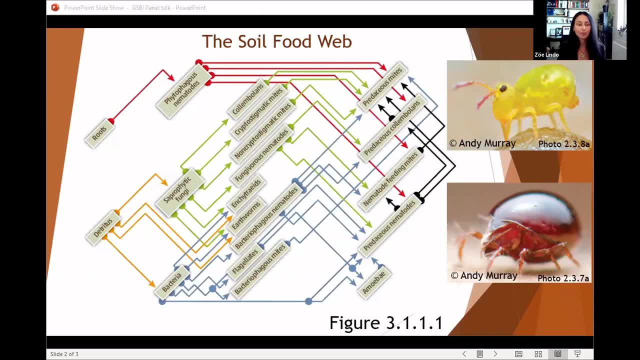 nutrient cycling and the formation of soil structure. As mentioned, the soil food web is instrumental in decomposition, That's, the breakdown and transformation of organic material into carbon and nitrogen and other elements, as well as into stored organic matter. As an ecologist, 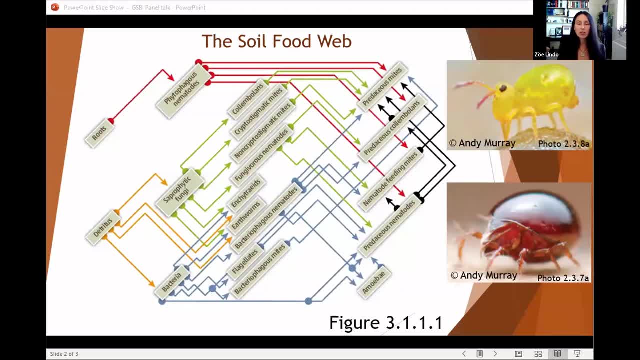 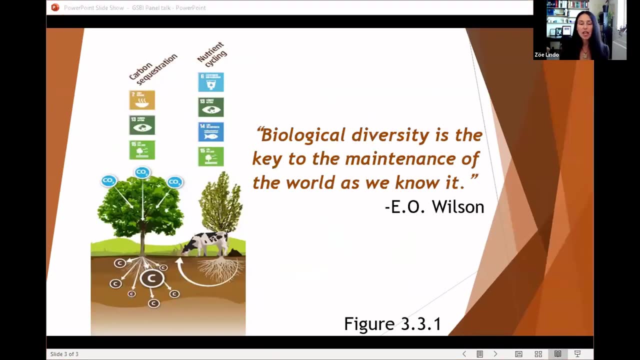 I work on the relationship between biodiversity and ecosystem processes. Specifically, I examine how changes in soil food web structure, like the soil food web I'm showing you here, affects an ecosystem's carbon storage potential. And that's because 90% of all the above-ground 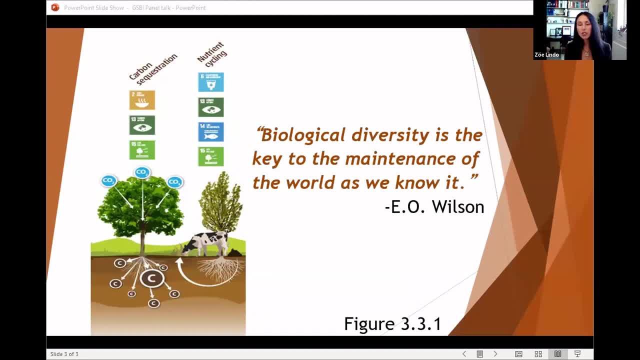 primary productivity is returned to soil systems for decomposition and nutrient cycling, And whether this soil organic matter- the largest terrestrial store of carbon on the planet- remains locked in soil systems or gets released to the atmosphere depends on the soil food web's characteristics. The soil food web, in particular, depends on soil biological communities and these. 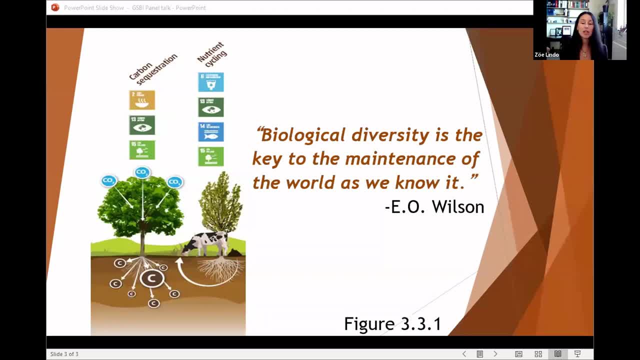 soil processes. As such, soils play a major role in global carbon budgets and therefore potentially hold the key to understanding future climate scenarios, And the soil food web is seen as a key variable of climate prediction models for global carbon stocks. yet soil communities and 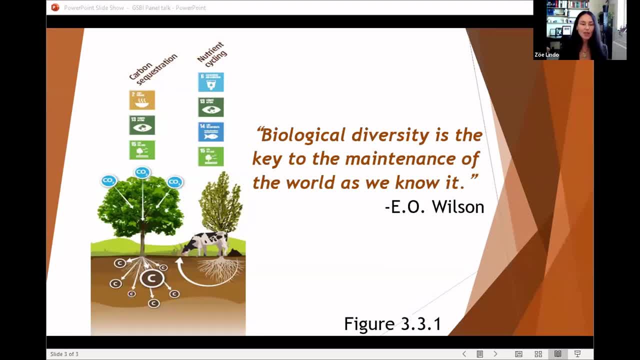 soil processes are not fully incorporated into these models yet. Given the importance of soil biodiversity in multiple ecosystem functions and climate regulation, my hope is that soil biodiversity will be seen as as important a measure as plant or mammalian biodiversity when considering things like environmental impact, climate change mitigation. 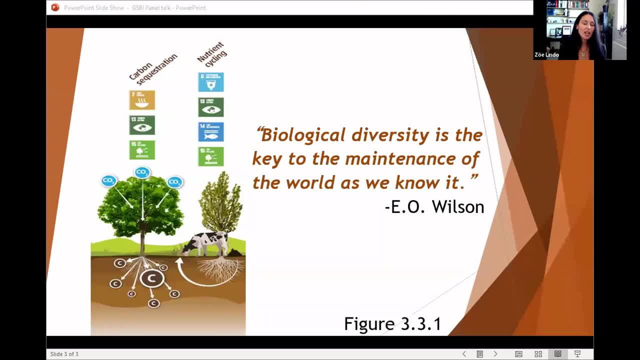 strategies and their related policies. Soils are as complex and beautiful as the oceans and equally important for the functioning of the planet, And yet the vast majority of people never get to see this wealth of diversity that exists right there beneath our feet. So my hope is that this report will inspire interest in the complexity 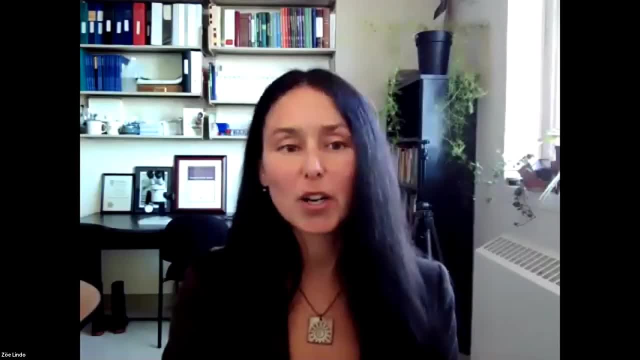 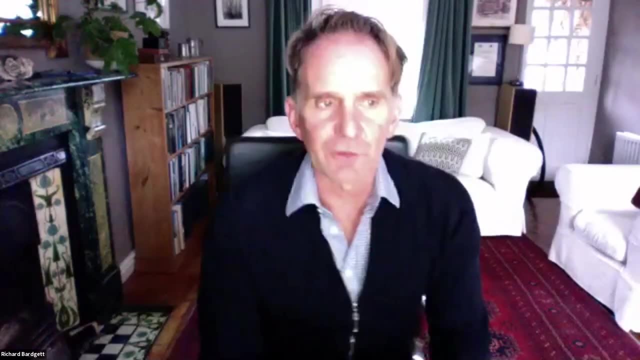 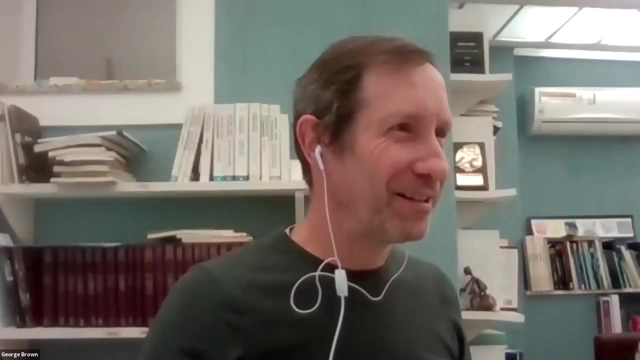 and beauty of soil, biodiversity and the soil environment. Thank you very much, Zoe, And we're now going to move on to our final speaker, which is George Brown. Over to you, George. Thank you again, Richard, and let me just share my screen here. 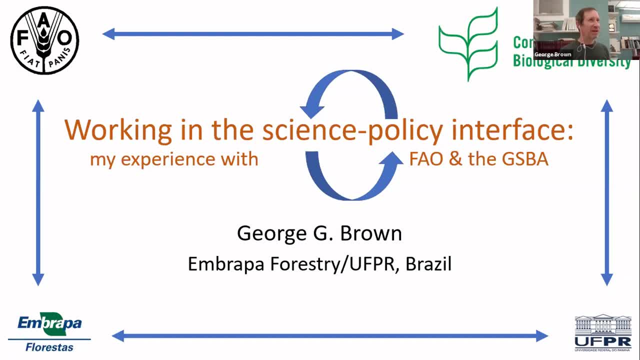 Thank you, good afternoon and good morning to all of you who are participating in this webinar. Thanks for this invitation. Diana and I'll be sharing with you today some of my experience in the science policy interface, in particular, my experience working with the FAO. 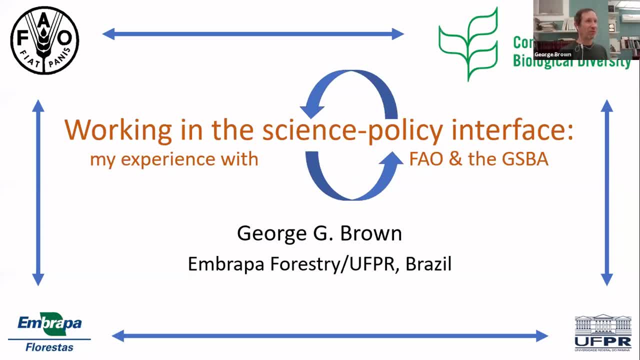 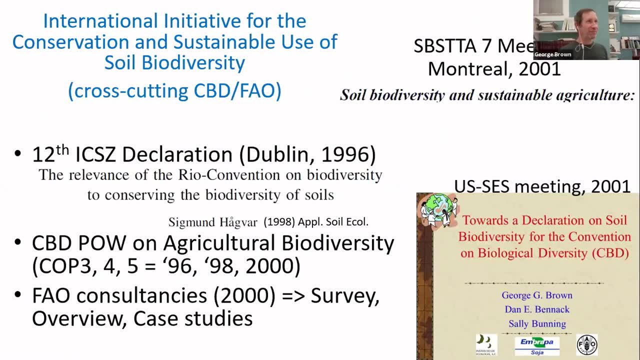 the global soil biodiversity assessment. We've been working with the FAO for over 20 years. over the last few years and more recently in the global soil biodiversity assessment, I'm going to go back in time a little bit and share with you that, actually my involvement in 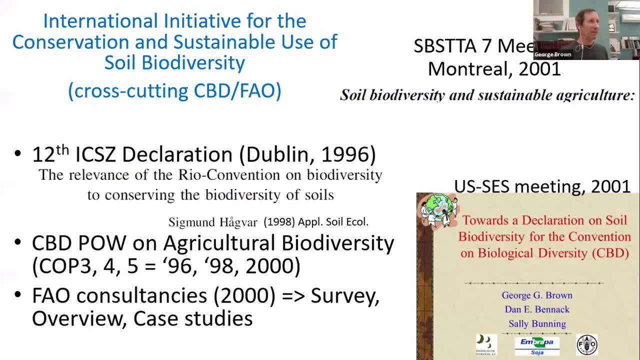 this in this process has been for over 20 years, leading up to what is the international initiative for the sustainable conservation, the sustainable use of soil biodiversity, which is a cross-cutting initiative of CBD, for instance, the Declaration of International Colloquium on Soil Zoology, which was sent by 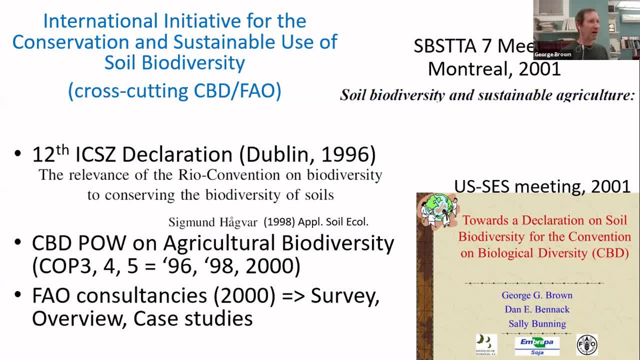 Dennis Parkinson to the CBD and then taken up by Sigmund Chagbar in a great paper in Applied Soil Ecology talking about the relevance of soil biodiversity to the Rio Convention. Around that time the CBD implemented the program of work on agricultural biodiversity and various cops called 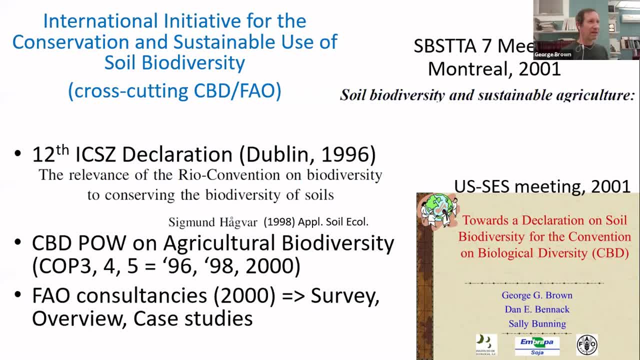 upon the parties to produce evidence and case studies of the role of beginning just with soil microbes but then expanded onto earthworms and all soil biota in the year 2000,. and their importance in agricultural ecosystems for productivity and sustainability. Just after I 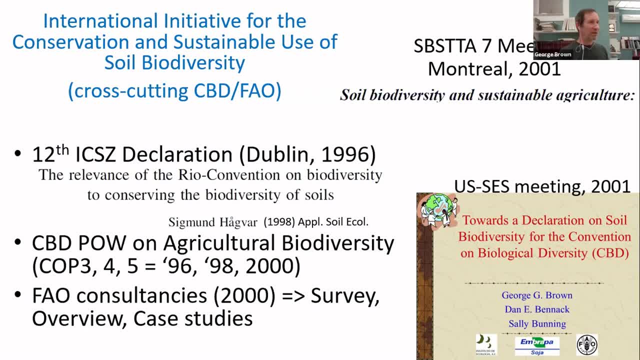 finished my PhD, I was hired by the FAO for a couple of consultancies in the year 2000,. and then I worked with Dan Benek, Adriana Montanez, Sally Bunning and a few other people and ended up. 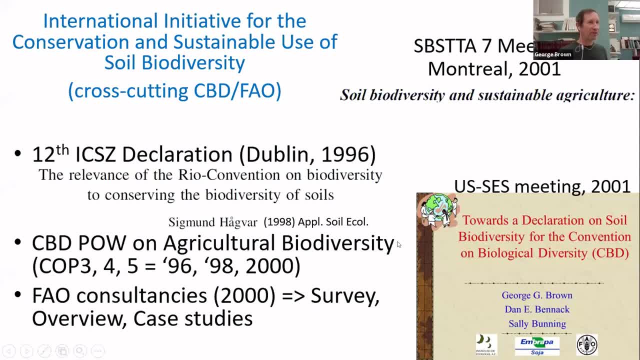 producing a survey, a global survey on soil biodiversity, which many of you probably contributed to and overpriced, And we also had a survey that was used to produce the soil biodiversity portal of the FAO. And then the next year, the following year. there were a couple important events also. We presented some. 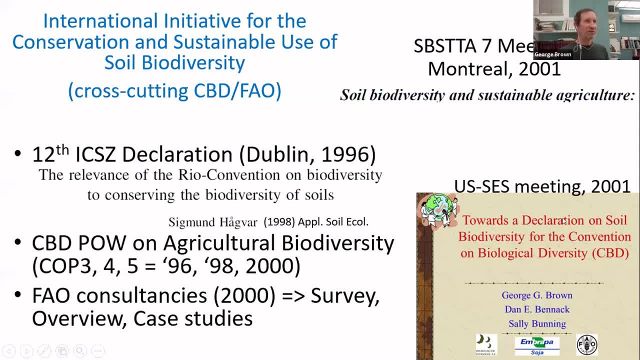 of this information to the Soil Ecology Society meeting in the United States and then in Montreal in 2001 at the SUBSTA. there was an important paper by FAO on soil biodiversity and its role in sustainable agriculture. So these were all important events that led up to the actual initiative, which was launched in 2002. but there 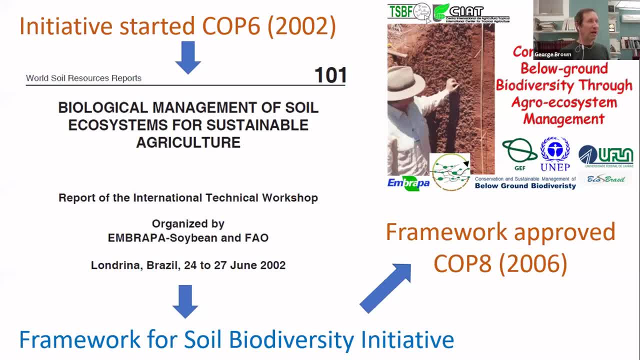 was not a framework yet for that initiative and how it was going to work, and so in 2002 there was a meeting organized by Embrapa and FAO in which we participated, which led to the framework which then allowed the initiative to actually work, and then that was approved at COP 8 in 2006. 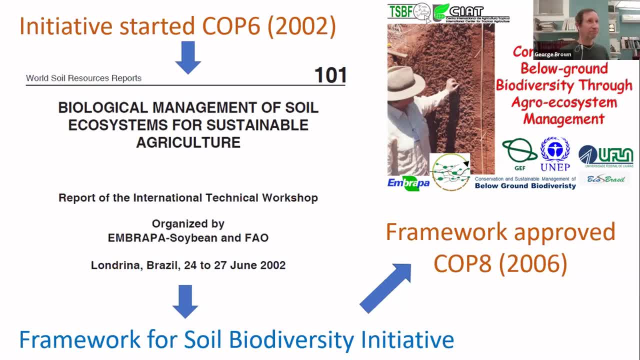 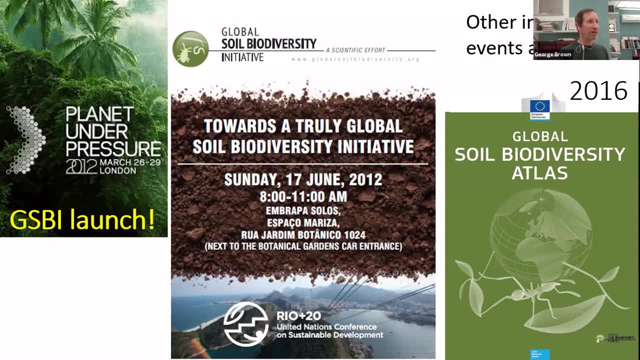 in which we also had a side event on the on the topic. a few more important steps in this process were actually the startup of GSBI in 2012 at Planet Under Pressure. a few months after that, there was Rio Plus 20 in Brazil, in which we organized this side event on truly so about. 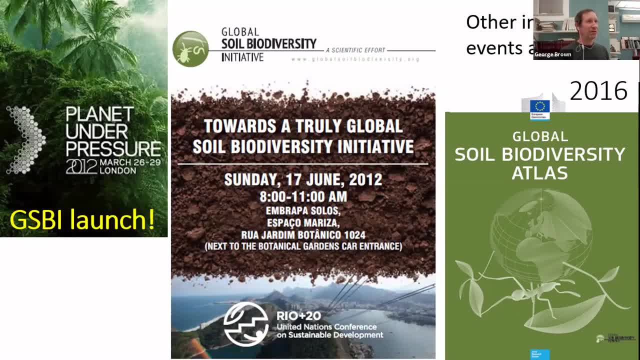 global soil biodiversity initiative and Luke Montanarela presented the why we should go for a global soil biodiversity initiative and we were able to do that. and we were able to do that. and then that was done and published in 2016. great publications, great information and then 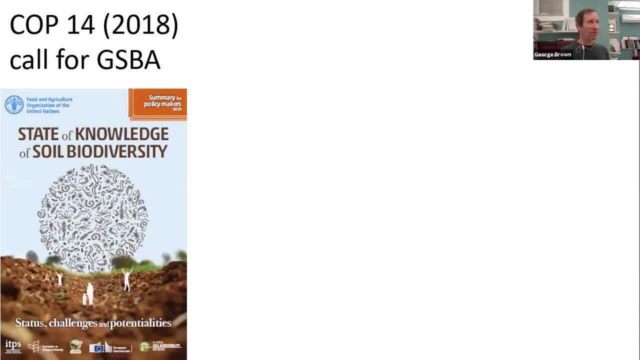 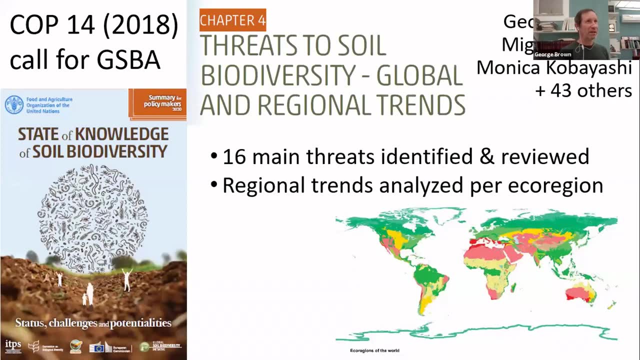 as Kelly shared, in 2018, there was a call for the global soil biodiversity assessment, which is what we're talking about now, and my role in that was together with Miguel and Monica and 43 other researchers and scientists from around the world and identifying the threats to soil biodiversity. 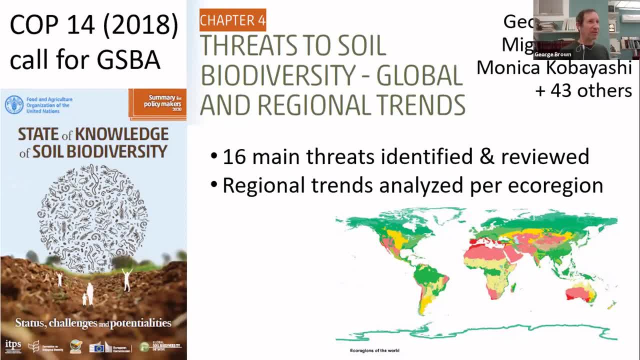 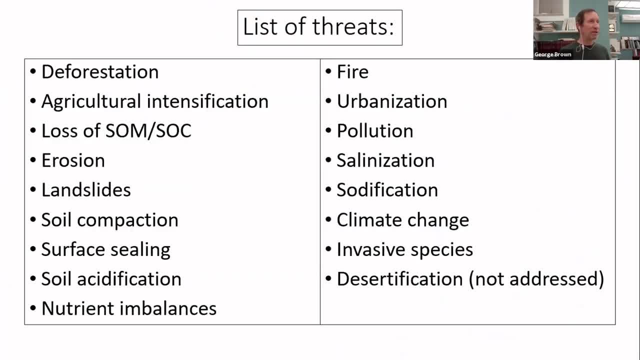 the trends were analyzed in and per ecoregion of the world. this is just a list of the threats. there's quite a few of them here. I'm not going to dwell on this, just to say that, unfortunately, desertification was one of the ones that was not addressed. otherwise, all the other ones were. 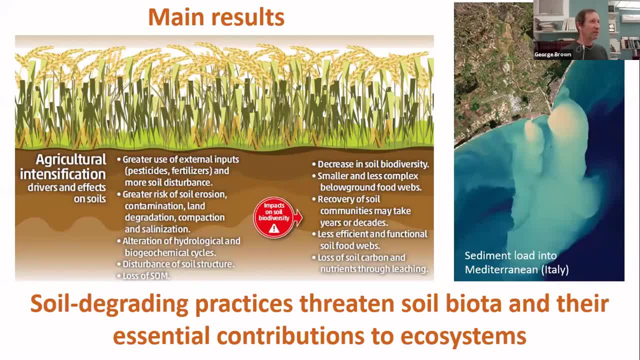 addressed and there were some great figures in that report which you'll be able to see soon. in this case is it's an example of agricultural intensification, with the drivers and the effects of on soils on the left hand side and, on the right hand side, the impacts on soil biodiversity. 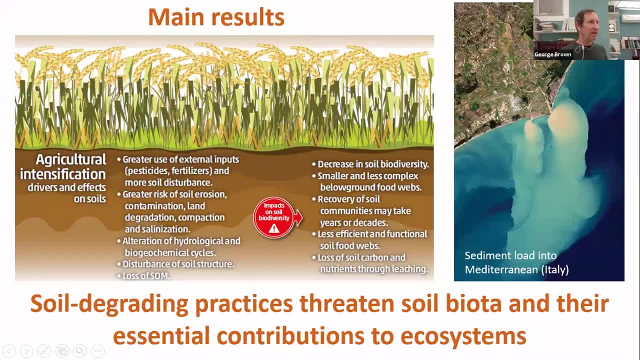 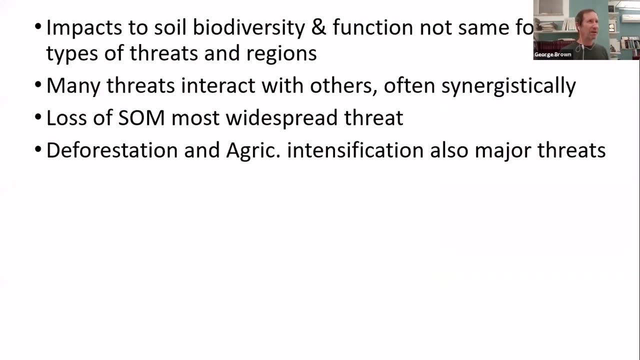 and they just summarized mainly that all the these threats, the soil degrading practices, lead to threats to soil biota and their contributions to soil ecosystems, but the impacts of these threats on soil biodiversity and function are all the same and in not all the same in all the regions of the world and, furthermore, 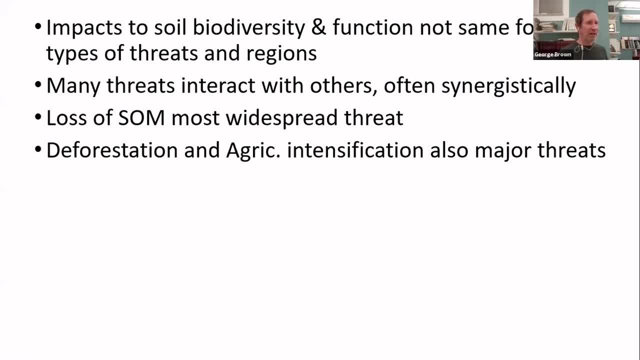 many of these threats interact with each other, often synergistically, so that their if impact is even greater on negatively on soil biodiversity. of all the threats, the most widespread, most mostly recognized, was loss of soil organic matter and often associated with deforestation and agricultural intensification, which were some also important threats identified worldwide. 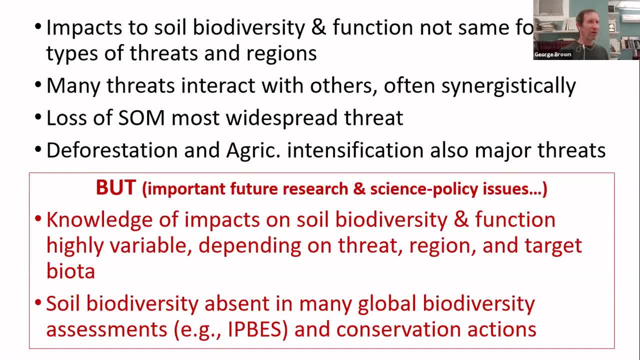 but there are some important gaps for research, and that's important for us and also for the science policy interface, is that the knowledge of the impacts on soil biodiversity of these threats is highly variable depending on the region and the target. biota and, unfortunately, soil biodiversity has been conspicuously absent in many global biodiversity assessments. 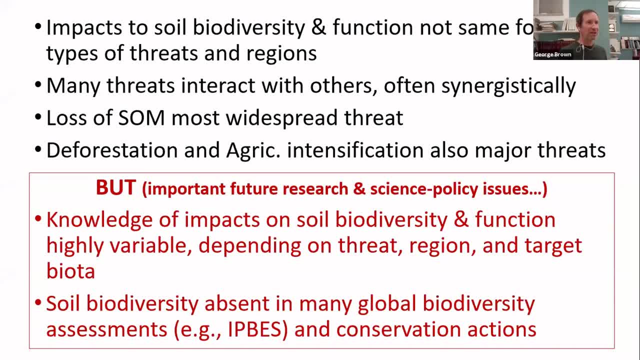 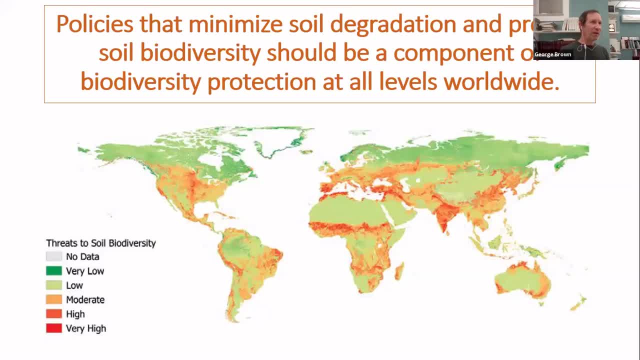 such as the recent one from IPBES, and also conservation actions both at the national and international levels, such as the IAUC and red list of threatened soil biota. so we basically summarize the report by saying that policies that minimize so degradation and protect soil biodiversity need to be a component of biodiversity protection at all levels worldwide. 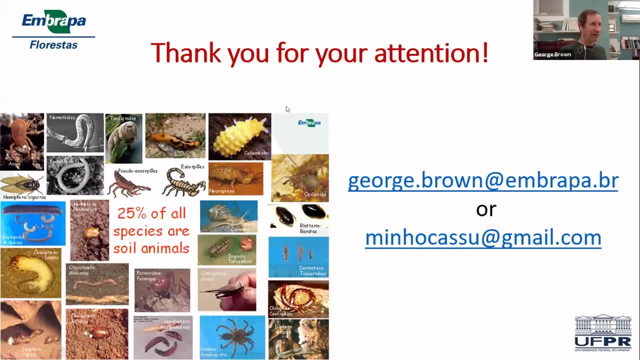 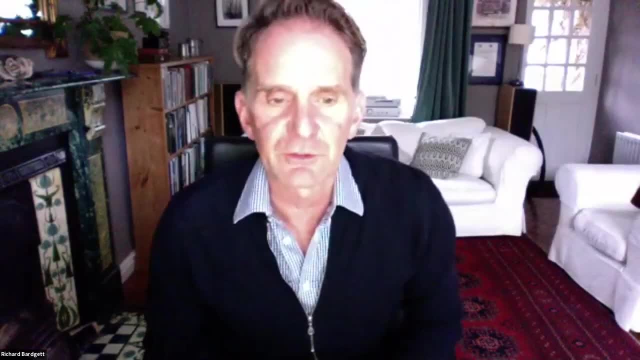 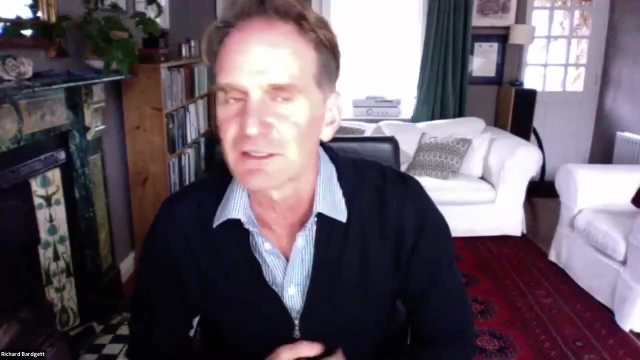 and so I thank you for your attention and thanks again for this opportunity to share. thank you very much, George, and also thank you to all our panelists for your presentations, which were very interesting and provide a fantastic basis for the Q&A session that we're now going to move in as 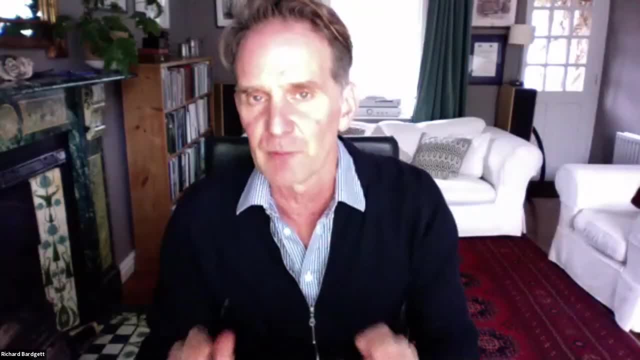 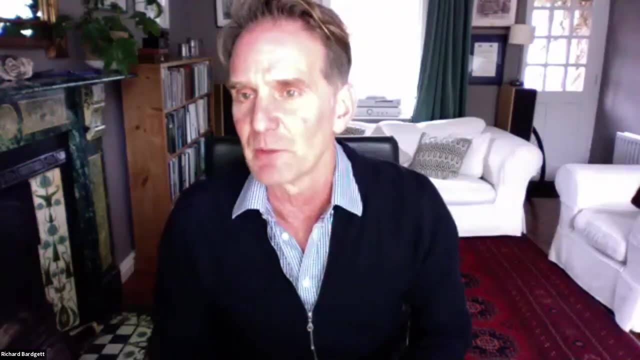 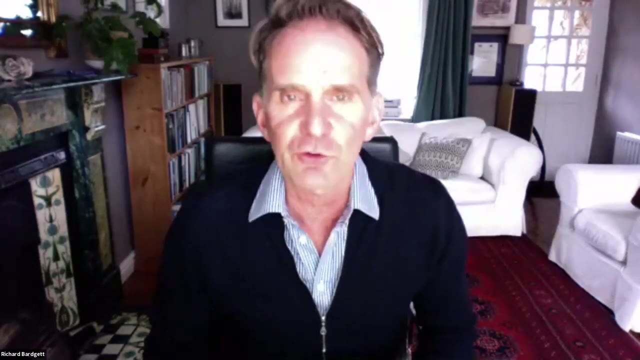 I said before, what we're going to try and do is address as many of those questions as we can. but again I apologize that there is a big audience and there will be many questions, I'm sure. so we won't be able to address them all, but we'll do what we can. I'll just ask. 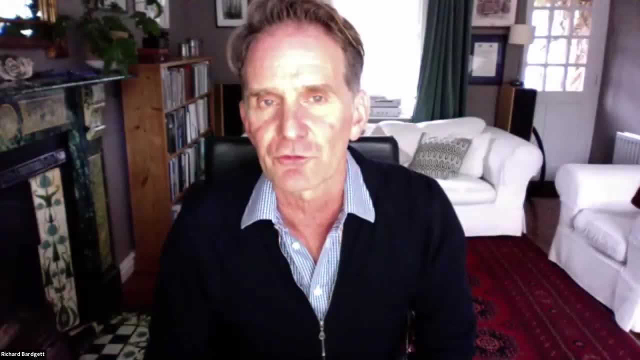 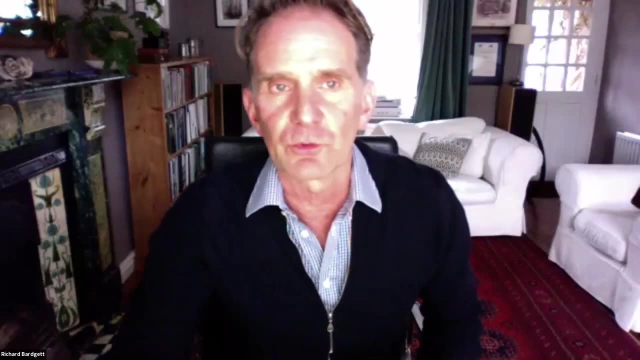 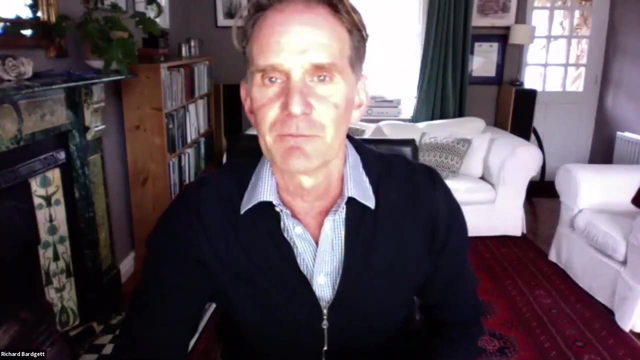 all the panelists to come up on the screen so that we can actually see them, thank you. so what I'm going to do is just go through the questions as we have them and I'll ask one of the panel members to address that question and the first question, which was actually the question that. 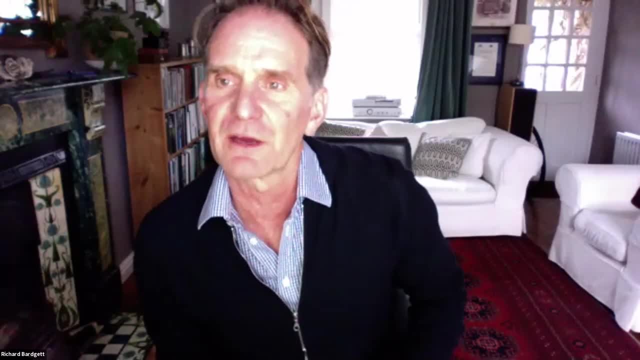 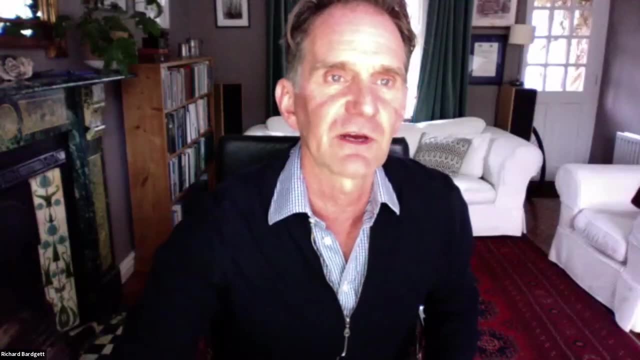 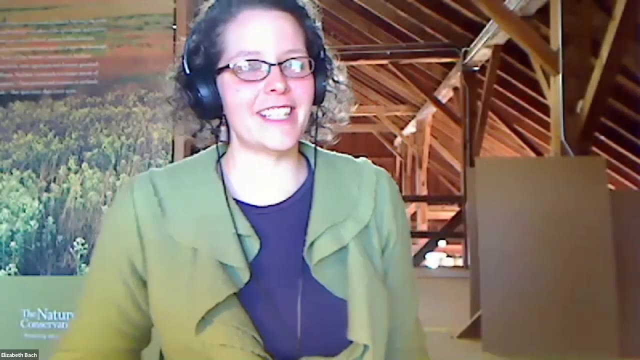 came up some time ago is: how can the soil biodiversity be an effective agent for soil remediation under stress? I'm going to ask Elizabeth this as someone working on ecosystem restoration. so, Elizabeth, sure, I think this is a really great question, because soil biodiversity straddles. 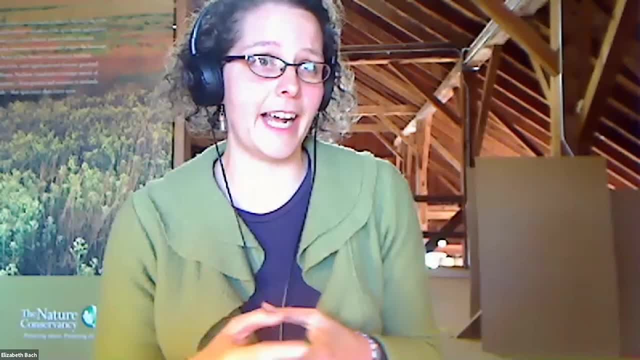 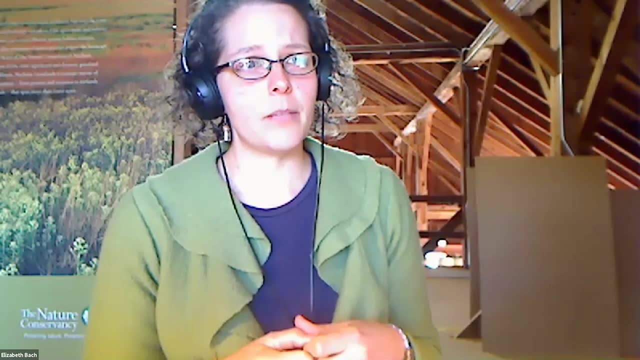 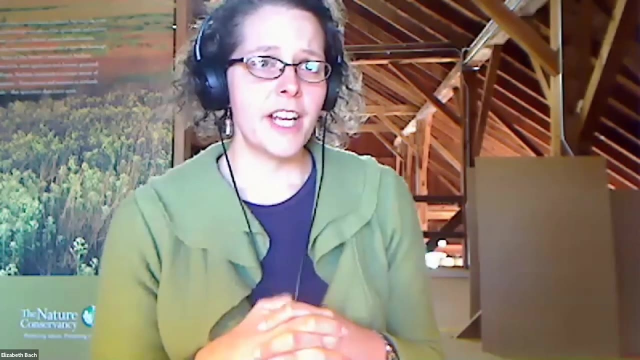 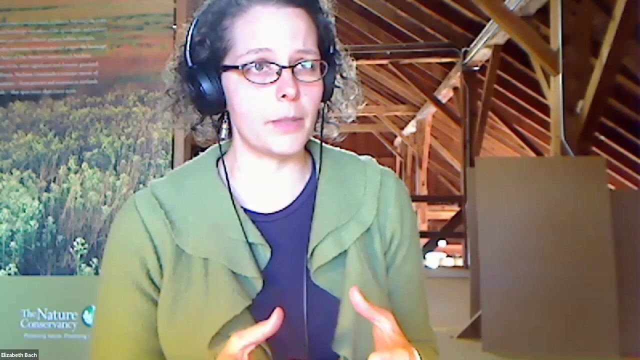 this role where it can be an active play, an active role in that remediation or restoration process, and there's example of organisms that can directly degrade pollutants or take up heavy metals from soils that have been impacted from those sorts of activities. there's also a variety of soil organisms that are really important to help plants establish and to re-establish native plant communities, when that's an overriding goal. 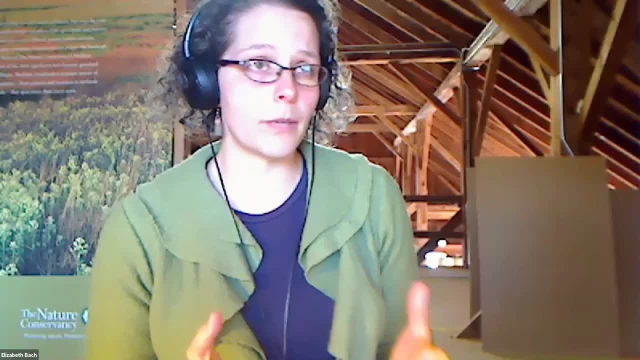 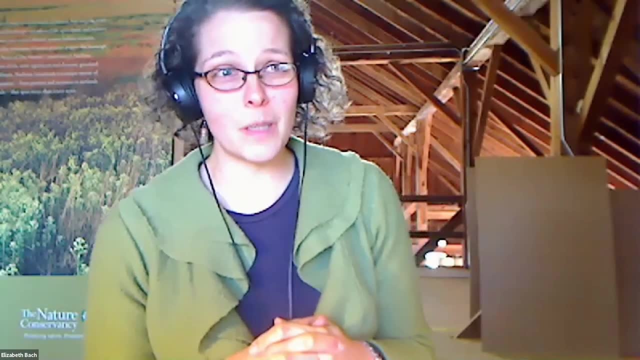 partners like mycorrhizal fungi, rhizobia for legumes, are all really important in that role and the specificities of that kind of depend on which ecosystem or the scope of the project you're working on. but yeah, I think that's one of the great things about. 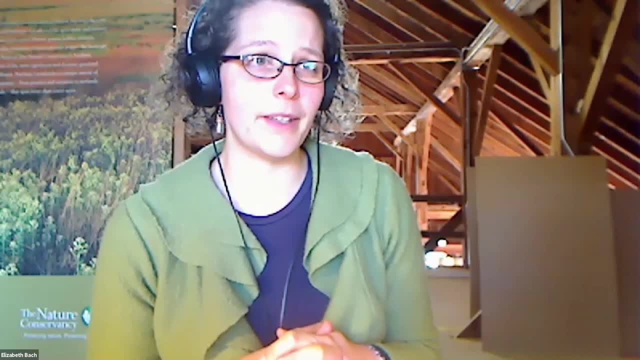 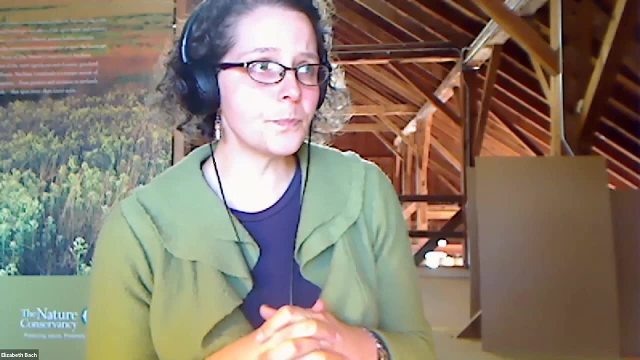 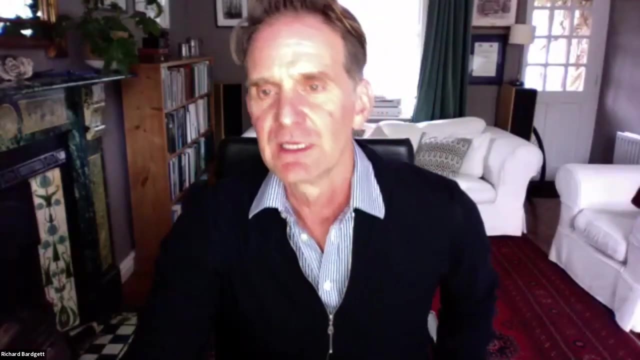 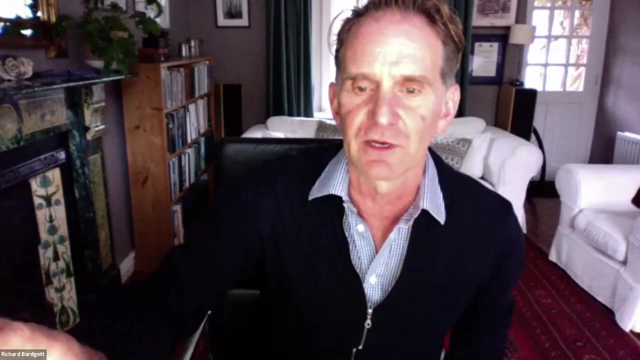 soil, biodiversity, and we're learning more and more all the time about how we can be a good partners, and we're learning more and more about the active role these organisms can play in restoration and rehabilitation. Thank you, Elizabeth. I think this is quite an important question because it's one of the issues that is often discussed by policymakers, for example. so I'm going to actually ask all our speakers. before I do, I just want to remind the audience that if you want to ask questions, please ask them through the Q&A session. 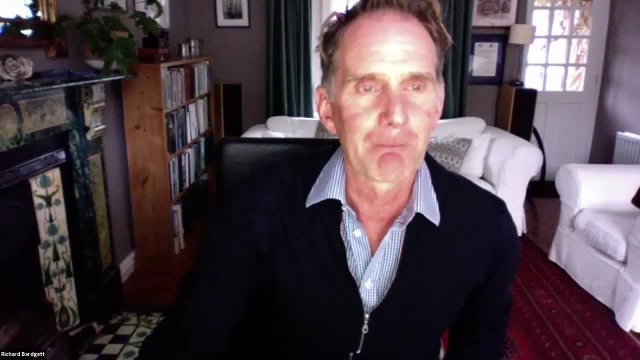 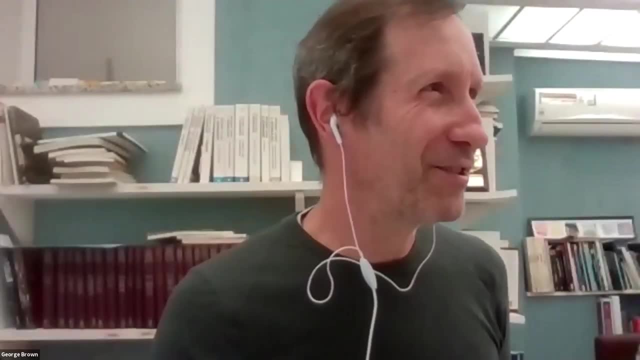 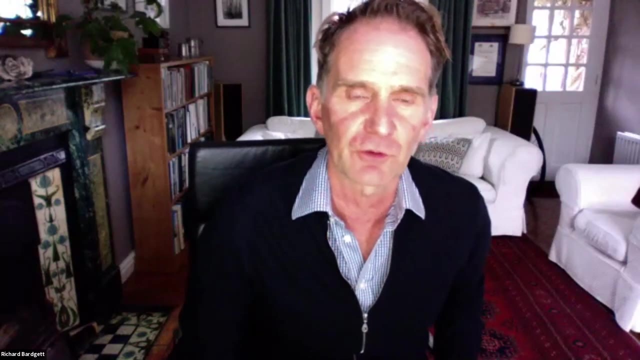 so I'm gonna go to George first. so George, you have to unmute, sorry, just a minute. repeat the question again so i can place it's: how can soil biodiversity be used as an effective agent for soil remediation under stressful conditions? okay, i will speak from where i i come from in the knowledge of the invertebrates. 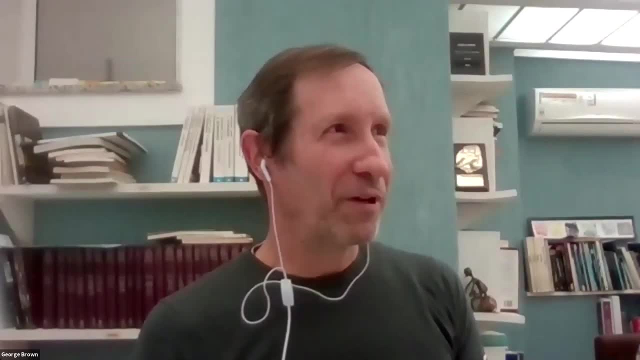 and in fact, before you can provide adequate condition for the invertebrates to to help in the remediation, you need to provide what they need to survive in those conditions. so, at top soil remediation, including, you know, revegetating, providing food, organic matter and all those sort. 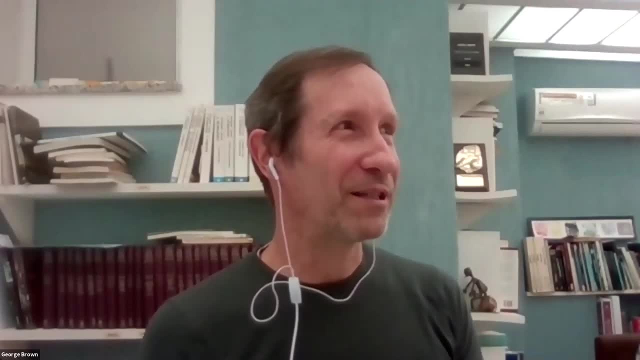 of things. so, basically, if if these aren't provided, it's very unlikely that there's going to be a whole important, really important role of these organisms in helping to remediate these areas, and this is, for instance, quite uh common in in mine mined areas- that then 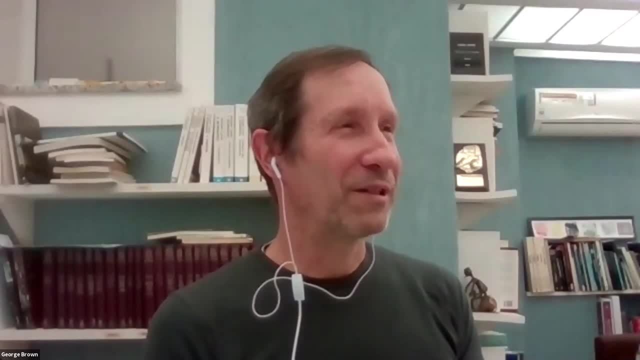 have top soil placed back and of course it takes quite a while, depending on the quality of the soil that's put back and how many stones and how much organic material has been put there. but, yes, once though they're there, there's even some really great examples of earthworms being 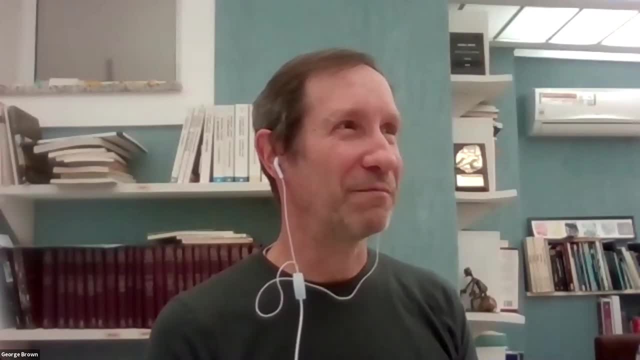 inoculated, and how many stones and how much organic material has been put there and how many stones and how much organic material has been put there and how many stones and how much organic material has been inoculated again into some of these systems to help promote um. 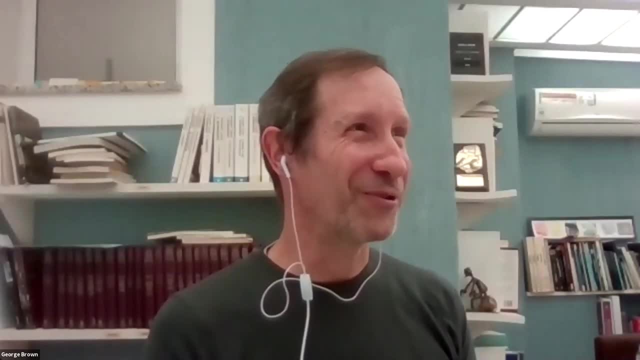 basically restructuration of this, of these unstructured soils. so, um, there, it's really important to provide the adequate conditions for them to come back. once they're back, of course, they're going to contribute more and more importantly as time goes by, to the restructuring and 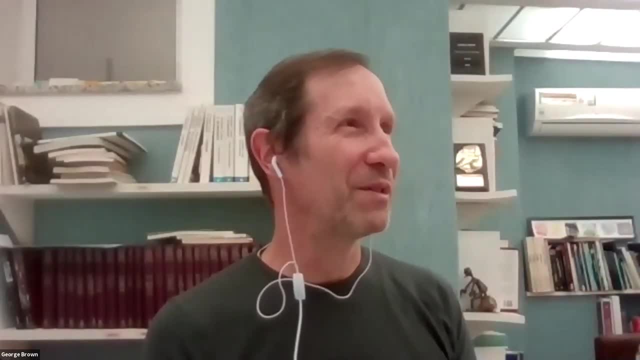 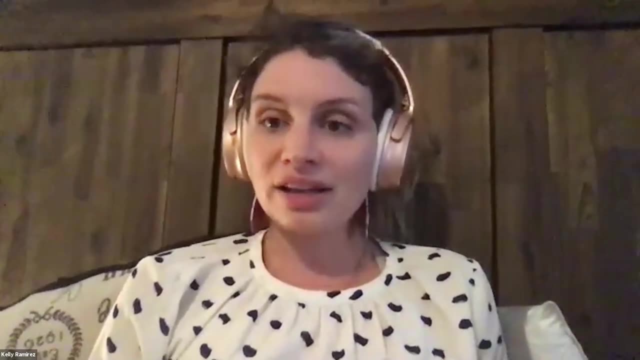 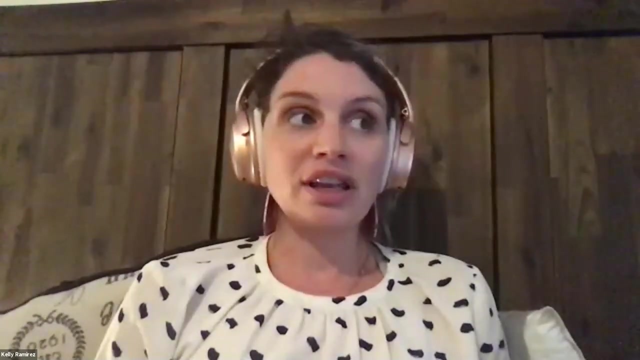 and re recovery of those of those uh systems. okay, thank you very much, george. uh kelly, if you could give us some perspectives, yeah, i think i'll. i'll answer this more from a global change perspective. um, and something i've been thinking about a lot lately is, if we want to. 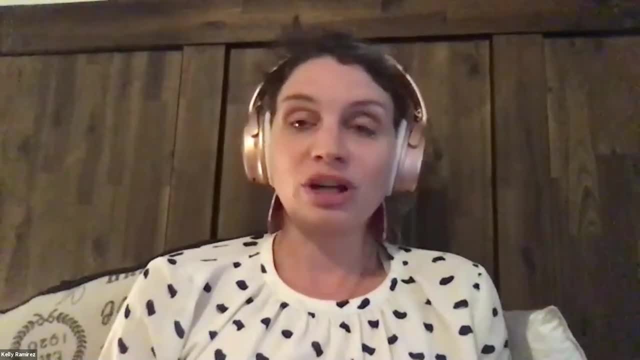 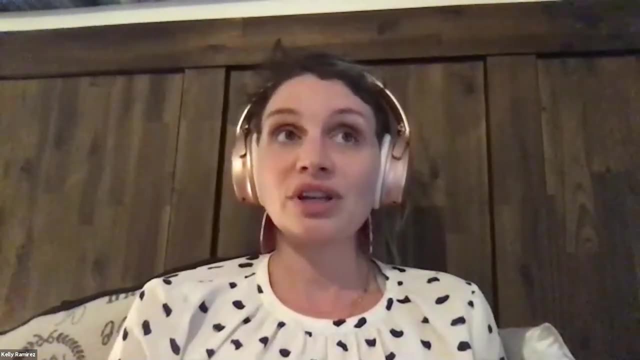 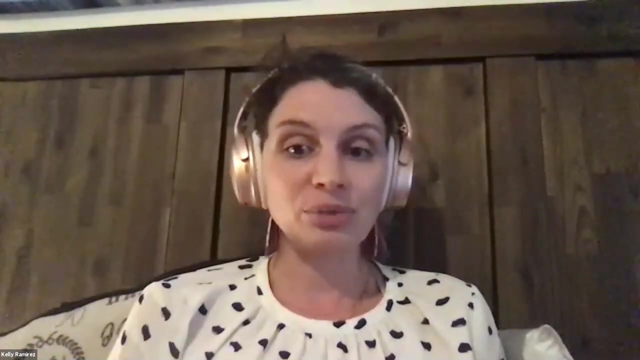 think about, um, bringing soils back to their whatever healthy state or remediating them. um, we also have to think about your. your the question asked under stressful conditions, but we could say under global change. so what if those that ecosystem now is warmer or is getting different levels of precipitation and we're not going to be able to get them back to their 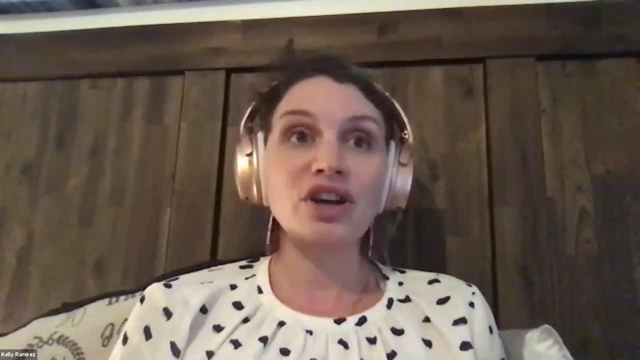 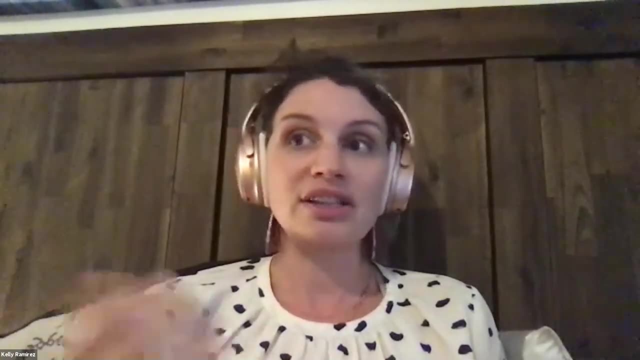 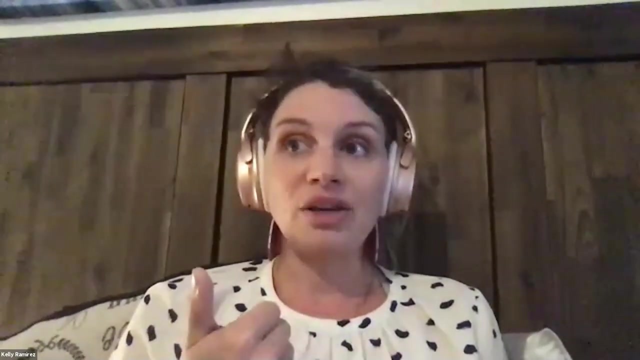 or these different um right pressures on the system. we can't just say we want to go back 100 years because there was grazing here at. you know, at the turn of the century they started grazing and we want to go before that. it doesn't it. we can't do that in most places because one um the 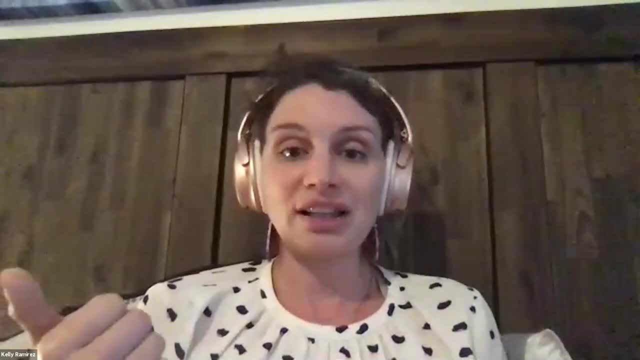 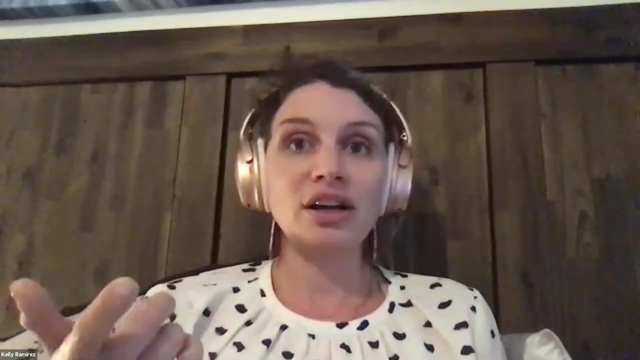 people are still using the land, and so we need to think about who's using that land and why. um, and we're not just gonna like say, oh, we just need to put this back to its pristine state. two, because if we don't, we're going to lose some of our biocomposting resources that we're going to waste. 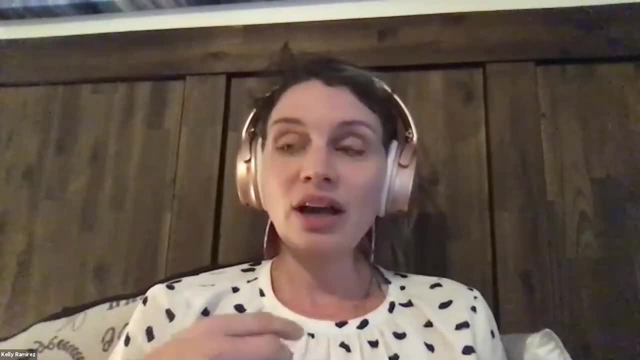 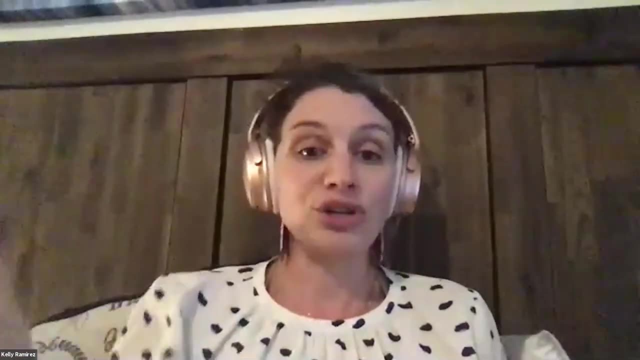 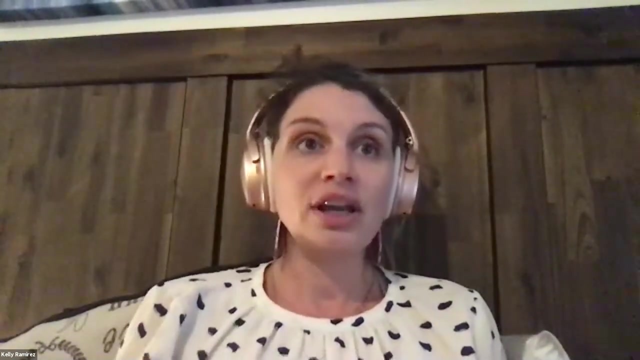 on our everything. um, we can't really do that in the in the future, but i think that the the environment now has changed and the climate has changed and those changes are affecting soil biodiversity, um, and i think that we have to strategically create uh experiments that test. 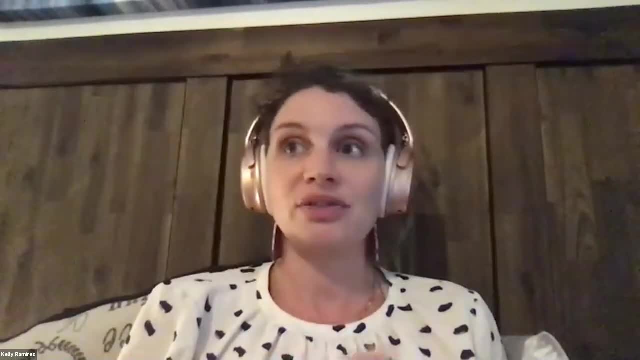 and kind of project into the future, what, uh, those stresses will be and if it's a right to remediate or restore soils, if it's in a mine, it's much more like harsh um and maybe that makes a lot more sense, whereas if it's in a grassland and there's been some grazing, how can we work with land management and what do you see as this change in the future? 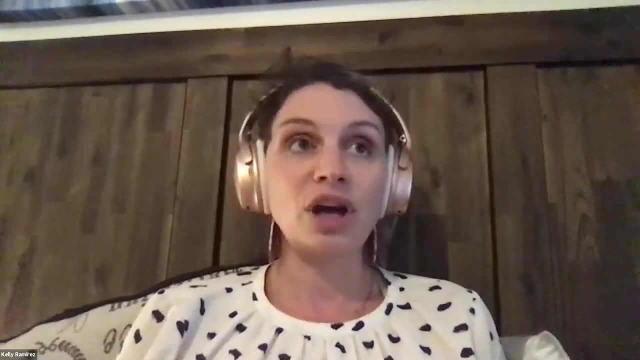 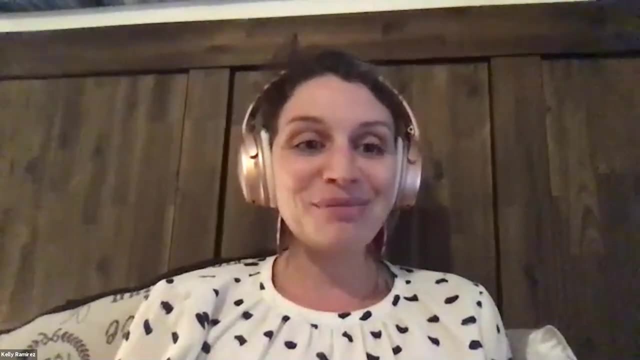 to say, okay, grazing stays, but we want to still get a lot of ecosystem services out of it, right? so always comes back to it depends which system we're in, but I do think it's a really good question and something I hope that research continues in, because it's definitely 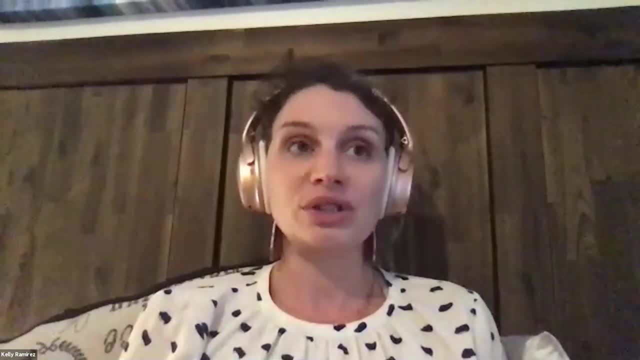 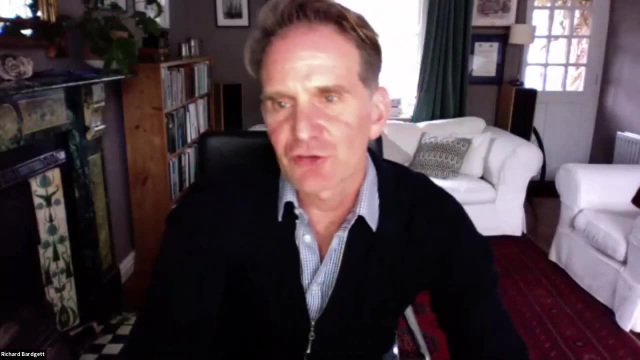 better, kind of like a. there's a lot of these sorts of questions that soil biologists can answer or start working on now. Okay, thank you. I'm actually going to change to another question now because I see that we've got a few, but I'm still going to ask Zoe this question because I 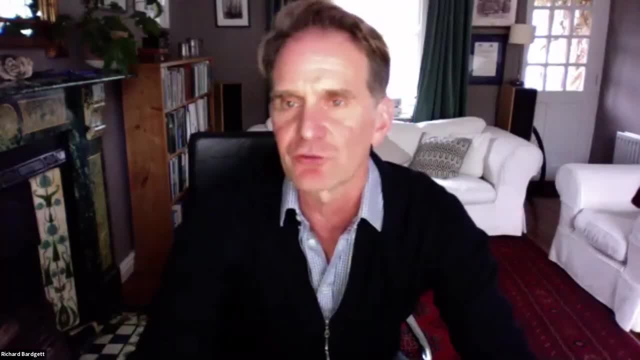 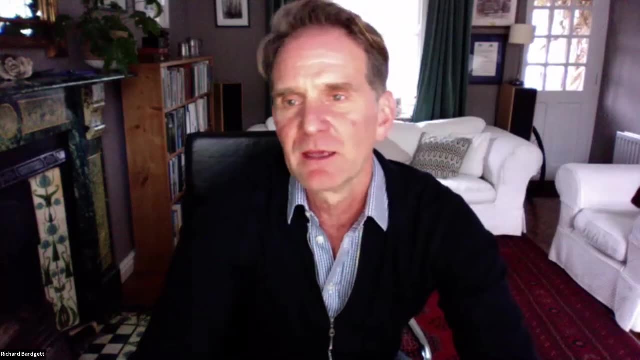 think this is a particularly important one. this is from Sally Bunning. I should say that the previous question was from Eamon Elberdry- I hope I pronounced that correctly- but this question from Sally is. she says that I think we need to also focus on how we can get practical applied knowledge from 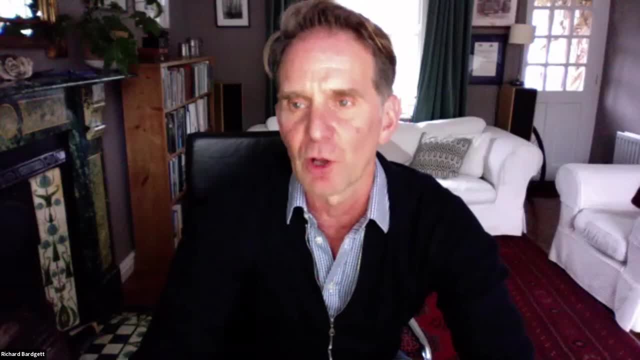 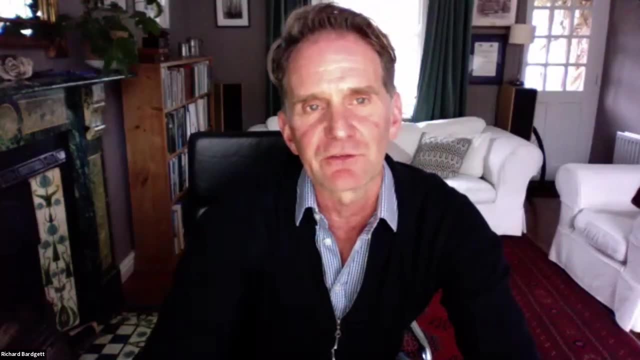 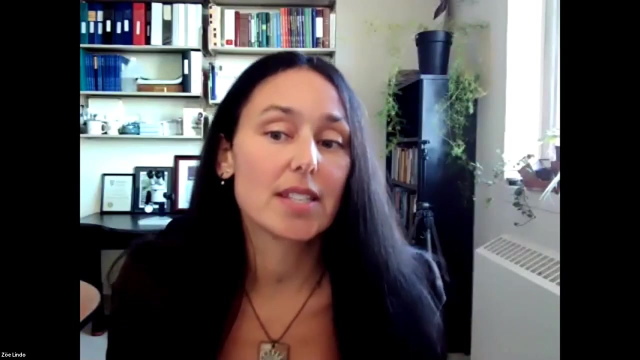 research to farmers and other land users and pollen makers to reduce the use of agrochemicals, etc. So I wondered if you could give some insights in how you think best to achieve that. Thank you, Richard. yeah, I agree, this is. this is also an important question and in many ways I 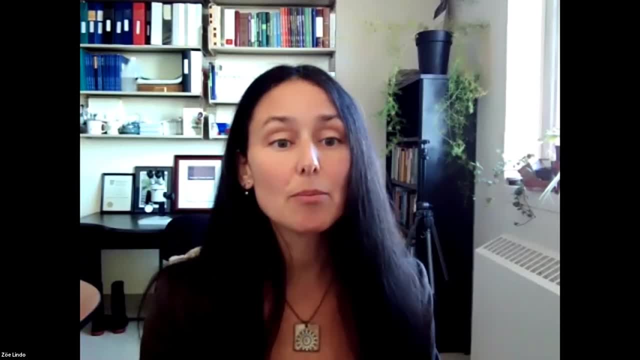 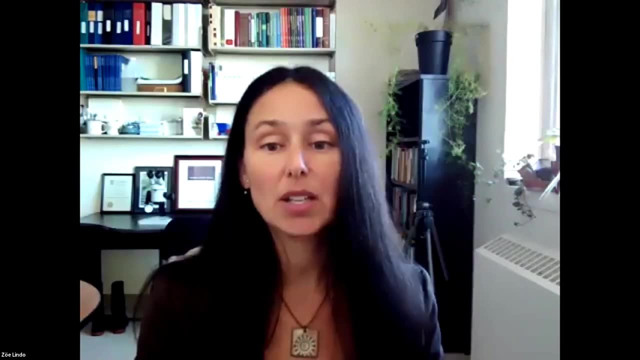 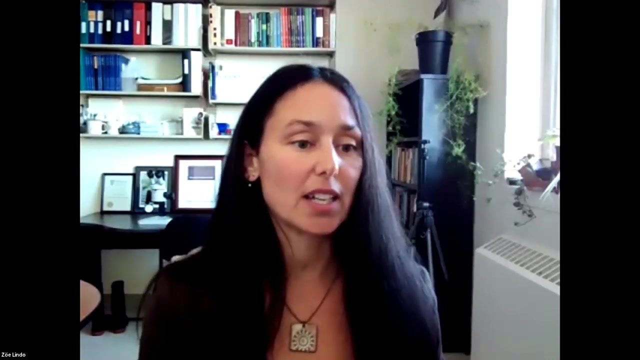 think it. it relates to our first question as well, which is the impacts that we're having on soil systems at local, regional as well as global scales, in terms of some of the stakeholders like like farmers, and some of the local scale. I think you know, here in southern Ontario we're actually highly agricultural as well and have been. 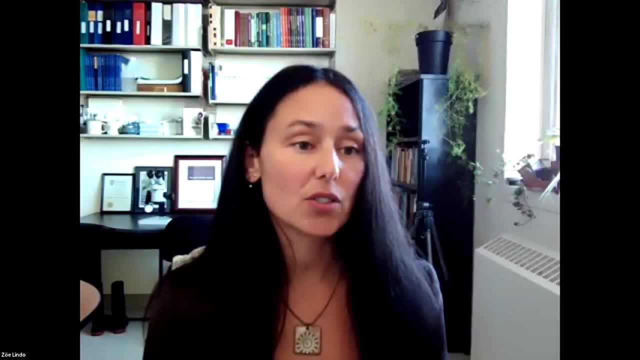 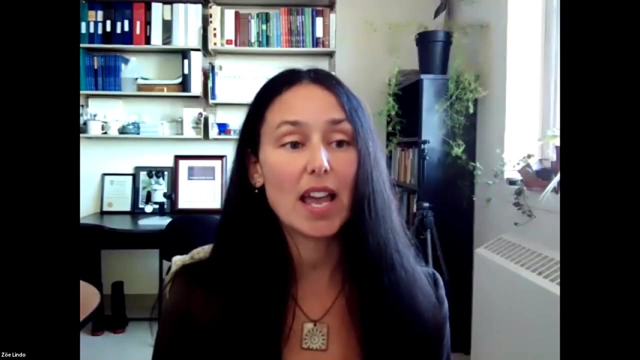 for for over 100 years, and so our soils are relatively reduced, and so some of the the ways that we can reach out to farmers is by getting them involved in active research as well, and so initiatives where we have students that can go and set up experimental treatments. 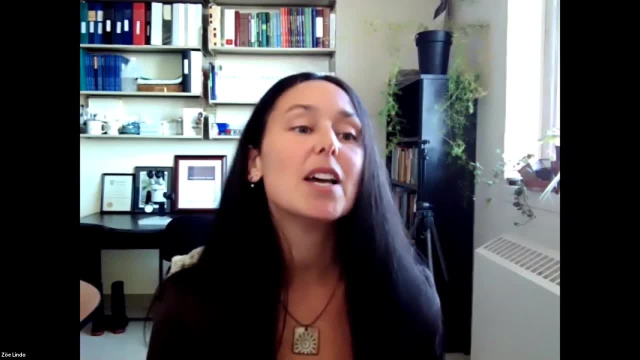 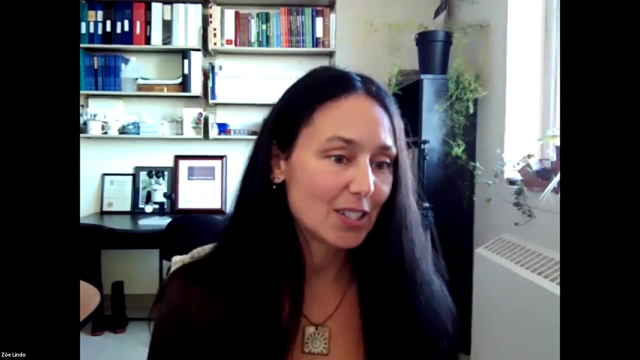 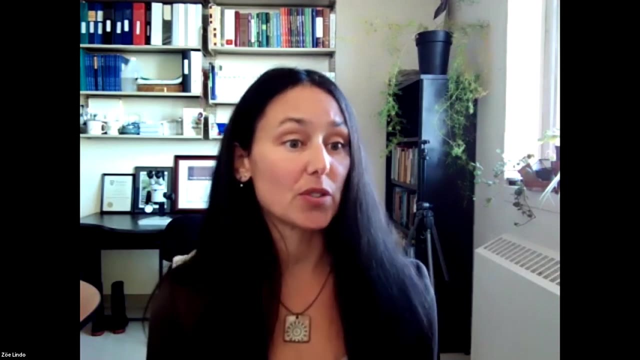 try different intercropping systems, vegetative cover and things like that, and I think that relates back to what George was saying in the first question, that it's really about some of these basal resources for supporting the soil food web that are going to make the soil system healthy, or 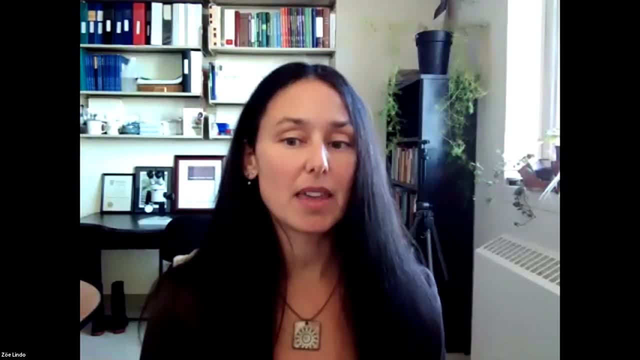 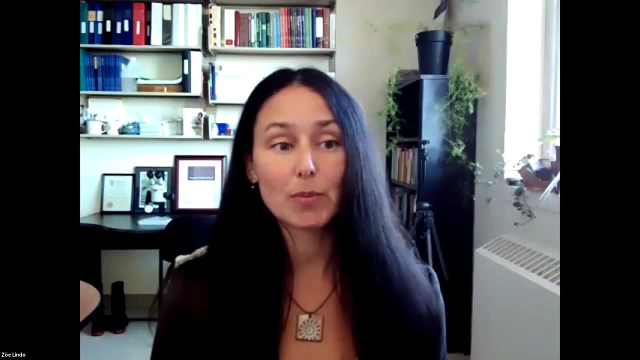 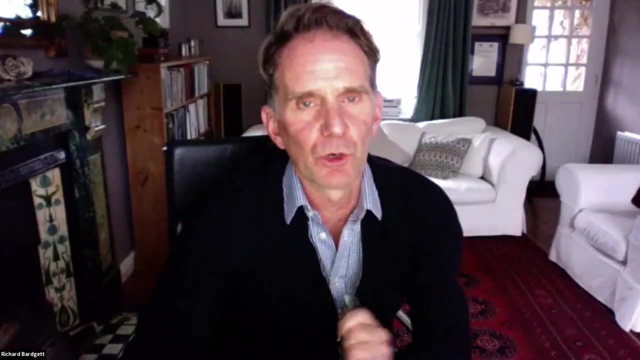 stable or whatever we would, we would like to call it, but I think getting getting farmers involved in, in active research, whether that's at small or large spatial scales, I think is a great initiative. Okay, thank you. I mean, Elizabeth, you're actually working on issues related to restoration. 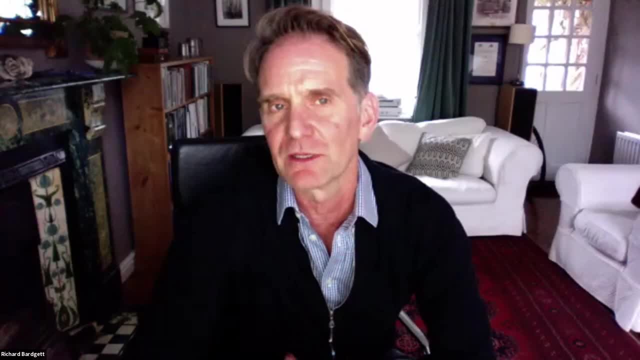 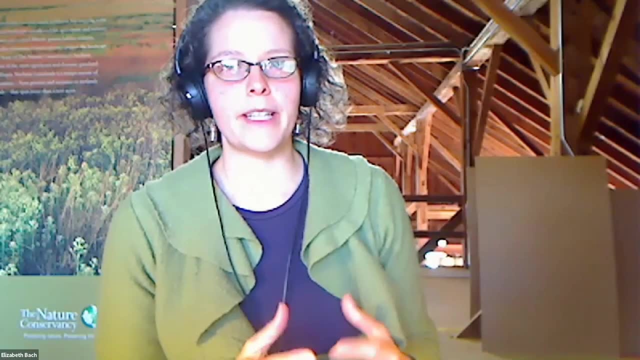 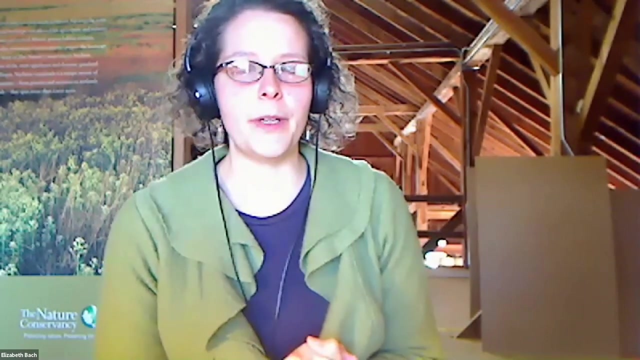 in tall grass prairies, So I wondered if you could perhaps give us some of the perspectives from that particular angle. Yeah, absolutely, And I work more directly with land managers who are actively working on restoration projects, But I'm also located in a very agricultural community, agricultural context, And there's a tremendous amount of 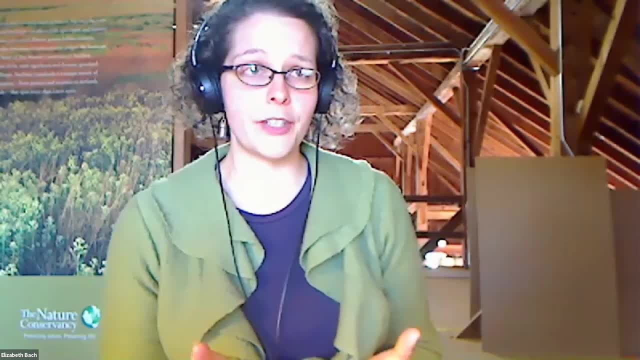 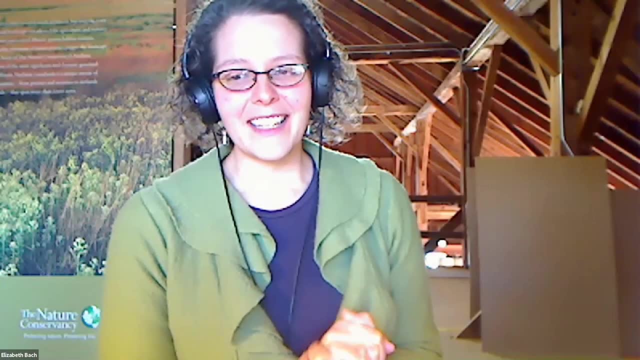 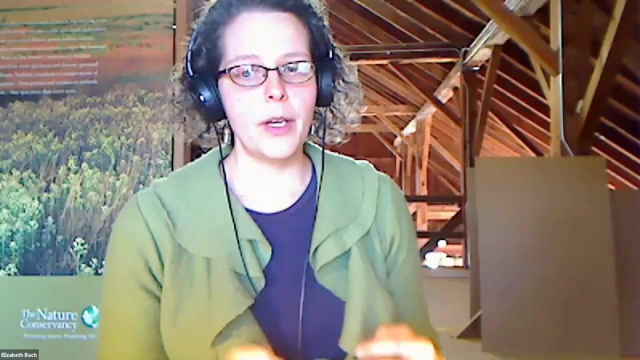 interest I find amongst land managers and farmers. I come from a farming family so my own family brings this up on occasion too And I think that just feeding that interest is really going to help us take some big steps forward And recognizing that it's okay that 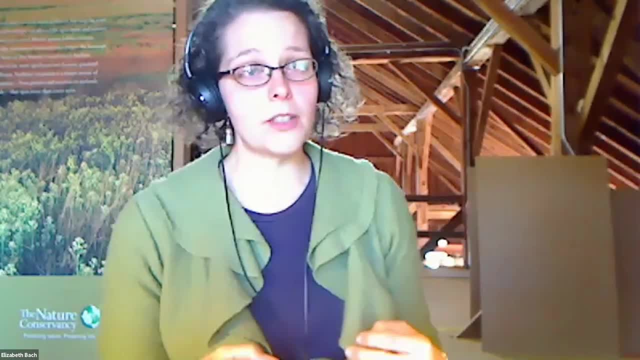 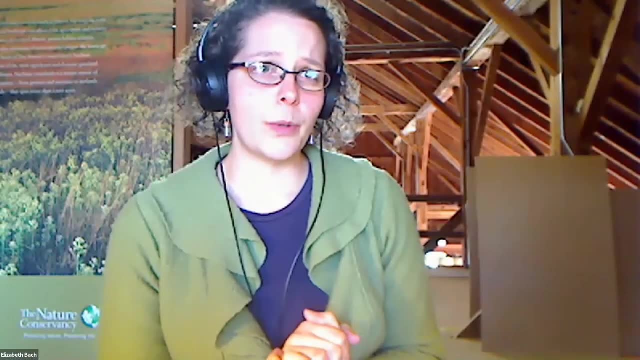 it's complicated and that we don't know all of the answers, but to be sure that we know some and we can, We can make some good recommendations for steps forwards. And I think Zoe and George's point about feeding the soil community. I think of it as feeding the soil community, so it can feed us. 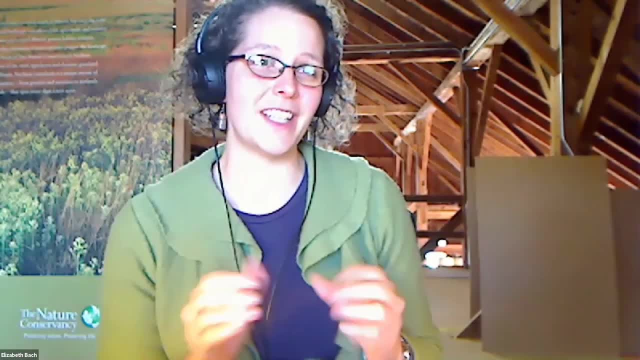 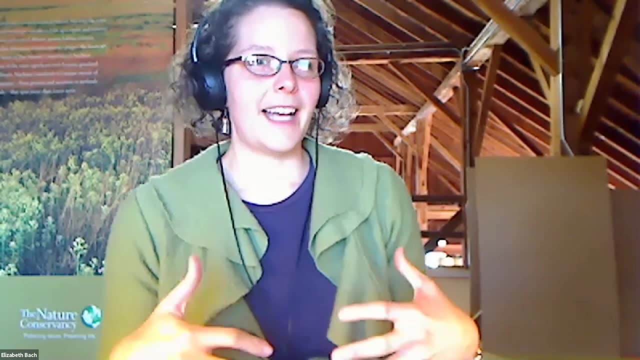 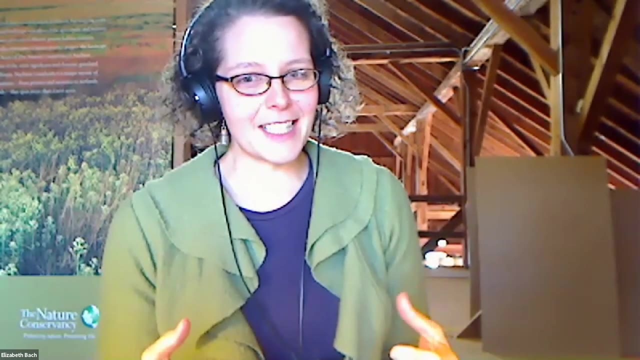 and really thinking about it as a whole cycle. It's not just putting your crop in in March and taking it out in October. It's about what's happening over the winter for that system to be ready to grow a crop next year. And if we're thinking about it in that sense, we can also 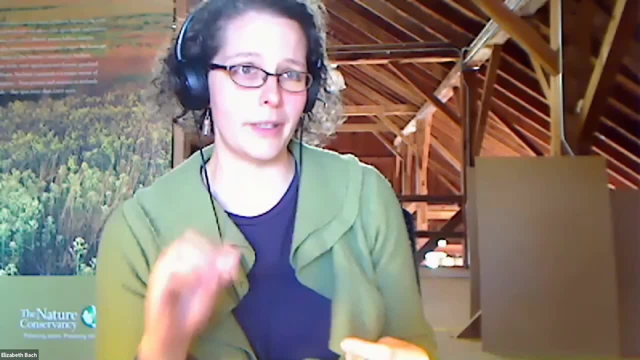 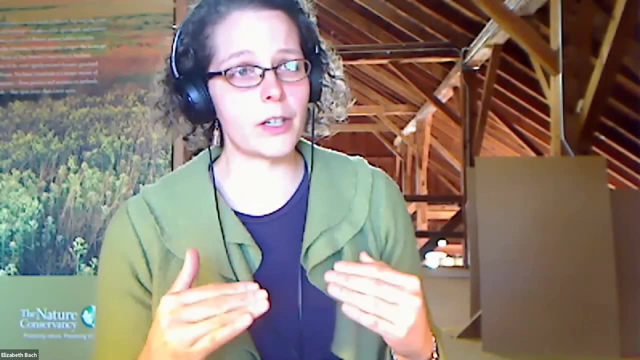 take a step back from thinking about: oh, I need to do a checklist of inputs every year to make this happen. And this comes down to that direct question about agro inputs: to realize what our soil and our soil communities can provide by themselves And in some cases we may need some. 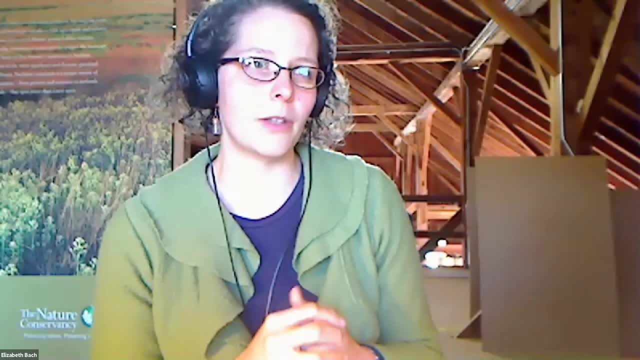 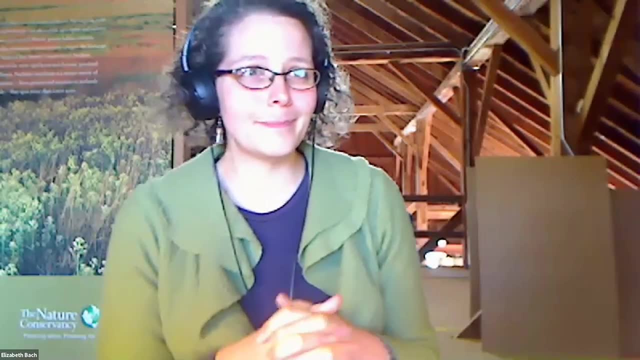 additional input, but to do that in moderation and thoughtfully with the whole system. So yeah, I think there's interest there And these are really important areas for us all to be engaging in. Thank you, I mean, this is really. 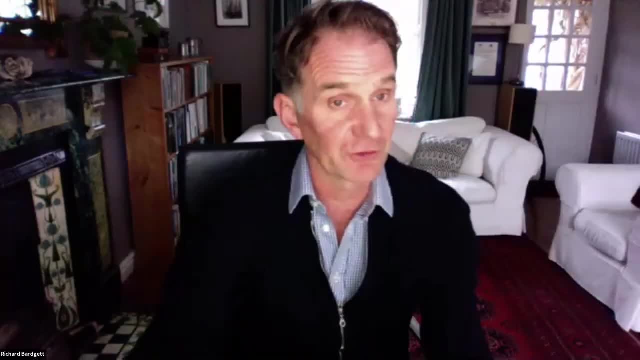 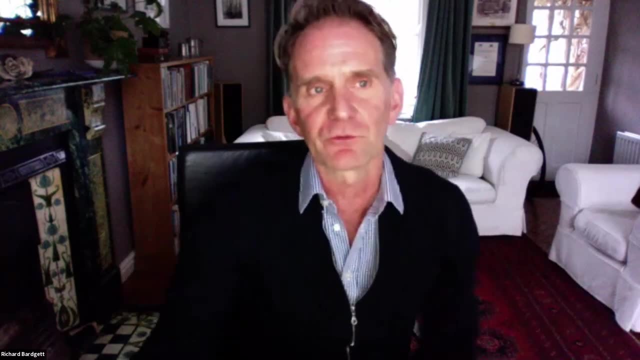 a key topic in soil biodiversity research and also for the report. So I'm just going to get one more perspective- actually from George- on this, because you work in very different systems- agro ecosystems in Brazil, for example- So I wondered if you could. 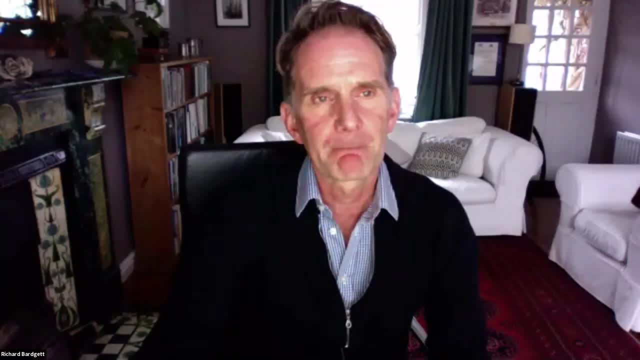 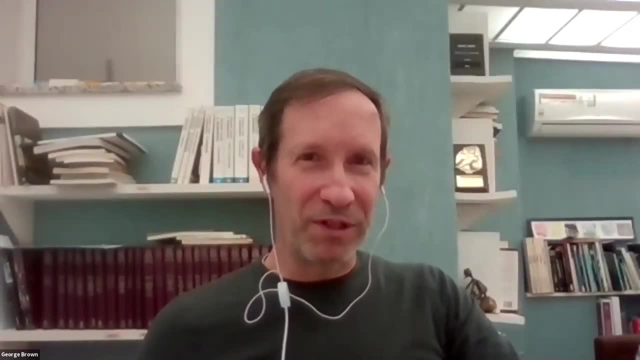 give us a few of your perspectives as well. Yes, actually, there are two very important things that occur in Brazilian agriculture which have to do with soil biodiversity. One of them is the very large amount of no tillage which is used in our country, And we know. 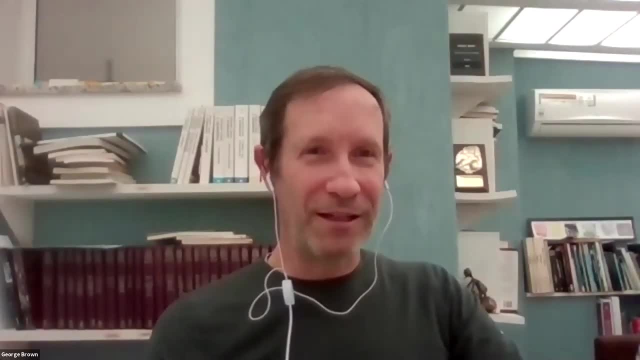 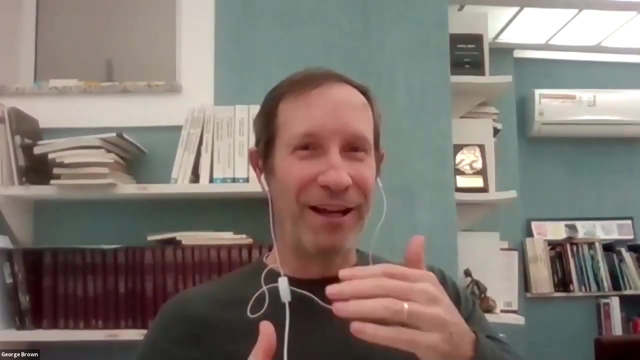 that by fact, many experiences showing that this is a system where many of the soil biota have a very important role And yet there's still improvements that can be made in that, so that there's a synergistic working in the sense that, you know, not only are you providing, lack of 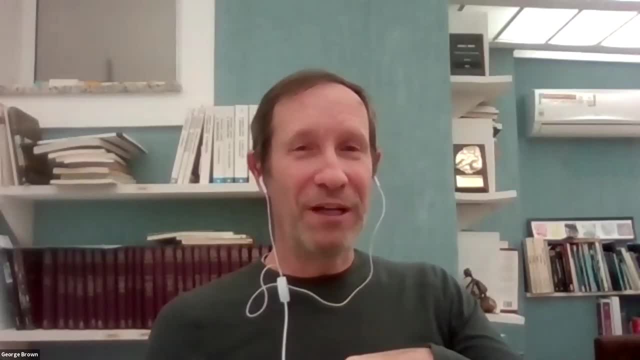 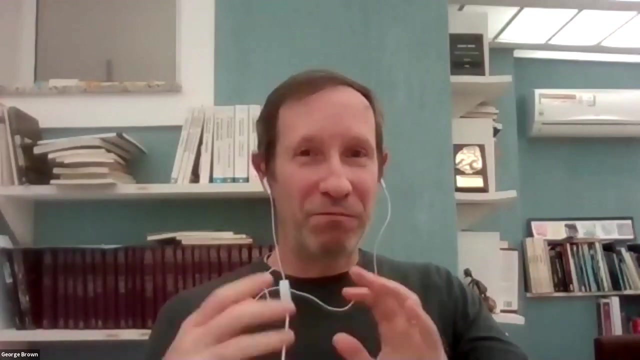 tillage so that there's more protection of the soil, but also providing the adequate- you know- inoculants, the adequate crops that can fix nitrogen, the microbes that can contribute to- you know whatever, rock, phosphorus solubilization, all sorts of aspects of this interactive and synergistic management, you know. 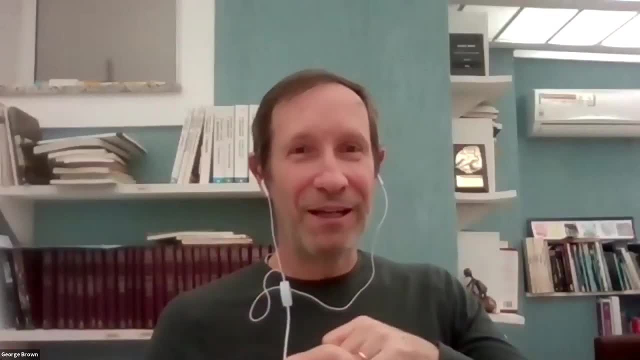 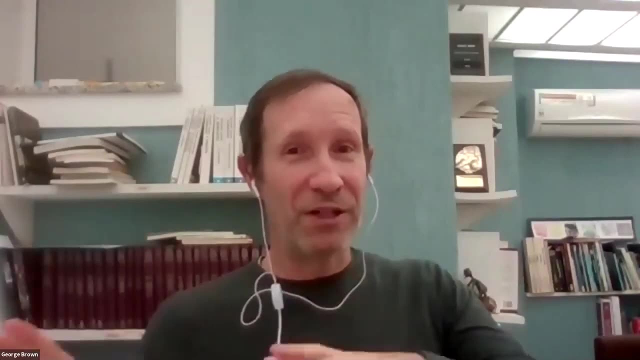 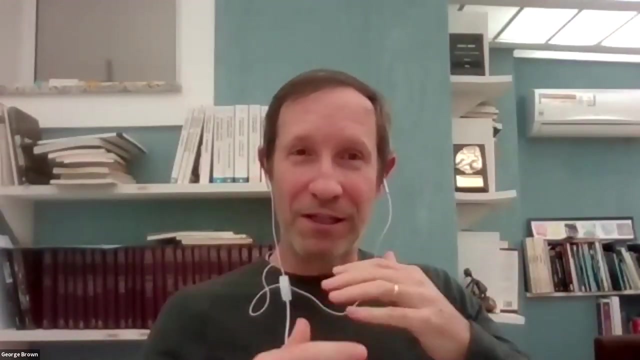 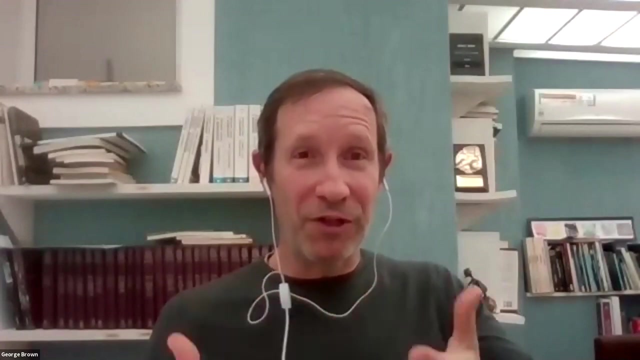 the crop rotations, not including trees, including what we call here in Brazil the integrated production systems, where you have rotations, with pastoral period, with ferment, with crop, with plants that are fed, feeding animals. All these contribute to basically improving the soil biota and reducing inputs. So this has been a really great experience here. 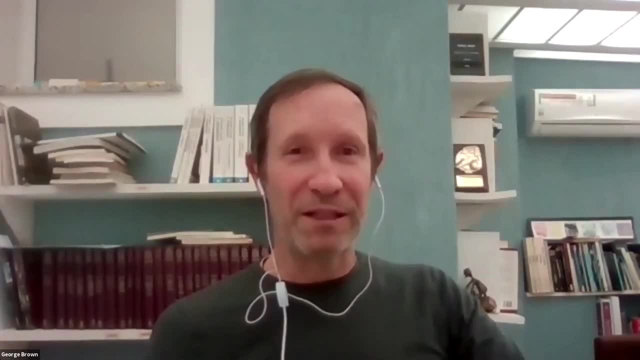 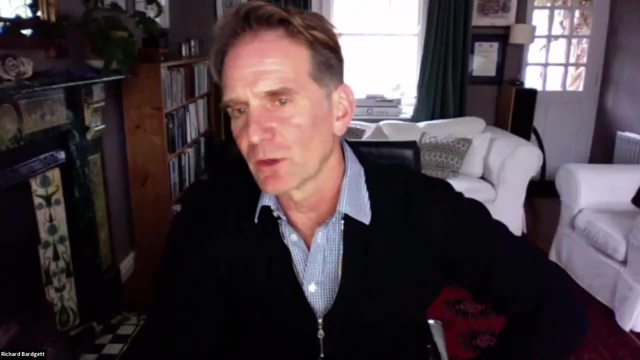 in Brazil, And I think it's applicable to many other places in the subtropics and subtropics worldwide. Thank you, Jorge. I should say we also had another question which is related, which I think has covered that, and that was from Ellie Moriam, which was about how we can integrate knowledge on biodiversity to land. 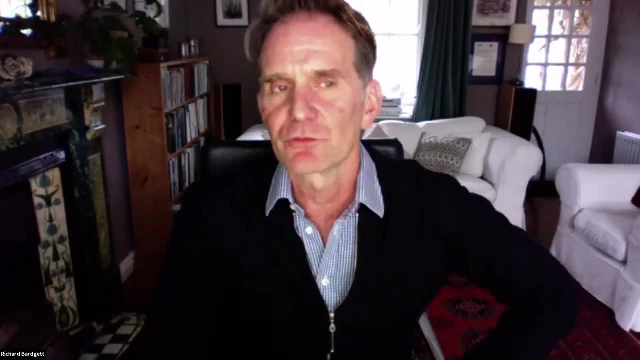 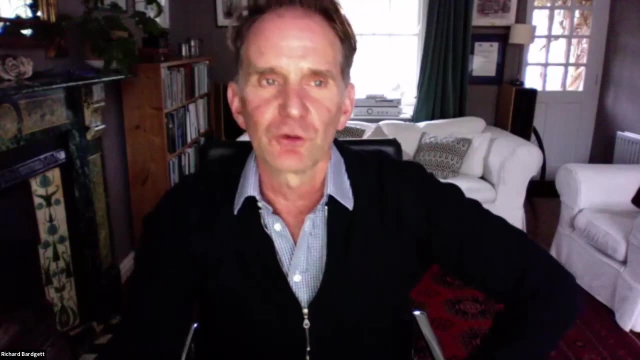 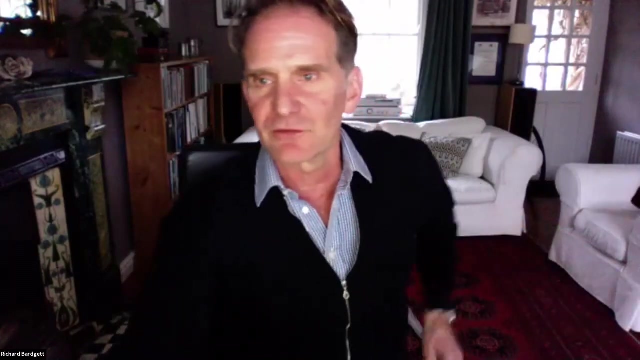 management, But I think that's sort of been addressed to some extent in those questions. Now, another topic that seems to be coming up quite a lot in the questions is to do with global scale analysis of soils, in that there's been quite a lot of effort recently in creating databases. 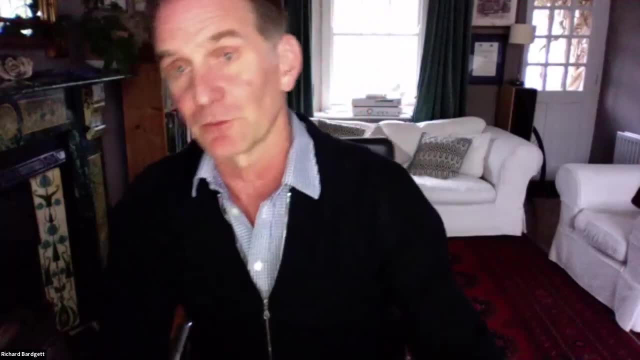 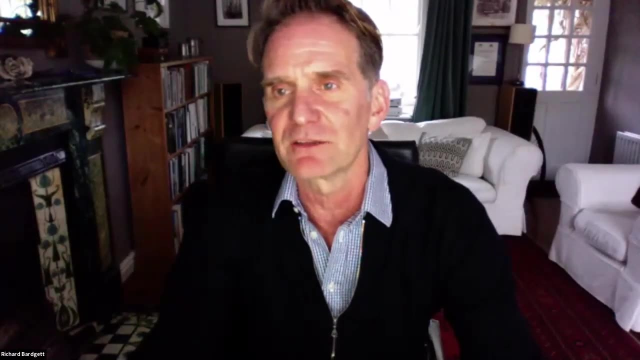 It's been also revealed end that there are some blind spots in those databases, databases, and there are two questions that come up, very similar ones from Louisa Durkin, which is: if you are looking to identify risks to soil health, what global sets are the most meaningful? 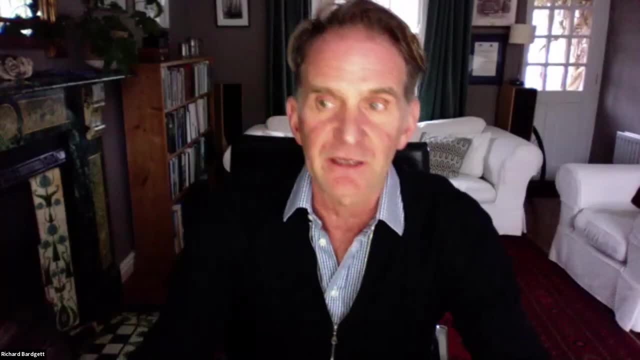 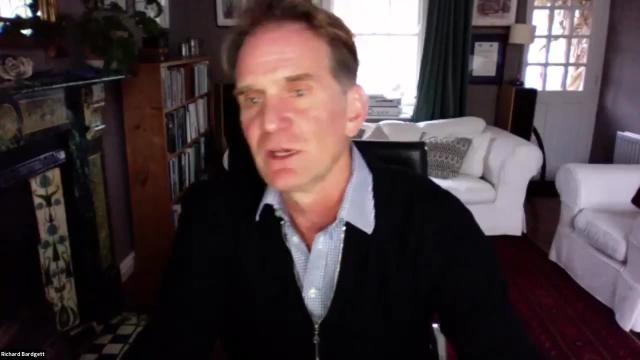 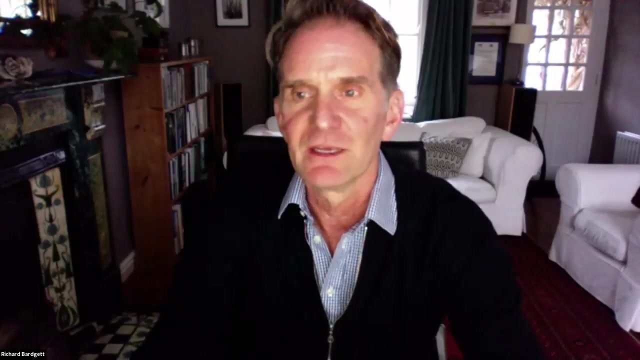 and, more specifically, what global data sets. things like carbon erosion, soil depth, etc. are most meaningful, and also one from Paul Cardell which raises a similar issue, but it's about global maps and the gaps that exist, in that most of the data- about 90 percent- is coming from Europe North. 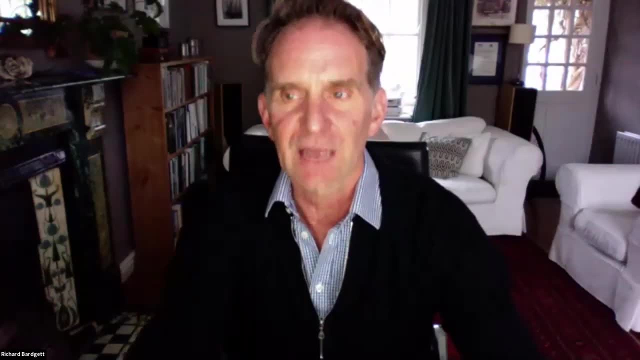 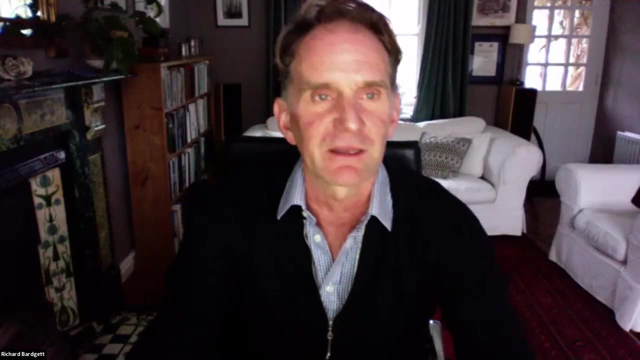 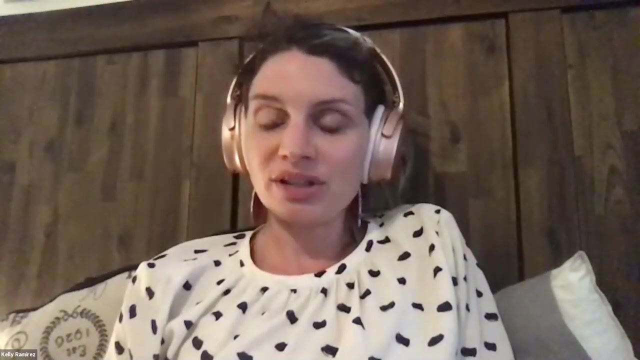 America and parts of China, and he's asked what initiatives can we take to fill those large blank spots in other continents? and I'm going to take this one to Kelly, because I know you do quite a lot of work on global scale analysis of soils. Yeah, thanks. thanks for the questions, Louisa and 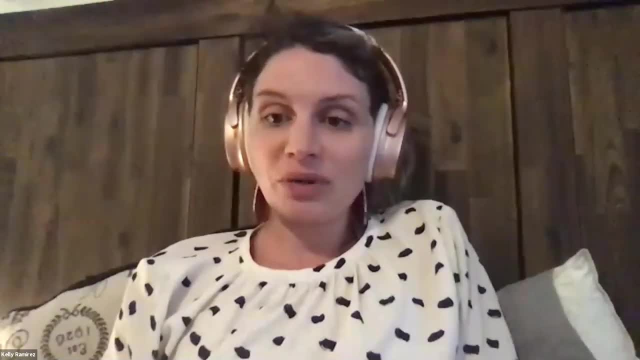 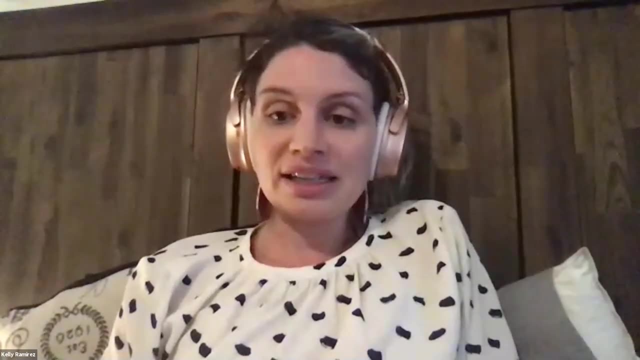 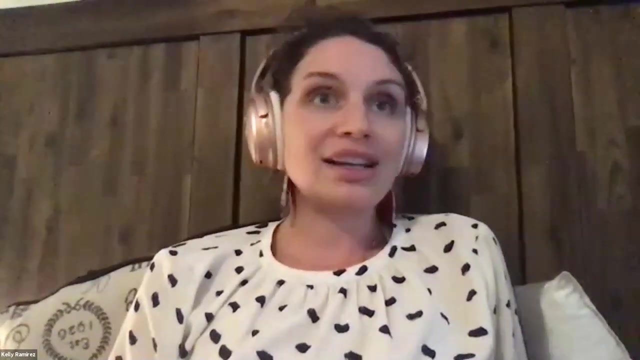 Paul. So I'll start with Paul. I think this is a really great question. we've seen a lot over the last 10 years really, Since high throughput, sequencing of these global studies, and you're right, they are mostly in a few select areas and I think some ways around this we've seen is collaboration, working with scientists. 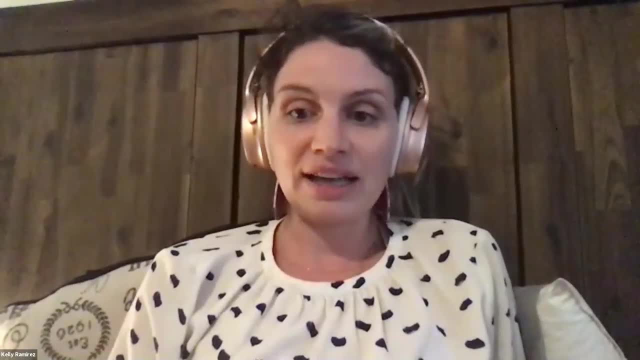 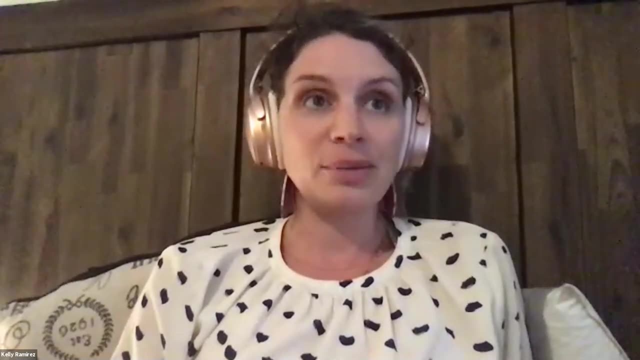 in other countries and finding ways to collect more data, and that's one reason the report, the value of this report, is to really highlight there are some big gaps in where we're sampling and so that's like one of the hopefully the solutions. if that's a huge gap, then we come back to the 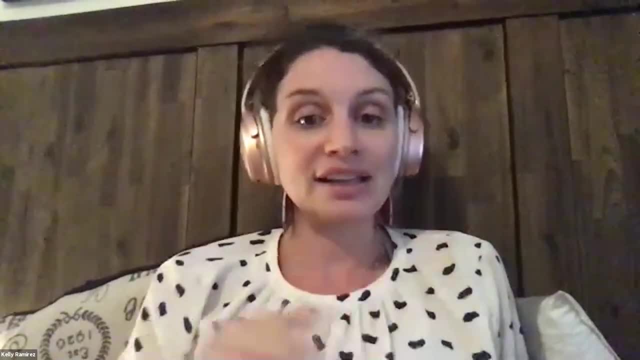 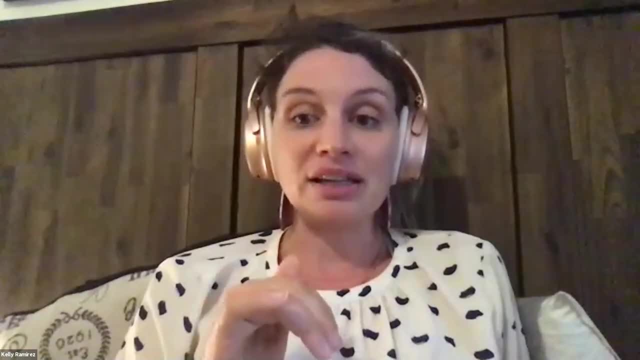 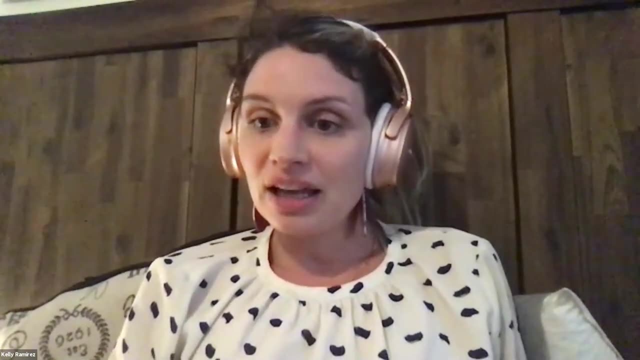 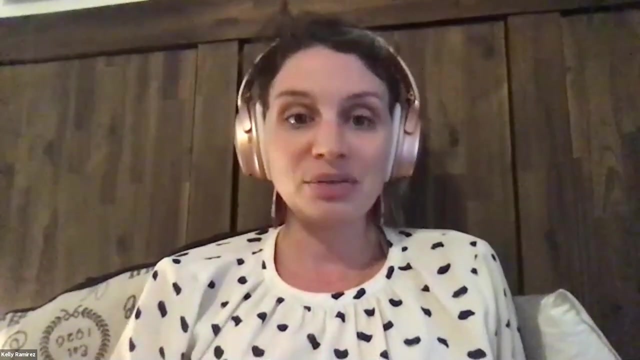 like getting us to do that research, whether that's funding, whether that's whatever, what ever mechanism that is. So I think this report like this is really important. Let's see I am reading. I think I do think something else that your kind of got out here is and then goes to Louisa's. 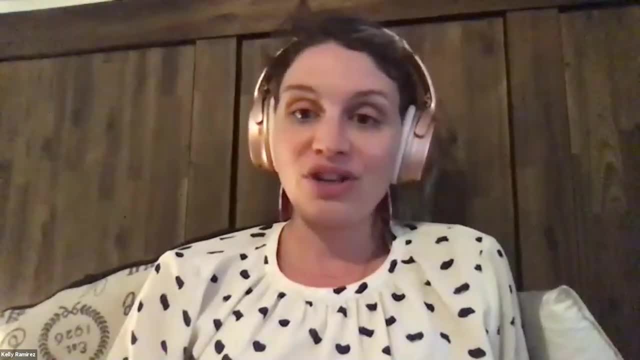 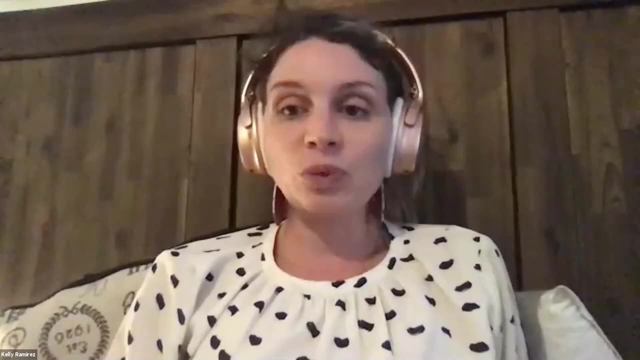 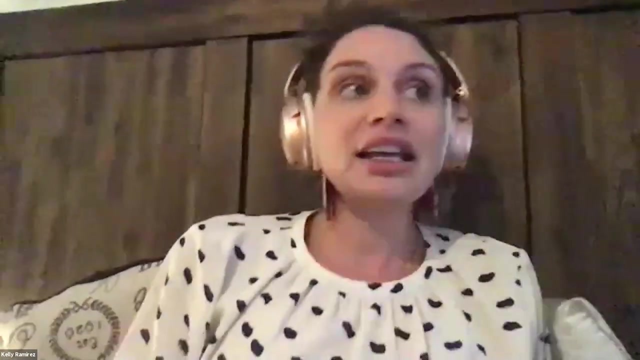 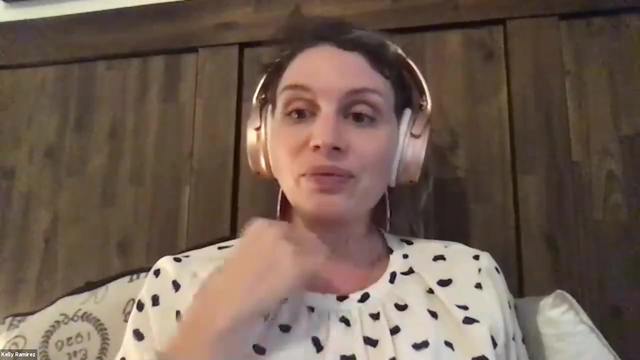 question like: what information is the most important diversity hotspot? sure, abundance and diversity is really all we need, But what about these other soil metrics like carbon erosion, soil depth, etc. And I think it depends on what organism you're thinking of this or what ecosystem service you're thinking of Getting them all? 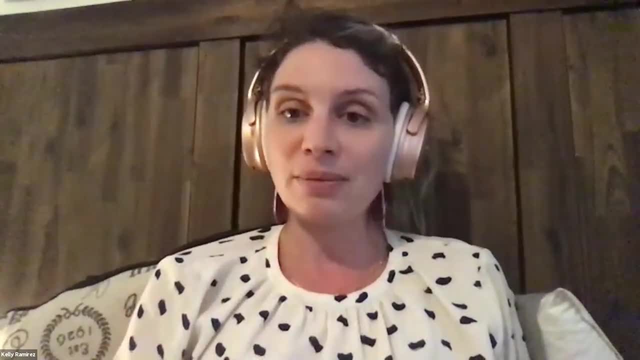 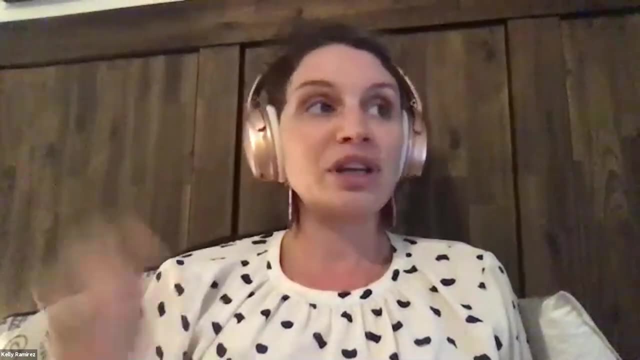 overlapped is still pretty difficult. right, We have a new paper out on earthworms and the distribution globally And we can relate that to plant diversity and carbon. But how do we start to integrate in fungal diversity or bacterial diversity And then within bacteria? 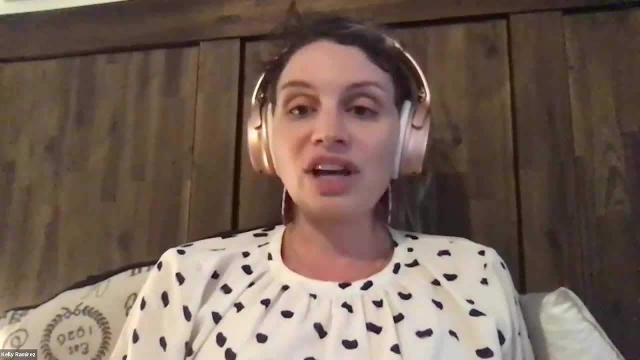 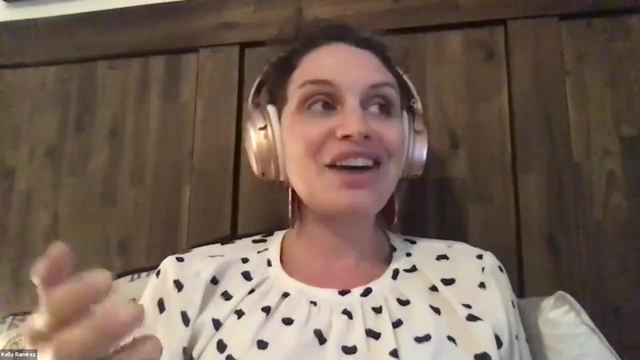 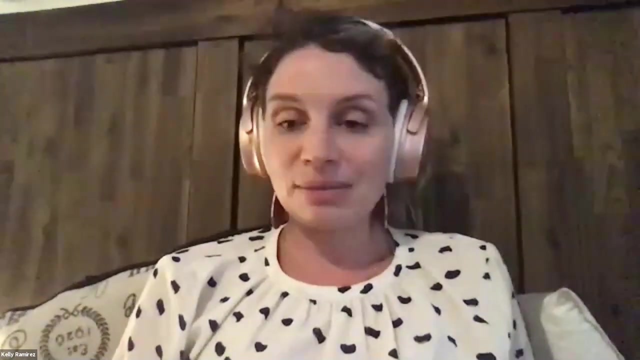 what are those specific functions? And I do think that we've kind of reached a point where we've made enough maps with the abundance and diversity, maybe, of bacterial communities, But now it's like the next step is functions and other organisms together overlapping. So somebody should write. 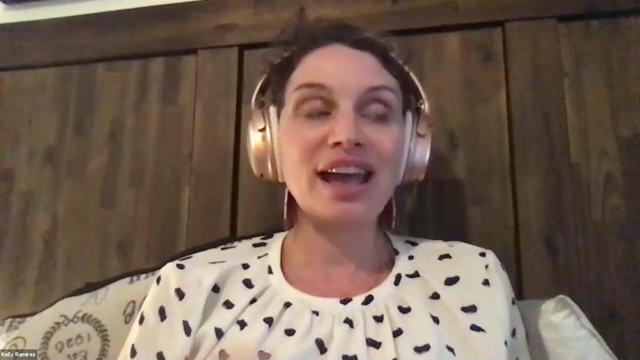 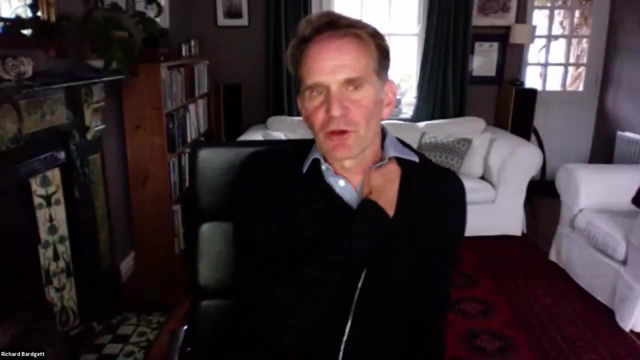 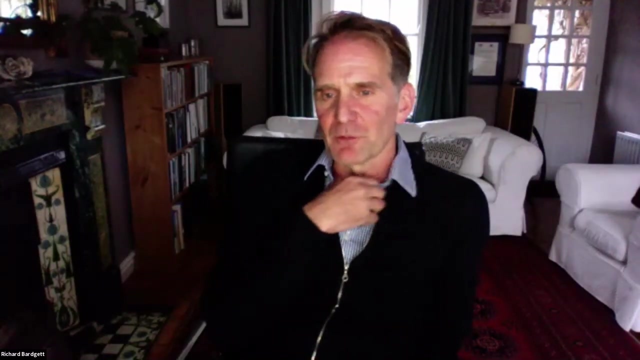 that proposal, But I do think these are gaps that we have highlighted in our report, So hopefully that's a direction that we continue to go. Yeah, I was going to ask a similar question to Zoe, actually particularly about these gaps in knowledge, which you know, as Paul has pointed out, is we have lots of information from 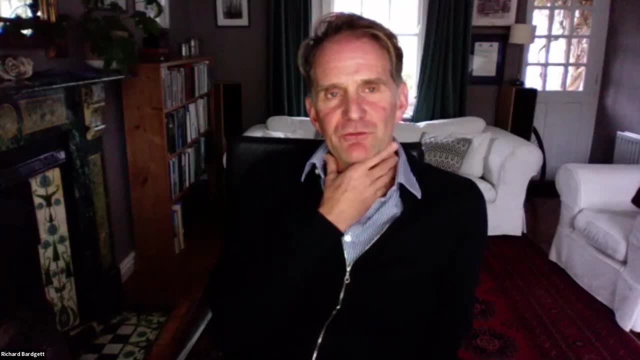 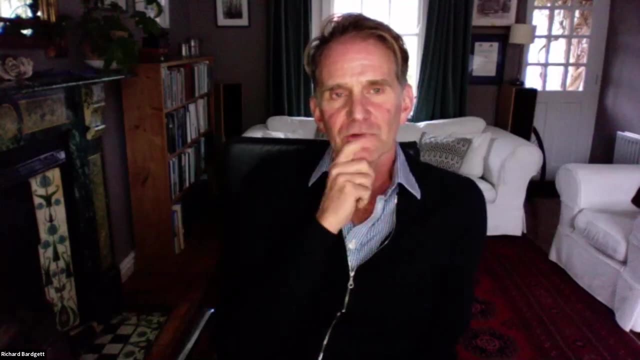 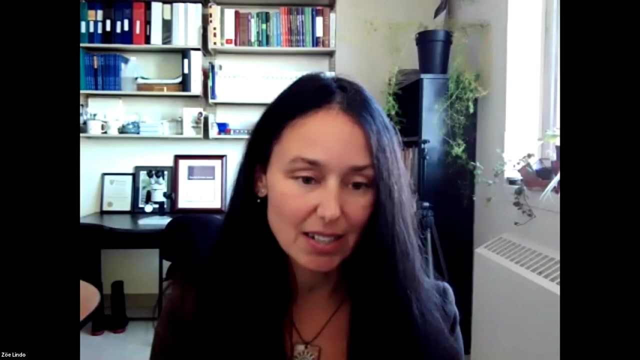 Europe, North America, etc. But these enormous or complete lack of information in other parts of the world, particularly Africa, South America, etc. And how can we actually overcome this? Yeah, absolutely Yeah. Thanks, Thanks, Paul. Yeah, How do we address these gaps? Well, my immediate response is: more money. 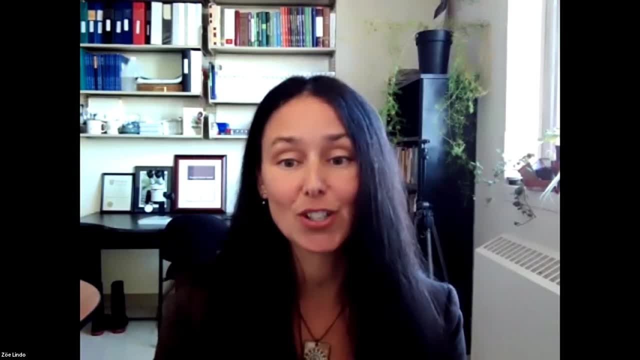 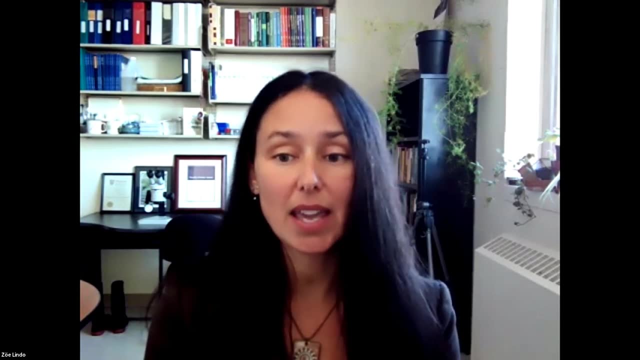 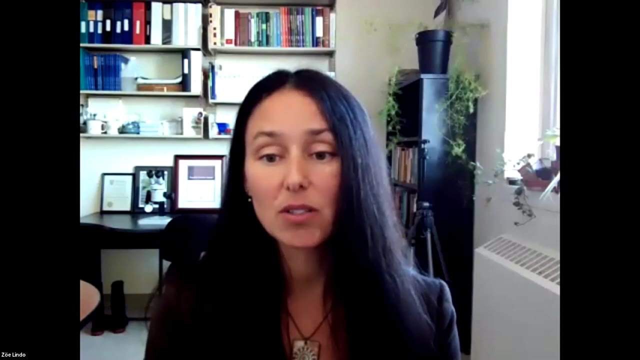 more funding, funding for basic research- But thinking about here in Canada, where we have such a big land base and we have so few researchers studying soil and soil biodiversity- it's exceedingly hard to get across the country, And so I think it's really important to address these. 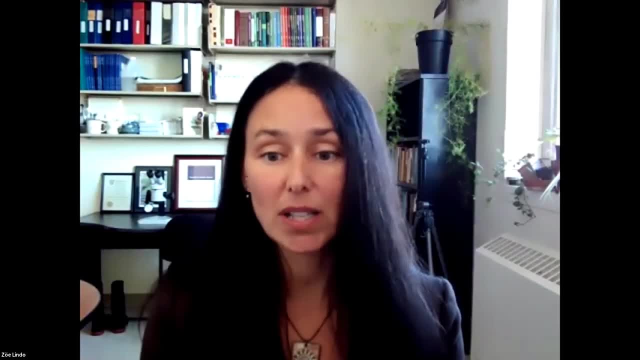 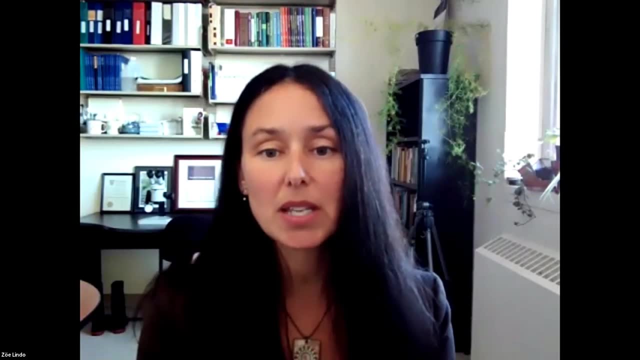 gaps and to actually understand who's there and what's there and fill some of these gaps. And that's where I think, coming back to the related question about some of these other global soil data sets, some of these can be, I think, indicators. So for instance, carbon, the amount. 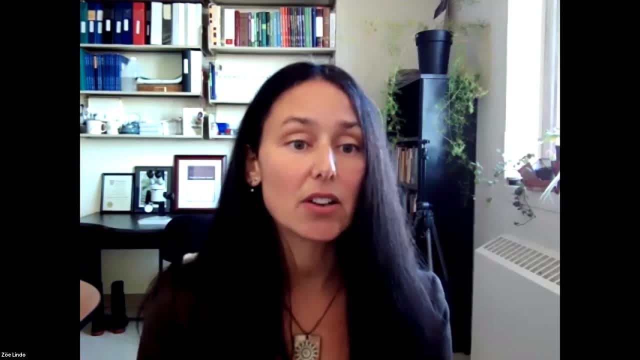 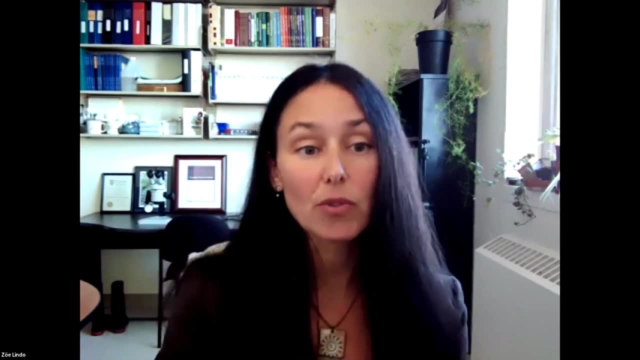 of stored soil. organic carbon is often an indicator, at least of abundance, for many of the major taxonomic groups. It might not be necessarily for the rest of the world, But I think it's definitely an indicator for the richness, but definitely it is for the abundance of a lot of the. 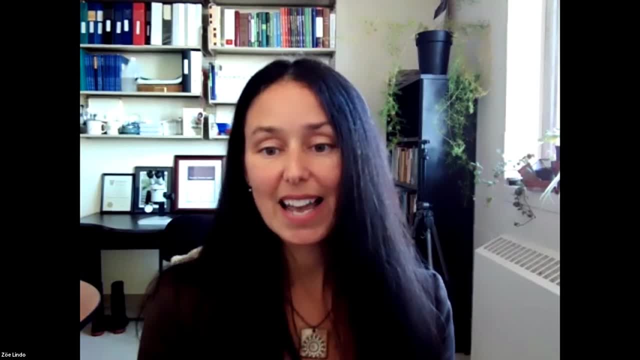 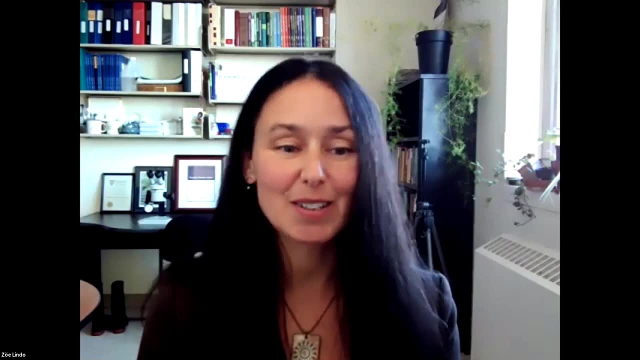 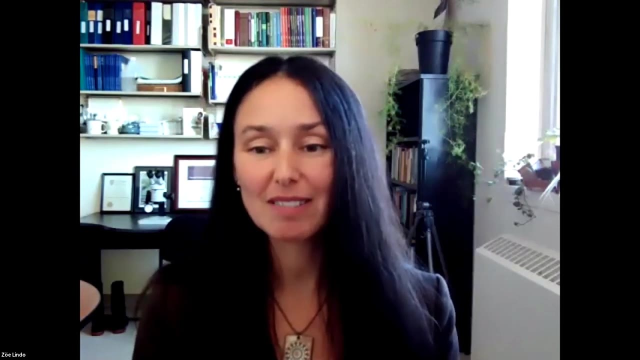 soil organisms. So how do we fill in some of these gaps across very large areas where we have very few researchers other than throwing money at it? That's actually a really good question. We're working on it, Yeah, But hopefully you know, in a report like this particularly, 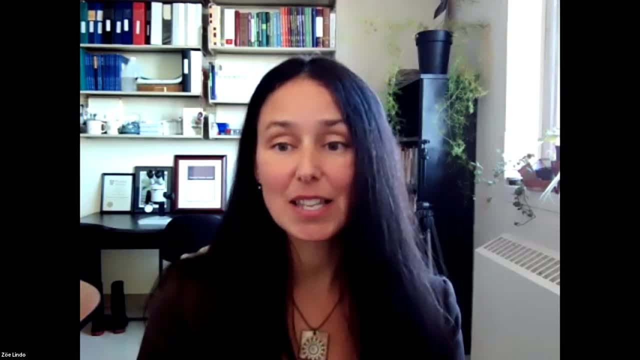 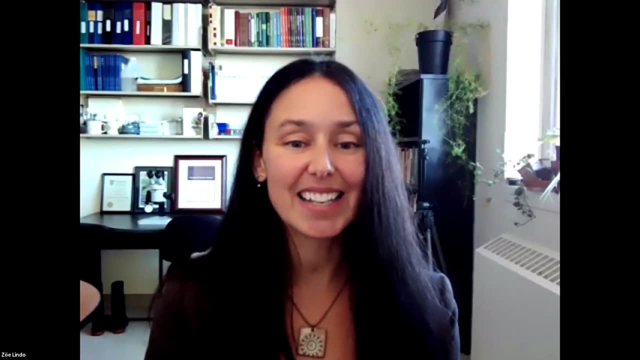 most of you, I think, haven't seen the report, But when you do, I think you're really going to love it, because it's just, it's so beautiful And it highlights these organisms that, like I said in my presentation, most people never get a chance to see. And I think when people start seeing 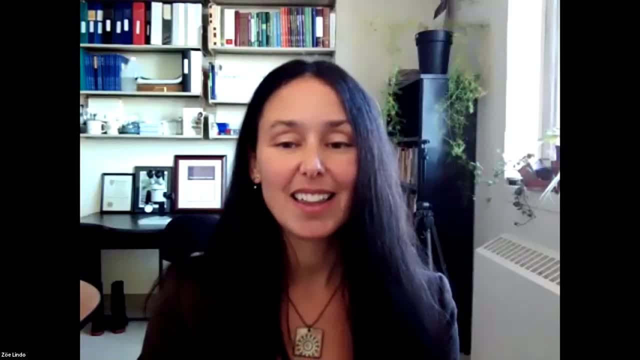 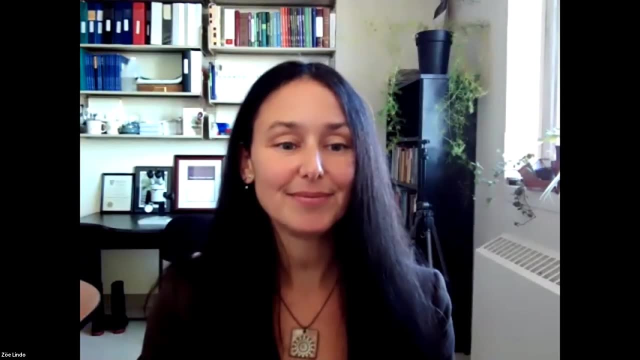 these organisms and how beautiful they are and how interesting they are, then hopefully we'll get more interest, as well as more funding, and be able to fill in some of those gaps. Okay, thanks, Another couple of questions that I mean. that's about sort of spatial gaps in soil. 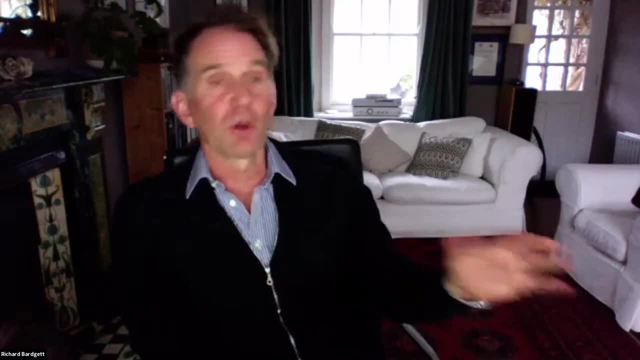 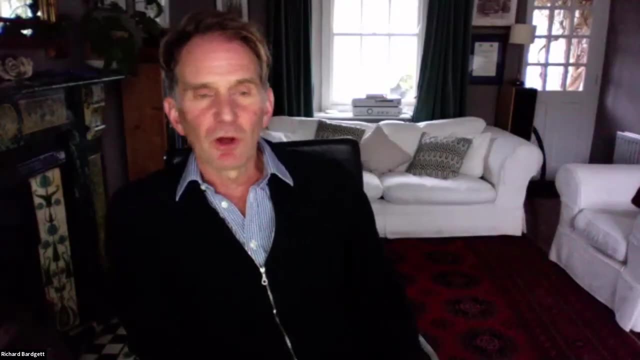 biodiversity knowledge. But another issue which has been touched on is taxonomic gaps, in that we have information for some organisms, perhaps the more obvious ones, like earthworms, for example, but other groups of organisms we know very little about or perhaps are less. 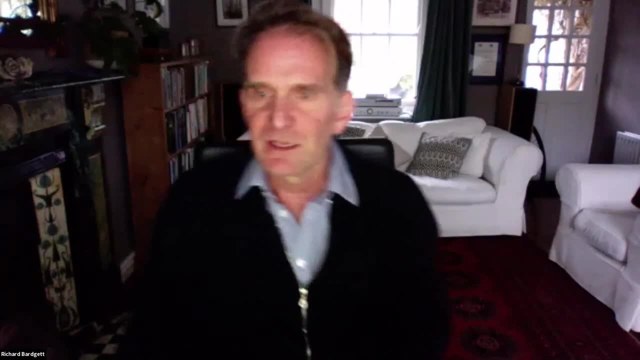 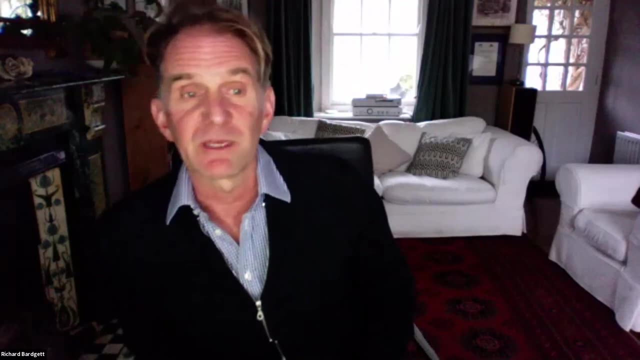 attractive to study And one of the questions we have here. we have two questions actually. One is from Matt Turnbull, who says only a small proportion of soil organisms have been found in the soil. So the two questions are the same question: whether or not soil organisms have been identified. 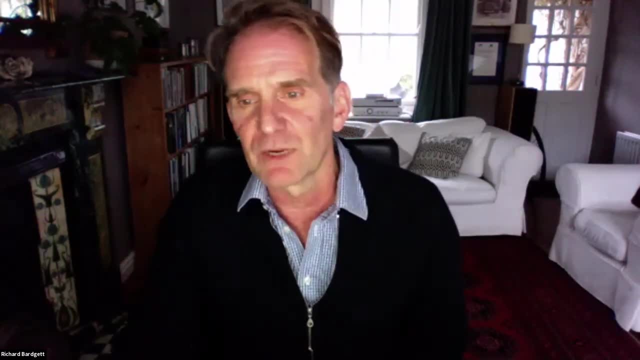 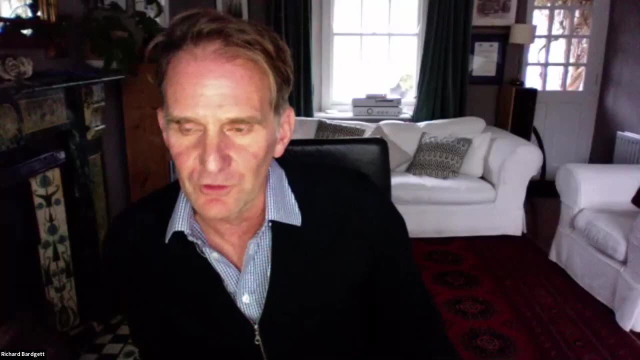 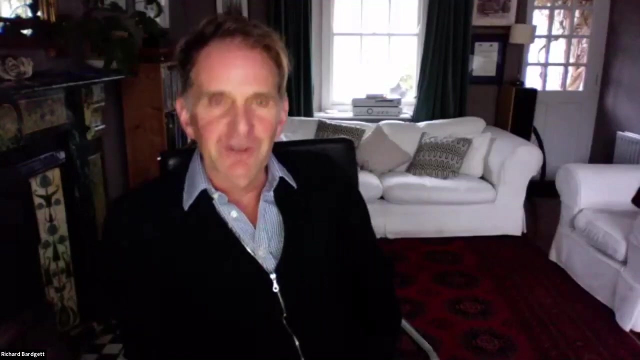 what policies or research funding priorities can be implemented to address that gap? But also a related question is by Isabell Feekes. I hope I pronounced that correctly. Do you think that red list for soil organisms is a good idea? I'm going to ask Elizabeth to address that first question. 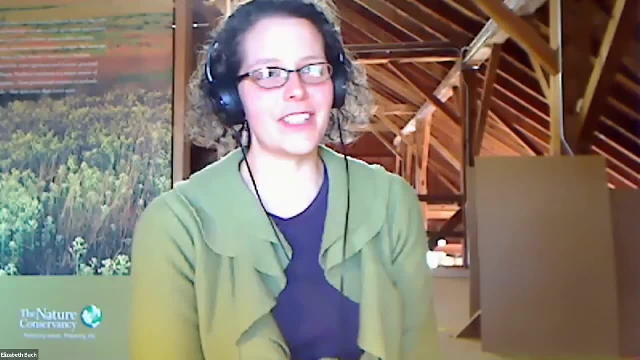 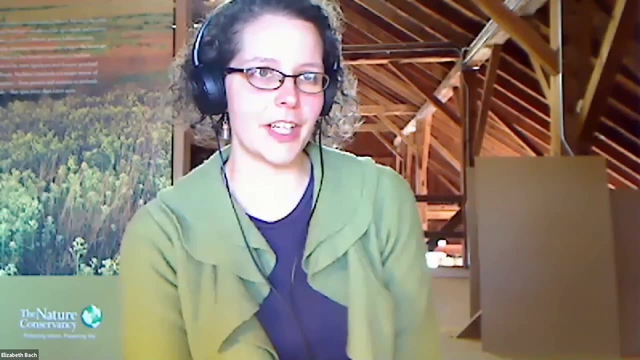 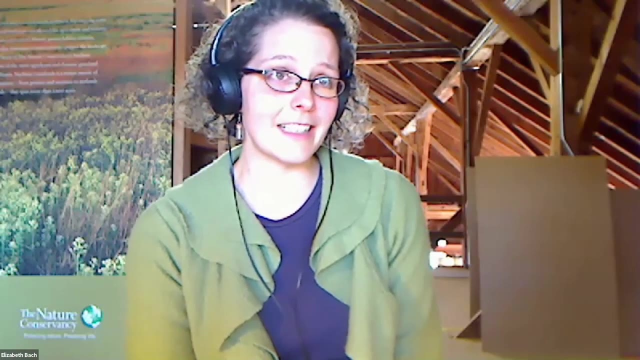 really about taxonomic gaps, and then I'll come to the other one afterwards. that's a great observation. Sequencing technology has really expanded our knowledge of bacteria and fungi to a great extent, And these were areas that we really lagged prior to sequencing technology. 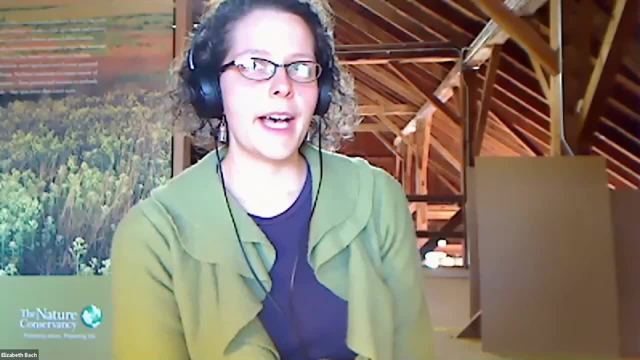 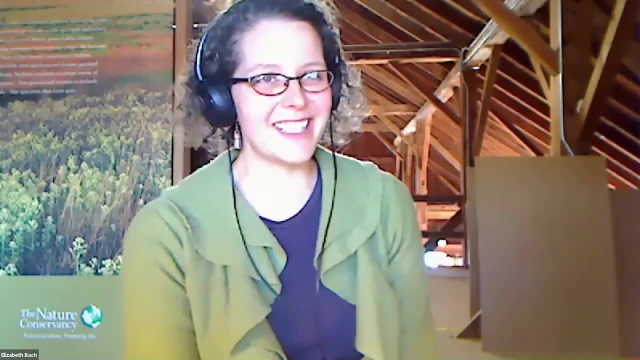 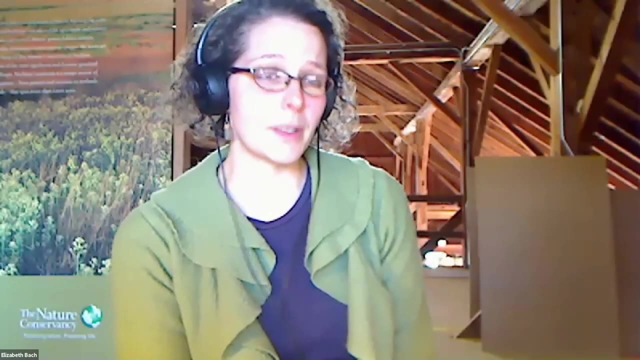 so it's been tremendous to see that growth. Some of these more microscopic invertebrates are really challenging. There's less funding for that kind of research. There's less taxonomic expertise. I get the impression that taxonomic expertise is aging as well. We need more young. 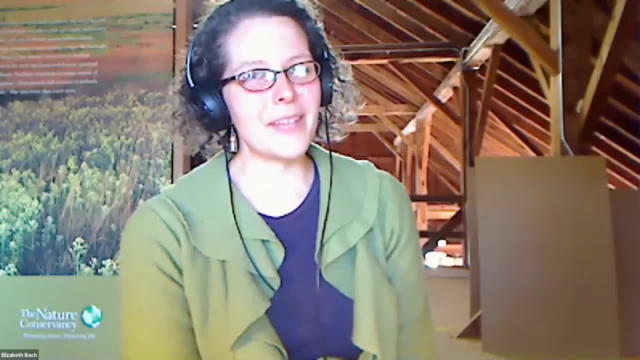 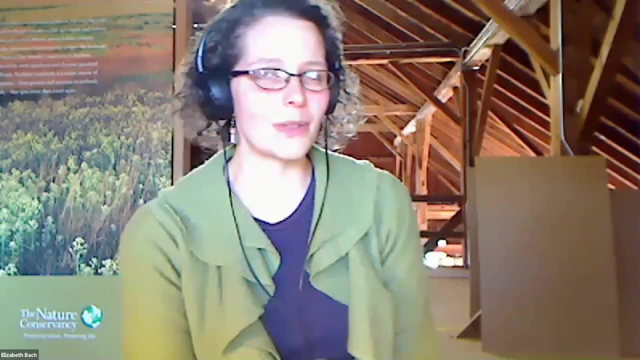 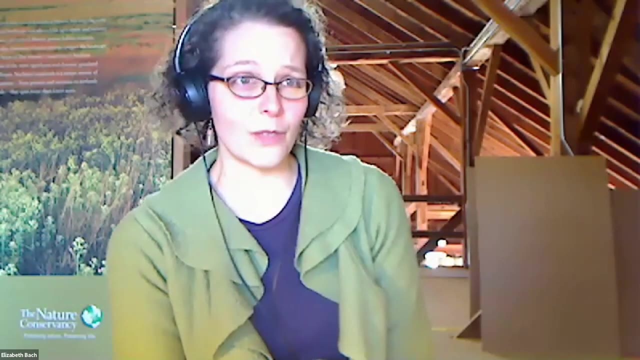 researchers really engaged with those organisms And I think building that interest in the way that we teach students at all levels is really critical to spark that interest so that people have that passion and push those fields forwards. I think that's really where we see lagging right now is. 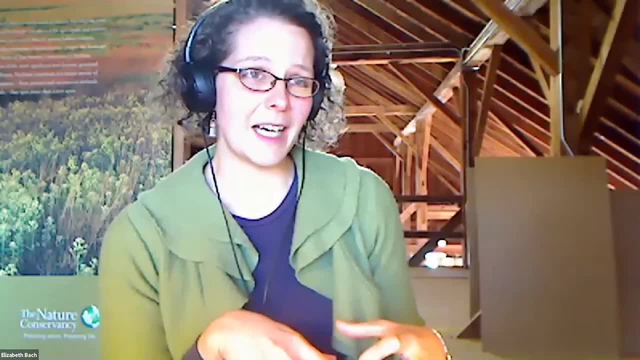 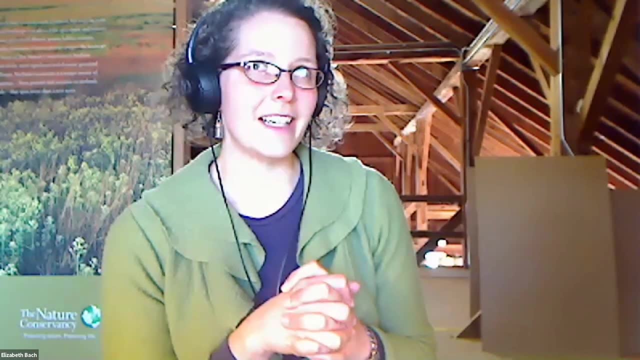 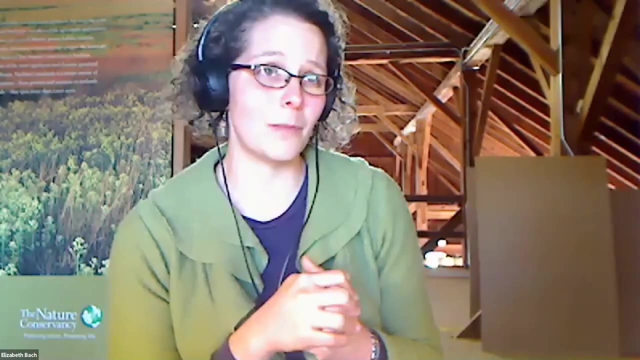 that organisms that are too small to really see without some microscope enhancement but don't have the sequencing technology. the primers don't fit well for those organisms yet And in general those organisms. there's a tremendous amount of biodiversity we don't know about. 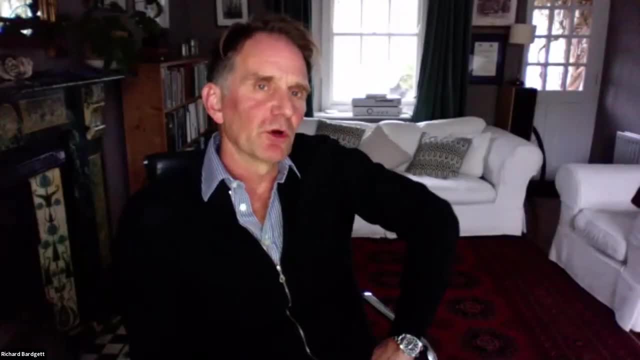 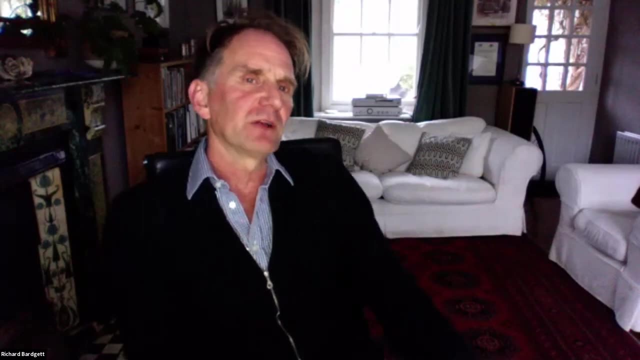 Thank you. I'd like to ask the same question, George. actually, I mean, you predominantly work on earthworms, which I said was one of the more obvious organisms, but obviously very important. But I wondered how you felt about gathering. 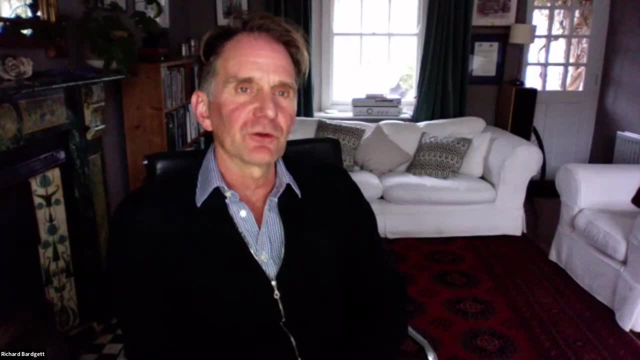 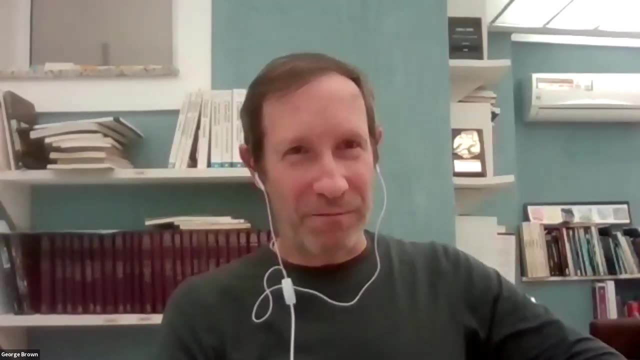 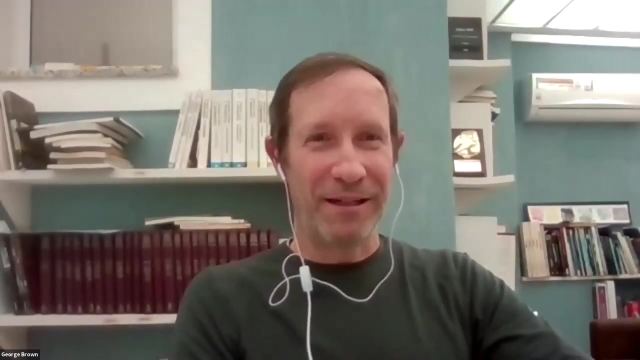 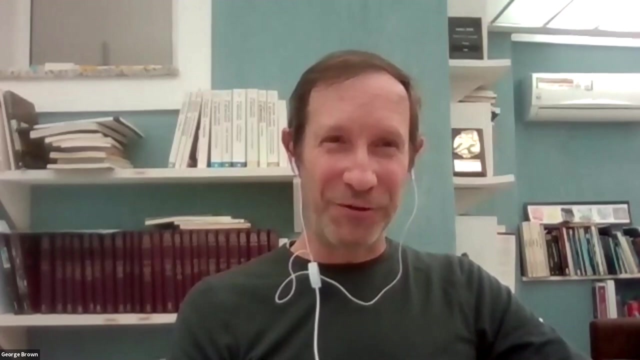 interest in other taxonomic groups that are clearly important in the soil. Yes, we've been quite lucky here in Brazil because we have some pretty good taxonomic expertise for some organisms that are quite biodiverse, like ants, beetles, but not so much for other organisms like mites and nematodes. But there is a great program here. 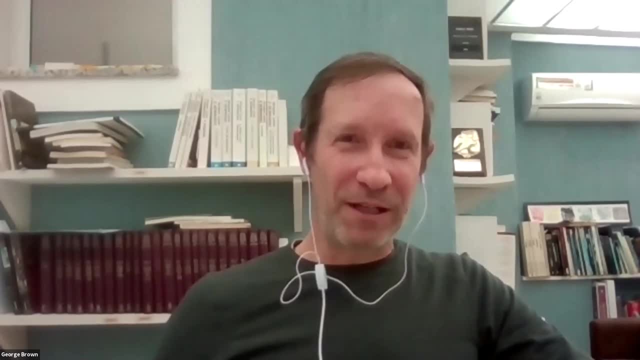 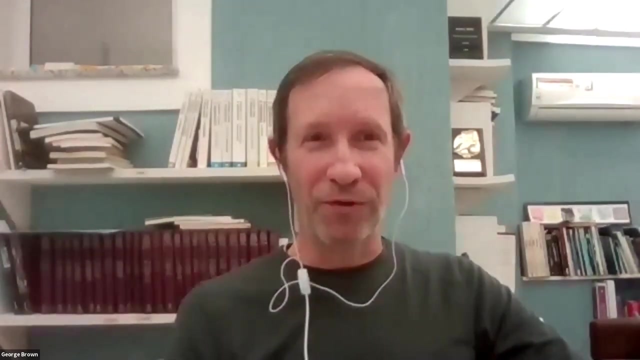 in Brazil, which is run kind of like the equivalent of the NSF in the USA, which is the CNPq program of taxonomic capacity building, which has been going on for the last 15 years almost, And this has been crucial to maintaining these students. 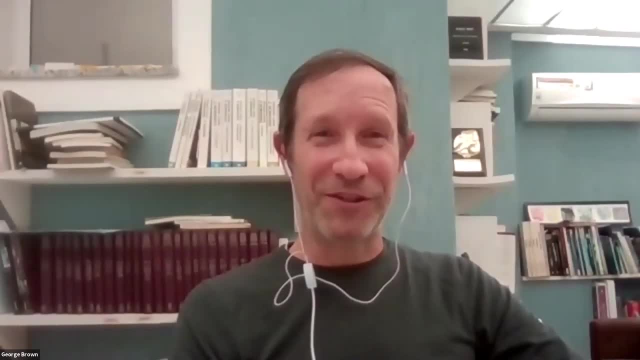 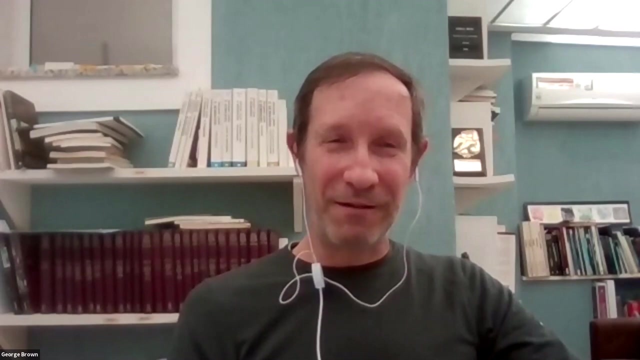 do get interested in taxonomy, to staying and actually eventually finding jobs that can maintain their interest and pay their salaries while they continue to do taxonomy. So this is the kind of thing that is essential that governments be serious about doing if they want to tackle this taxonomic impediment. 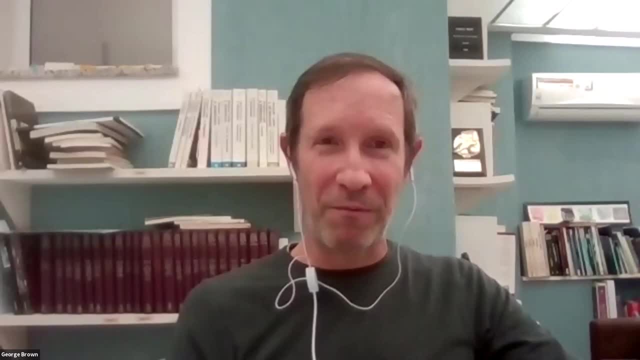 And Brazil is host to like 10% of the biodiversity, probably for the world. Like I said, there's some negligence groups there that really need to be worked on, But this kind of policy at the national level is crucial for that. It doesn't just depend on us getting the students interested. 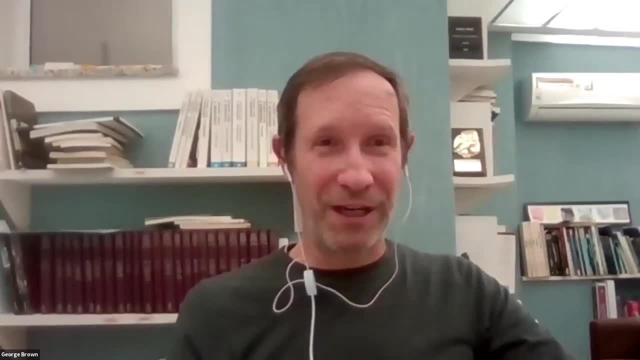 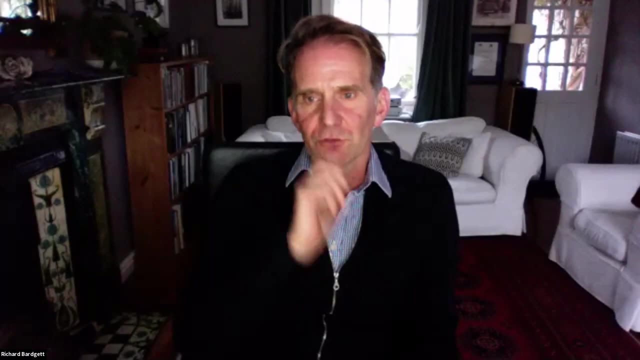 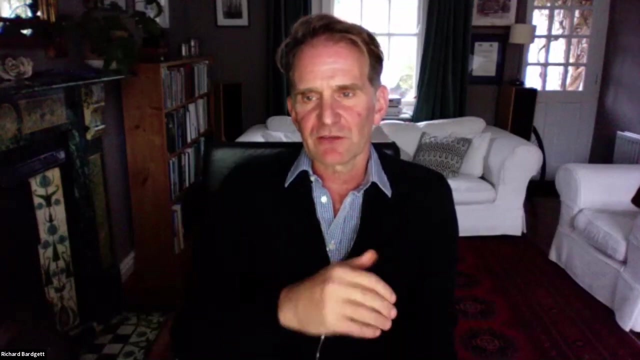 They later then have to be able to get a job to keep active in the field. So, yeah, I've got another question actually, But for you, George, because it's about how you can actually get farmers involved. This is a question from Patrick Lovell, and he's asked about how you can get farmers actually. 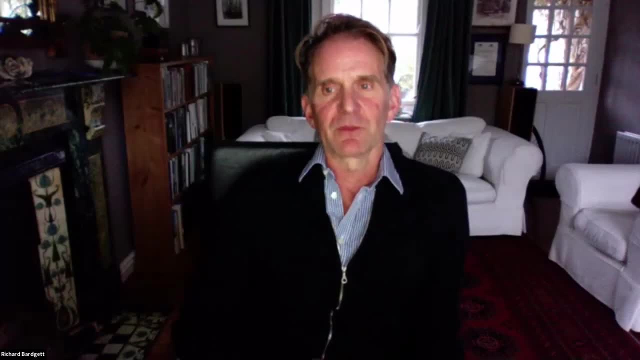 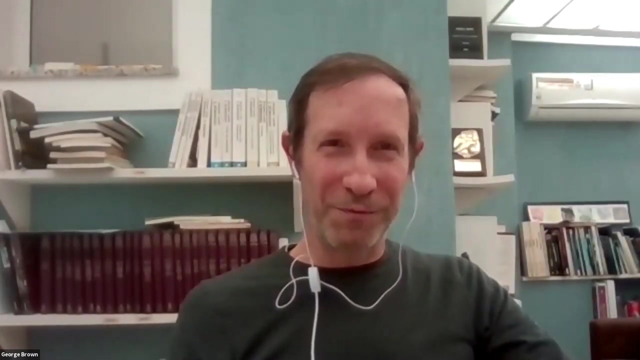 involved in evaluating soil biodiversity and make them the actual actors in building the public and policy appreciation to support sustainable agriculture, for example. Sure, We've had a few good experiences with this in Brazil, of course, mainly with earthworms And because they're just so easy to see. 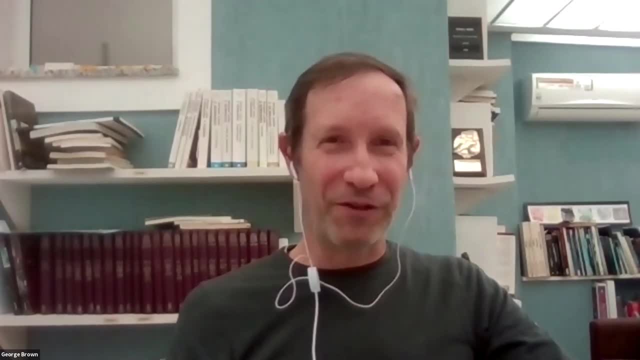 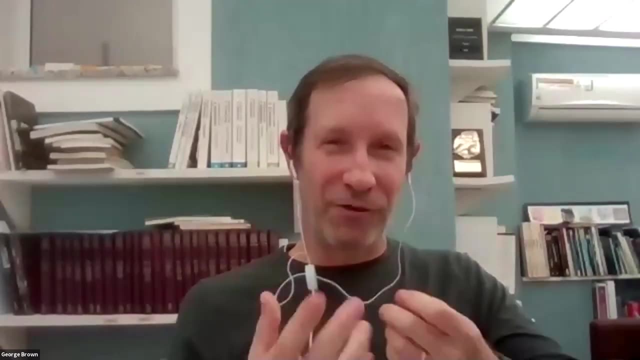 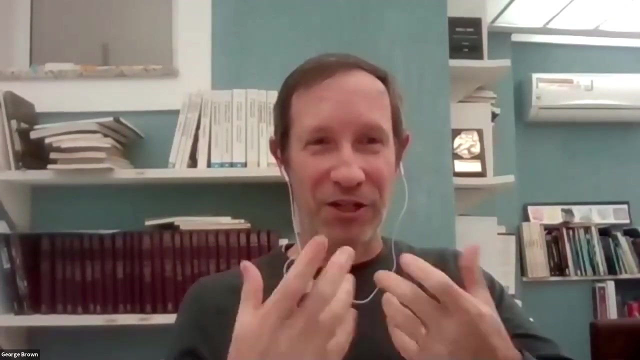 And basically you can show the differences between the worms that go a lot and the worms that don't, and the worms that are colorful and the worms that aren't. And they're great instruments of environmental education because you don't just see them, but you see what they do in the soil, with the holes and the casts and the poop. 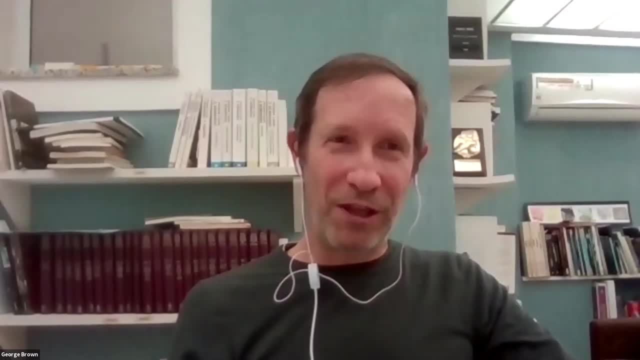 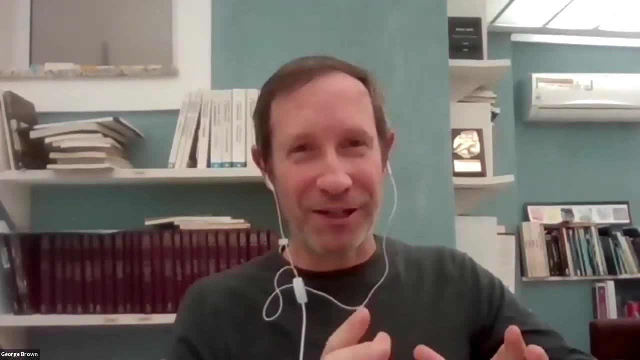 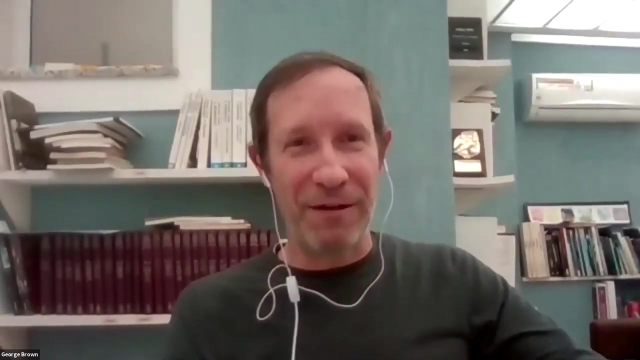 And you can do all sorts of things with those organisms that show the importance of why we should have more Of them and not, you know, consequently, other organisms too. You know we don't want to just focus on them, But if you basically, if you feed the worms, you're going to basically be feeding a whole 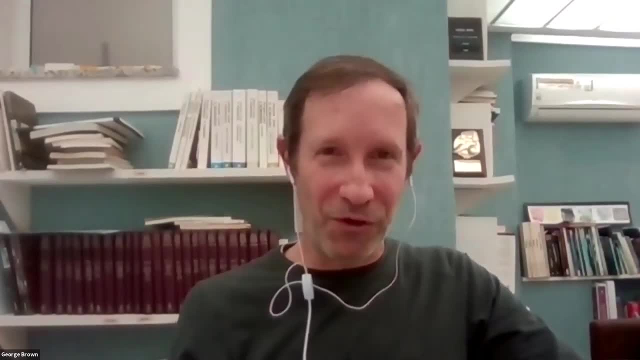 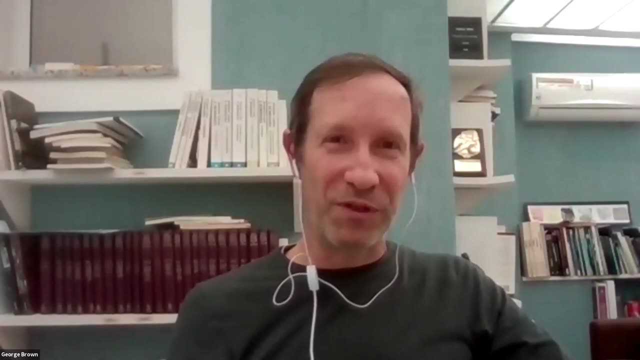 suite of other organisms, also because you're you're taking care of your soil And this has been really useful for us working with farmers, mainly in the no tillage association here in Brazil, which we've had projects over the last few years, And, yes, sometimes they accompany us to the field and they and they- you know they don't- 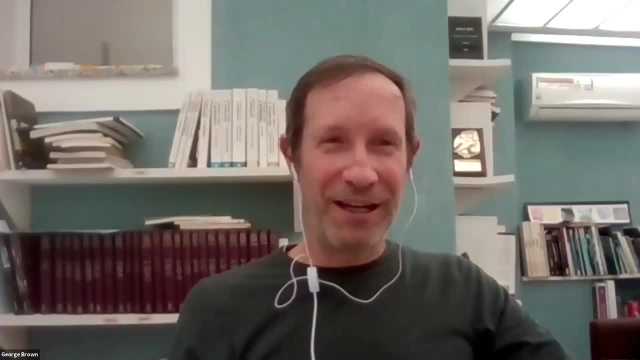 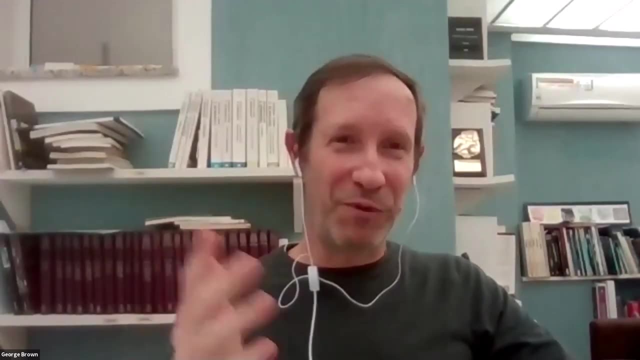 just let us work On their field. they sit around and ask questions- And I know those are great moments for us to to share what we know. And then sometimes they get really excited And pretty soon others, their neighbors or others- are also becoming involved or asking. 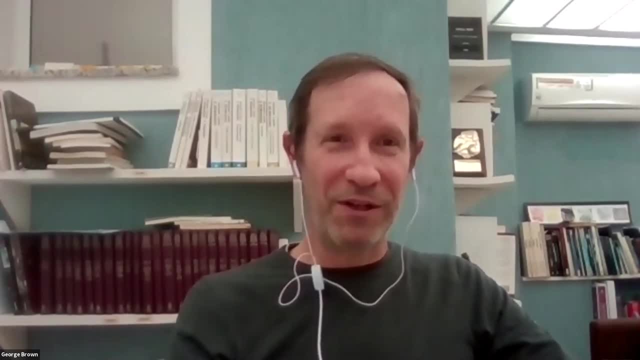 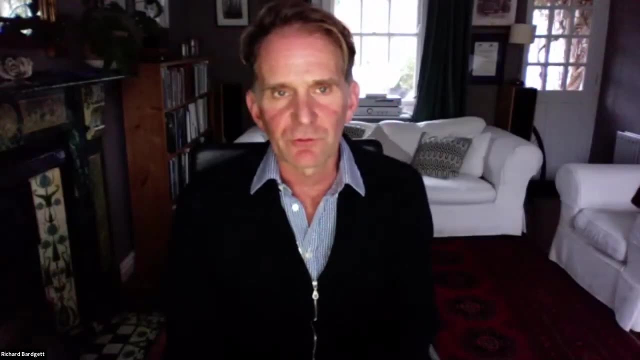 questions and wanting to know more also. So this has been our experience at least to share. OK, thank you. I mean again, when we're talking about the taxonomy of organisms, we also come into the topic of conserving and protecting. 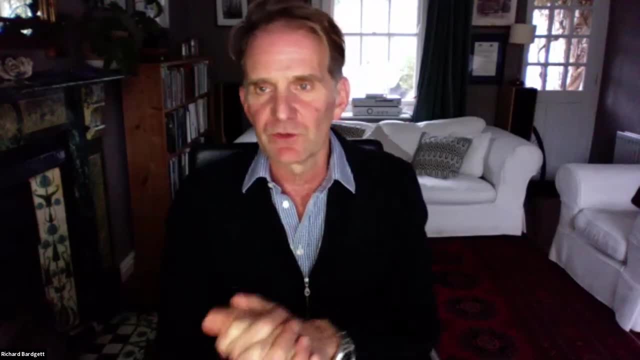 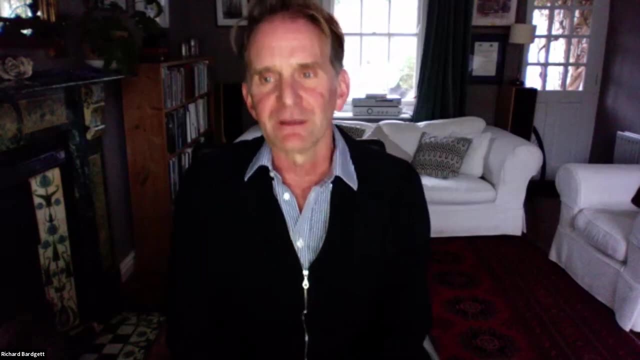 Those organisms, and I just want to go back to a question that we didn't really address before, which was by Isabel Feeks, I think again- I hope I pronounced that correctly And it was: do you think a red list for soil organisms is a good idea? 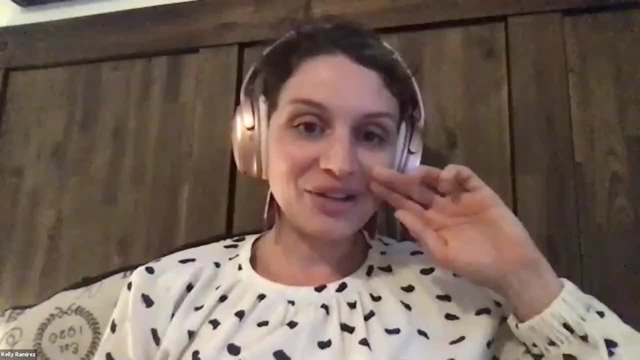 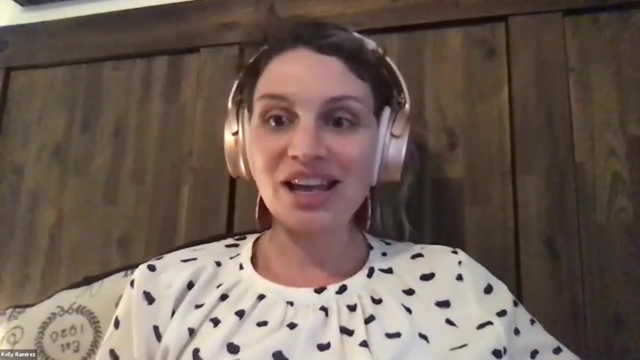 And I'm going to ask Kelly that question. I like that question because I don't really know the answer, And people ask this a lot. actually, when I give seminars to non soil groups too, I think it's. it's interesting, you know, like what George is talking about. there are some 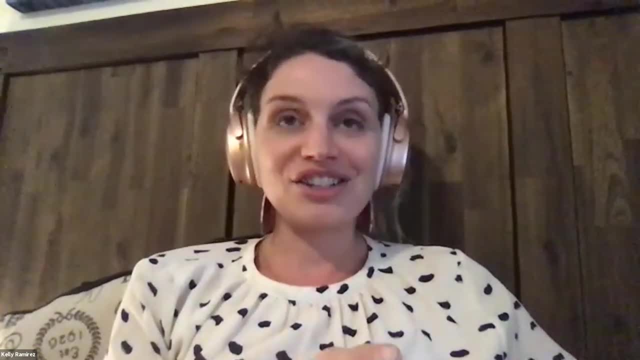 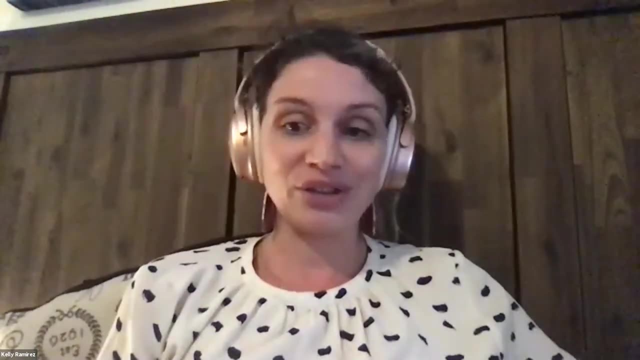 organisms that are visible and it's a little bit easier to characterize them and say, yeah, we don't have this here anymore and it could be on a red list. I think for the microorganisms that's a really difficult question, because what really those? 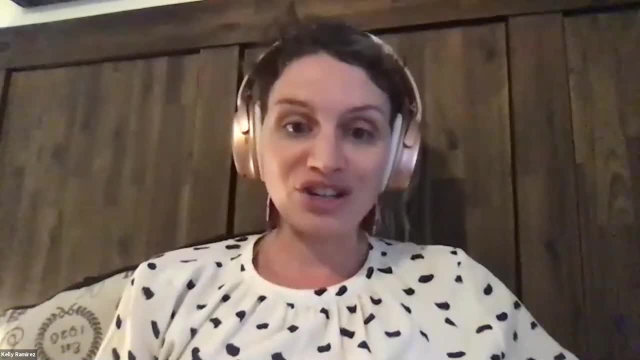 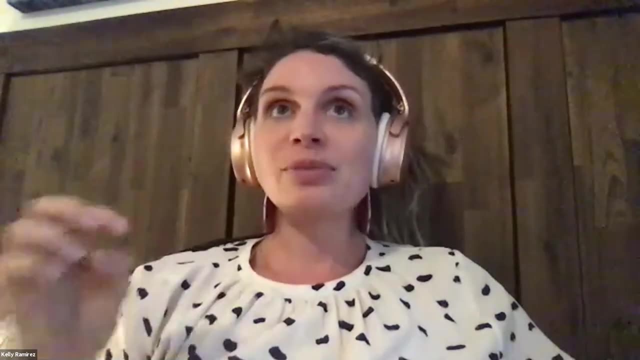 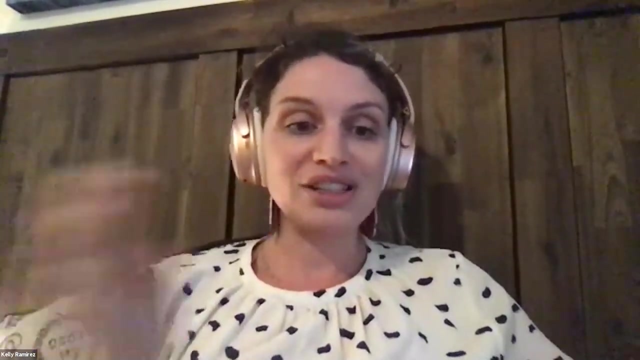 microbes have are traits for metabolic functions that are important for ecosystems, Right? So nitrogen cycling or very specific, Yes, Let's start with nitrogen cycling, Right? Not all organisms can do that. They can transfer those genes, So, if need be, right, there's like a different way to think about these organisms in the soil. 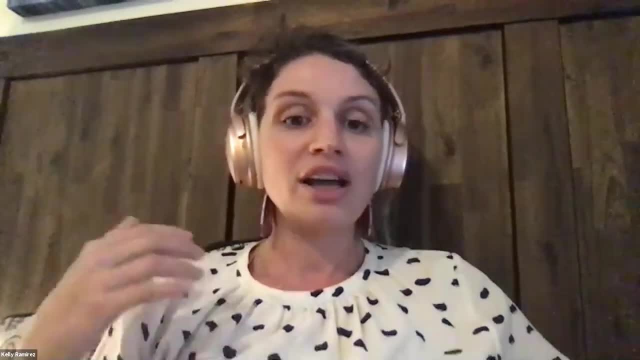 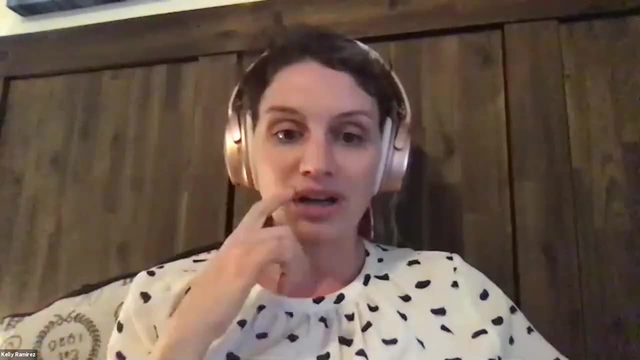 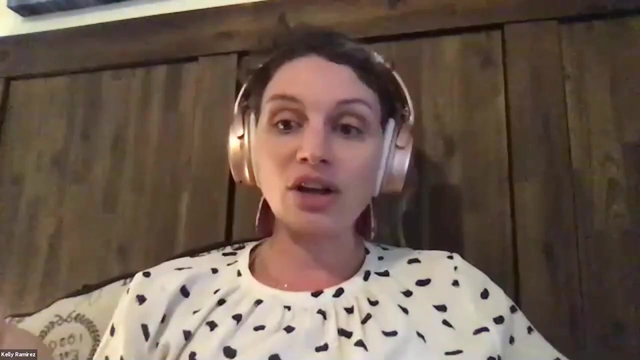 than our typical sense of species that we think about, for organisms that are larger, that you would collect for a museum, for example, And there's a question below that. So the GBIF right, the Global Biodiversity Information Facility, they collect all this. 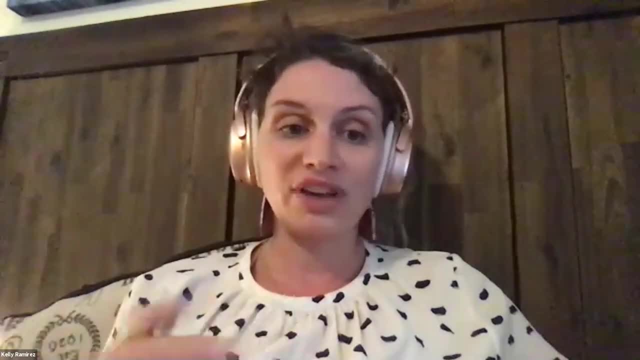 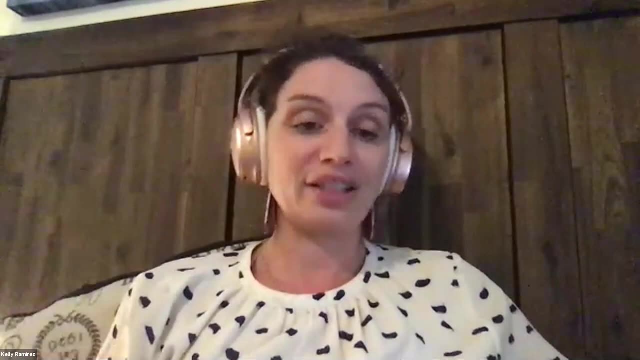 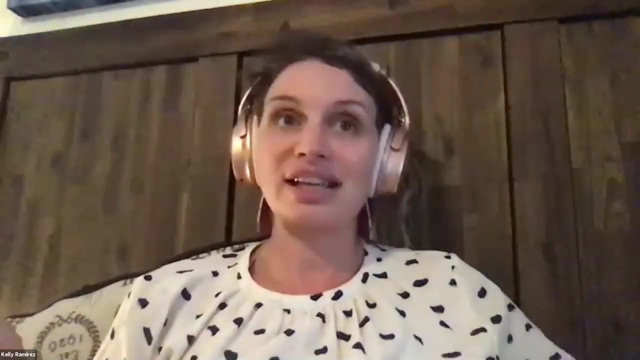 data on organisms, where they are, what, who, what was found where, Right, And so for soil data sets. we can link a data set to a lat long, But if it's a high throughput microbial data set, it's it's really kind of doesn't translate to somebody else's high throughput data set. 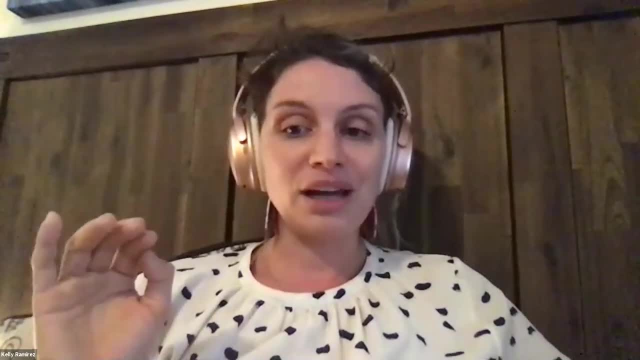 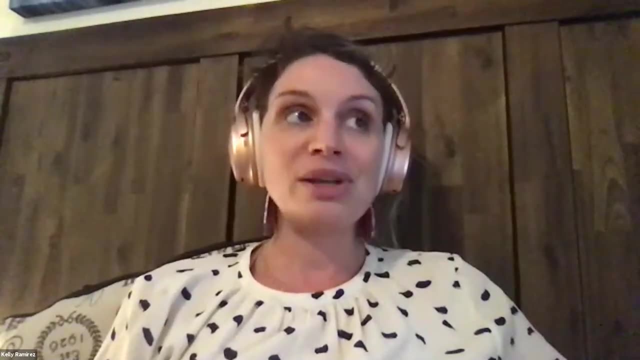 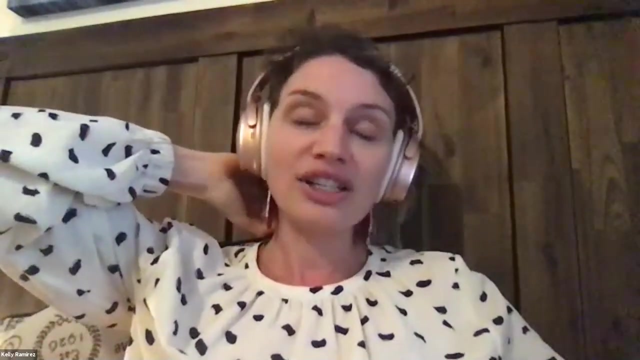 So we have to start thinking about questions of species, like for soil organisms, differently than we do for macro organisms. So it perhaps red list maybe would be. if we wanted it would be more like red listing a specific site, because it's hard to predict or know exactly which organisms have been lost, unless it's something like an earthworm that was really monitored. 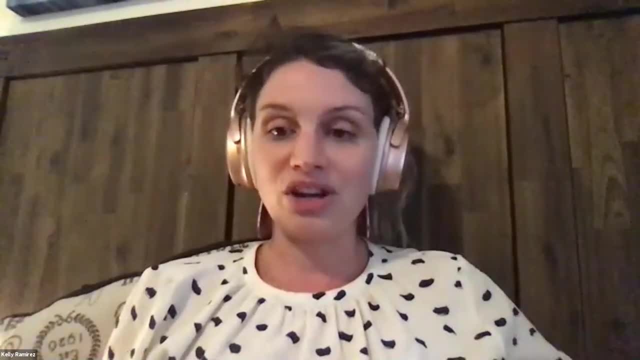 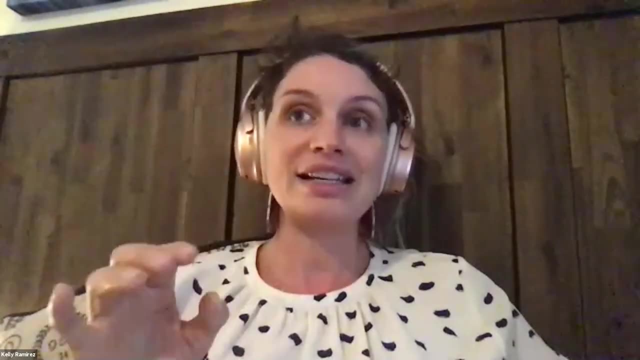 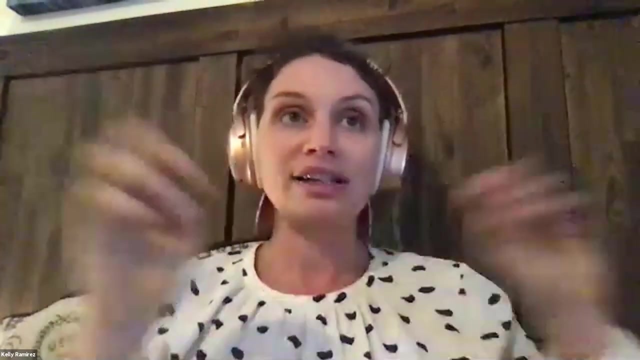 If it's a bacteria, like how, how would we even know? And so like instead we. I think what we need to do is start changing our perceptions of a species idea for especially for microorganisms in the soil, and then use that for, like this museum idea of where we're collecting points. 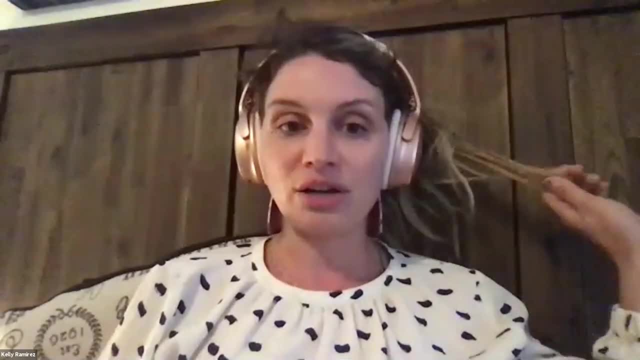 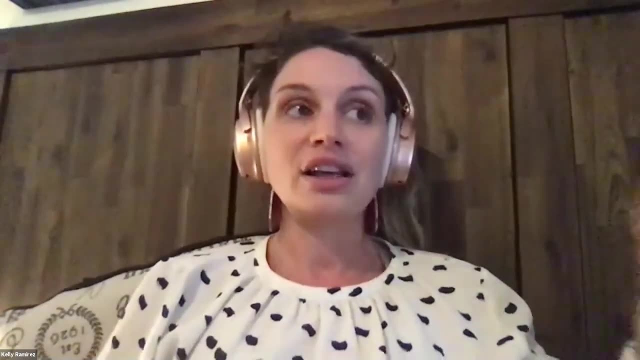 We thought that's what I worked on it. I did So. I know, Demetri, that was your question- And Marcus Doering Came down and talked with us And it is really challenging because a lot of our soil diversity data sets are huge matrices of lists of organisms and their abundance. 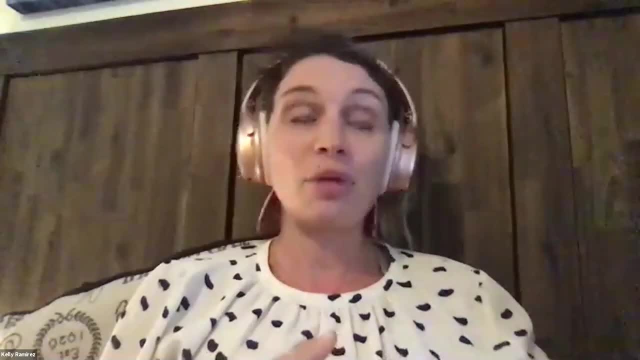 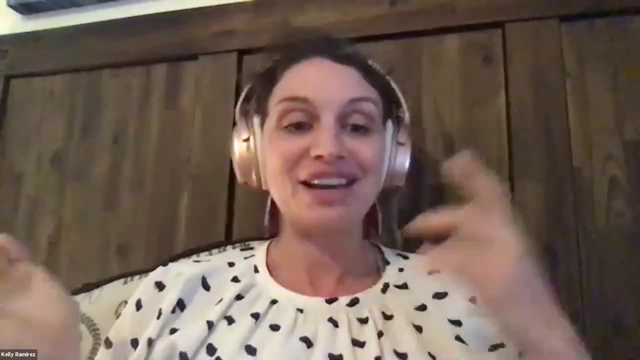 And how does that translate to a like a data set that's just like a panda was found here, right? It doesn't, because a panda is only one organism when, where my data sheet has like 5000 organisms or more, right I don't know if? Yeah, that's, it's a funny question. 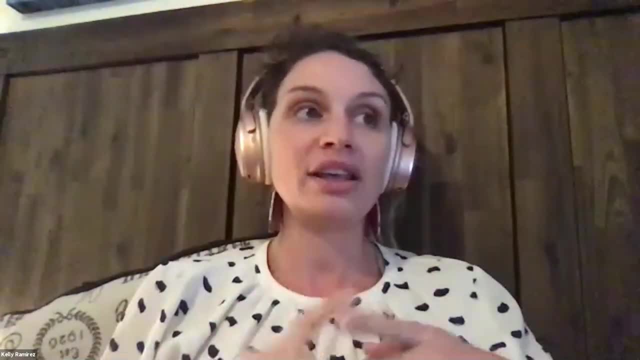 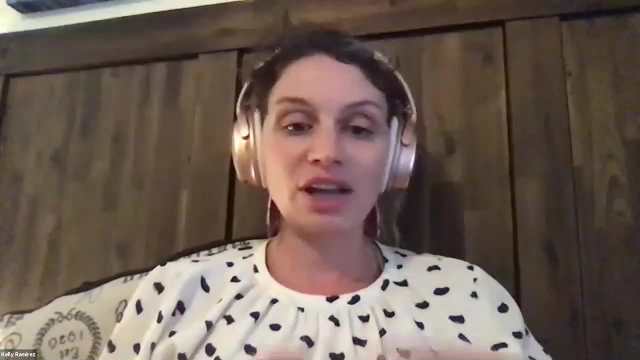 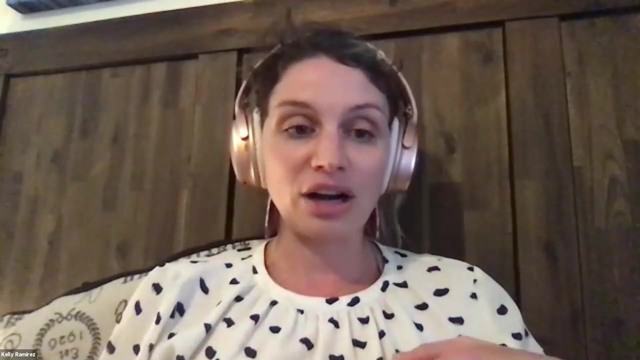 I think we're just at the beginning of things And I think communicating with People Who are thinking about modeling or organisms across the landscape from a more like jeep of kind of perspective- not just like projecting, like some of us do in our work anyways, but collaborating with people who think about these things and are have the computer power to do it. soil ecologists need to get better about sharing our information and how we're doing that. 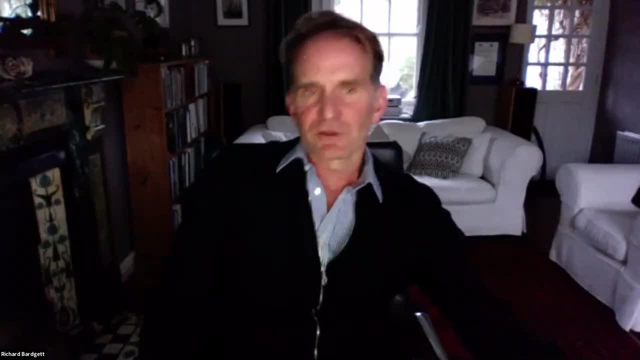 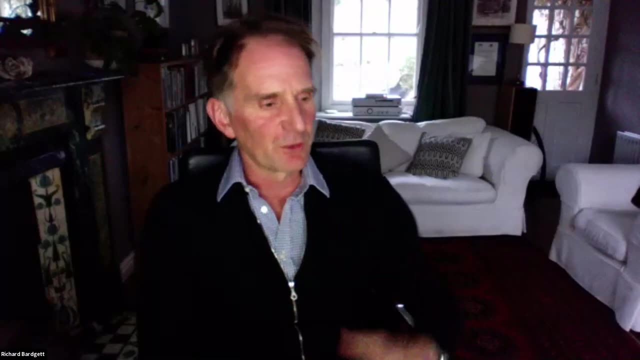 Okay, thanks, Kelly. I'm going to ask a similar question as Zoe actually, but more in, I guess, sort of related point is whether we just need to do it. Which was also picked up by Kelly is whether we should be focusing on protecting the habitats. 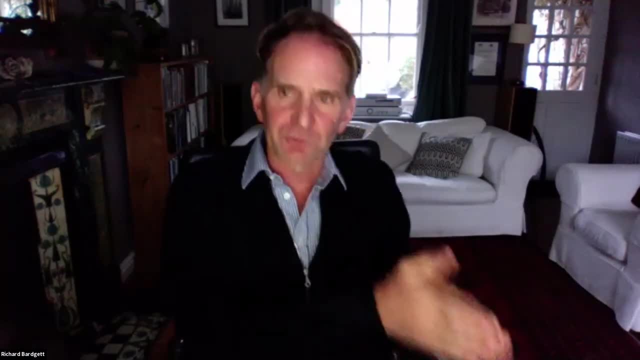 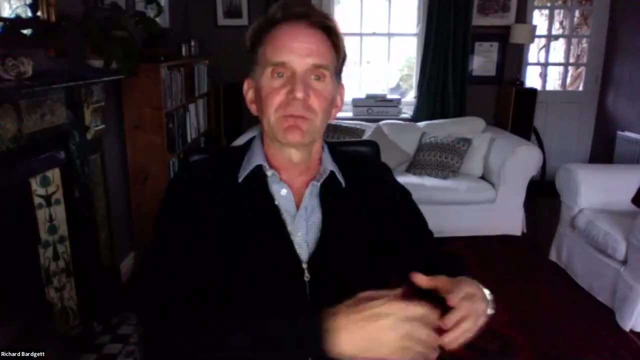 As a whole, or whether we should be looking at policy that is focused directly and actually protecting the biodiversity. So because? but soil features in much policy, but it's usually in policy related to something else, So it's not central. So I wondered how you feel we should be moving forward in that. 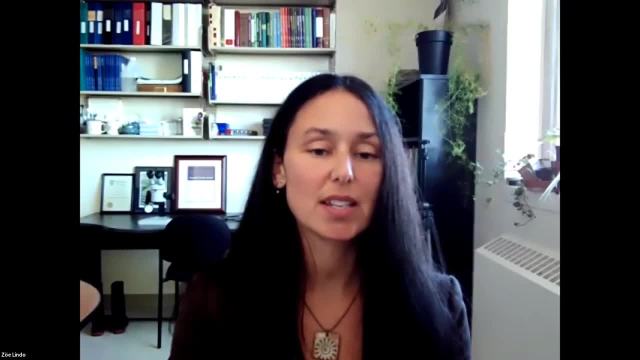 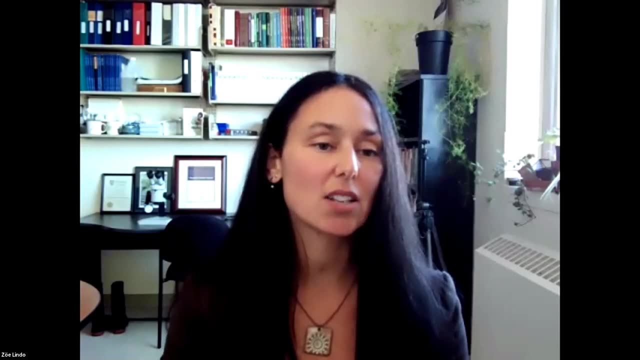 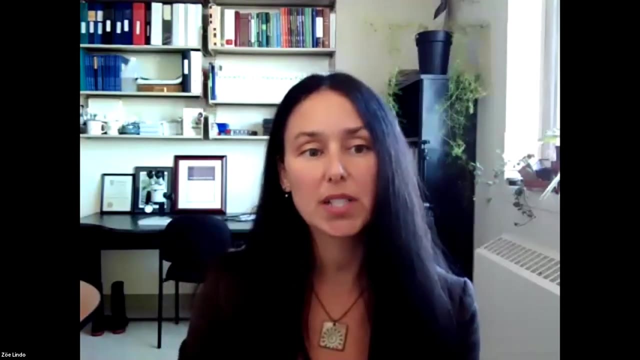 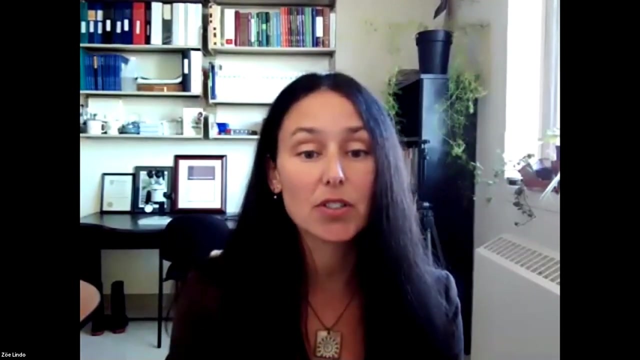 Yeah, I agree. Maybe just to step back and address the, the idea of a red list and More sort of ridder, reiterate what Kelly was saying, that the the red list concept just simply doesn't really work for soil biodiversity. A lot of the frameworks for protecting specific species don't translate well to soil organisms and part of that is because of their size: They're so small. I've actually tried to get a mite red listed and 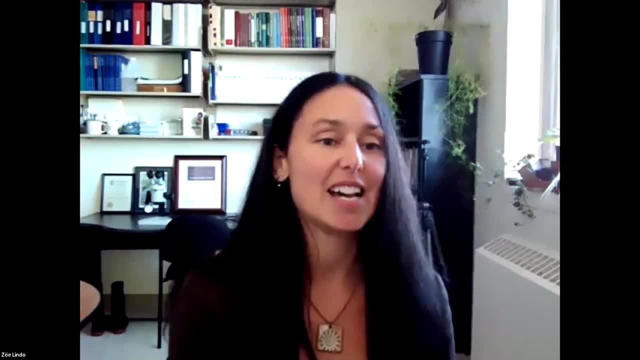 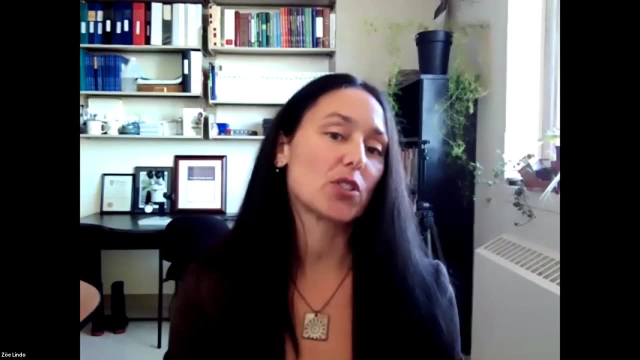 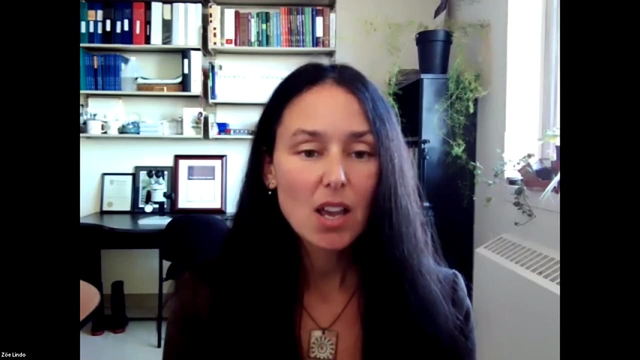 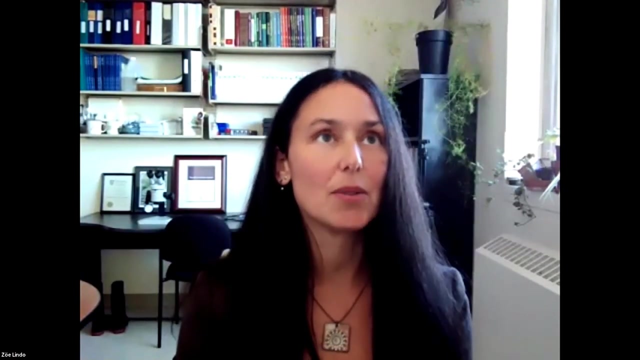 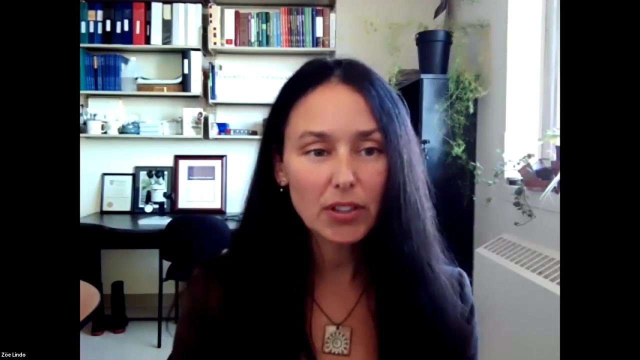 My ability, even as a taxonomic expert and field ecologist, to be able to To get enough data to satisfy those criteria is it was virtually impossible because because of the the scale that soil organisms interact with their environment. so, Yeah, sorry. So, thinking more more broadly about protection, protection of soil biodiversity- I think it. I think in many ways it has to be definitely re envisioned. but 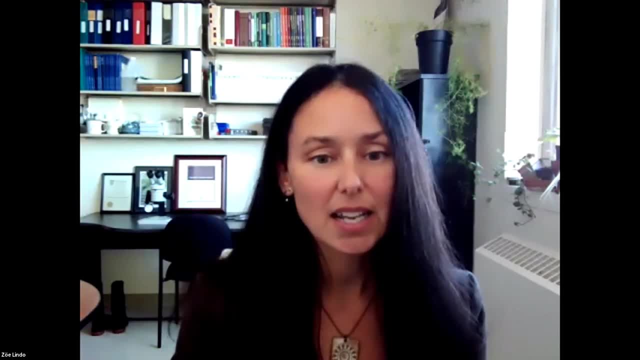 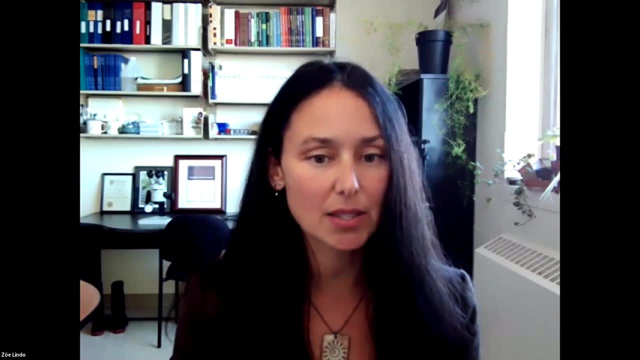 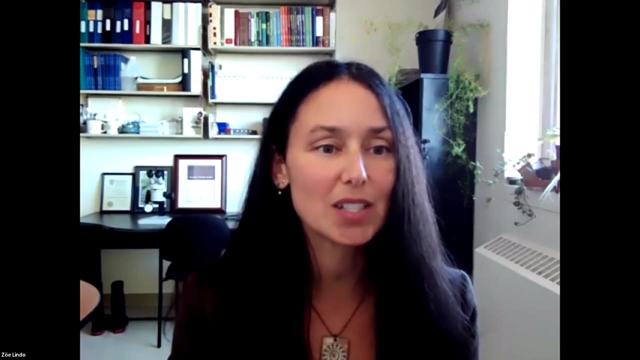 I'm not sure That it's necessarily a habitat specific. I think again, what Kelly was was sort of inferring is that it almost has to be a functional based assessment, Which is exceedingly difficult because we're still working through the taxonomy, these organisms, we still 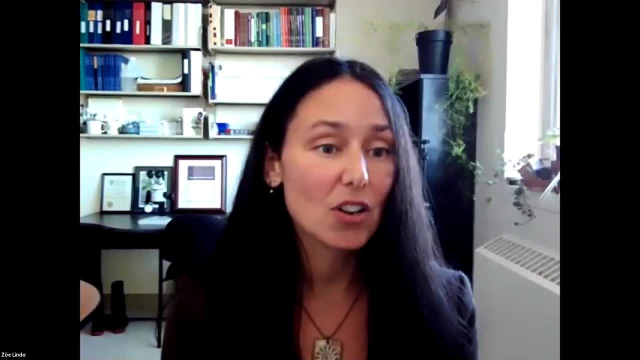 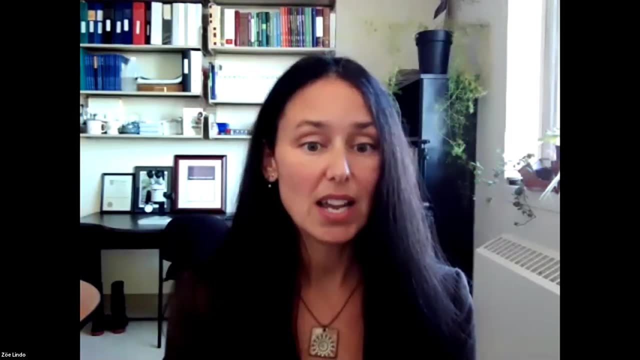 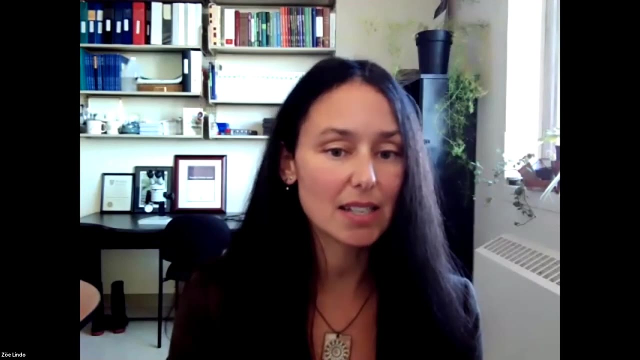 And again relating back to some of the questions, like Matt Turnbull had and noted that we know so very little about these organisms, who they are, what they do. that Getting it to that functional based assessment I think is is exceedingly difficult but but I think it has to come back down to a functional based assessment. 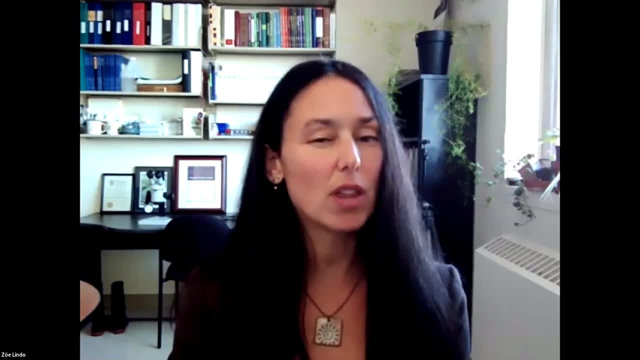 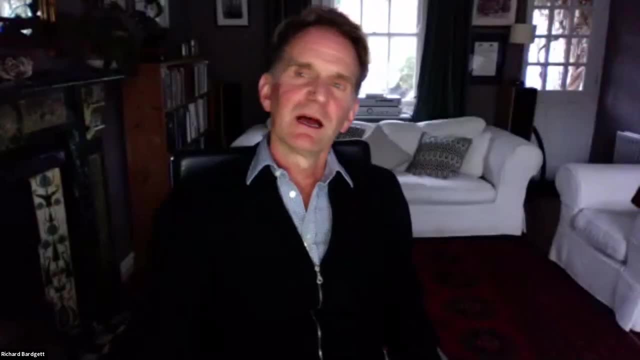 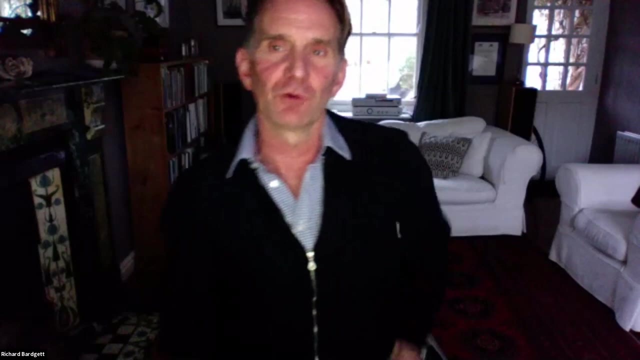 Because it's really the role that these organisms play, rather than who they are per se, that that's important for for sustaining soils. Thank you very much. And that that raises a an interesting question about the actual function and the relationships between the diversity and function of organisms, And one of the questions that we have is from Wenjia Wu. 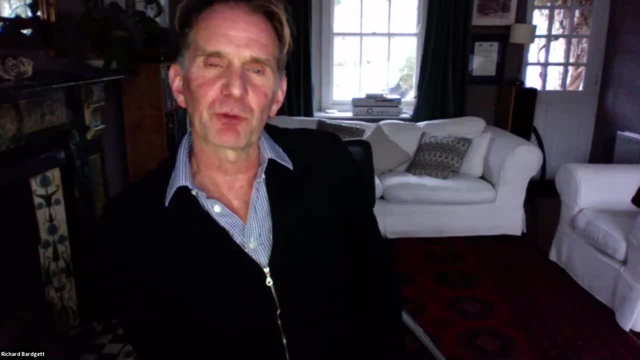 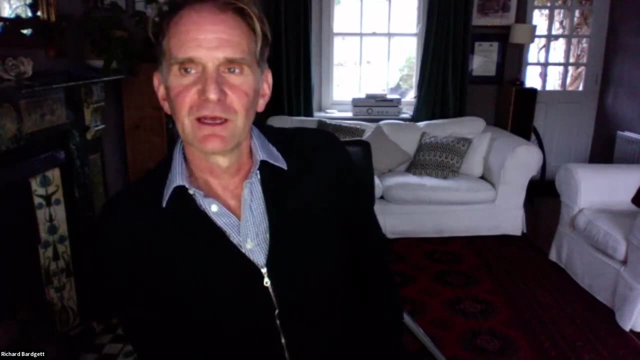 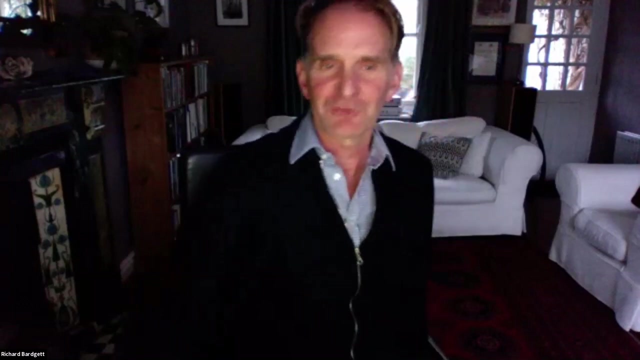 Again, I hope I've got it right. do you think there is a perfect combination of diversity and abundance of diversity of soil organisms that can make the sulfur web function and work efficiently? And again, I'm going to ask Zoe about that because I know that's your just ask you a question. but I'm going to ask you again because I know that's your area of research. 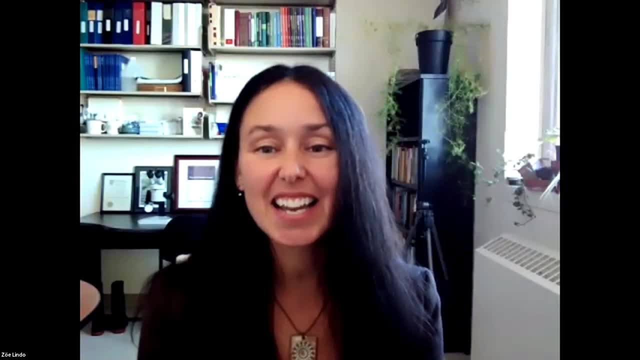 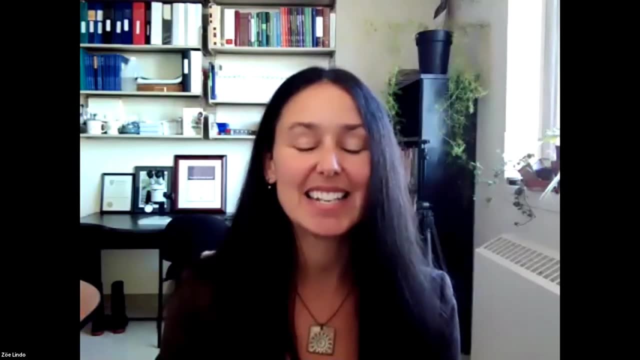 Zoe Scheltenberg- I love this question, Zoe Scheltenberg- And I would love to think that. Zoe Scheltenberg- Yes, there is this perfect combination of diversity and abundance, And that's where I think of the soil food web. 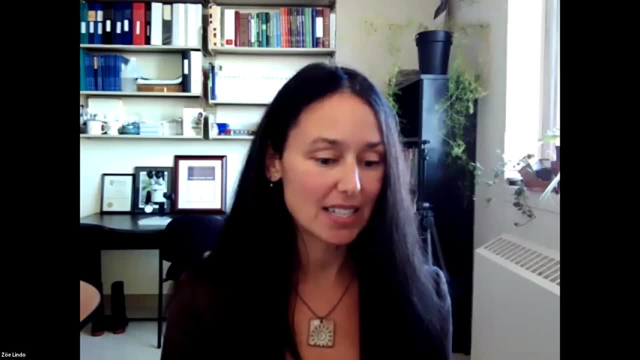 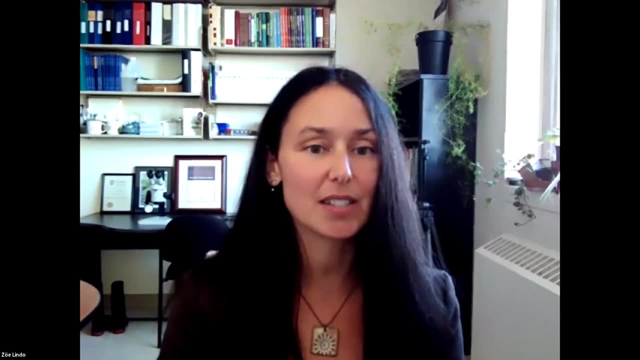 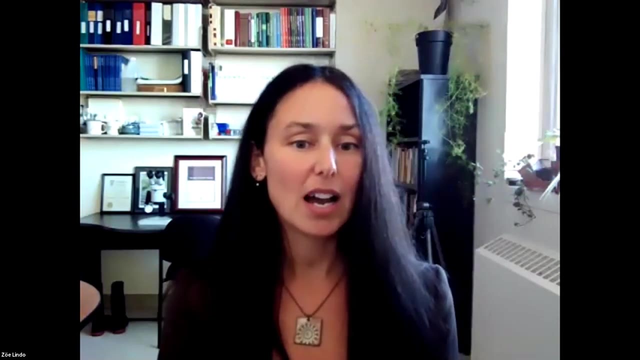 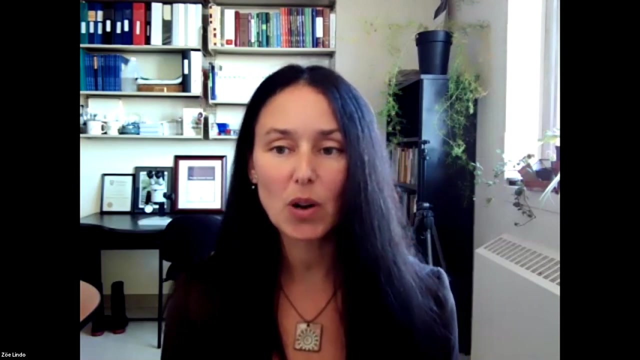 as this comprehensive system. In ecology, we refer to high diversity, highly interactive systems as complex adaptive systems, And that means that within this complexity, it allows for a flexibility when changes occur, for instance- And so the way that I think about soil- food webs. 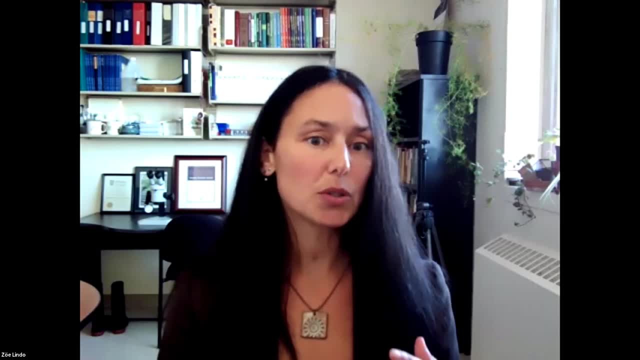 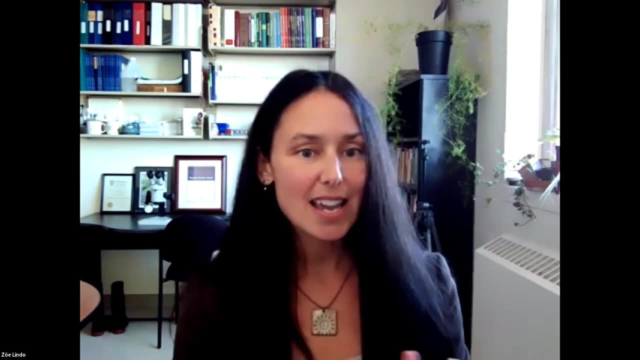 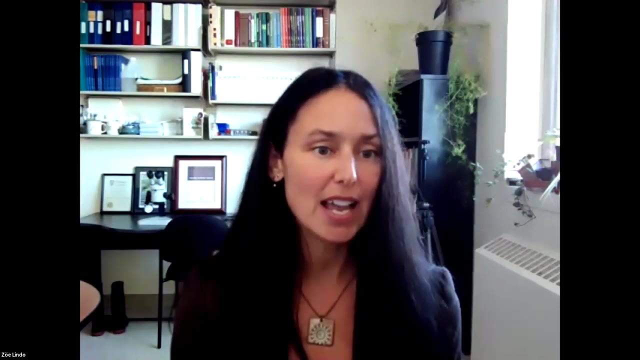 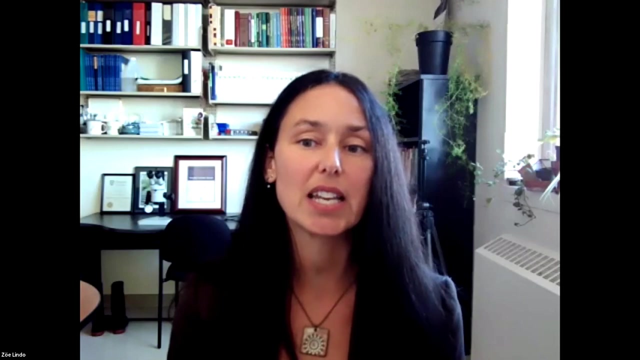 is even just breaking it down into multiple channels of how energy flow through this system. And it's because it is this dynamic system and it allows for the system to be flexible when changes occur and to maintain that overall structure and function. And so I do think that when we lose soil, biodiversity, 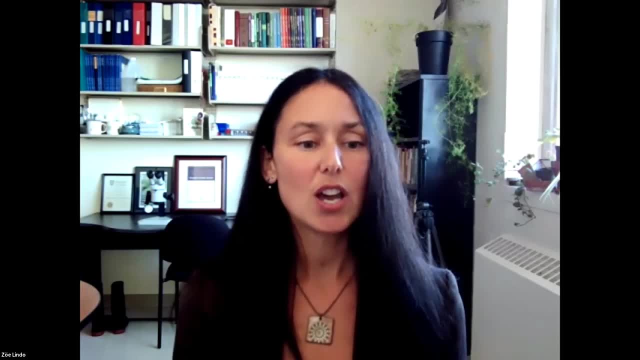 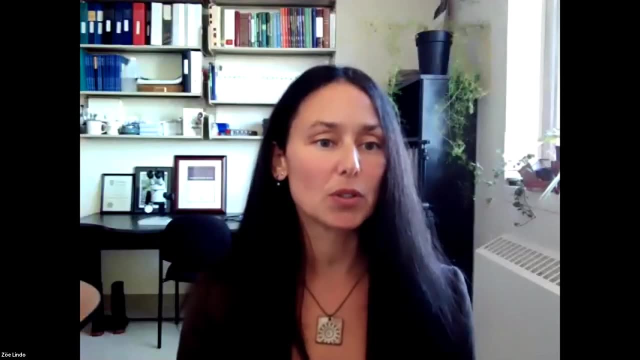 we start to throw that off, we start to break those connections, We start to tip a balance towards one energy channel versus another, And it's really about those multiple channels and the way energy can flow through the soil food web that allows it to be what it is. 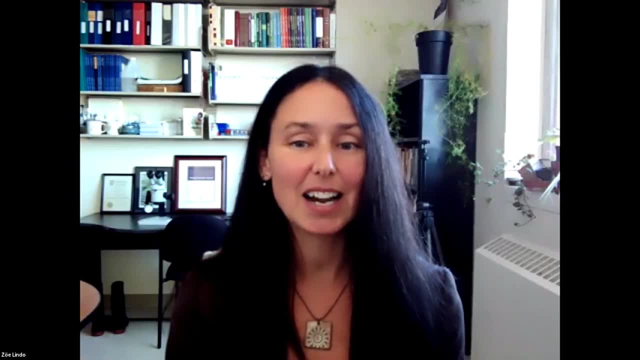 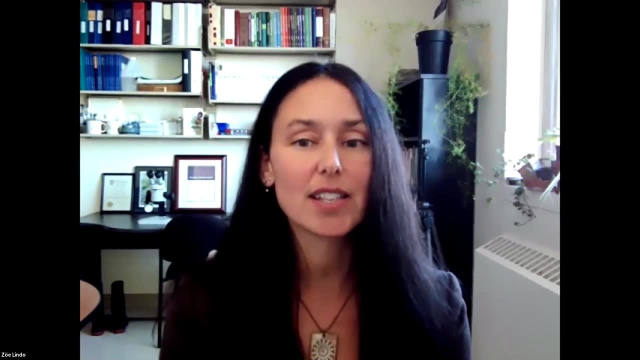 So I do actually think that there is a perfect combination. I don't think that we know what that is yet, but I think we're getting pretty close to understanding it. Okay, I'm gonna ask Elizabeth the same question. I mean, do you think there's a perfect combination? Yeah, this is a really interesting question And I think my perspective on this is: there may be, but it might be different depending on the type of ecosystem or situation you're in, And that perfect combination for a desert might look really different from that perfect combination. 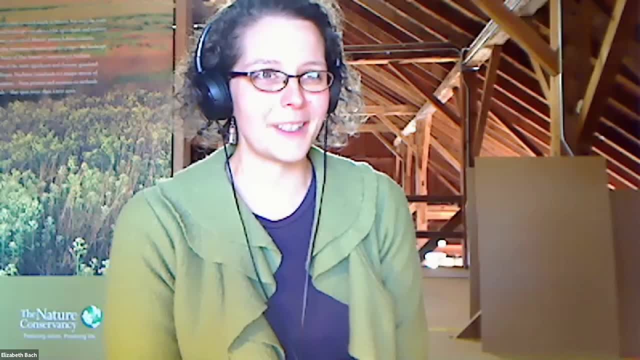 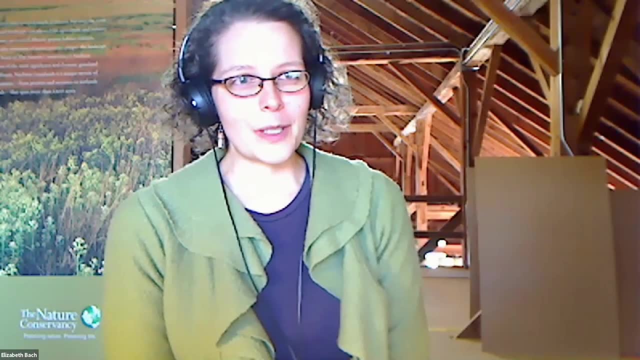 for a wetland or an agricultural soil or a mountain or a prairie or a forest, And so I think this is a great avenue for us to continue to explore and look into, and it's certainly the kind of answer that would move things forward. 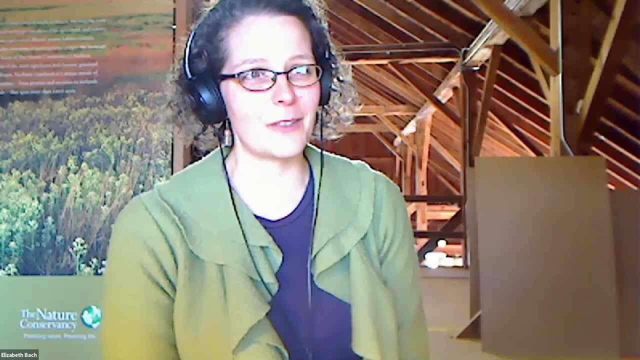 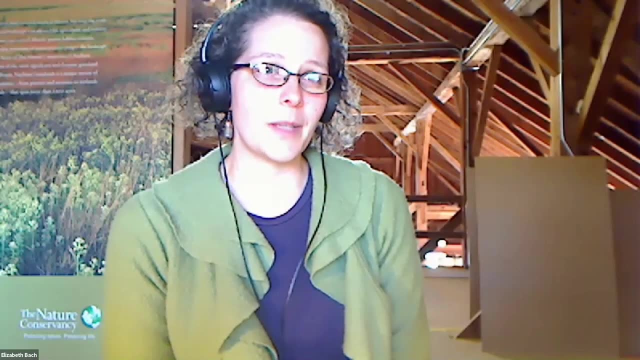 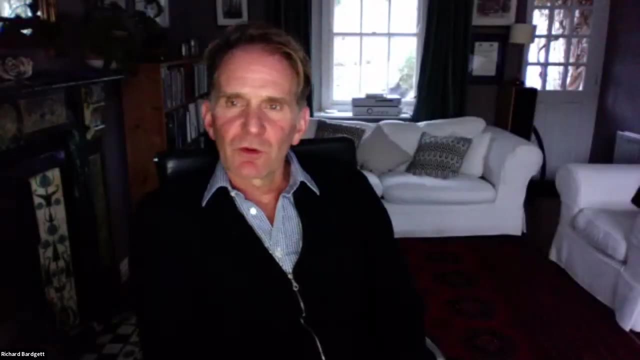 both for policy and land managers and farmers, to feel like there's a goal there to get to, but to keep that perspective that it's gonna look different in different parts of the world and in different ecosystems, and to keep that in mind. yeah, Okay, and what about one of the other questions about this? 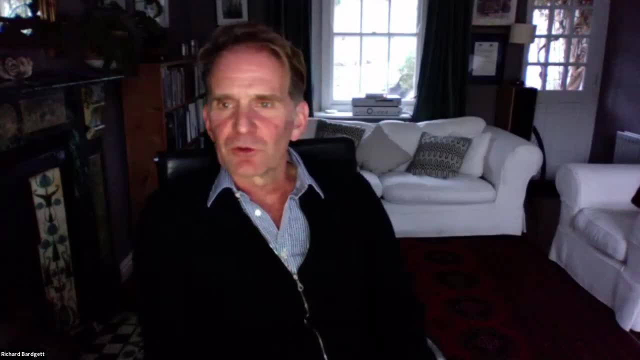 is about sort of artificial use of microbes, And I assume this person- it's Masaki Bekai, and I think he's talking about soil inoculation. I hope I'm representing his question correctly. But I mean, how do you see a role for those? 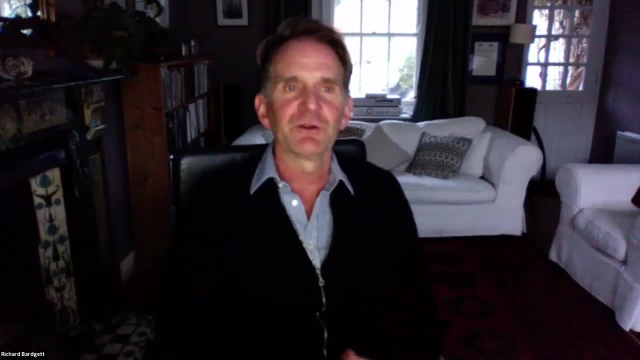 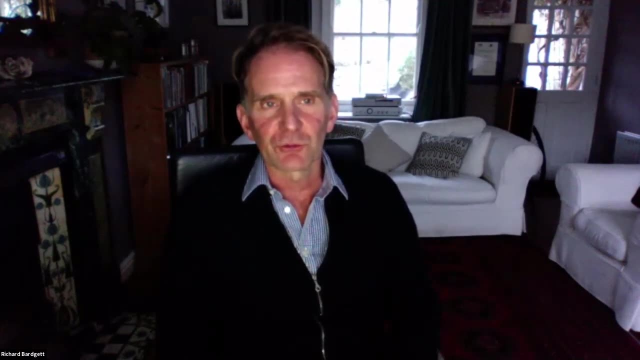 You've talked a lot about encouraging diversity, feeding the soil to improve the organisms, et cetera, and their activities, But what about introducing organisms? I'm gonna ask George this question, as you talked before about feeding soil to benefit the earthworms. 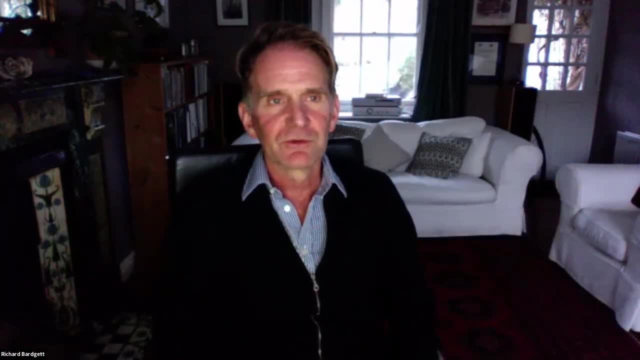 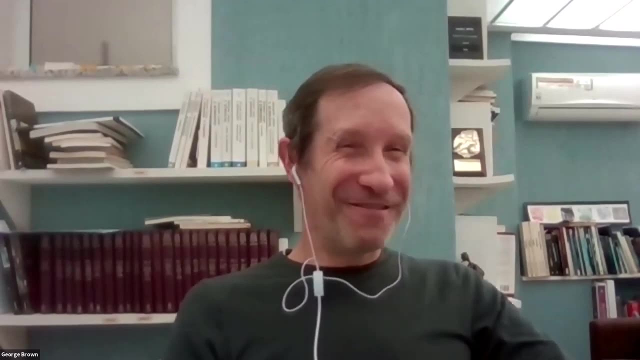 which would then benefit other organisms. But what about adding organisms? Well, in terms of the microbes, I'll let Kelly answer that. sorry, Turja. Okay, Barging in on this, Richard. But in terms of introducing organisms, such as larger organisms like earthworms, for instance, 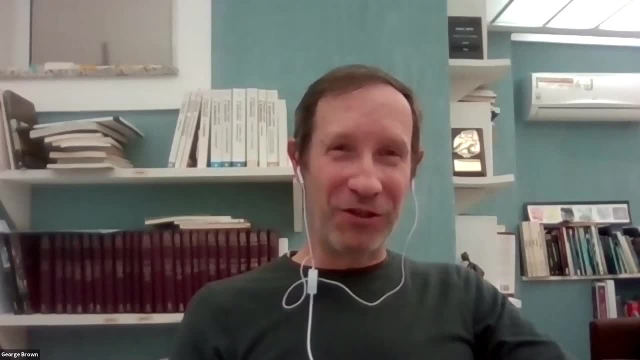 this is something that I was challenged with when I arrived here in Brazil was for the no tillage system. for instance, how can you inoculate deep burrowing, you know anisic type earthworms that are gonna take the litter and stabilize that organic matter? 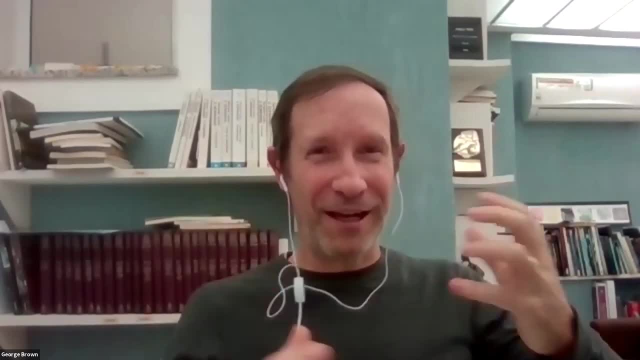 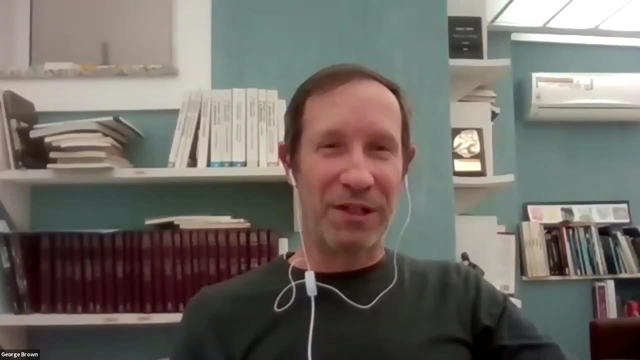 that's accumulated on the surface further down and help promote carbon sequestration and all that kind of stuff, And really because we have very few of these kinds of earthworms here in Brazil and my gut reaction is always: well, you know, a lot of organism introductions. 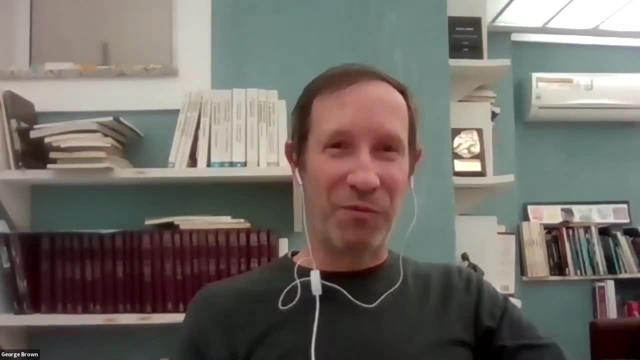 throughout the world, have wreaked havoc, you know, have caused more problems sometimes than they really were aimed to solve. And so, you know, thinking of what you're gonna introduce and where you're gonna introduce. it is very important, And you know if it's an ecosystem. 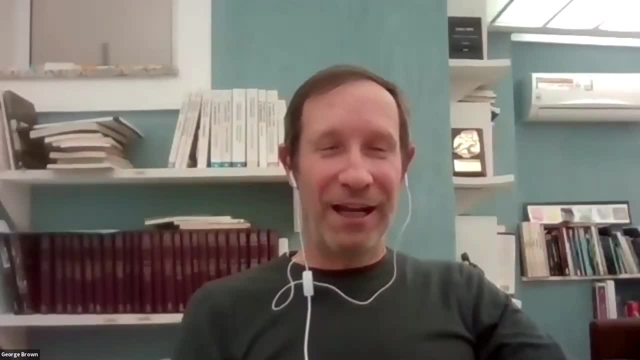 that's basically well contained and you can guarantee that that's not gonna go wild and that it's gonna spread all over the place and that it's gonna become an invasive species, then okay. But otherwise it's always an issue of bringing in an exotic organism. 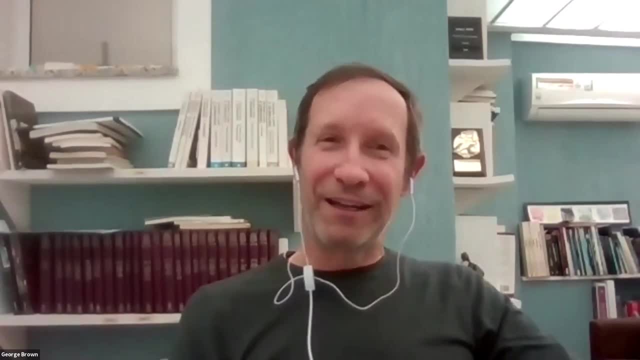 or an organism that's not native from the site, and what problems that may cause. Now, if it's a species that's already present and it's just re-inoculating it, of course, then that's fine. But for our experience with earthworms, 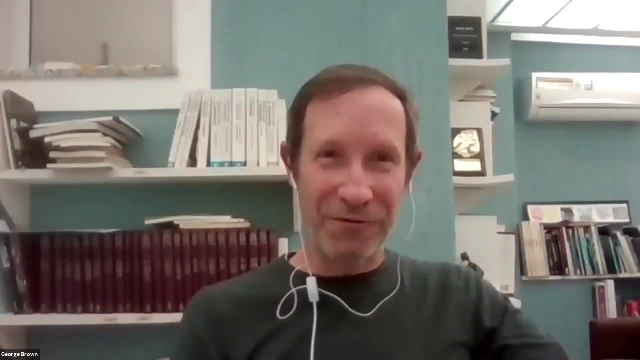 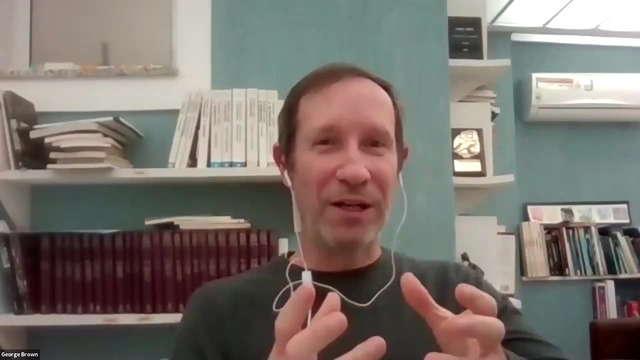 is that it's really quite difficult. You know you have to again feed that organism and maintain it in the soil And you have to think of a whole suite of management practices that will allow it to stay in the system and contribute to its ecosystem function. 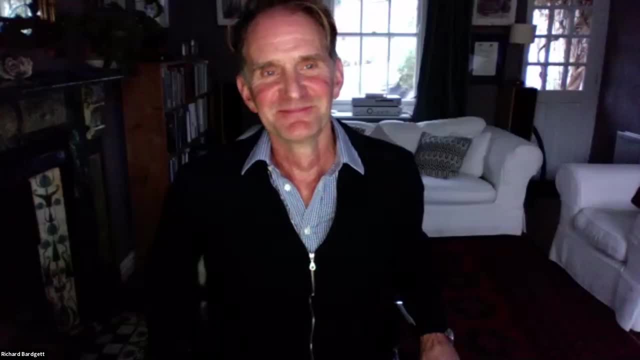 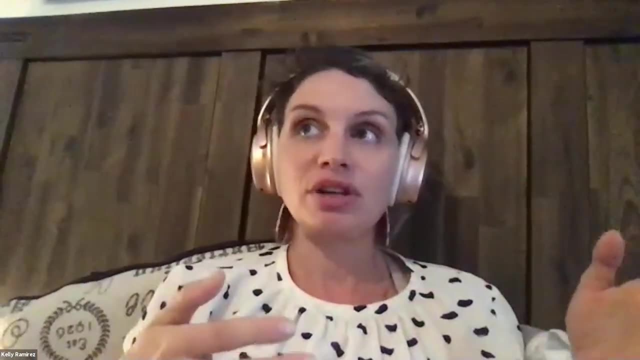 George. so, Kelly, what about microbes? Yeah, I think what George said would be the same for microbes: just willy-nilly like thinking that one soil could easily be transferred with the microbes could be dangerous if you don't know all the organisms there. You could bring a nematode. that is a pathogen right? I do think that there are. so at the NEO, yes, Jasper Wubbs did a really cool study where they transplanted topsoil to like a barren field. 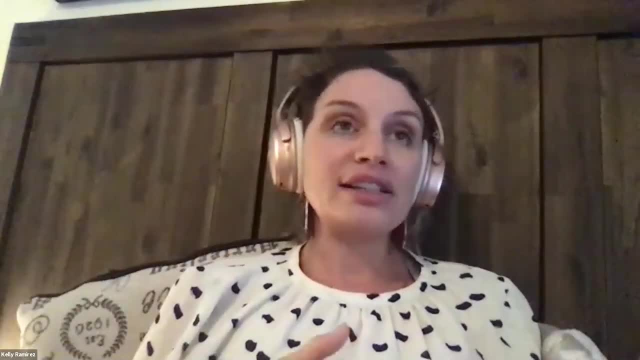 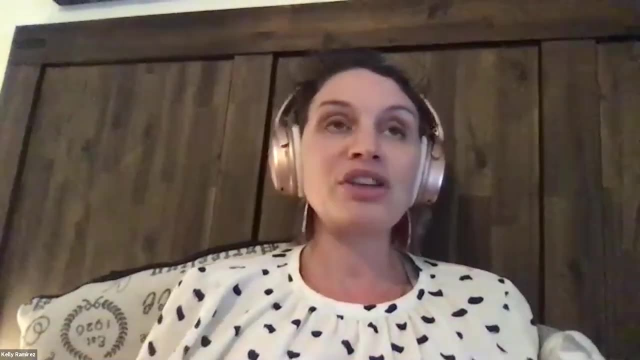 to see what would happen, And they did multiple ways, Like sterilizing at first, if it's just the seeds that go on, versus with microbes in the seeds, And that was really a lot better. So there are, but they're taking soils. 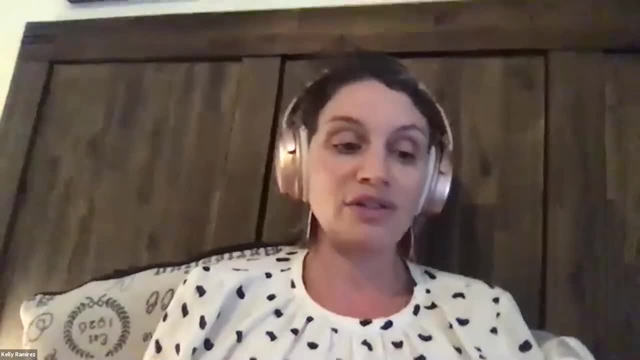 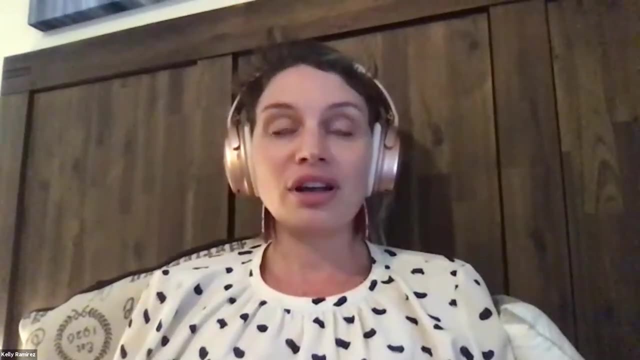 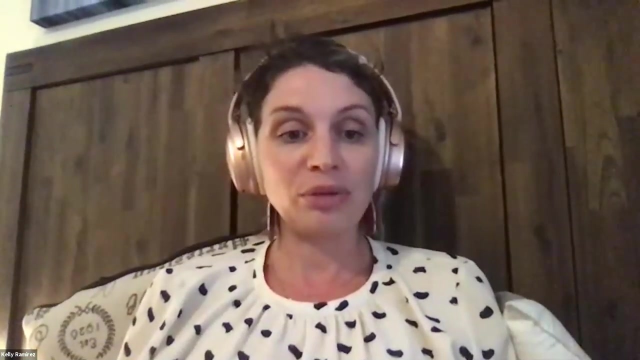 from not that far away. They're not. they're from the same region, right Or even pretty locality. So I think there can be some clever ways to do that. Some other thoughts. instead of actually adding an organism, it's perhaps promoting organisms that you think would do. would be better for your system. So perhaps you just need to add a lot of carbon in nitrogen to get the microbial community going, the decomposition cycle going, and then you're going to have that food web build back up again, right? So it might not, the microbes might already be there. 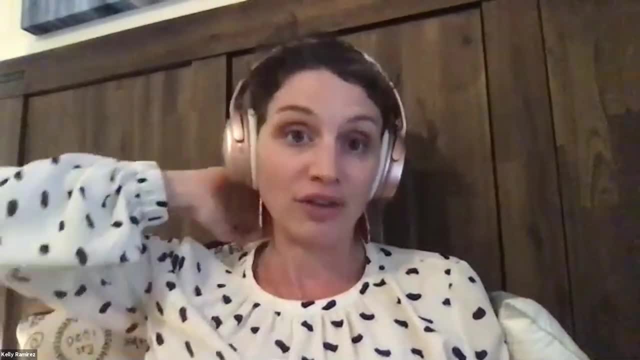 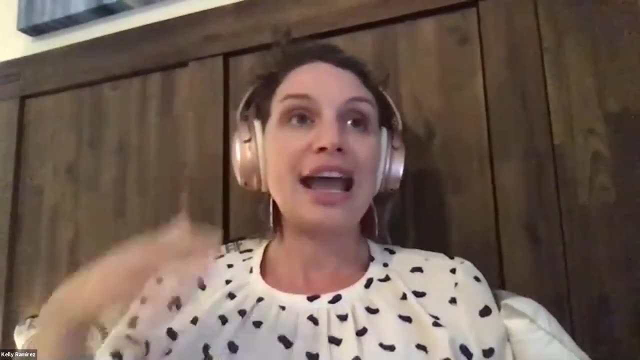 They might already have those functions for those just some, those basic soil functions that we think about. And then it's like how can you layer on the rest of the food web If the microbes start being really functional and the nematodes are happy then and the mites are happy? 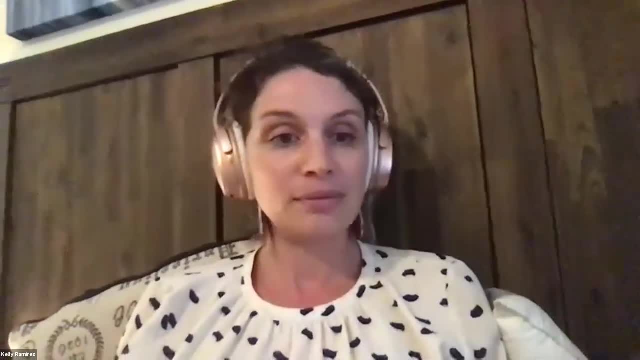 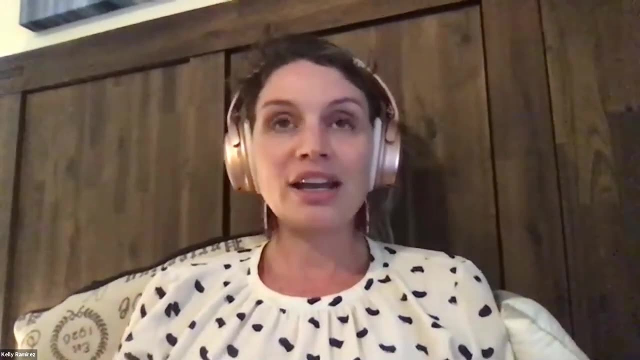 you know, like it's kind of going from there thinking of it as a bottom, bottom up approach in size for organisms. That's what I would say. I think it's a really interesting topic, though, And I don't think that we're close. 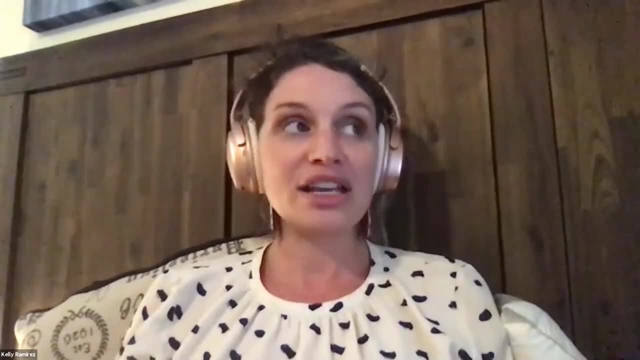 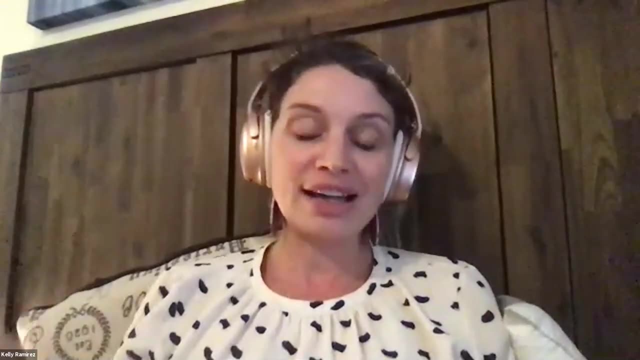 to having one answer for it because, again, if you're thinking of doing this in agriculture, it's really, really important to worry about pathogens, But if you're thinking of doing this maybe in just a grassland, you don't have to worry that much. 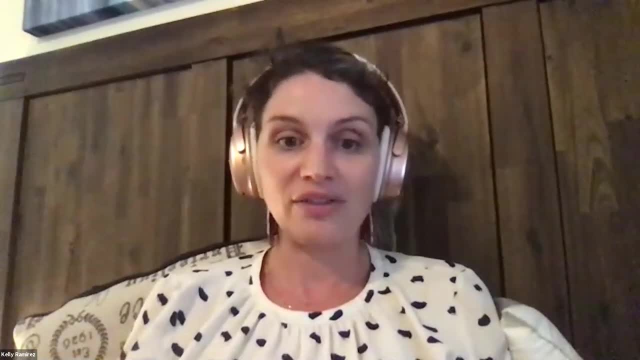 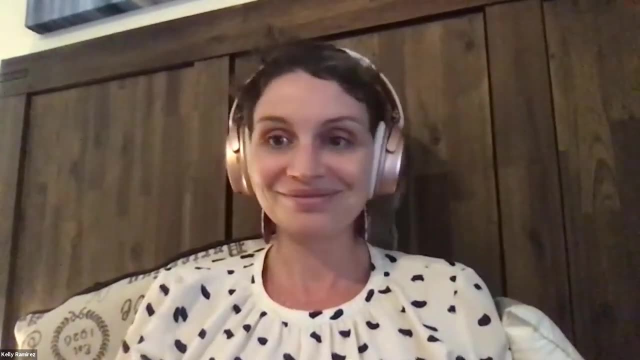 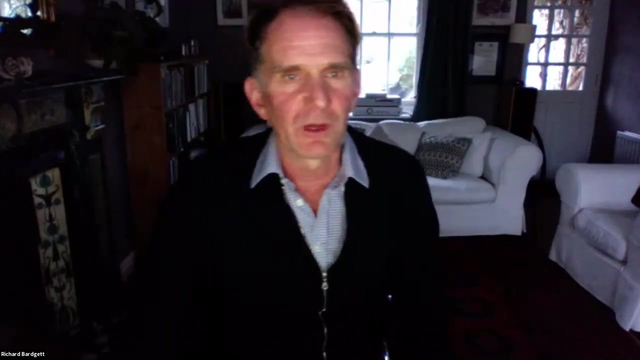 because you're not relying on that crop to survive and probably a high plant diversity can overcome something that you bring in. Yeah, that's sort of some thoughts. Okay, thanks A lot of the questions that have come in. I've talked about threats to soil biodiversity. 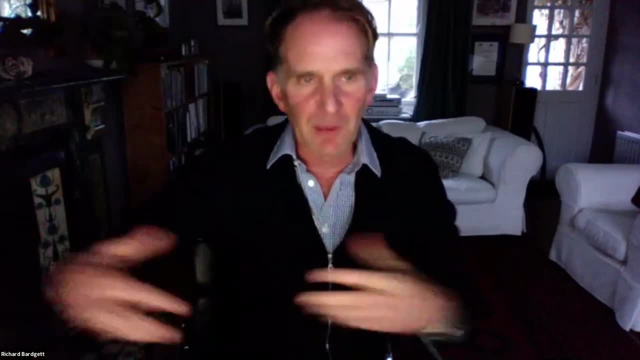 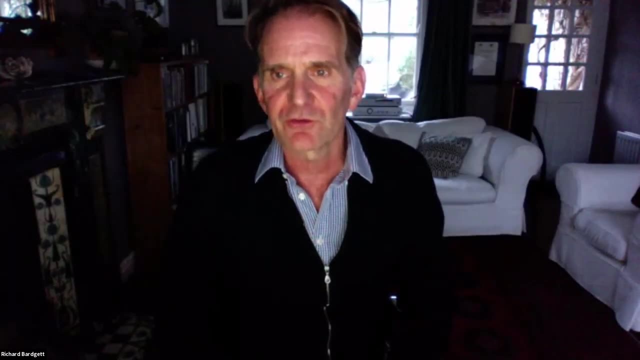 We talked a bit about how we can encourage biodiversity and the beneficial sides of biodiversity, but there's quite a few questions coming in about what are the main threats to biodiversity, And one of them, sort of picked up on me, was from Jean-Pierre Caliman. 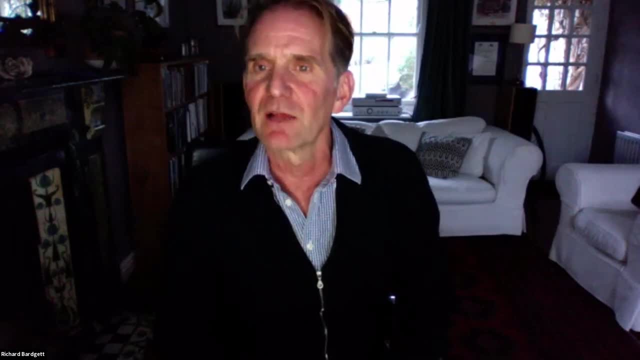 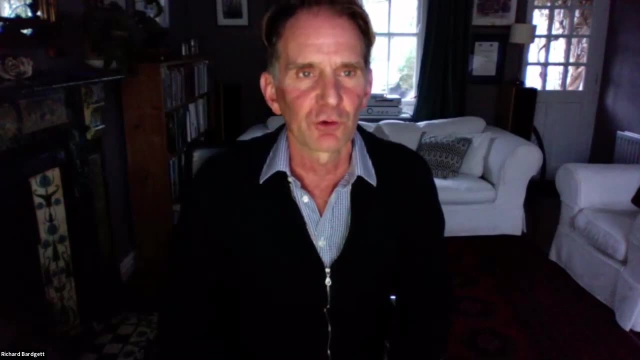 who asked the question a while ago now, actually, And it was about: is all agricultural intensification negative for soil biodiversity? Because we often talk about intensification being one of the sort of biggest threats, or land use change as well as being one of the biggest threats. 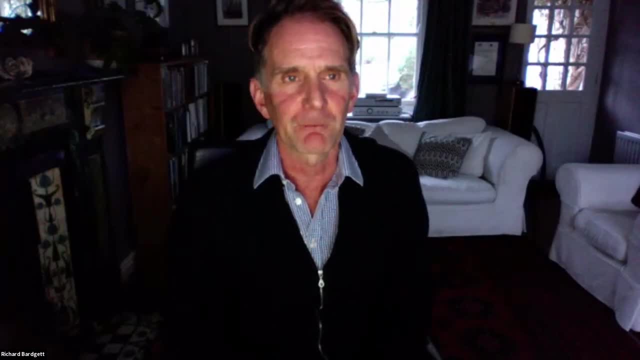 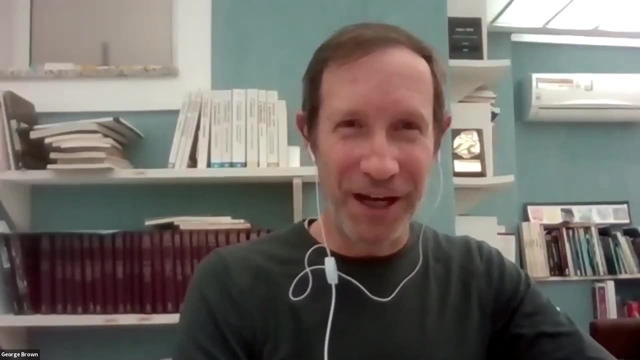 but is it always a bad thing? And I'm going to ask George that question. Yes, I saw this question and I thought it was great because, yes, there's all kinds of intensification pathways and there's all this talk now about sustainable intensification pathways. 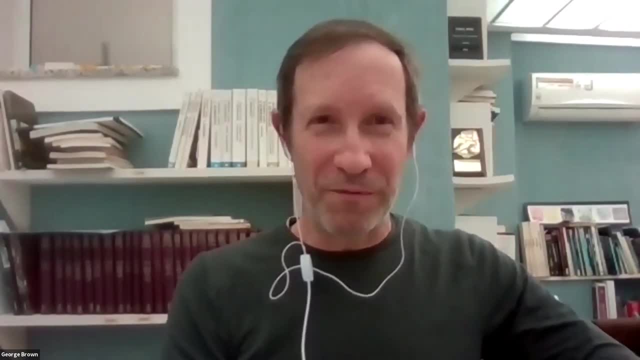 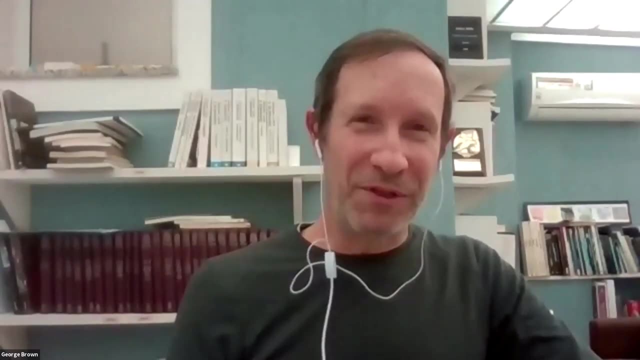 And, of course, these are means of obtaining more from your area per unit area, but not necessarily putting more in, So it's oftentimes a question of making the system more efficient in what it does, And so having including certain plants that can be deep rooted. that can bring back the nutrients that have leached, or including plants that are nitrogen fixers so that you can add nitrogen to the soils for the coming crop. And what are the coming? pasture, or pastures that are mixed with legumes and grasses. So all sorts of pathways that involve a lot of management, tweaking in a sense, so that you are improving nutrient cycling, internal cycling within the system, And then, of course, if there are particular inoculants that you need to do, like inoculate with nitrogen, fixing bacteria. 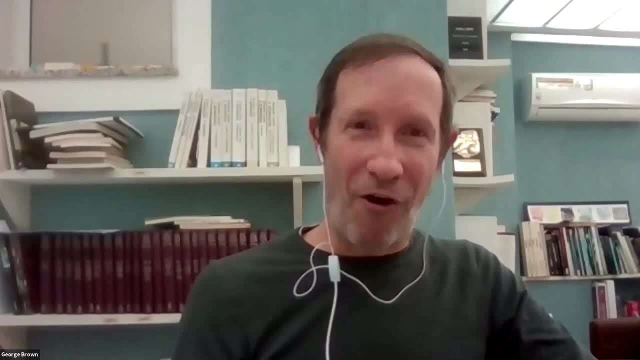 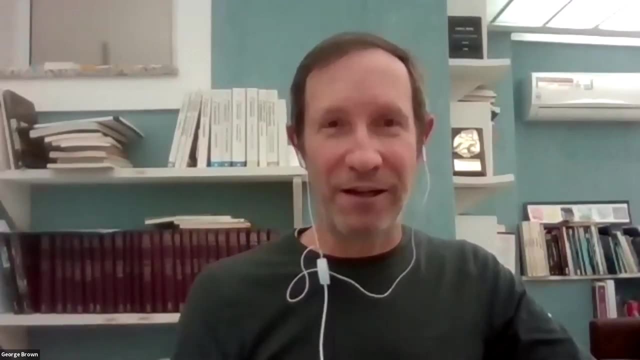 yes, you go ahead and do that, And so various techniques are already available for improving managements and intensifying the use of the land without necessarily bringing on more inputs and with reducing costs to the farmer. So those are means of ecologically intensifying agriculture. 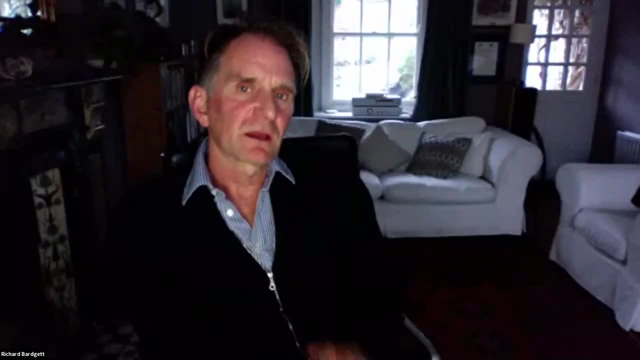 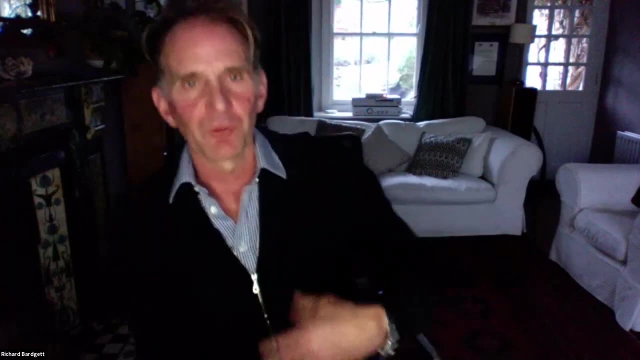 without leading to soil degradation. And I'm gonna ask the same question of Elizabeth actually, because again you work on sort of restoration, which is a different kind of context. It's the opposite almost. but I mean again, would you? 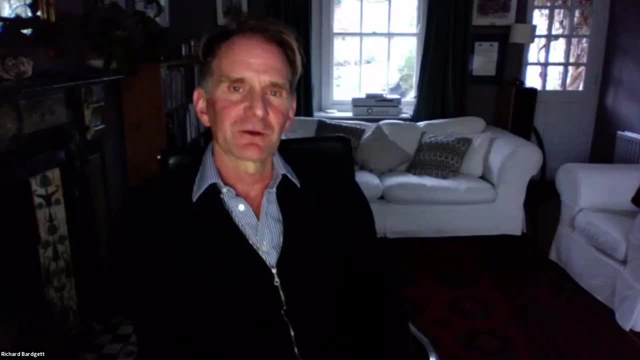 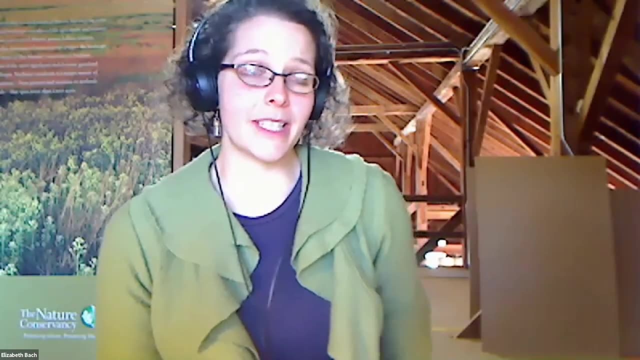 would you say intensification is always a bad thing, or can it kind of be? Yeah, I think that's a great question. I thought George's answer was really lovely for this and that it kind of depends on how we think about intensification. 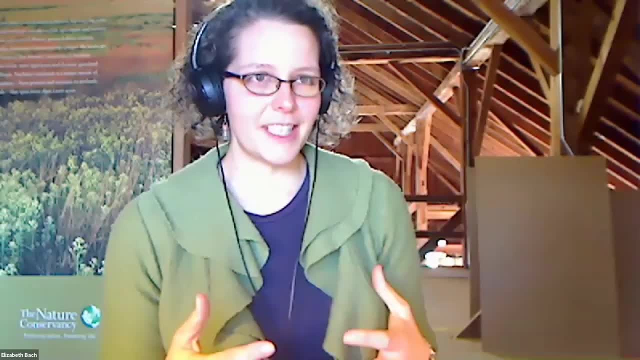 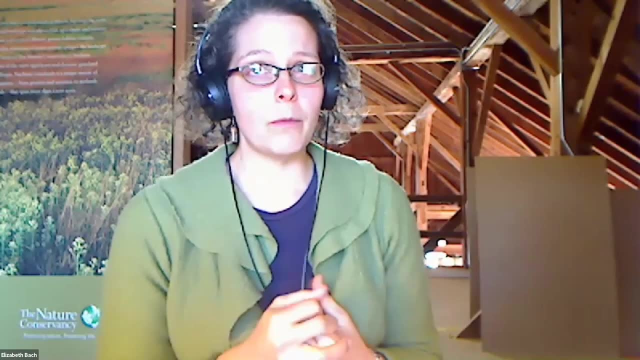 And if we're really thinking about it as building efficiency and bolstering ecological connections, that could be a boom for soils. Yeah, in my work we are. we're exactly thinking about the opposite of how do we take land that's been intensely farmed in? in a row crop context, These are usually corn and soybean fields and bring plant diversity and animal diversity back to that, And the soil communities are a huge component of that. So we're often thinking about how do we get more carbon and nitrogen into that system and reestablish those. 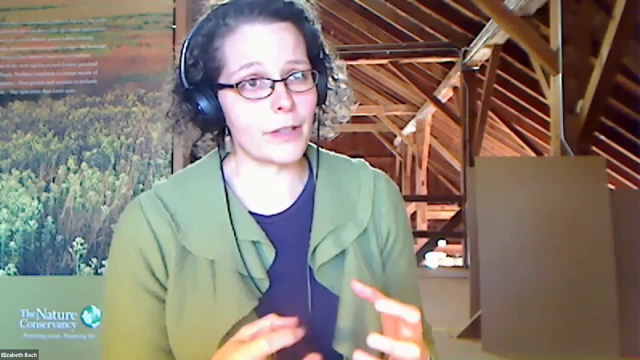 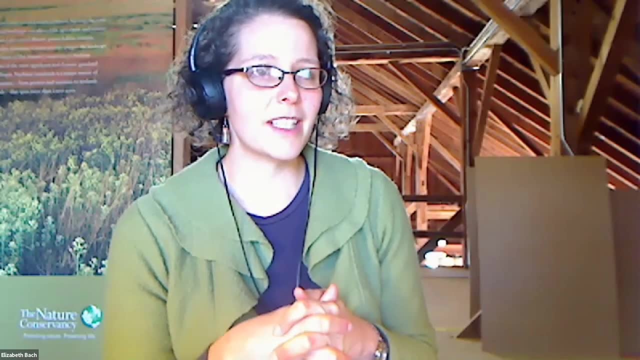 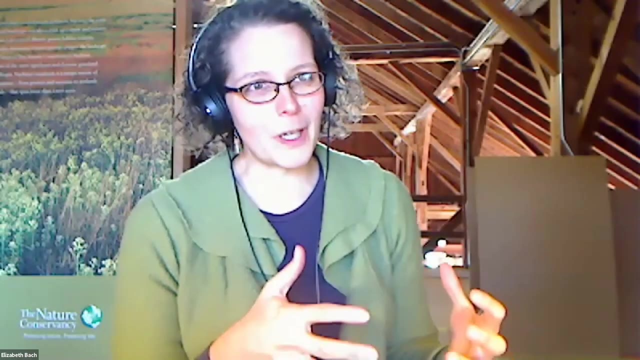 those food webs and create, I guess, a tighter system, a more efficient system, And that could be a way of thinking about ecological intensification And it's also, I think, in kind of a landscape perspective, useful to think about mingling, restoration work. 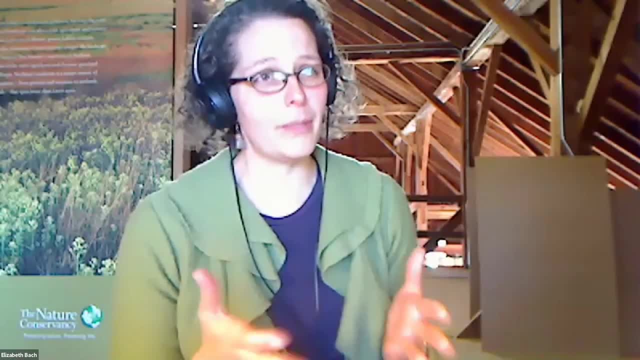 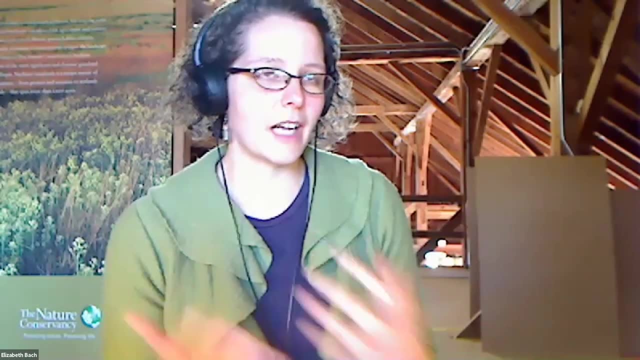 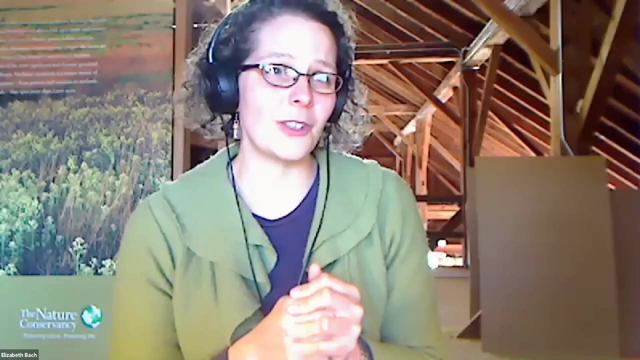 with agricultural work within a landscape so that they're both benefiting from each other, and restorations can help balance some of the, I guess, outputs from an agricultural system, and agriculture systems can benefit from things like increased pollinators and natural pest control from these restorations. 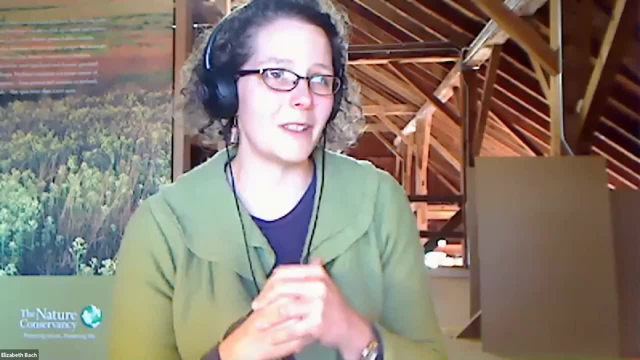 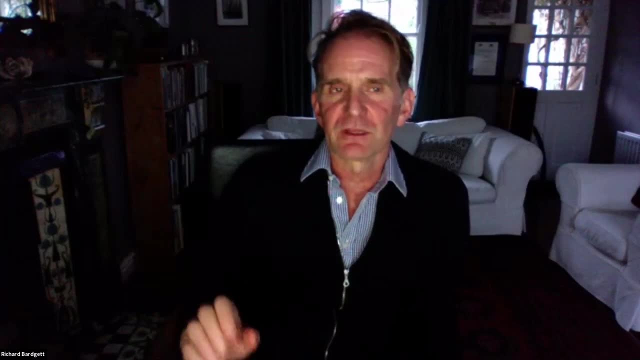 So from a from a bigger landscape perspective, that might be another great way to look at that. Okay, I'm aware that we're running short of time. We've only got about 15 minutes left and we've got quite a lot of questions. 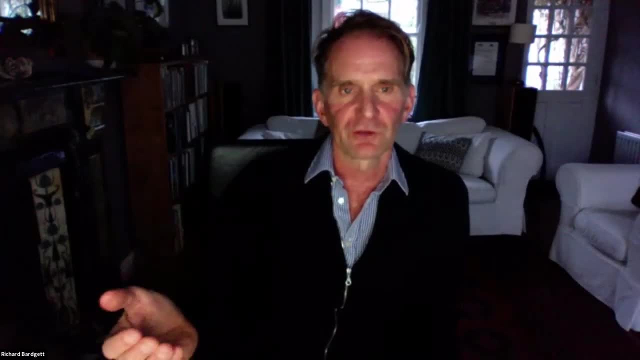 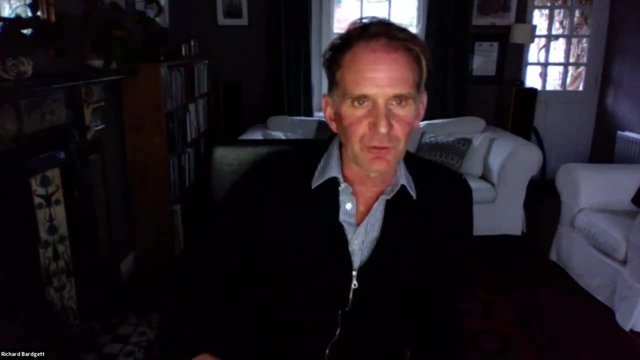 and quite a few of them are asking about a topic we discussed earlier, about actually translating soil biodiversity knowledge into practice, which is something we talked about. It's something we talked about when we were introducing the subject, So I just thought I'd spend a bit of time. 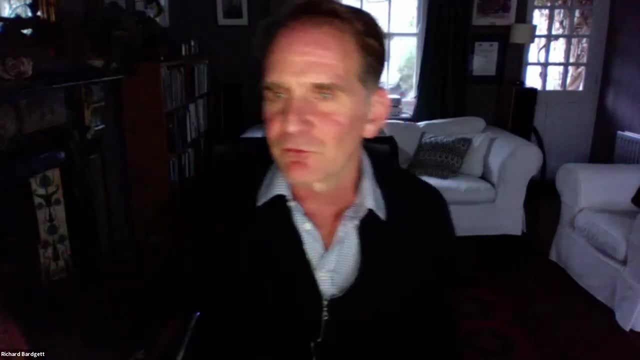 on that particular topic And one of the questions I can't- I'm afraid I can't see who asked the question at the moment, but it's one that seems to be quite common- I'm going to actually ask all of you this: 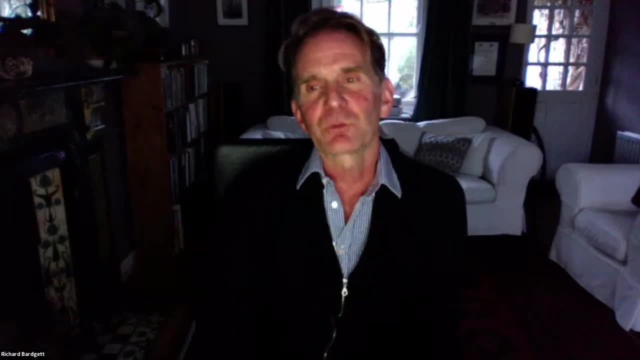 but so I'd ask you to give a short answer, if you can. is what? what would you say are the biggest barriers to actually getting this knowledge into policy and into practice? And I'm going to ask Zoe first. She looked the calmest when I asked that question. 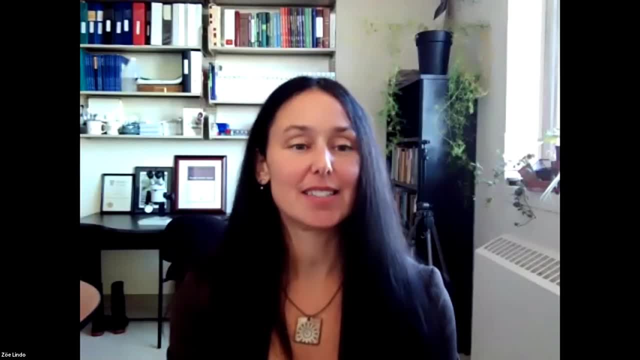 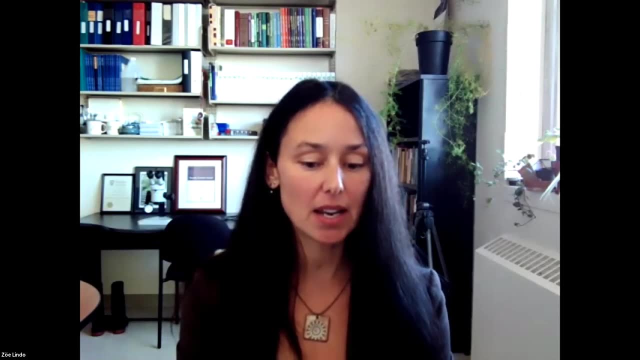 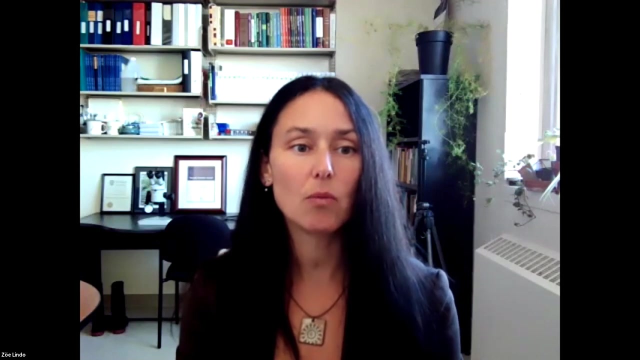 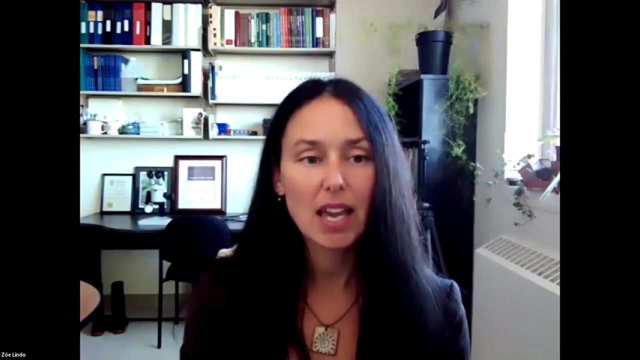 Oh dear, the biggest barriers, I think. I think, historically, the biggest barrier has been almost the fact that soils are so ubiquitous and they're everywhere, They're right there beneath our feet- that we do tend to forget about them. We tend to forget about the functional role that they play. 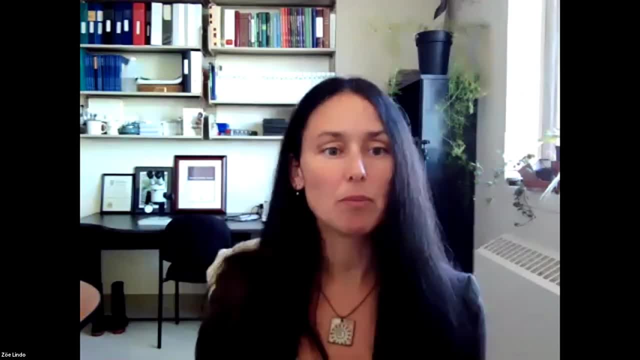 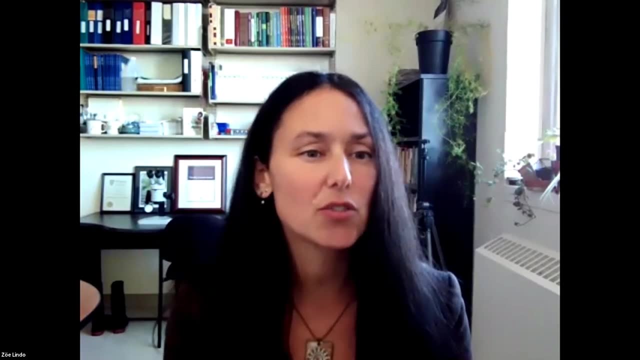 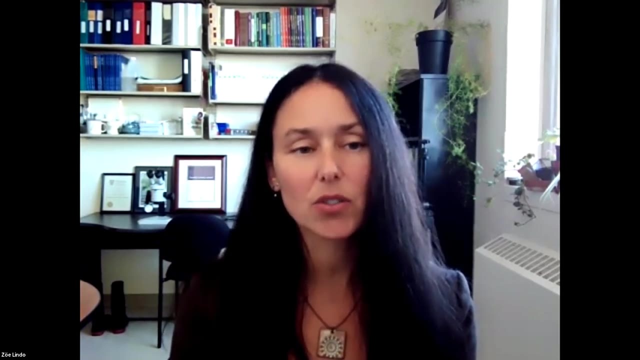 not just in agricultural systems, but some of those broader functions like climate regulation, And I think the biggest barrier historically has just been that they've been ignored, And I think that's why reports like this are so important, because they just bring our knowledge to the forefront. 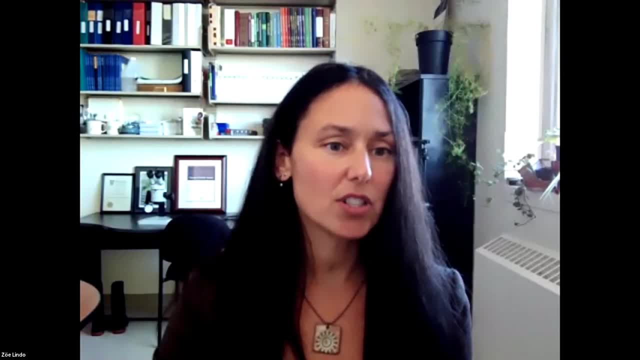 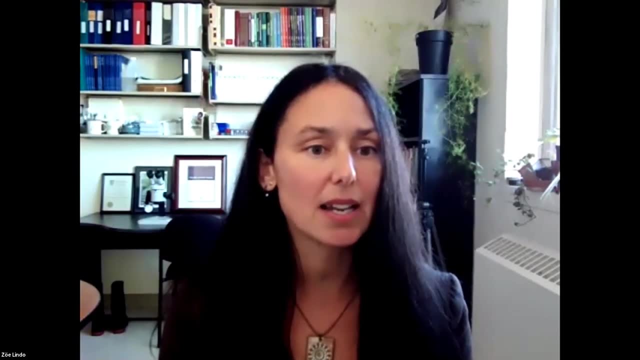 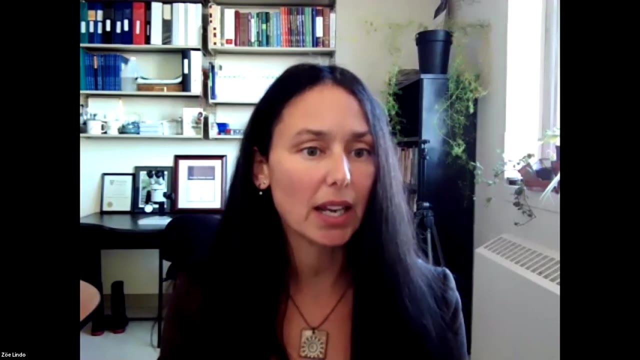 and they put it in front of the policy makers, And I think just that information going forward will translate into policy, because I think our research is clear: Soil, biodiversity play an important role in the functioning of the planet and we can't afford to ignore it anymore. 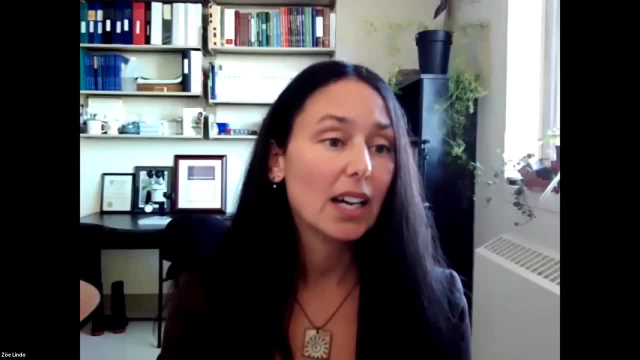 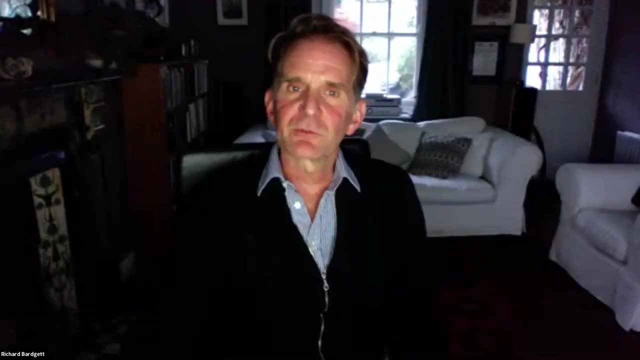 And I think once we just bring that information forward, like we are, I certainly hope that it's going to translate into policy. Okay, thank you, Elizabeth. Yeah, this is a great question and certainly something I wrestle with, I think, on a daily basis. 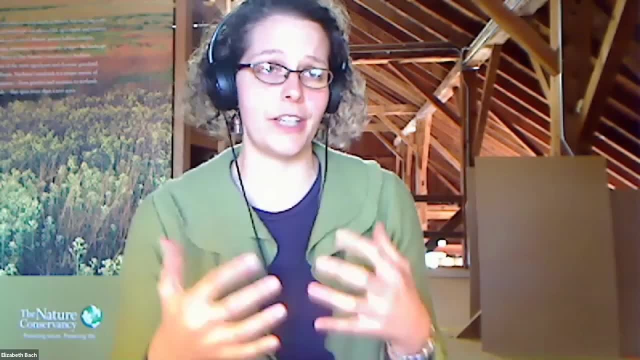 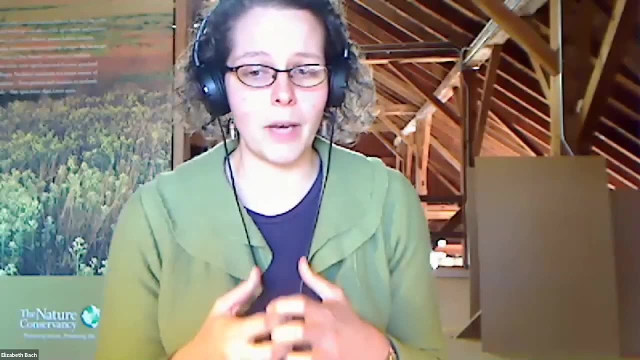 In my experience, when we're really talking about this, when we're really talking about this, when we're really talking with land managers and farmers, they want concrete information that they can bring into their daily practices on the ground, And that's things like: 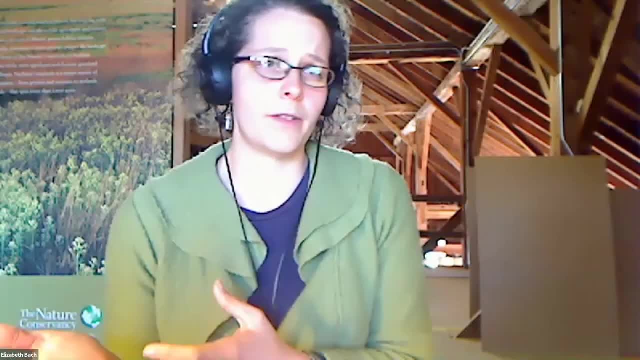 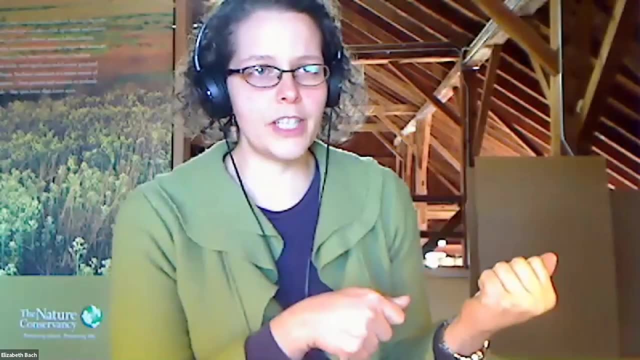 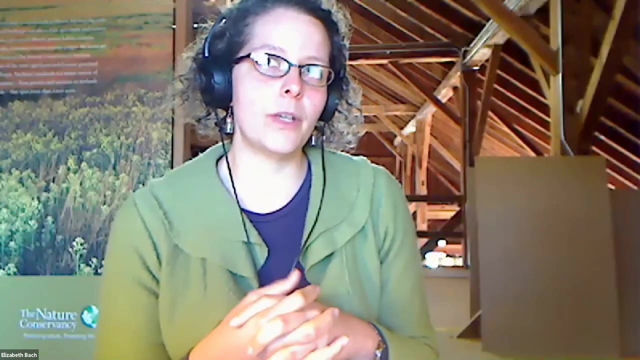 should I be inoculating with my crazy for this rare species I'm trying to reestablish, or should I be managing to get more earthworms in my field? And it's very local and context specific And I think one of the hurdles that we face is science is always looking. 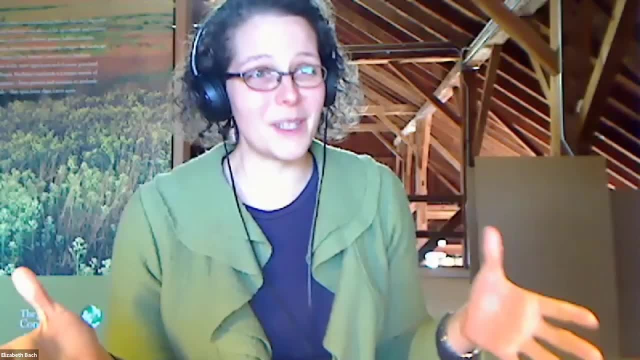 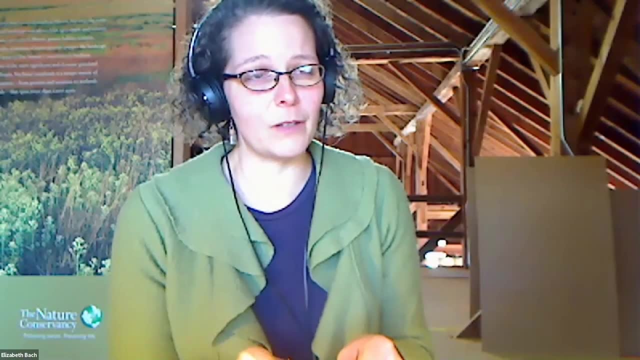 for these big general patterns, which are super important because it helps us understand what works generally across the board. But sometimes that can be a bit of a barrier for providing really specific local advice, which is what a lot of managers and farmers really want to know. 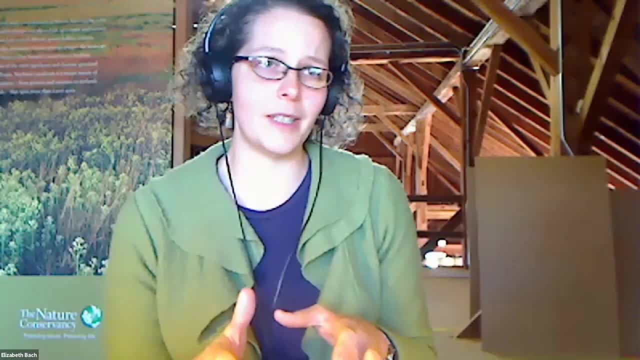 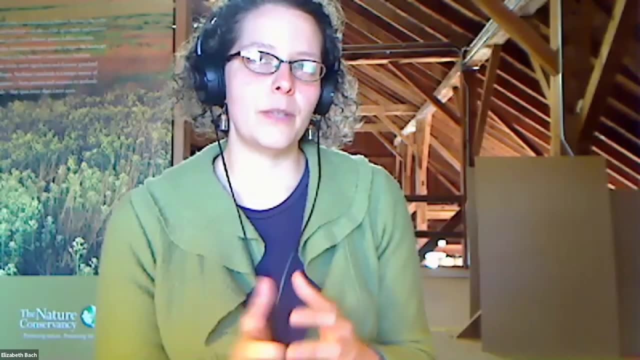 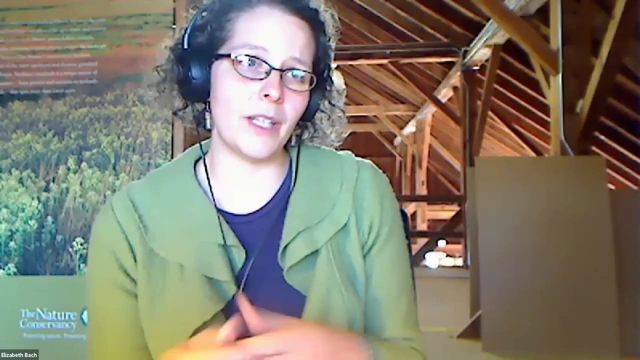 And so I think, continuing to build this bridge- and people are working on it on both sides, but we still have a ways to go to. you know, bring that conduit from understanding general principles and advancing general principles and distilling those down to actions that people can do on the ground. 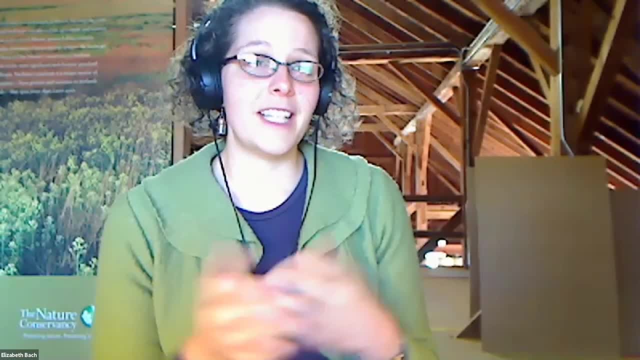 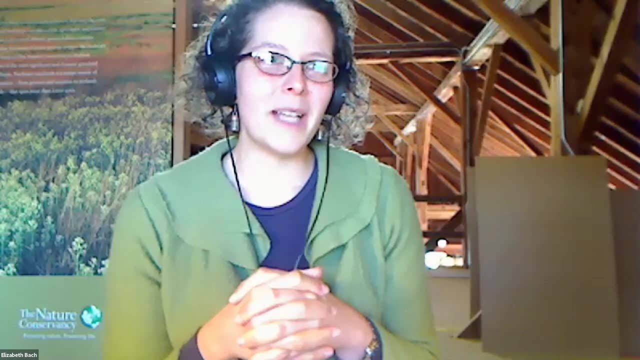 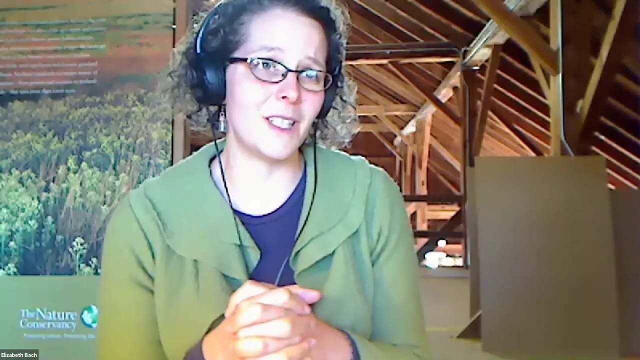 So a lot of times I personally advise things like: well, feed the soil and benefit- and it will benefit all these critters in the soil community, as opposed to rushing to inoculate when we're not sure if that inoculation could turn into a pathogen or an invasive species situation. 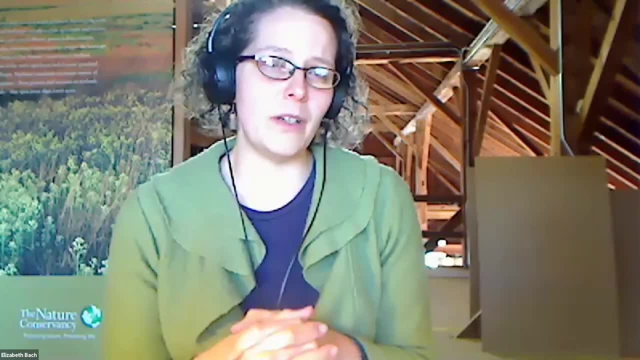 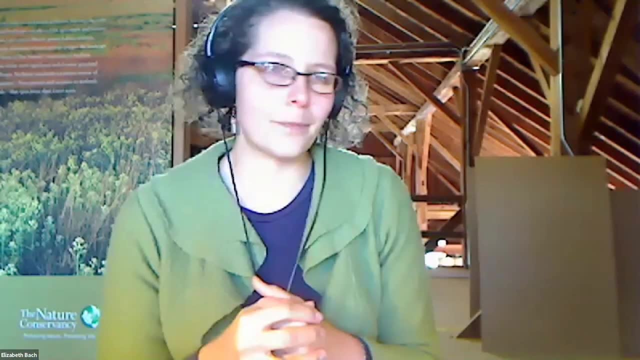 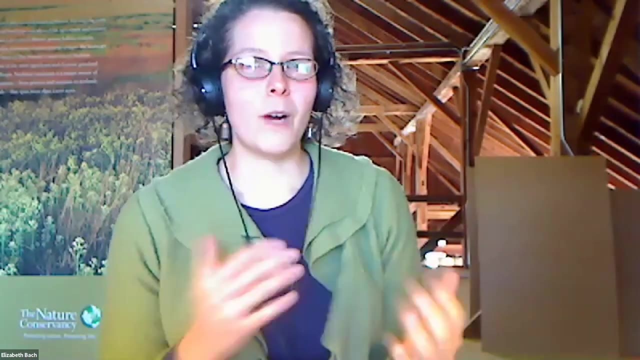 because we know that feeding and supporting that community will be a benefit. and here's some examples, in you know your specific context, of how to do that: leaving you know litter on the ground or altering prescribed fire regimes, that sort of thing. so i think that, um, walking that balance of 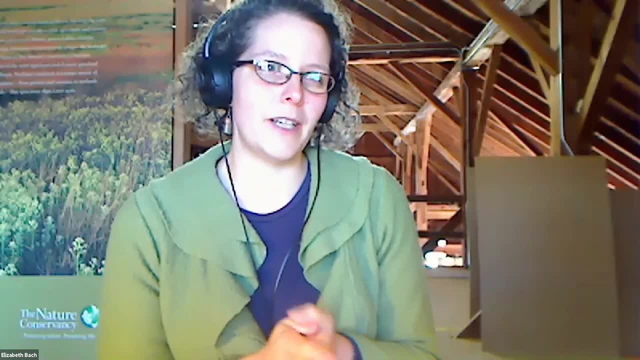 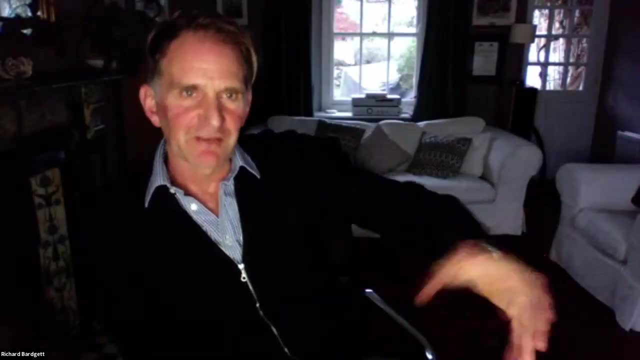 bringing that advice down to be as concrete as possible with land managers and farmers is really important. thank you, i'm gonna ask kelly now, but but i'm thinking that you- i mean you- were one of the managing editors of the report, so you had a very senior role. so i wondered, you know, in the 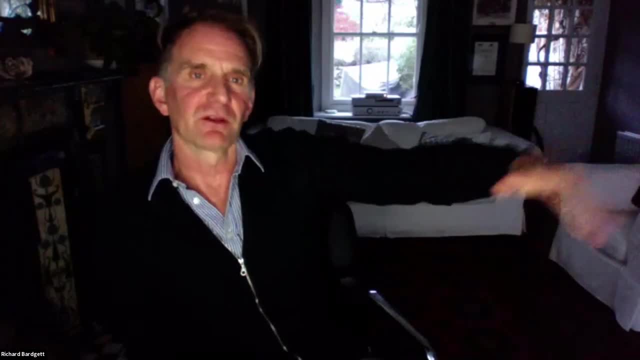 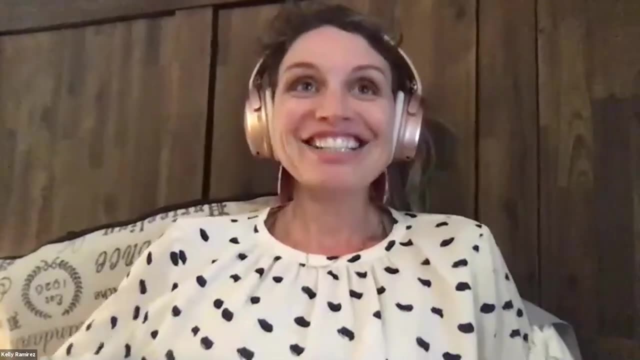 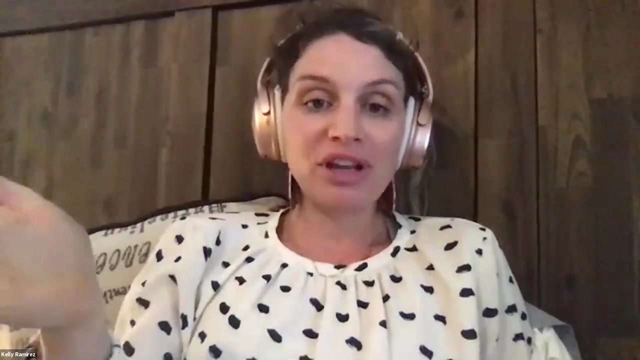 context of report. what kind of messages are there in relation to how we best achieve that translation to policy? oh, so, i think that what we found is there's not enough. there's not enough pathways to get information to policy, people, land managers and also the public. um, and so i was, since, uh, zoe. 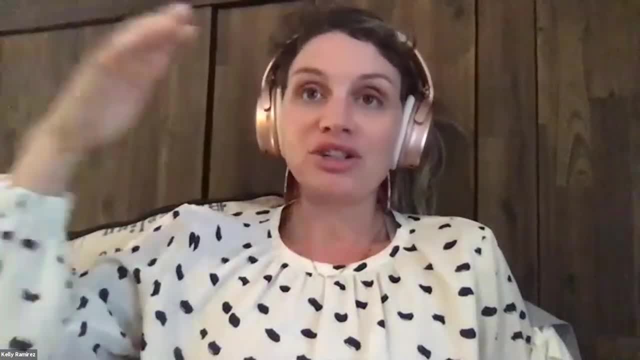 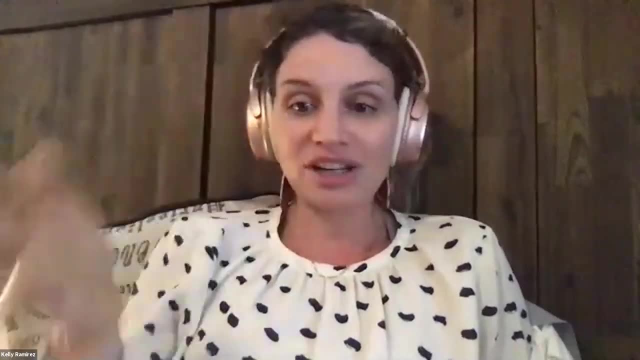 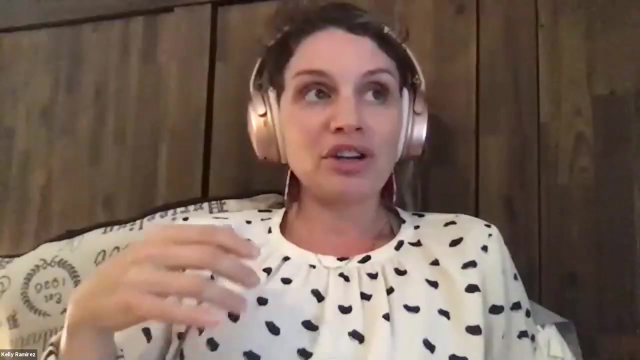 and uh, elizabeth talked about kind of like reaching land managers and policy makers. i'm gonna. i think one area that we can is almost low-hanging fruit is like public um, and someone actually put in a comment on: we should have a soil biodiversity museum, um, and education of soil biodiversity, while soils are ubiquitous like zoe. 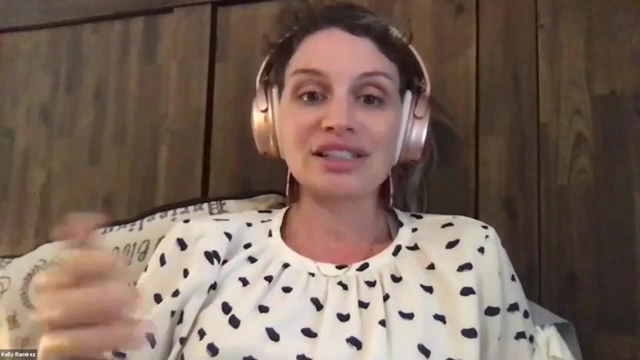 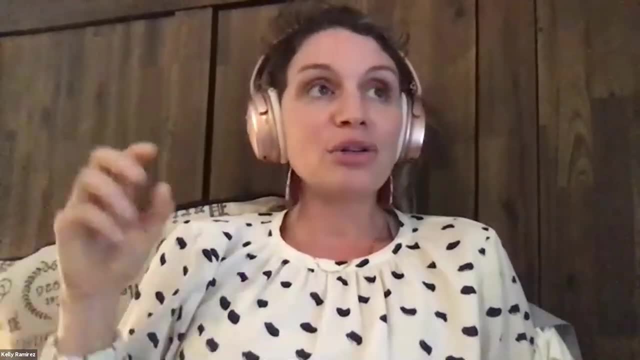 said we're also. the majority of people today are disconnected from soil. they get their food at a store. they don't have to go farm it. perhaps they have a small farm in their backyard. but those that the public can make with the soil can go a long way, because then it becomes something that 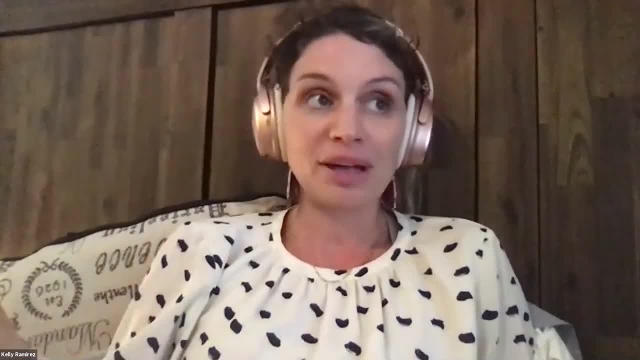 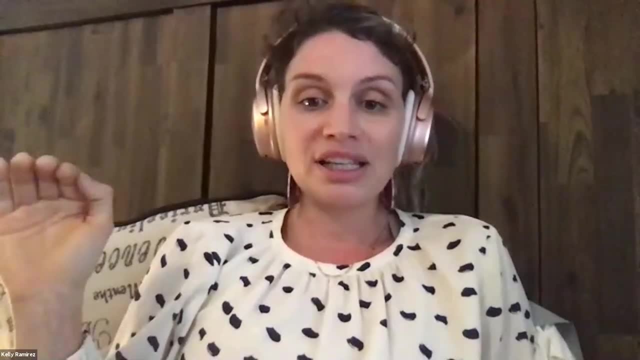 the public is asking for in their environment. kids grow up learning about soil biodiversity and it grows up to be something that's important in their- uh- local government perhaps. um, we see this in the netherlands. they do a soil biodiversity count every year. everyone knows what a nematode is. 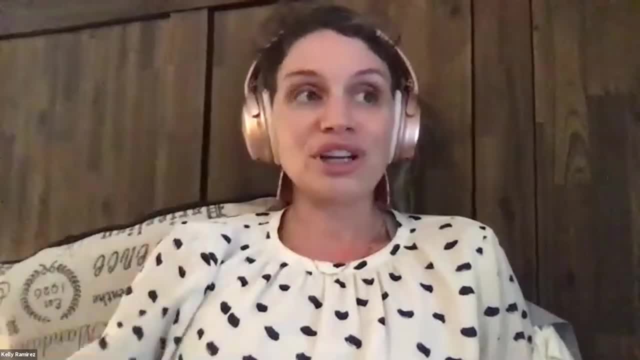 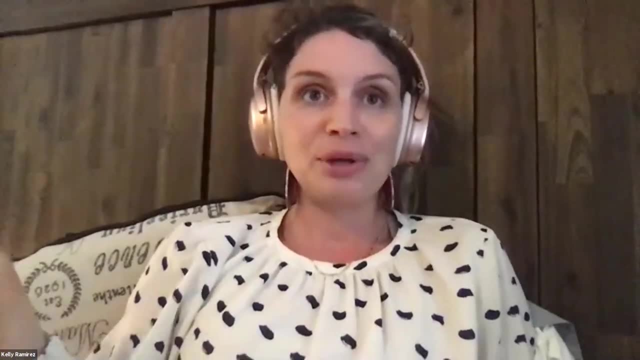 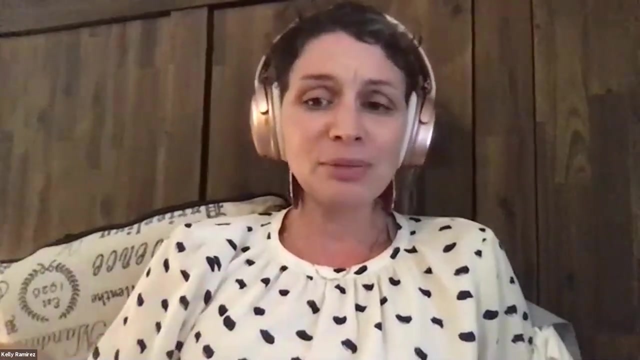 in the netherlands right and so that public outreach, whatever it may be, if it's a museum, if it's. we did a paper on soil biodiversity in central park and people loved that. right, they want to know that soil that is right outside their door can be interesting- the people that do the antibiotic work. whether you could send in your. 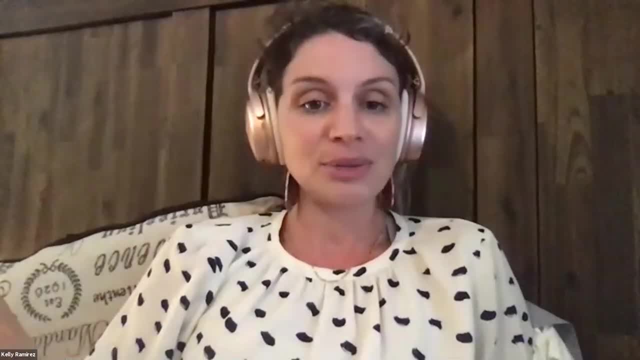 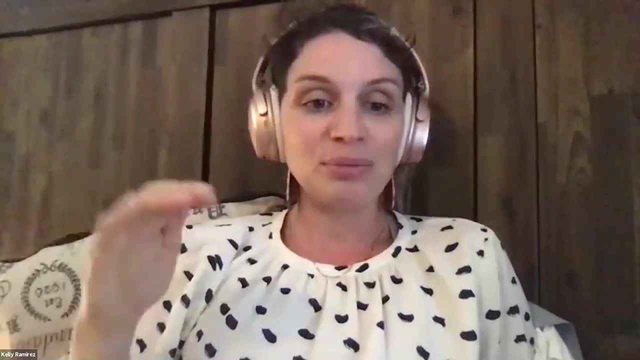 backyard soil and people would look in it to see what new antibiotics were there. this is just community science. this isn't. this isn't like um. a scientist went and collected all the soils. people went into their backyards and sent it in, and i think projects like that um breaking down. 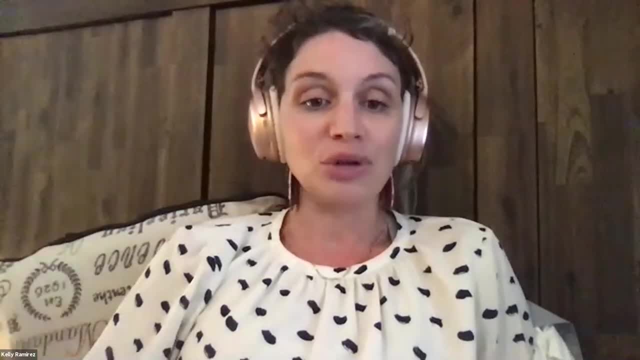 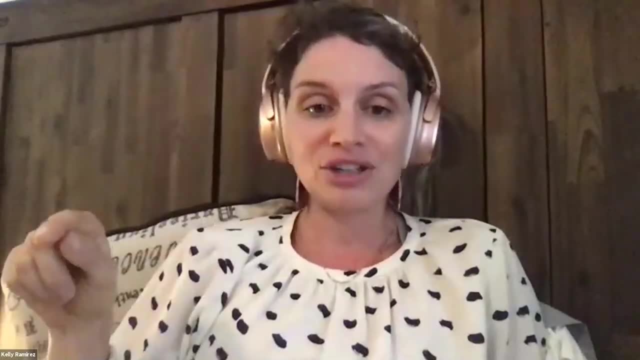 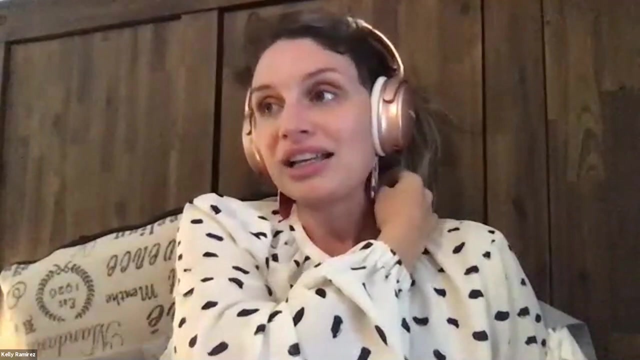 the wall between the public and the science and communicating is a really great way to go and like a different pathway to get in the end to policy makers. maybe that pathway won't get to land managers, but, um, i think that turned out to be like education in the public eye is one of our big gaps. i think for sure few people learn about soil. 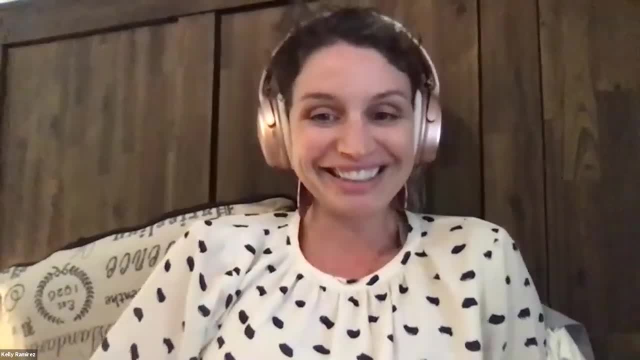 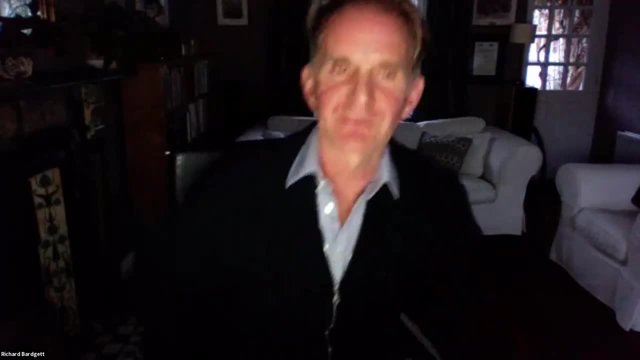 biodiversity in school, unless i'm your professor, actually that i was going to ask another question, very related, that was from kirsten uh hofmockel, about how you know what we can do as scientists to actually um, accelerate protection and policy and diversity. but again i just want to go back with george to the 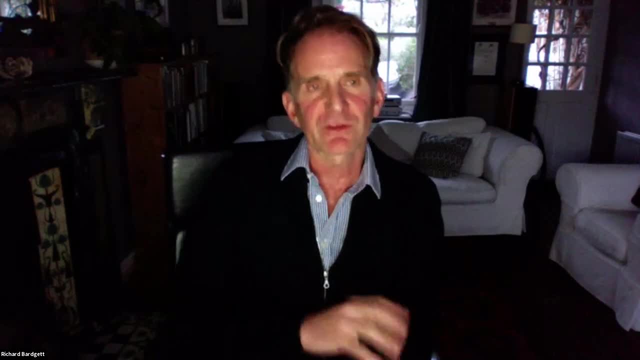 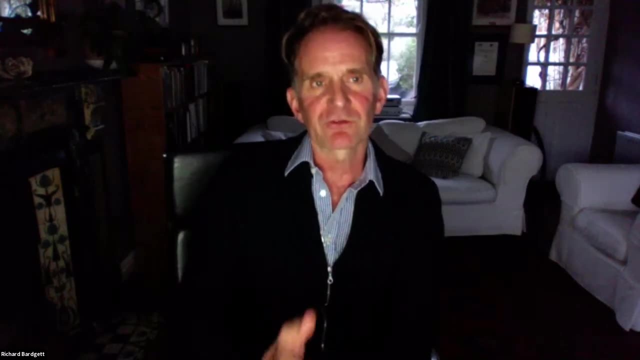 barriers question because, again, you work in a very different context to many of us in brazil, so i wonder if you could just say a few words about what you see as the most significant barriers to transferring that science, knowledge on diversity into okay, i think. i think that actually. 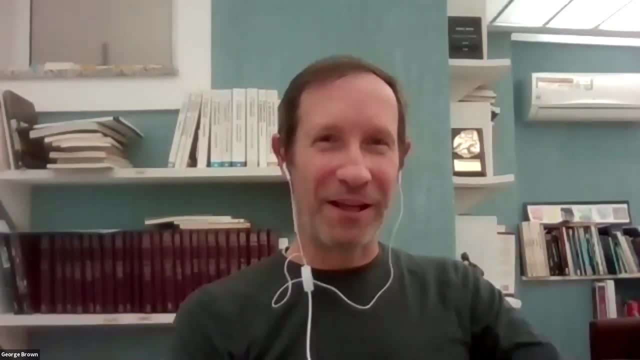 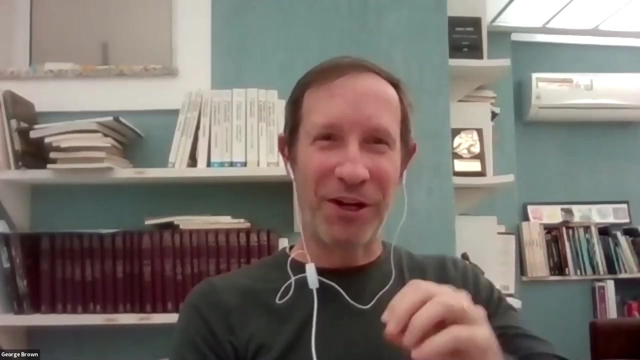 what um kelly, zoe and elizabeth have have said basically apply to what i'm i'm living with here in, you know, in my institution and in brazil, one of the things i'm sorry i'm gonna, i'm gonna not answer the question in that way. i'm gonna answer, i'm gonna come back to. 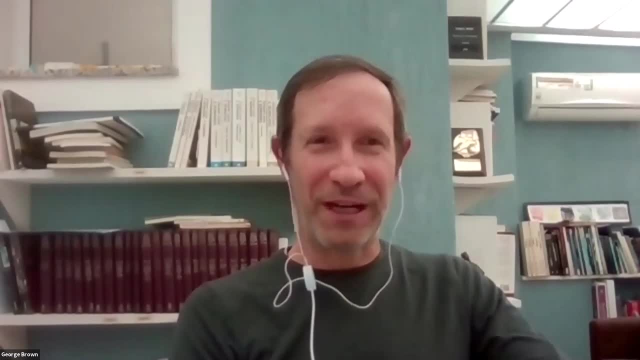 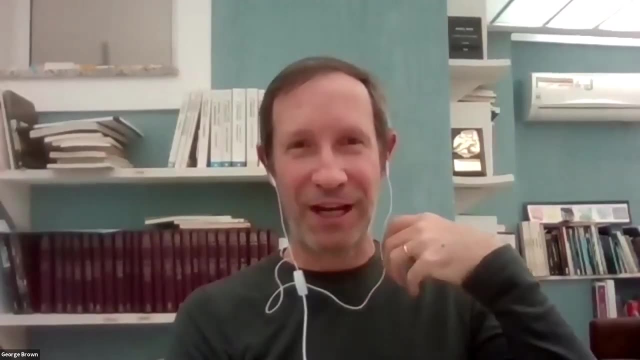 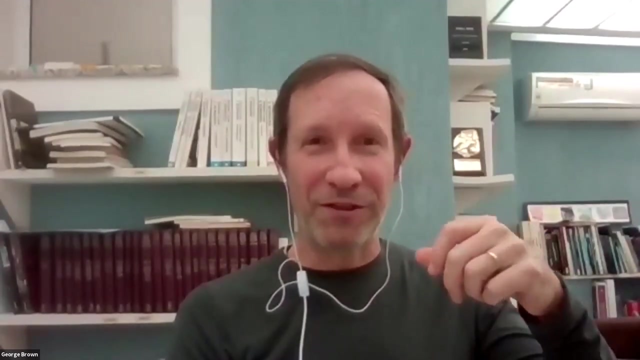 why we we did this webinar and why we thought it was important is really as scientists. why is it that we should be involved in this? and i think this this comes down to one of the one of the barriers, which has to do very personally with each of us, is that we, we need to choose to be involved. 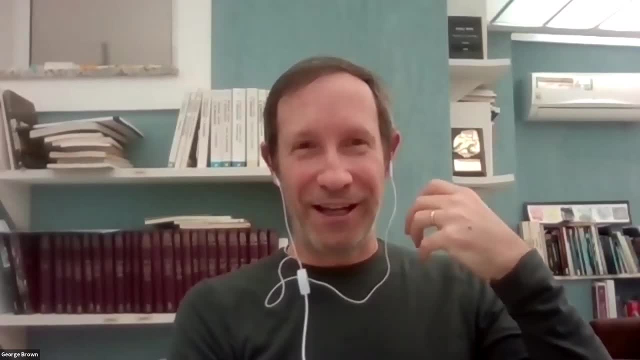 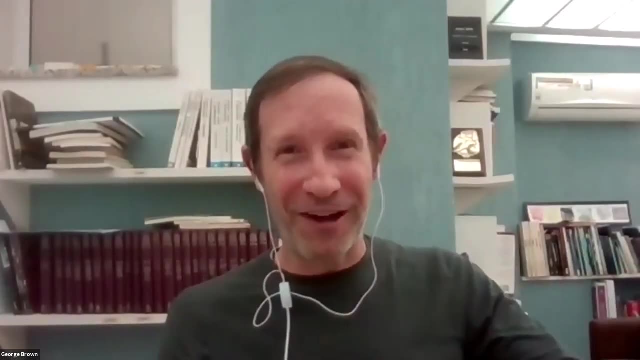 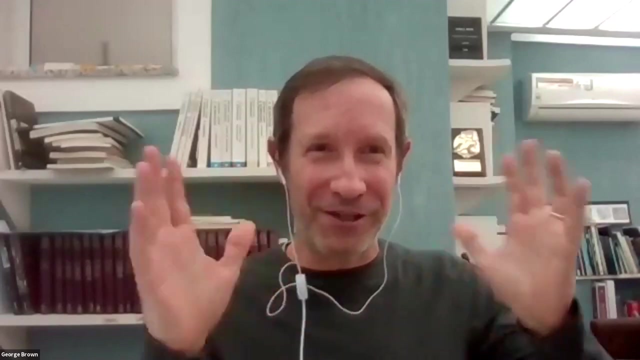 to become involved and to to actually get out of our little box and our comfort zone and expose ourselves to the media, to talking with farmers, to talking with policy makers, to going to these, these, these cop meetings that are. they're probably a big bore for, you know, in terms of scientists, because it's, all you know, different. 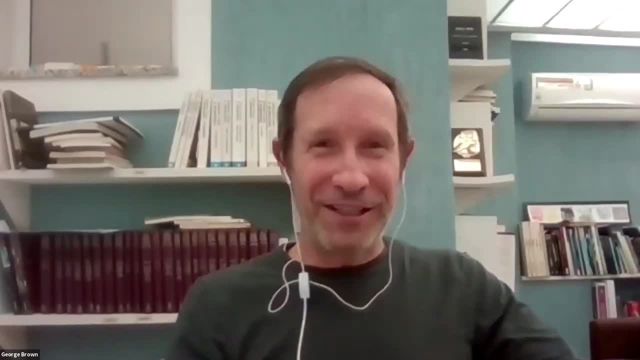 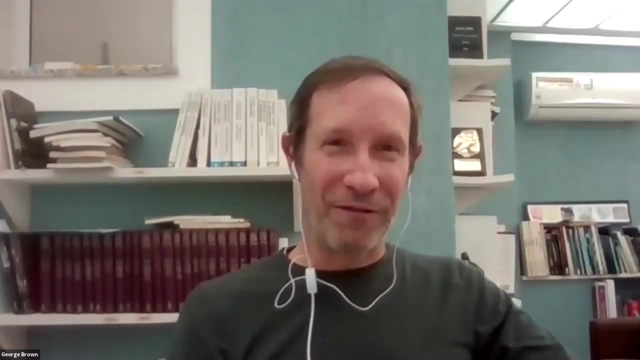 language. it's a different, different world, and you're not talking science, you're talking policy, and i think it's it's one of those challenges which which came to me in becoming involved in all of this and i i often shy away from it, very, very sincerely speaking, um, because it it does really mean going out of your comfort zone and it means 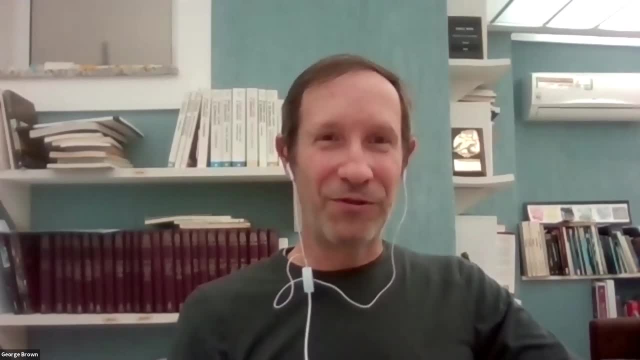 that you're going to be exposed to things that you're not used to, to a language you're not accustomed to, you don't know very well, and that involves not just the policy but the land manager often, because, if you know, it's not like elizabeth, where you come from a farm background, or i actually 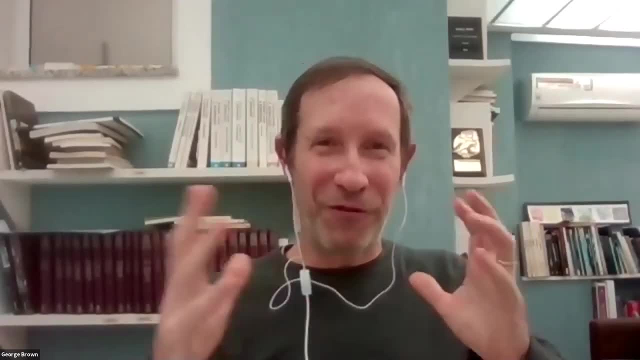 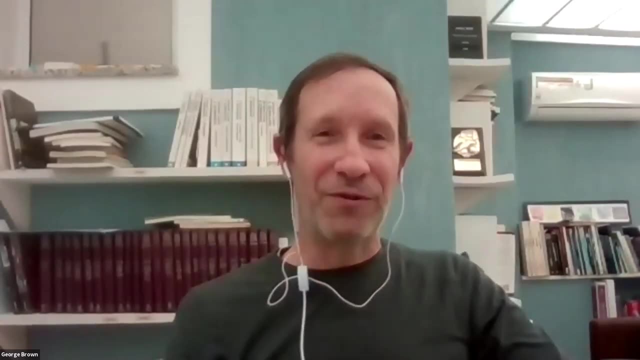 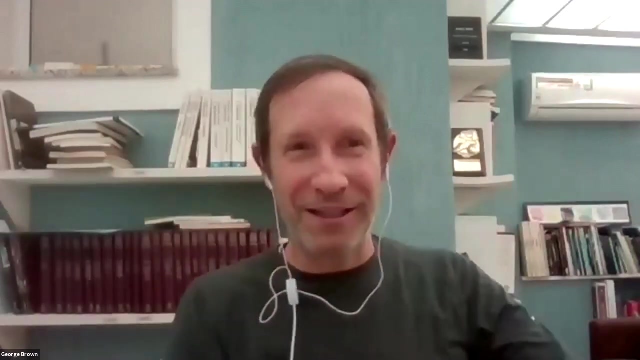 was grown, grew up in a rural background, so it's okay, but for those who don't, it is really learning how to communicate and how to say to somebody the importance of what you're doing and why you should care about it. so i think that is- uh- maybe not, you know- a global, big, humongous, uh barrier, but it has to do personally with us. 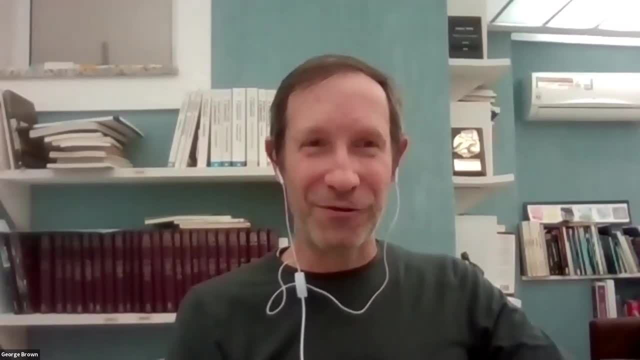 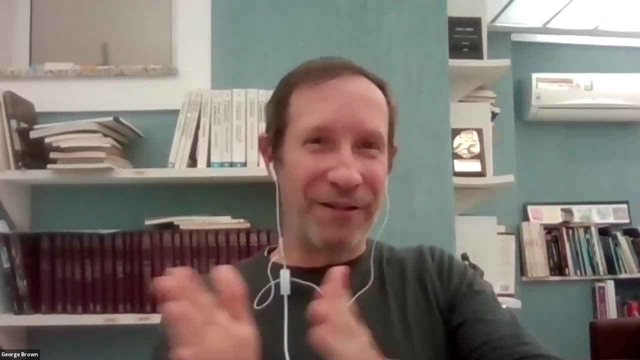 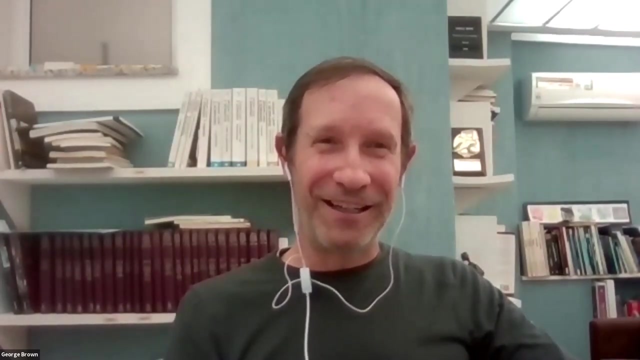 i think, as many of us who are listening and speaking now, our scientists, who are maybe used to a particular uh- vein of of work, it's. it really means getting on a different train and boarding on to it and and saying, okay, here i go, you know, and and and getting, getting any getting. 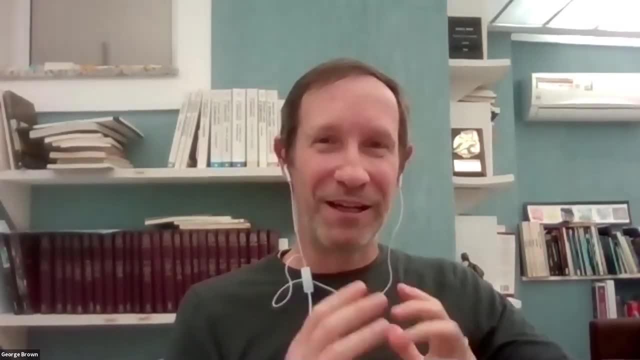 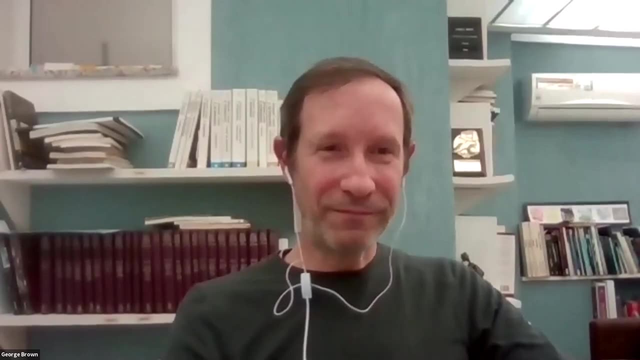 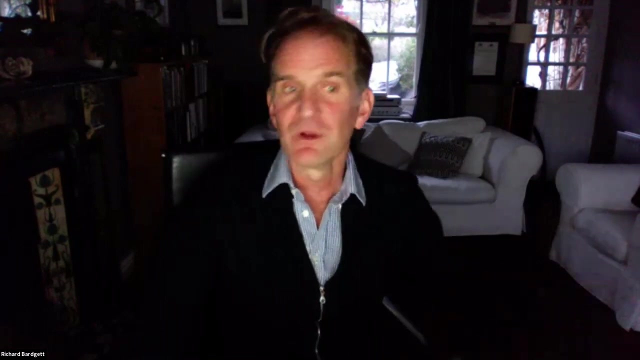 a challenge and going forward and just keep going forward, because i think that we are a voice that needs to be heard and that uh has things, important things, to say. so the message from all of you is to get out there and communicate uh the importance of diversity to users and demonstrate how that 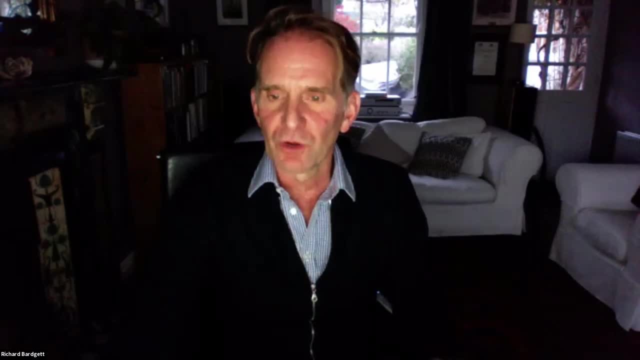 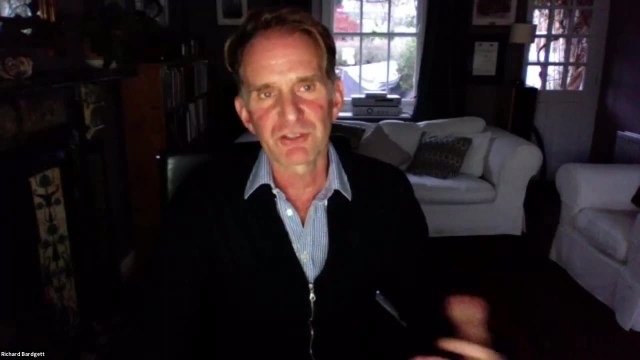 can be. um, i i'm. i am very aware that we're running short of time, um, but there are two areas that i just want to explore before the end. one is more about how you measure diversity in the soil. i mean, all of us have talked and many of us give talks telling people. 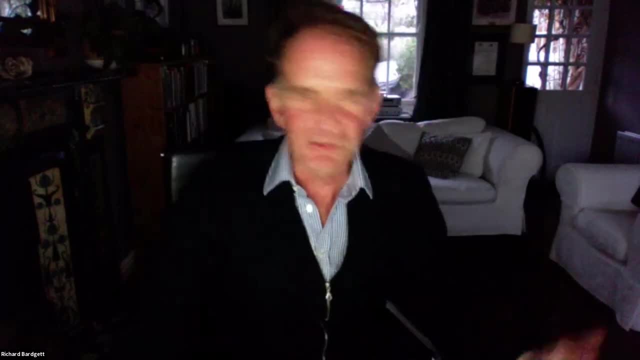 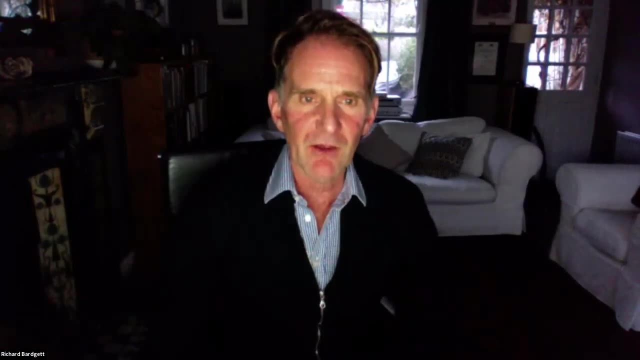 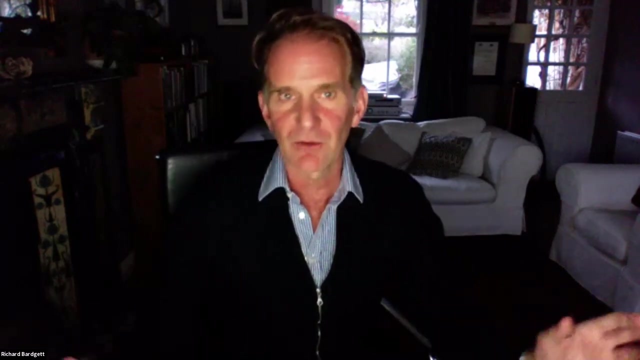 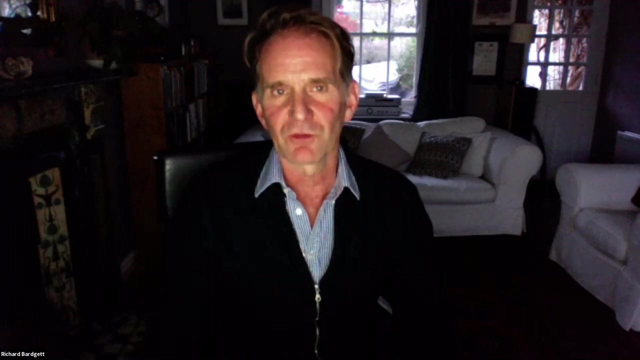 about how diverse and incredibly the number of species in a handful of soil, etc. so that raises the question: if we're trying to communicate with landowners, farmers, about how on earth do you measure that diversity of soil in a meaningful way to give you any indication of how healthy their soil is? so, again, i i quite like everyone's perspectives on this. so 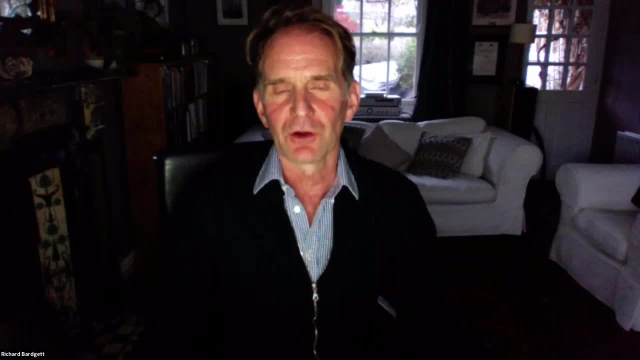 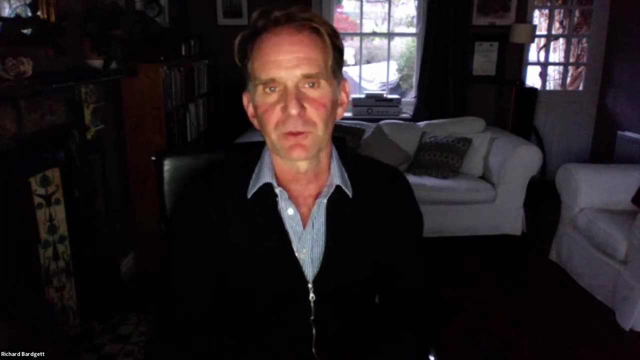 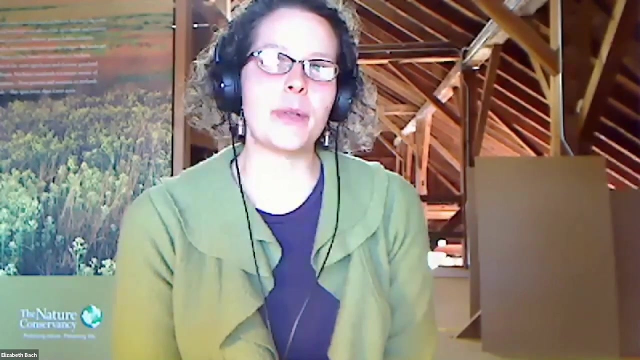 i ask you to give a very sort of short answer because we don't have too long about. you know how? how do we best use soil organisms to measure the health of soil? and i'm going to start with elizabeth. oh, that's a great question, um, and it's, it's a really important question. on on the one, 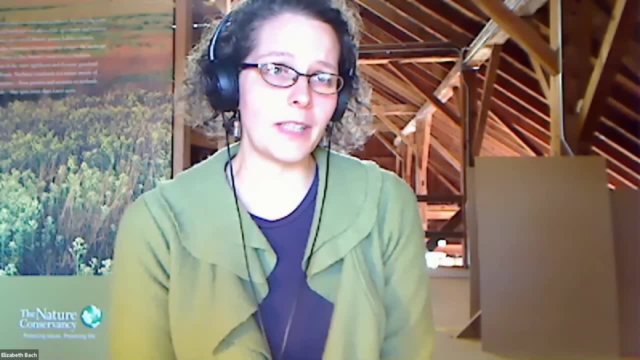 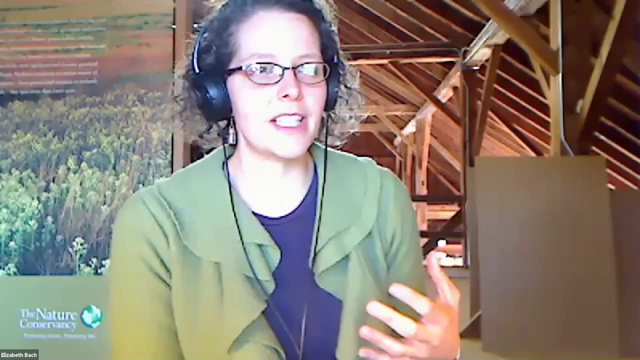 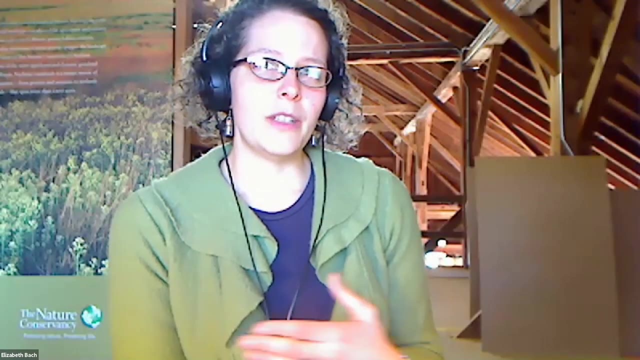 hand, there's a lot of very technical things we can do in the laboratory to really explore and understand that. um, i think some of these efforts that kelly mentioned about scientists leveraging people sending soils from their backyards or their their local areas- are really opening the door to these um measurements. um, that can do sequencing. 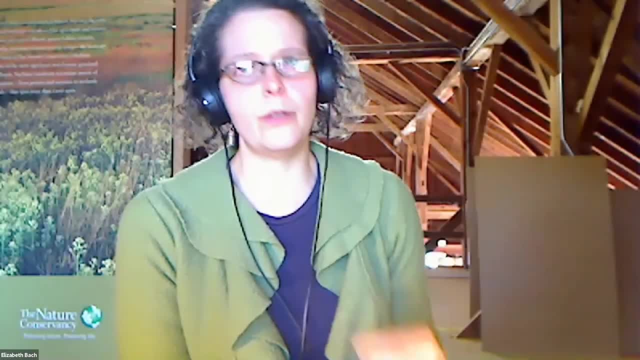 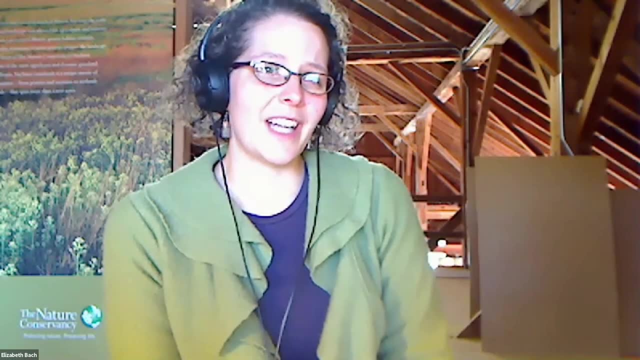 measurements in the laboratory or or bring them to an expert who can, who can, analyze these communities is really important, um, and it would be, i guess. i would love to see something in soil ecology similar to what i naturalist has done above ground, where folks can be, you know, even just sending um. 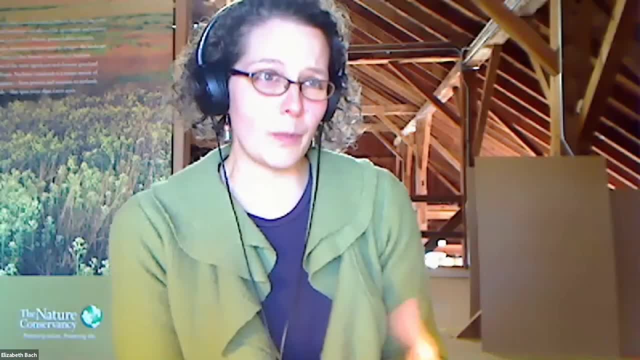 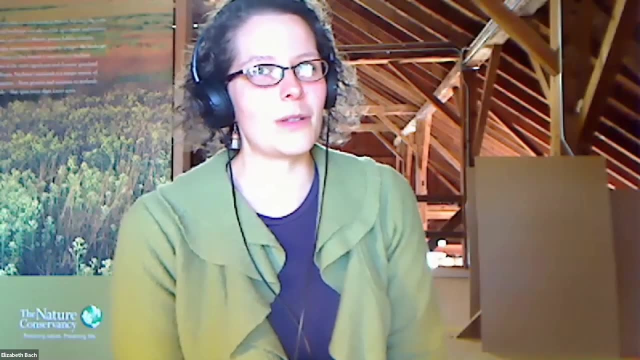 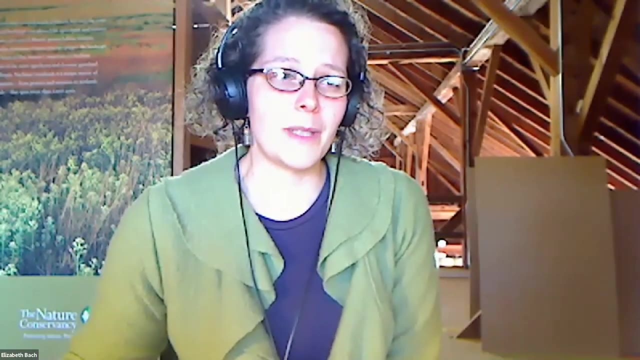 electronic snapshots or uploading. i saw this worm, or i saw this bug crawling around or this. you know this larvae, this grub and and uh, really opening the doors that way. um, but it's really difficult. i don't think there's one measurement that works. i think we have to look at a variety of measurements. 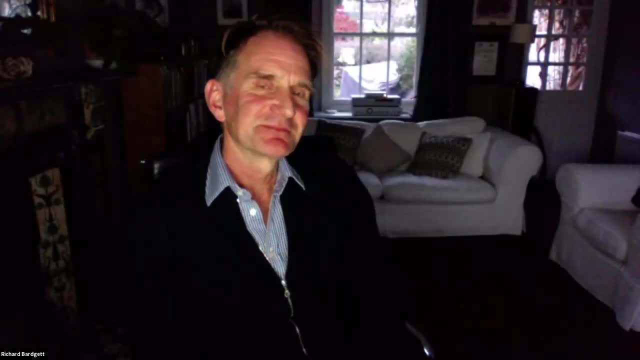 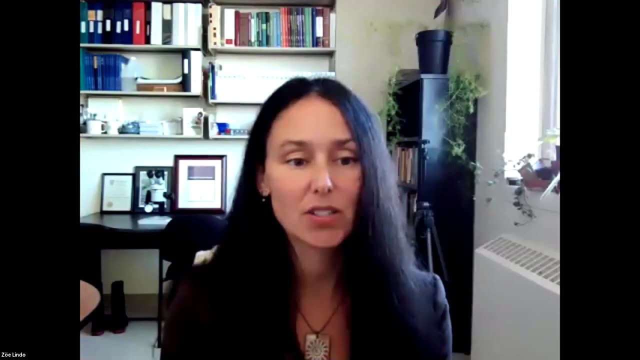 okay. so, zoe, i agree, there's definitely not not one measurement that works, and uh, part of this is is related to- as as i mentioned in my talk, the uh, the fact that soil organisms span multiple orders of magnitude in terms of their body size, so one type of sampling for one type of organism is definitely 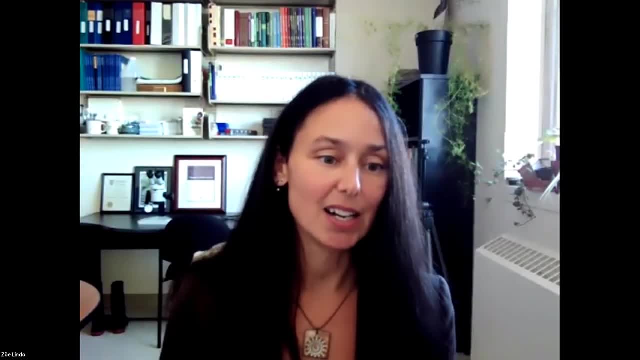 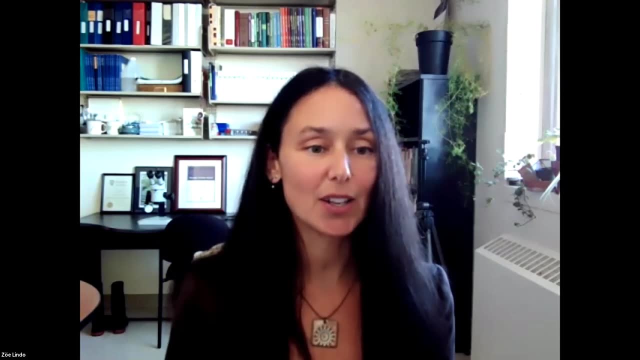 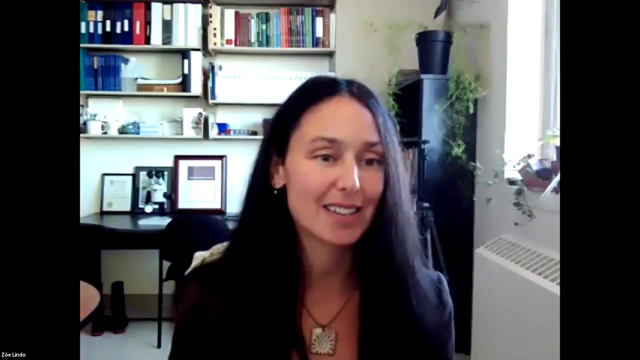 not going to work for another type of organism. um, for me personally, i'm i'm heavily rooted in in taxonomy. um, part of my interest in taxonomy is that i'm very visual. i get to see the organisms and i have an inherent interest in them. i think they're, they're, they're. 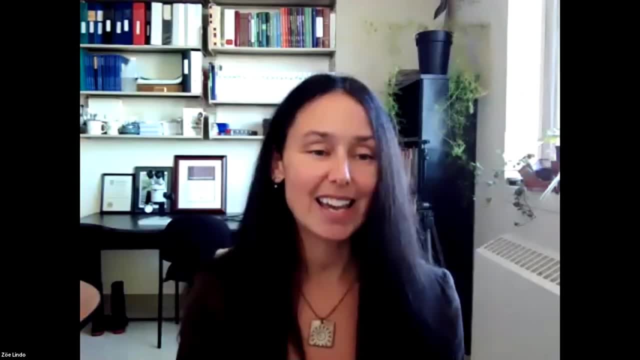 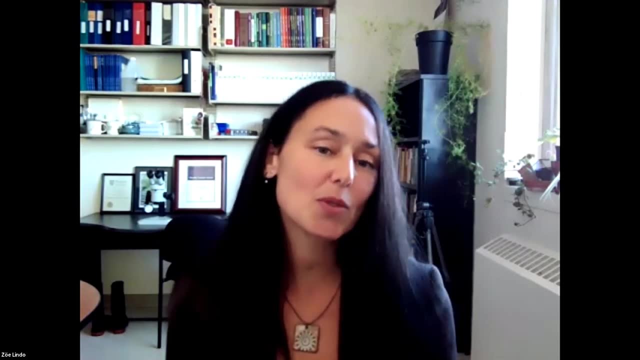 cute or they're beautiful or they're funny or they're interesting, and that's what keeps me interested. but that obviously doesn't work for some of the some, some of the other soil organisms, and that's where i think we're. we're making great strides in things like e-dna techniques. 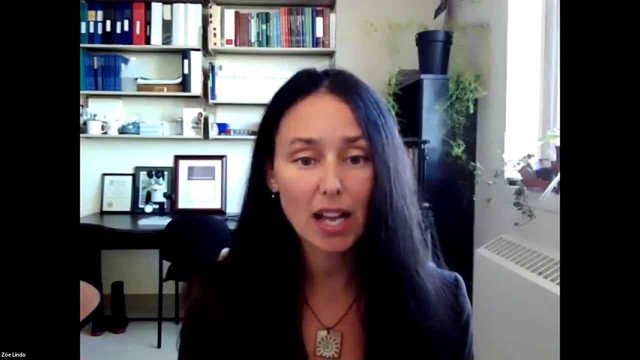 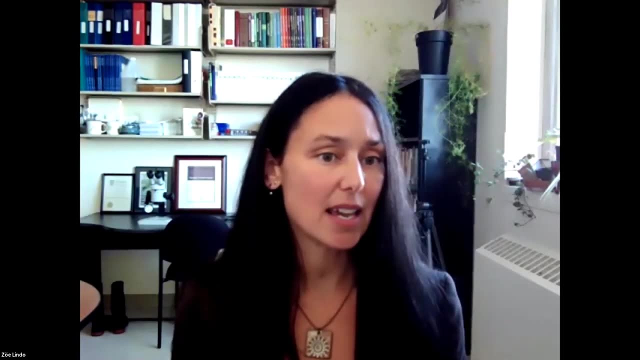 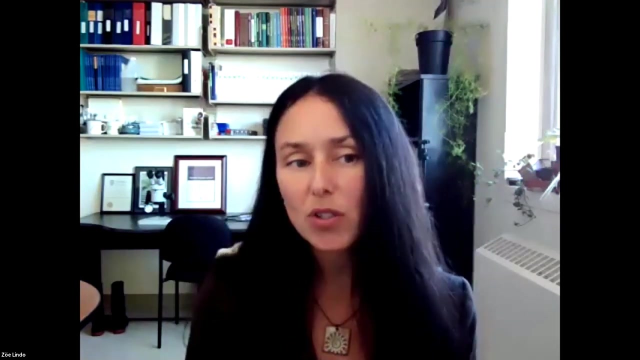 and uh also considering, again coming back to functionality, so functional diversity and some of those indirect measures, whether it's uh, enzyme assays and um, carbon use efficiencies, eco plate type, uh type assessments and things like that- that can be done without the highly skilled taxonomic information as well. so i think there's a variety of approaches to study soil. 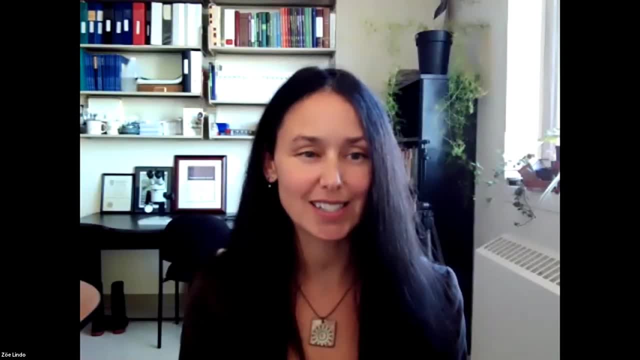 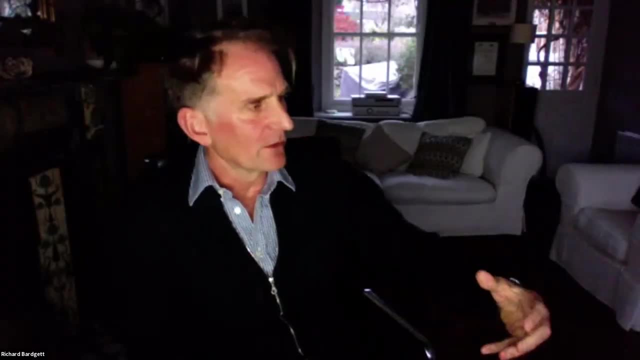 biodiversity, and i think it depends also on what your question is, what you want to know about it. okay, i mean, one of the things that uh occurs to me when, when we're talking about these things as well, is: not everyone has the capacity to measure all these things as well, and we're 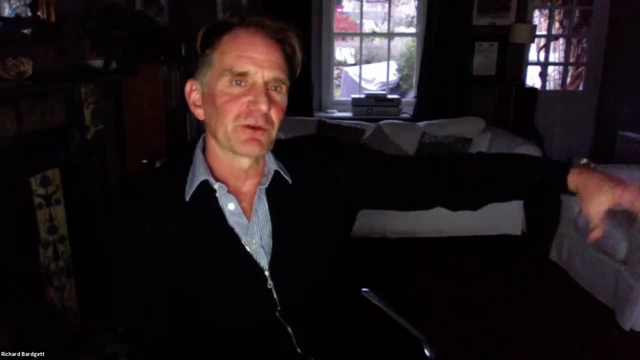 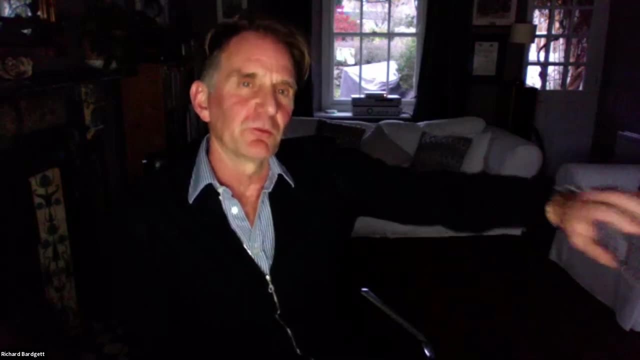 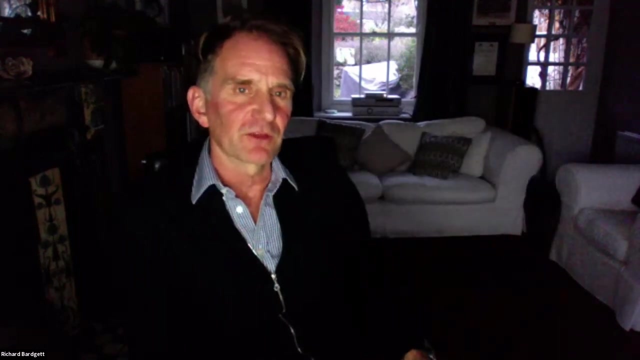 talking about communicating with farmers, landowners, often in places where they won't have that uh technology available. so i'm gonna ask george again that question, but with that in mind, about what measures they can do now to actually get some indication of the health of their soil, and then i'll come finally together. yes, um, that's. 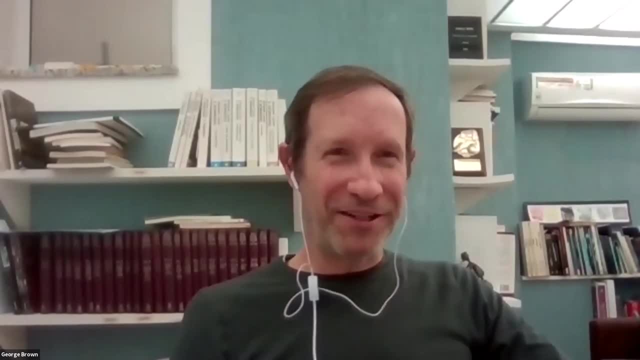 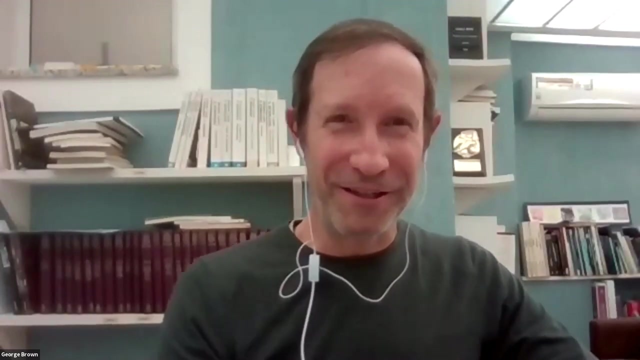 true, uh, we we see a lot of great uh publications and papers going really deep into the sequencing era and we find that, of course, uh, that's quite difficult for many people to understand, uh, sometimes even ourselves, if you're not trained in in the particular genetics and you know metagenomics and stuff. 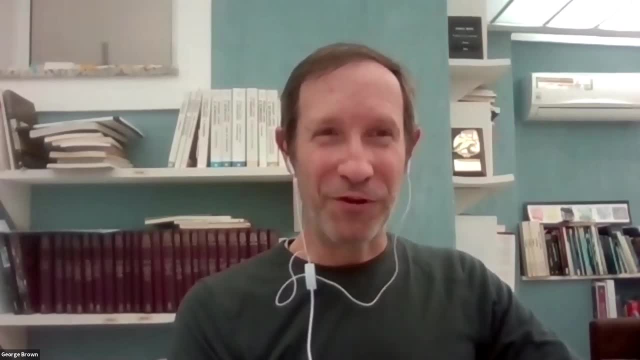 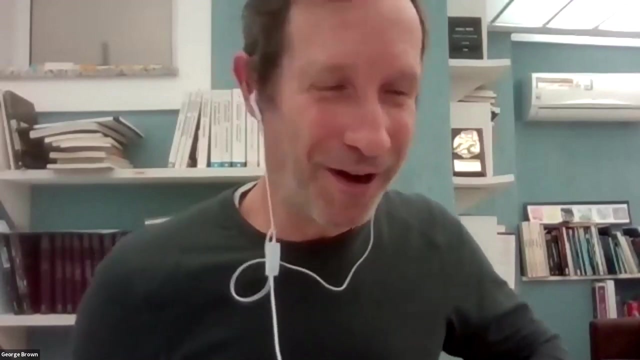 like that, so it can be a also a completely different world, which is even harder sometimes to communicate to the land user and a man manager. i think that you know, in the situation of how to measure and what to measure, if we're going to be easy, uh on, on the people who are, who are actually 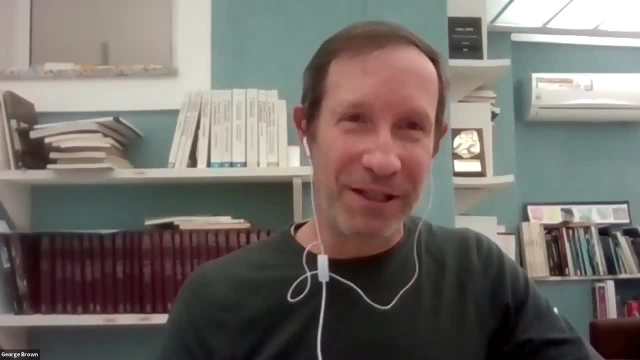 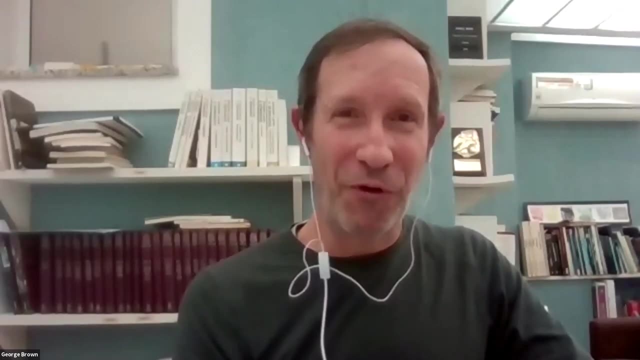 out there. they're different. you know they're, they're, they're, they're, they're, they're, they're different ways of communicating that. you know you could have the sample sent to the lab even if, if you're out there with a farmer, um many ways they can, they can, they sometimes got to be frozen. so 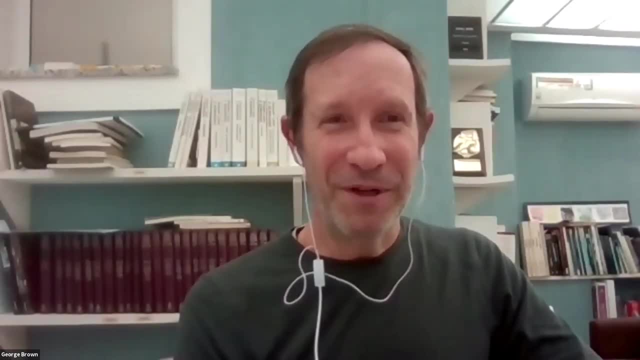 there's a whole question of logistics, of how to do some of these things, but you know um easy measures that are easily visible, easily performable and particularly something that the farmer or the land manager himself or herself can, can do, are, of course, preferable, uh, in in the sense that 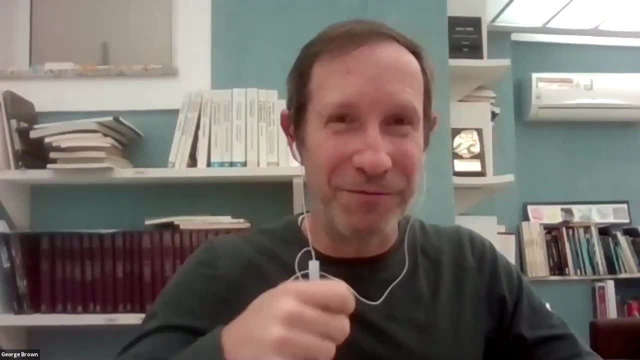 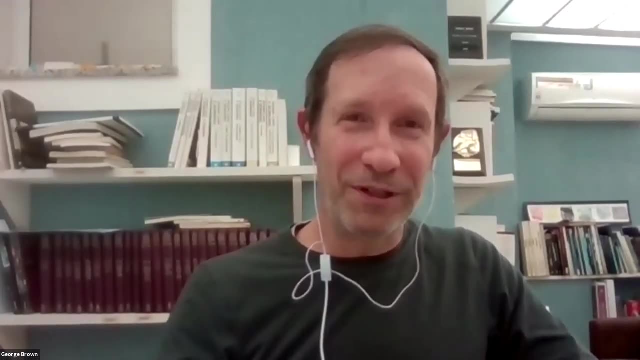 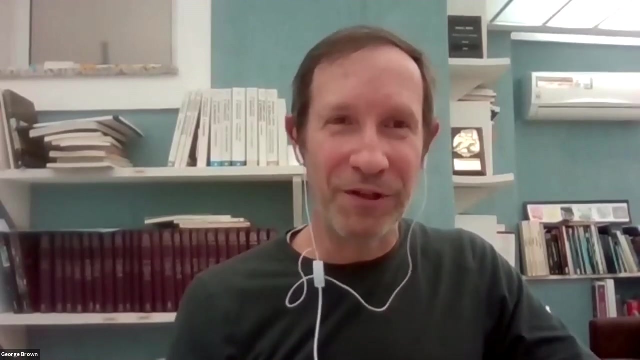 you know, if there's even just a regular uh, you know, a magnifying glass or a scope that you can take and that you can provide, uh is a whole world opened to, to many of these people, and so i think that there are simple things that we can do and that we often do in the field here in brazil. 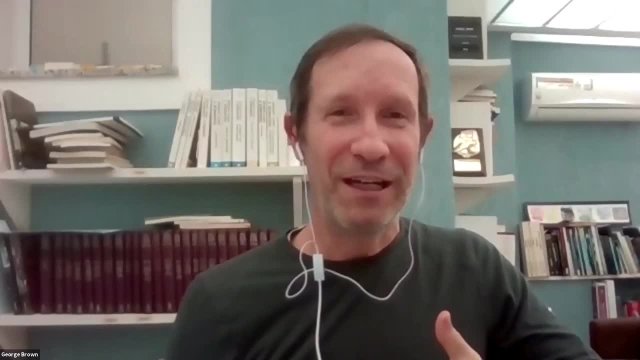 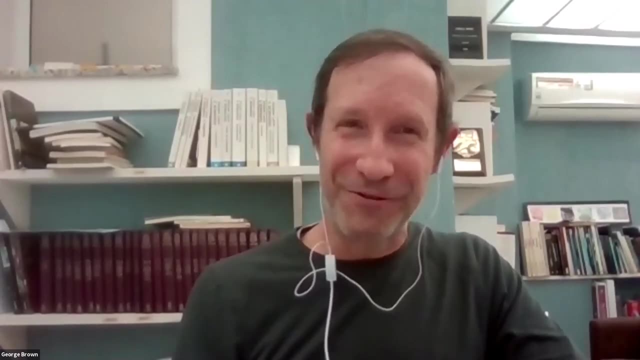 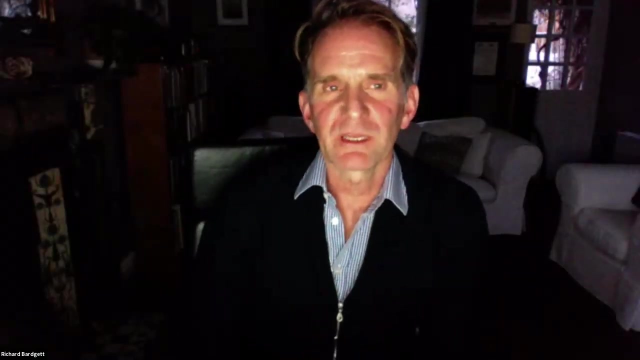 that do reveal the soil biodiversity and that they're quite easy to measure, and i think those in situations where you don't have access to all of these great tech things are are really quite, quite good. okay, i'm aware that we've only got two minutes left and 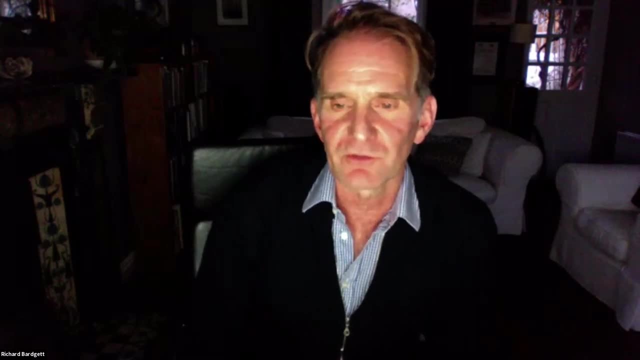 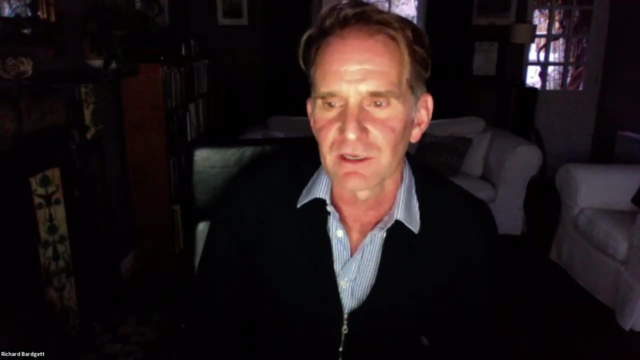 there is a burning question that i want to ask all of you, and it's a very quick question, and this is one from anya krieger. uh, so i'm just gonna ask you all very quickly, because we've only got, uh, one minute left before i wrap things up, and it's what? what's your favorite soil organism? 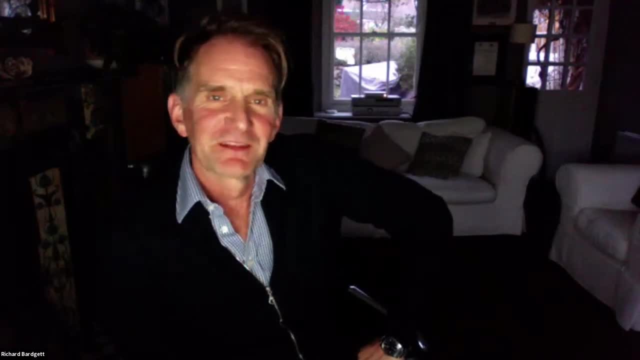 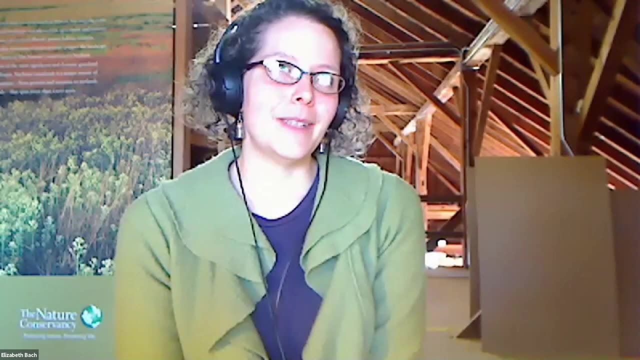 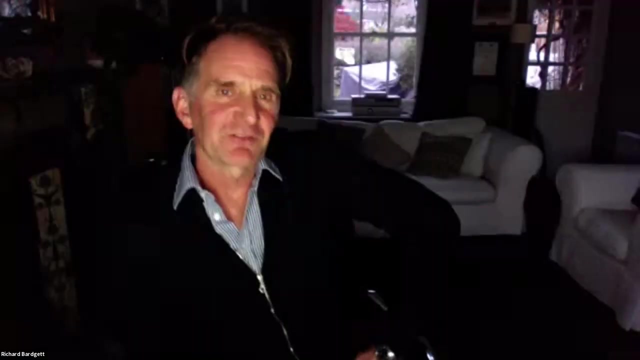 and i can start with elizabeth: um, it's always her to choose. i think my favorite soil organism is probably um an arbuscular mycorrhizal fungi, because i feel like they just do so much um, and there's such a big network in the soil. okay, zoe.